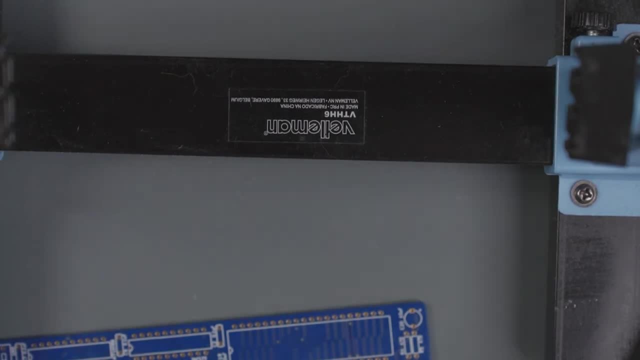 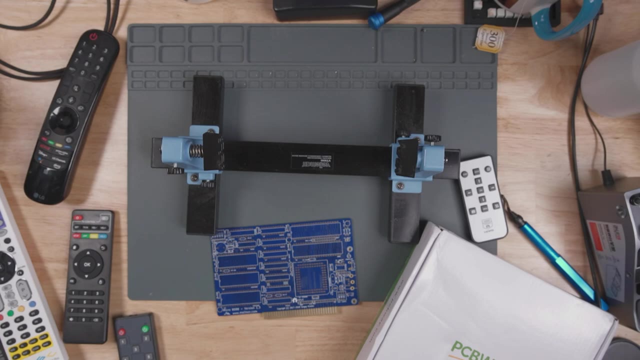 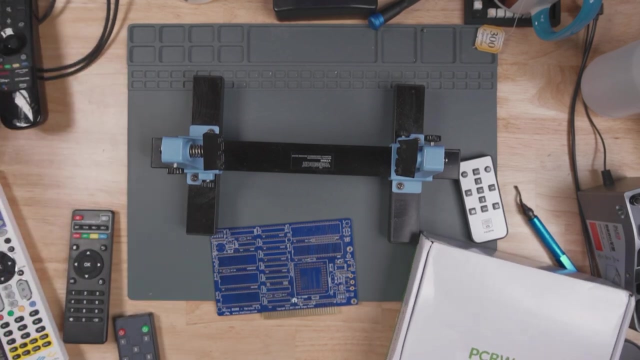 let me put this up there. Well, this is going to be kind of a difficult Okay thing, and not really. but um, yeah, I've just got a bunch of stuff on my, my, my desk. I've been 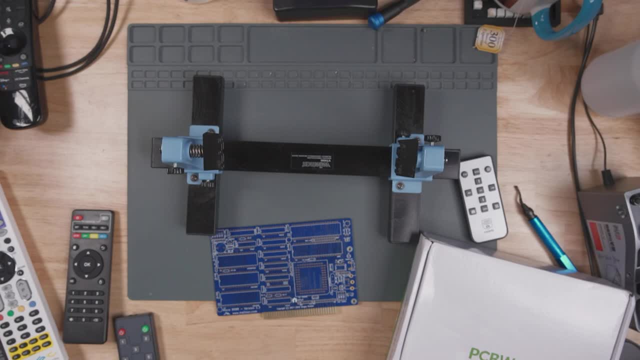 kind of trying to clean. uh, I'm just giving my iPhone app one more try. hmm, there's some weird. there's some weird thing we could try. I know, uh, I'll be with you guys as far as what we're doing tonight in a second. but let's see, what was this called? OBS cam. 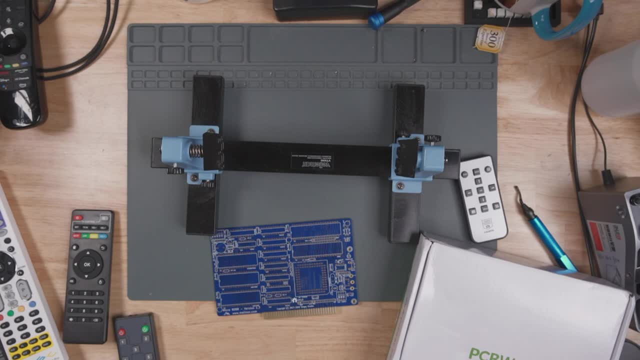 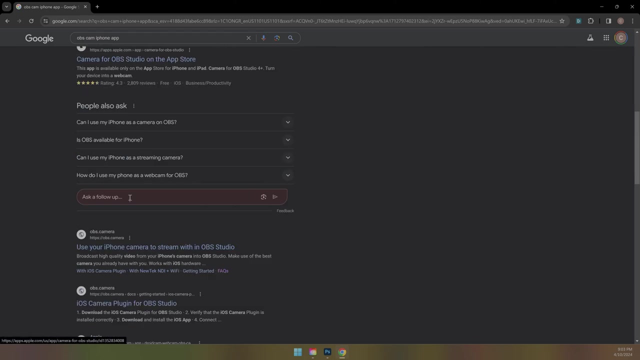 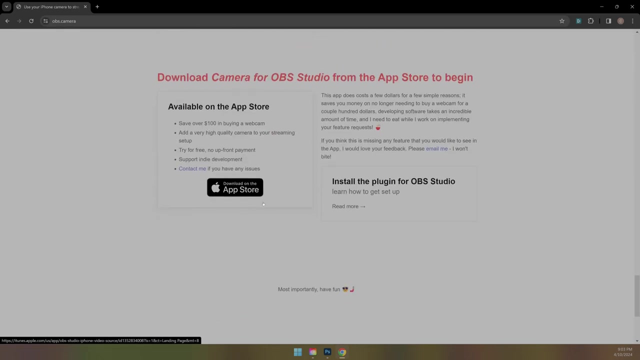 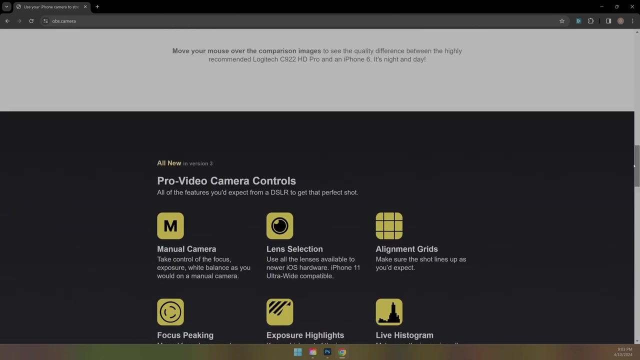 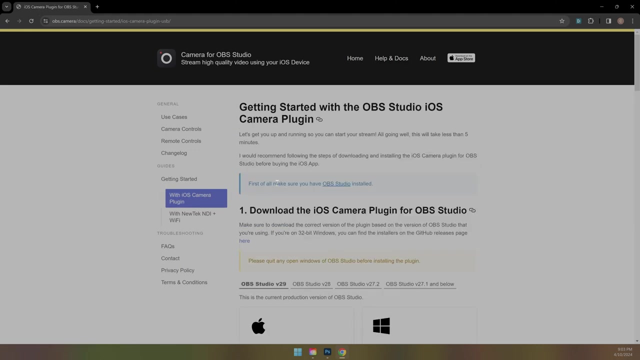 iPhone app. um, then we can do this. uh, this. there's like a weird. where is there like a wiki or something? docs helping, docs. okay, USB. all right, we downloaded the plugin, did this. I have iTunes running. 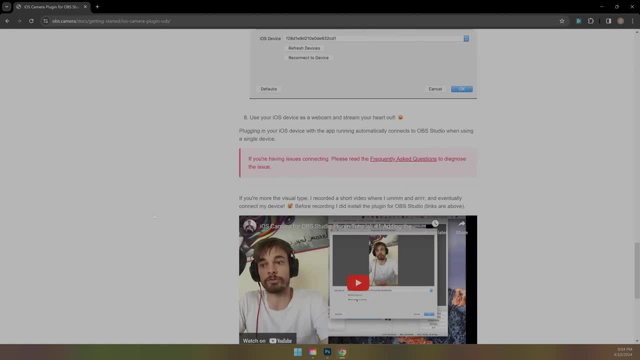 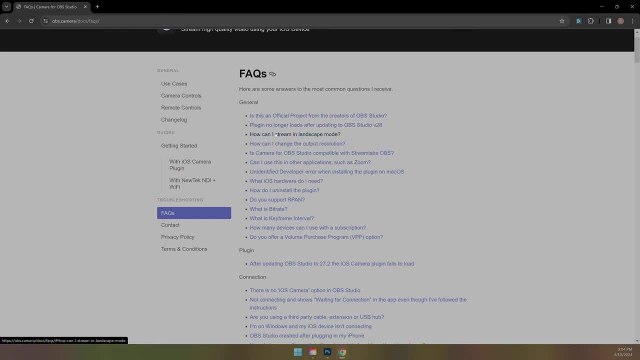 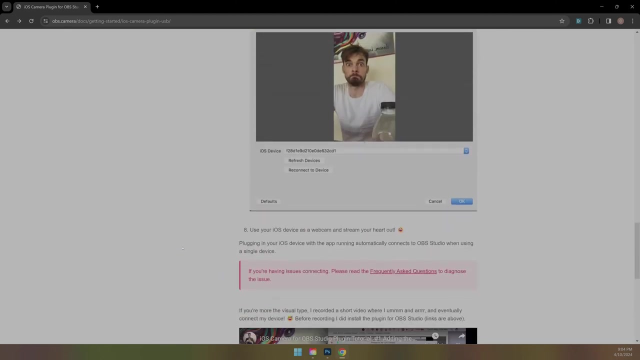 uh, there's like a magical um list that works every time. if you're having issues connecting this plugin no longer loads, I'm gonna stream change. nope, go back. uh, this is cringe, I'm sorry, guys. 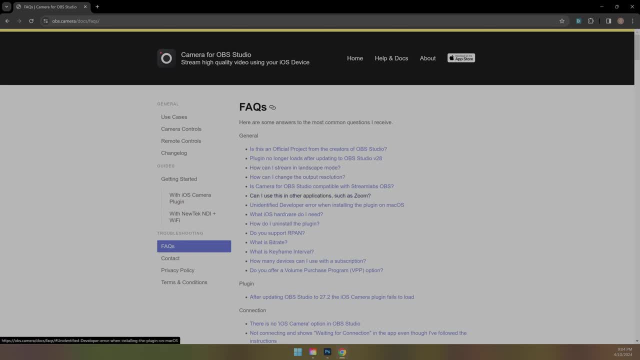 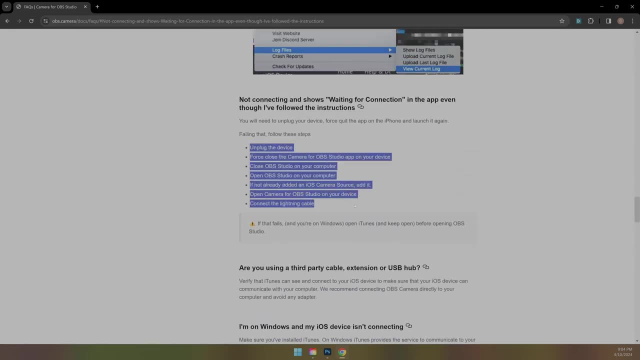 uh, there's no connection, waiting for connection. okay, this, this stupid thing. list of things. well, I can't close. I can't close OBS studio- whoops. but I can close the camera app and I can't reopen it. so, hey, it's already open. okay, now. now we open this app on the phone. 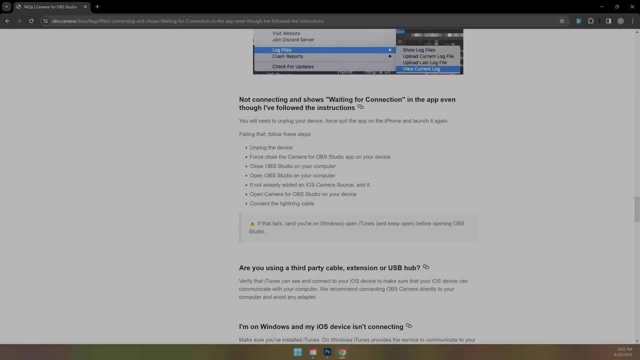 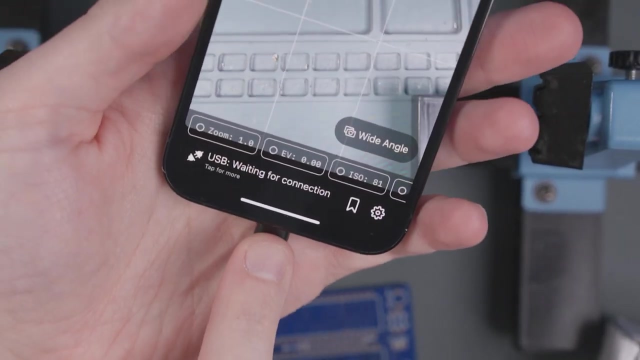 and now we plug it in? no, absolutely not. why would that work? okay, this is what I'm talking about. wait a minute. oh, I have this app and it has this. it's basically just a USB through the thunderbolt. 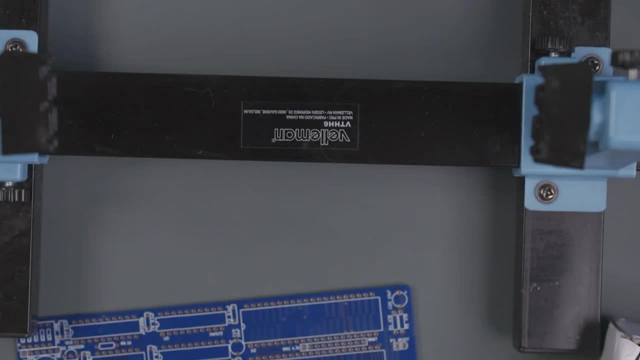 geez, it'd be funny to work now, but sometimes it just it just doesn't connect, and this is waiting for connection, even though it's connected, and so this is like weird dance you have to do. 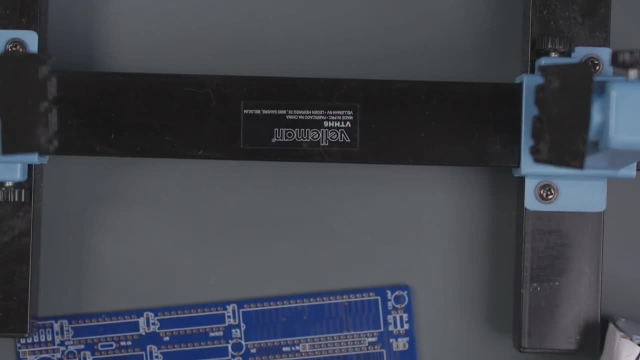 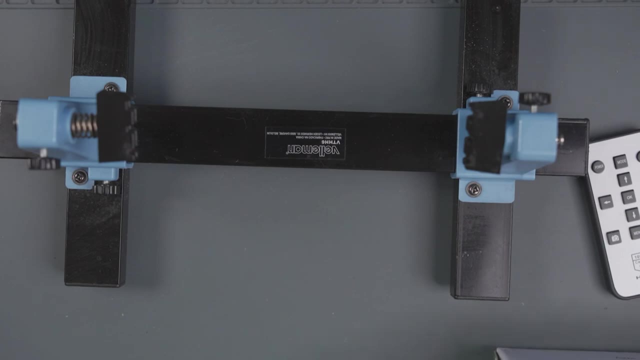 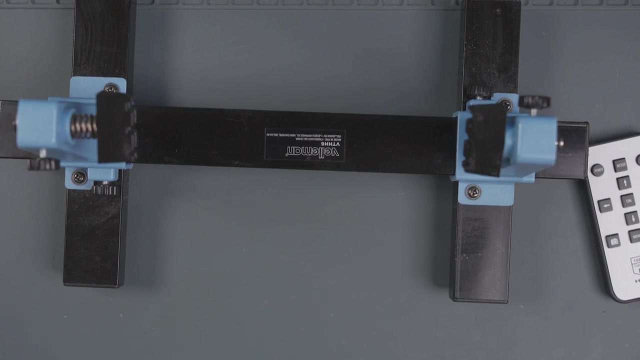 with having iTunes installed and this and that. well, whatever we're winging it, sorry about that, I gotta figure out a better solution. um, all right, so hello everyone. hope everyone is doing well. I know this is a a different stream than normal or than the usual recently. 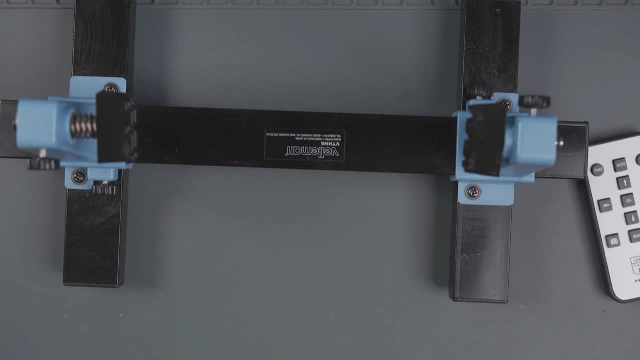 I suppose with the Morph stuff, which is fine. um, guess I'll just take a little break and um, you know, I I've already said that my one of my goals this year is to finish this whole project. 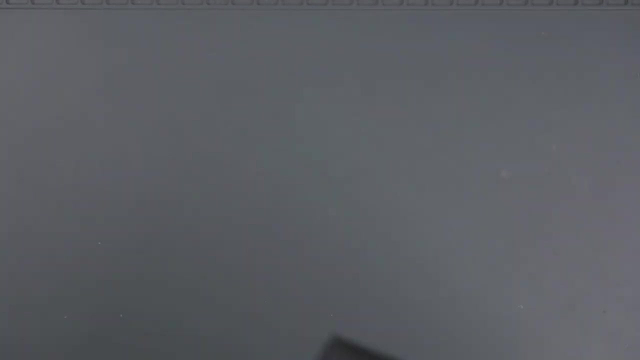 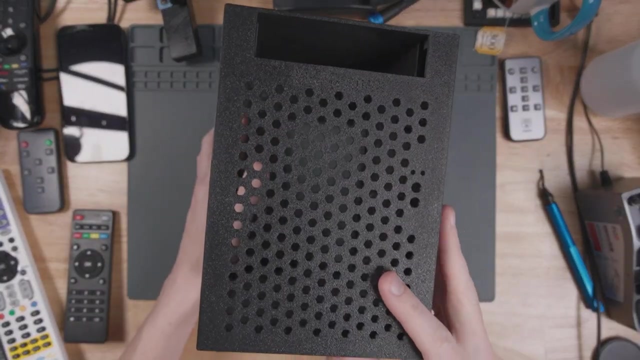 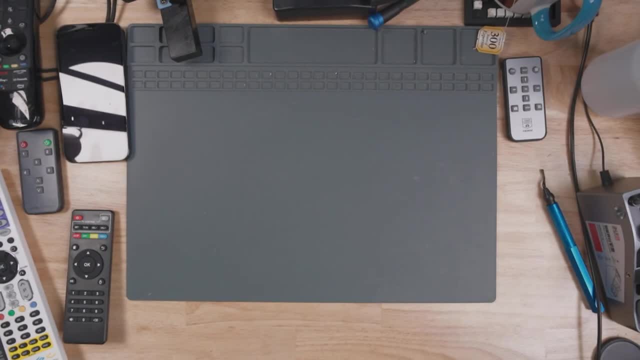 I guess we'll do that. we might as well do that now, since I can't really uh, use, show my face or anything. uh, well, you know, what should I also talk about? well, maybe we'll do that at the. 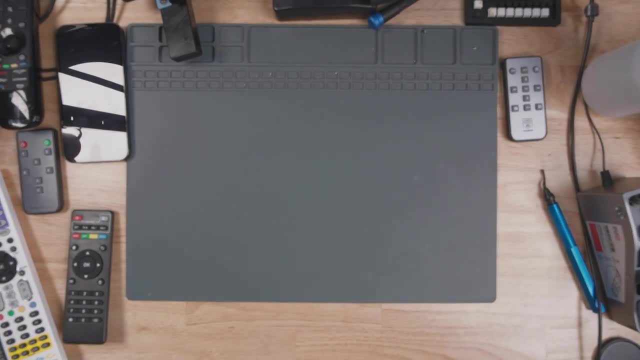 end. I did manage to watch a little bit of um Voltar's Morph video and I guess I'll say that, um, well, I don't feel it was. maybe 100%. um, what's the word I'm looking for? independent? 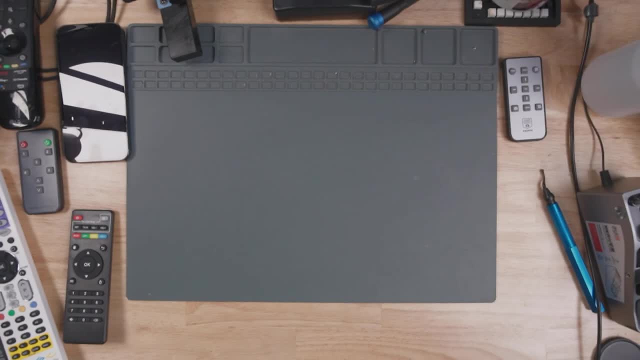 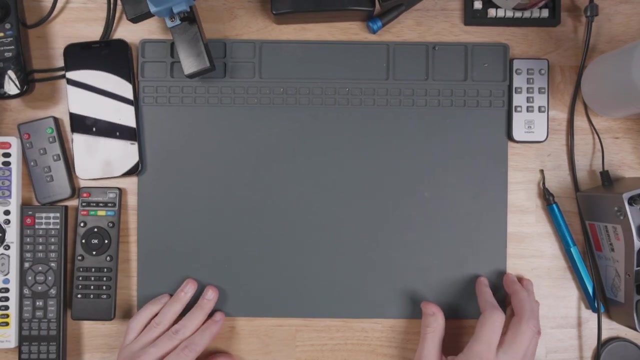 um, it was fine. like you know, I understand that there's some some uh hard feelings- not hard feelings, but just you know there's not unpleasantness between them and pixel effects- but I think overall he was giving his best attempt. that's what it looked like to me. 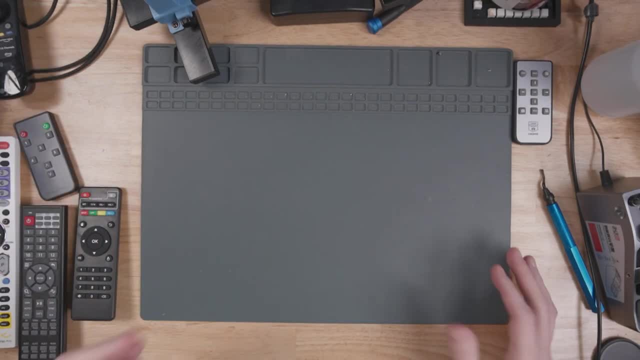 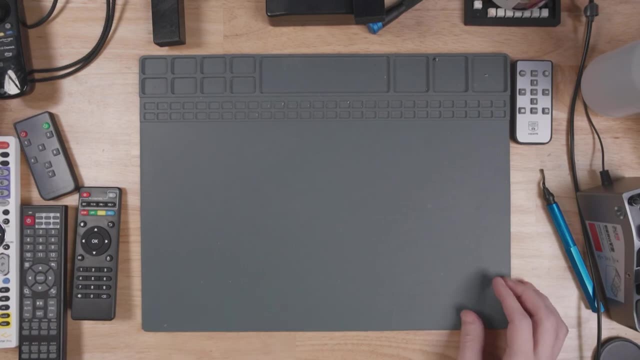 as far as um trying to- and I don't really like how he called it a review- I don't really think you can review something. I mean, this is just a nitpick, but I don't really think you can review. 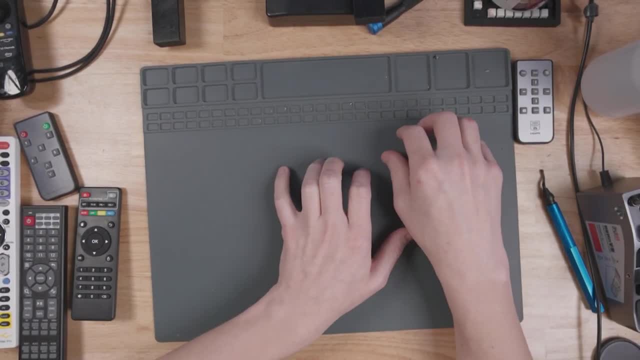 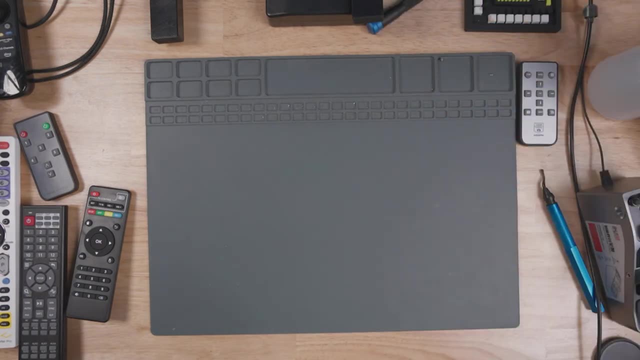 something. I don't know how long he's had it for, but, um, he was kind of doing what I was doing, you know, just just um testing different consoles and things. I also have some tea, uh, and you know, just giving you know when things can't went. 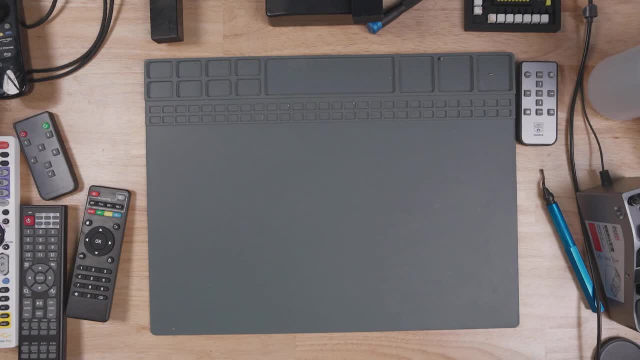 wrong in certain circumstances, then he would just talk about that. so, yeah I, I it's, it was fine, um, but you know I'll watch more of it. I did take a few notes, I don't know. we'll talk about it at the end, I suppose. hey, Ian, how you doing. 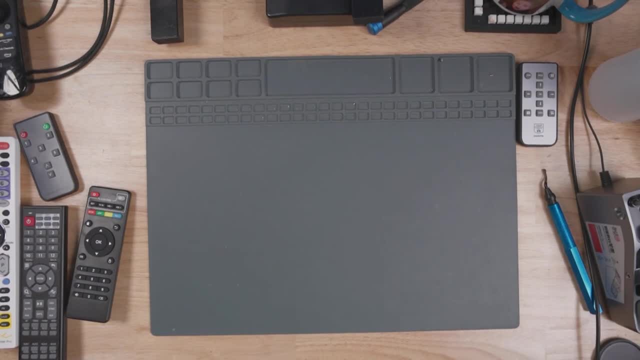 um, all right, um, let me pick up. uh, let me get the documentation here going. I don't remember where I even first stopped. I'm kind of uh, not freaked out, but like the, my face cam not working is making me a little not happy. so, um, let me find so. 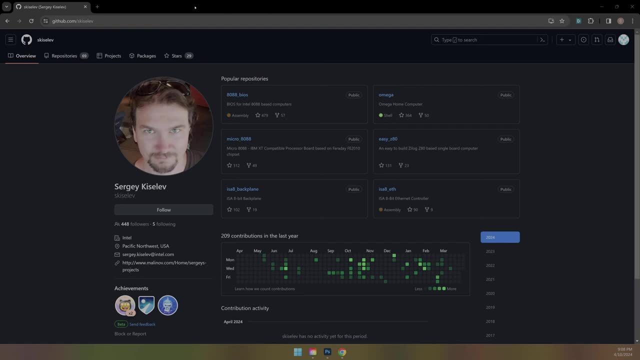 let me go to here. okay, so this is the, the person, um, that is behind this whole project, and now, if you go to their GitHub, there's a ton of different, uh, repositories, so we'll kind of go over what I. 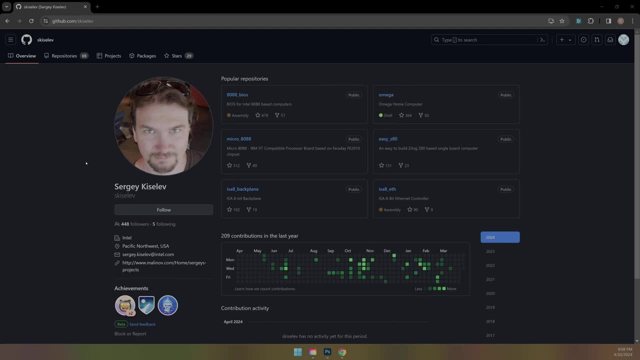 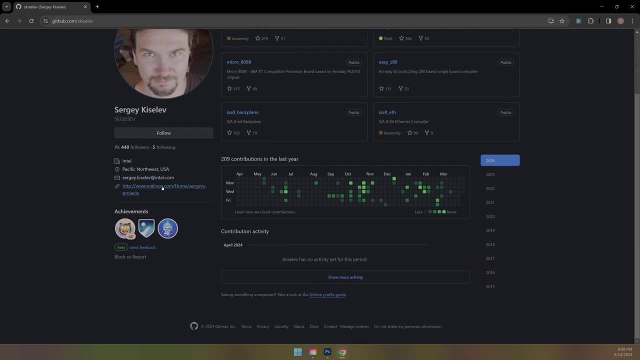 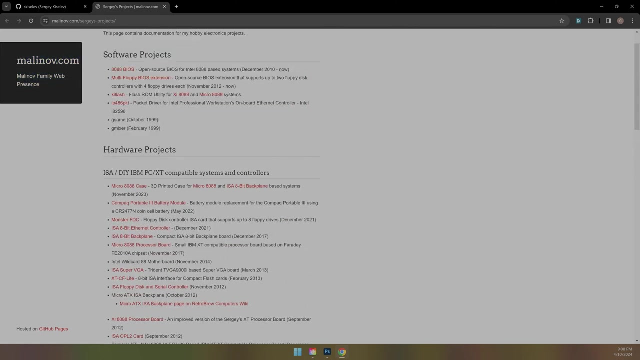 think is this kind of collection of uh of being one project, but Sergei Kisilov and I couldn't find their Twitter or anything. if they had a Twitter, they do have their own website. maybe that's what I saw. uh, anyways, these like this is kind of like a list of um, the products that 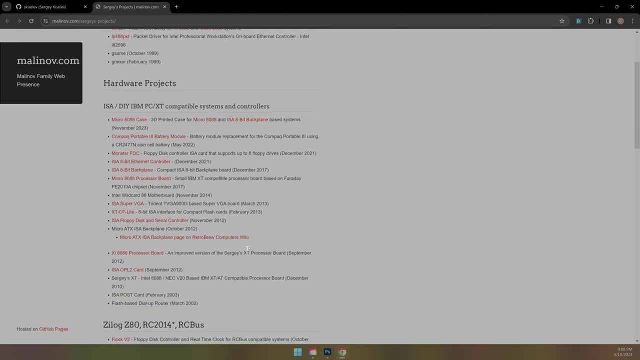 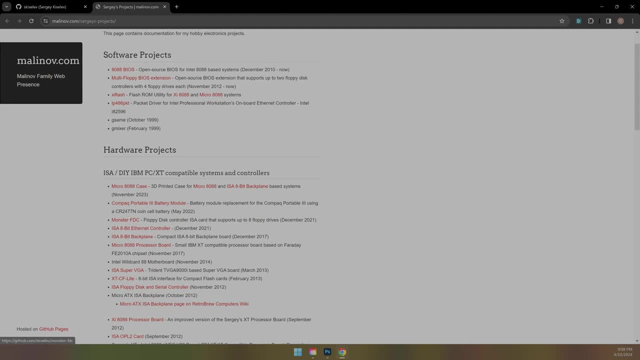 they're working on more like they're in a a like a date order, right like things they've worked on recently and back um. so it's possible that I've I've heard of this monster floppy disk controller. 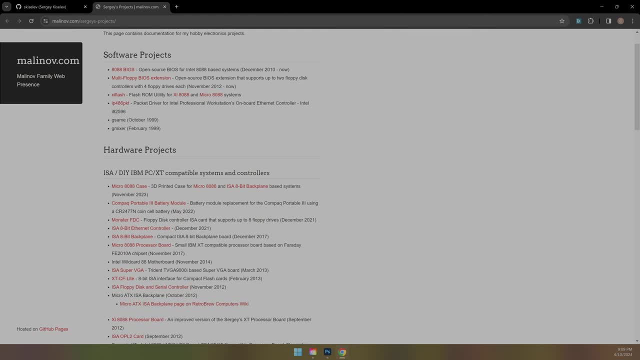 thing. so it's possible that I got to there from here. uh, I think also in the past I was looking up at least some XTIDE, uh stuff so they they might have an XTIDE. um, I got an old Merlin's. 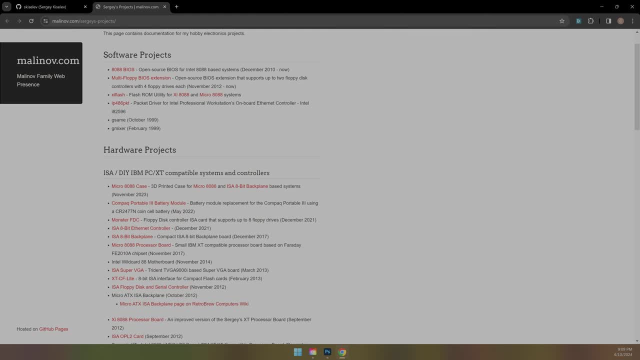 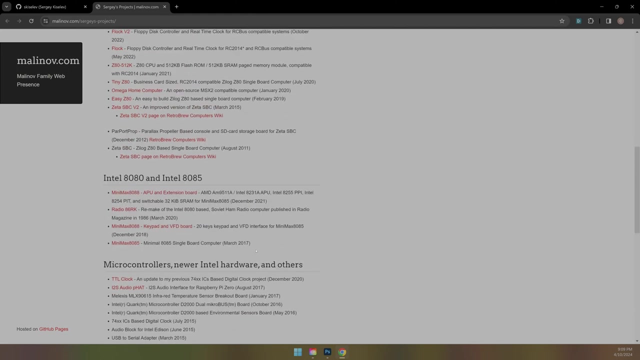 says I got an old Toshiba Satellite laptop and have been running DOS and DOS games on it has been brought, has brought back some great memories. 8088 built looks interesting, yeah. so I think, uh, this is going to be kind of an- I hate to say- introduction, because I really think that if you 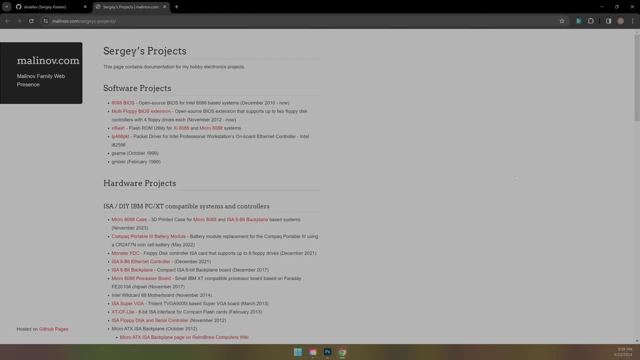 are trying to get into retro games, then older is not better. uh like, if you, if, at least if you were not in the time period or you didn't grow up in the time period, you're not going to be. 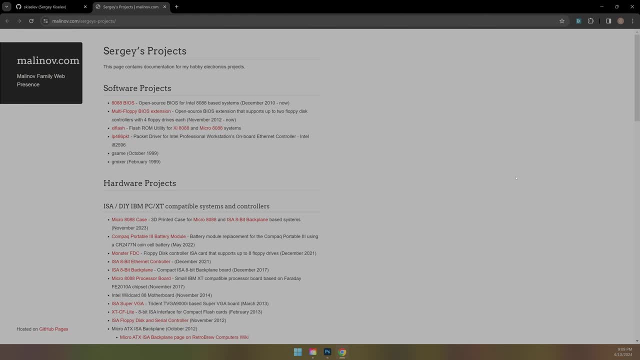 in the time period when these, um, when at least this particular type of computer, so like IBM PC and XT class machines like I, was not alive even, uh, in this most of this decade. actually, I was. 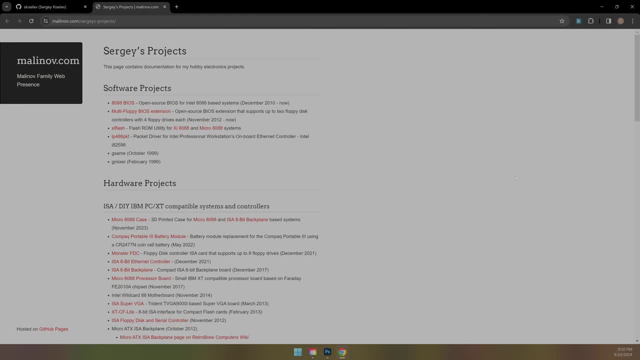 born six days into the- or it was six days into uh left of 1989, I was born on December 24th 1989, so did I just dox myself, Uh, oh well, anyway, so it kind of gives you, I like I've. 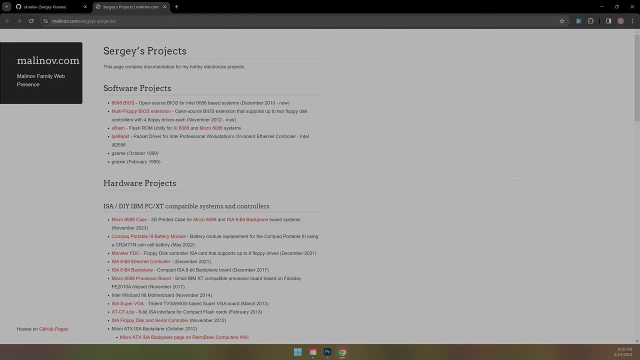 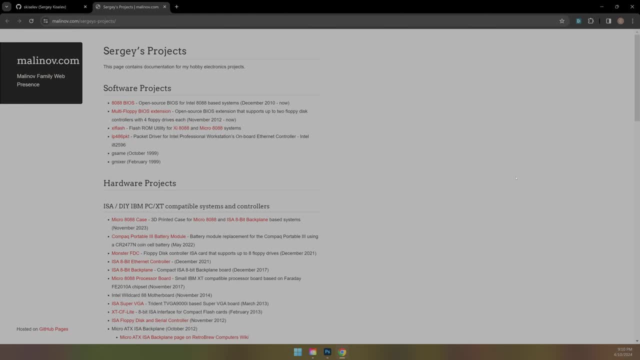 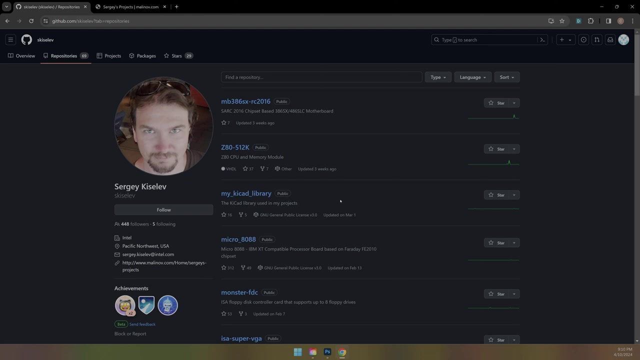 uh, all right, so I guess I'll try to talk about, um, let me find that picture and I'll. it kind of shows the whole kind of setup. uh, maybe it's one of these repositories, it that. that's one of the gripes that I would say about this whole thing. 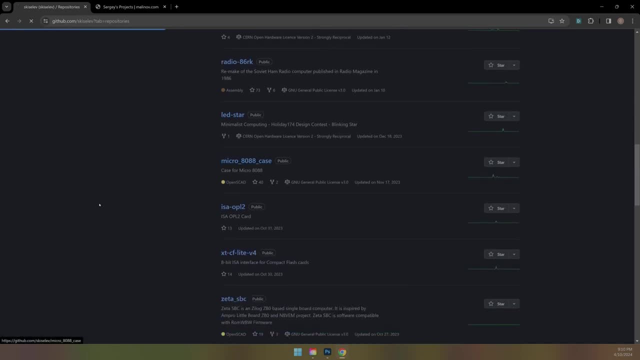 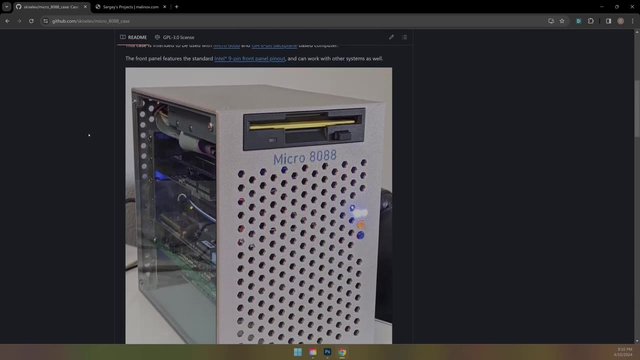 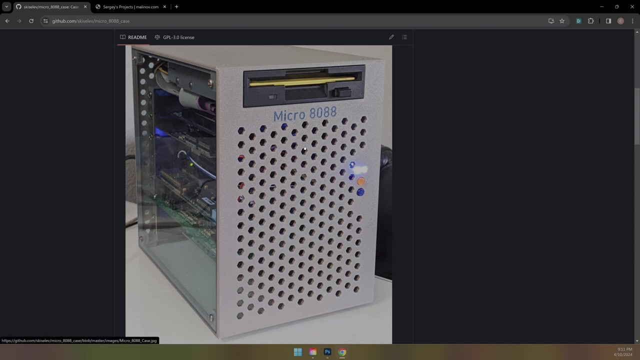 is: uh, here it is. the case is that it may be a little disorganized because it is multiple different um projects instead of like one kind of lead thing. so here's a, a cool picture of a, a finished product and um. you know, there's sort of the ability to put like 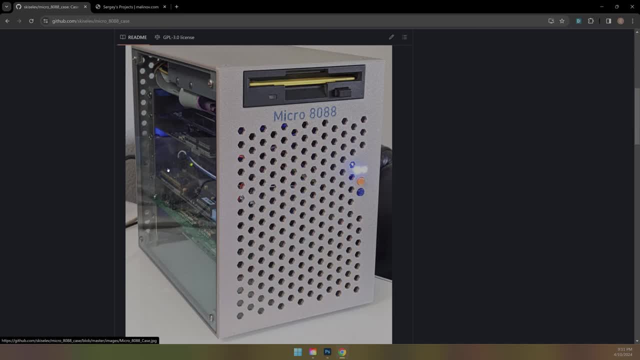 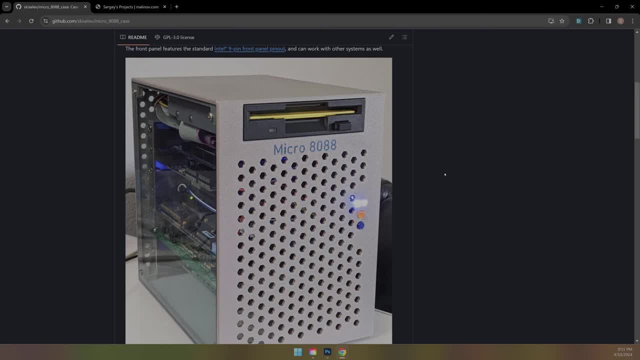 the same hardware as a um IBM XT and an AT. so we'll talk about what that is. um, I guess we'll talk about what that is first. so I, alright, maybe we'll talk about. so when I started getting back into retro stuff kind of more recently, I, I, I can't, I can't. 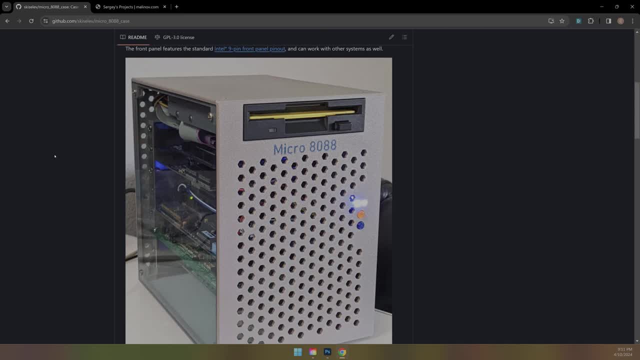 show you my face, because I my face, my webcam's dead. I could plug in this old piece of garbage. wait a minute. uh, okay, except for I don't have any more USB ports. well, this is a problem. oh, I can't plug that because that didn't work. yeah, hold. 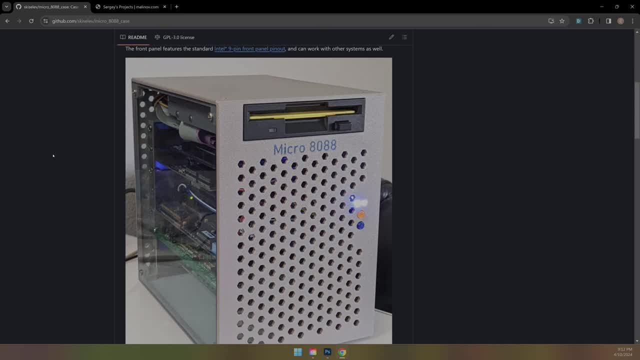 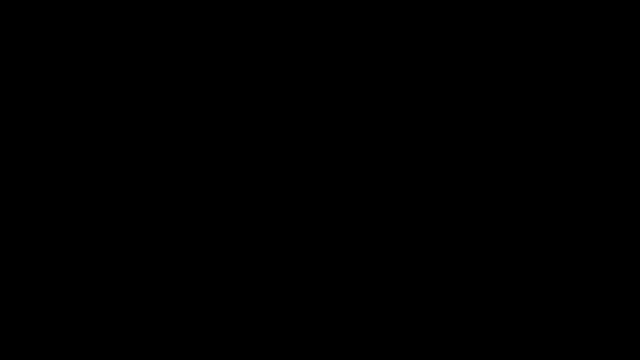 on hold that thought hello, hello from under the stairs. uh, this hello. I don't understand this. why? okay, well, that's not working. okay, fine, all right. fine, we're good, I biffed it. I'm just gonna talk with my hands here, Hello. 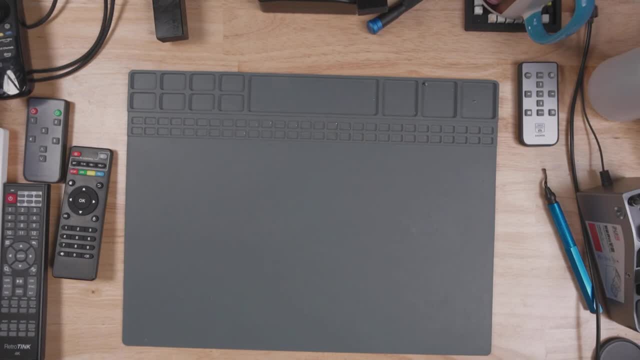 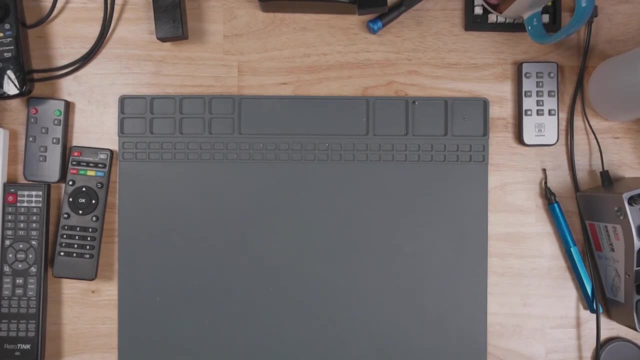 Okay, So I guess I'll get, like I said, my beginning. okay, maybe I'll draw a picture. Is that stupid? Maybe not? I don't have any paper. Let me get some paper. Okay, So we're gonna do like a timeline between: 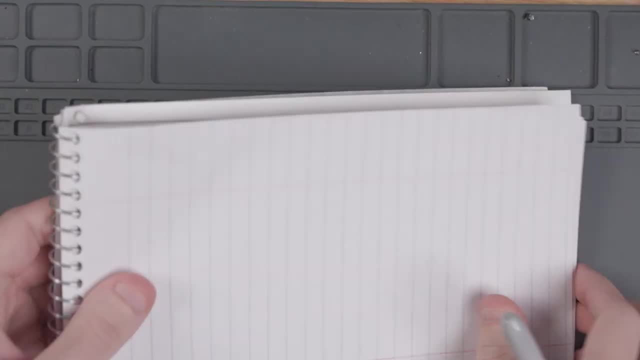 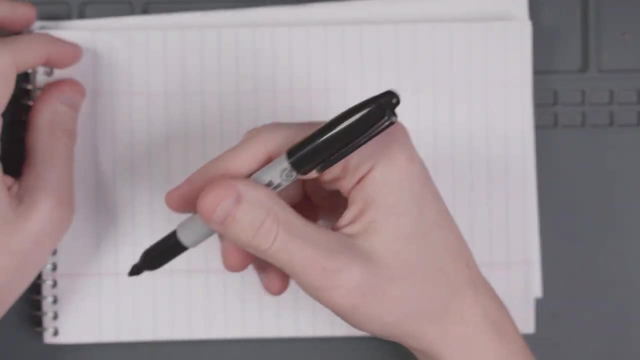 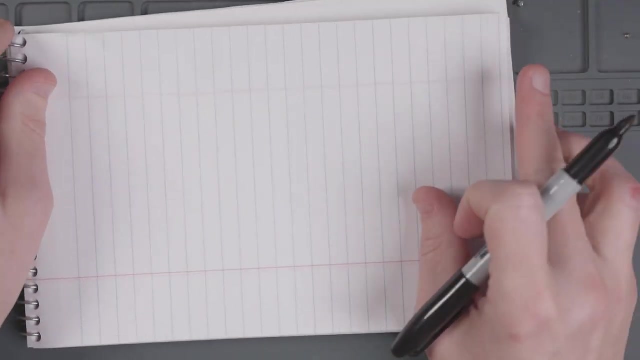 it's helpful to know where this fits in. You know, I kind of was thinking today, how could I relate this in like a console time period? So, like you know, I would say the IBM, the original IBM PC and XT, was like around the NES era. 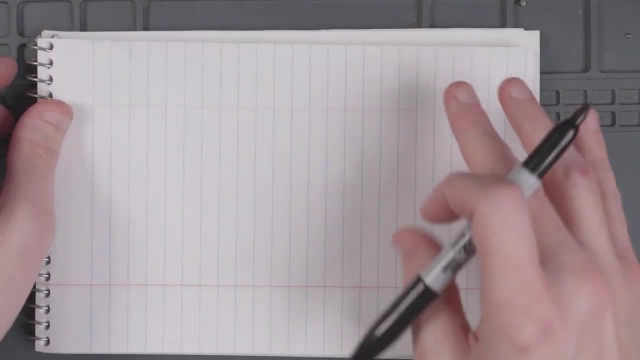 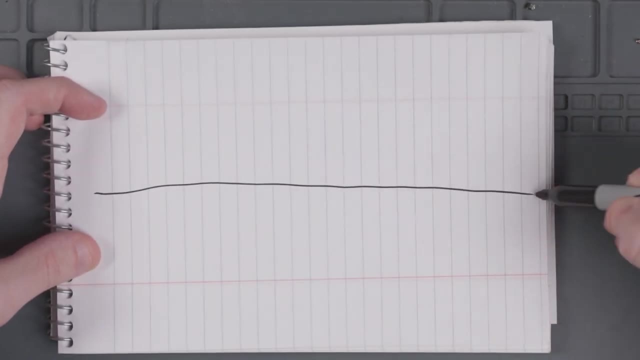 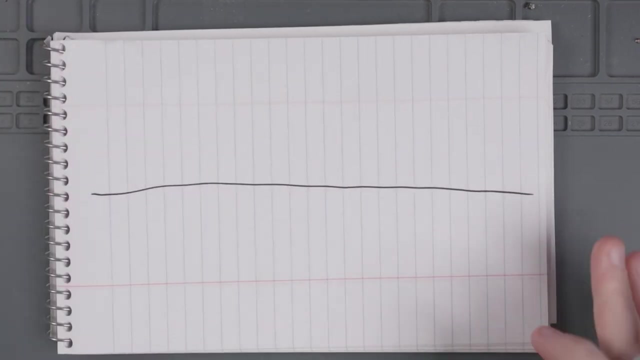 So I would say, if this is so, let's call this the timeline. This is the timeline that I'm gonna be using today. Okay, The sacred timeline of gaming. We'll call this. well, let's see what was the release date of the NES. 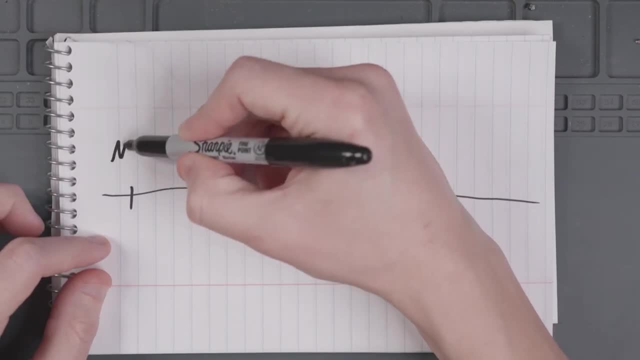 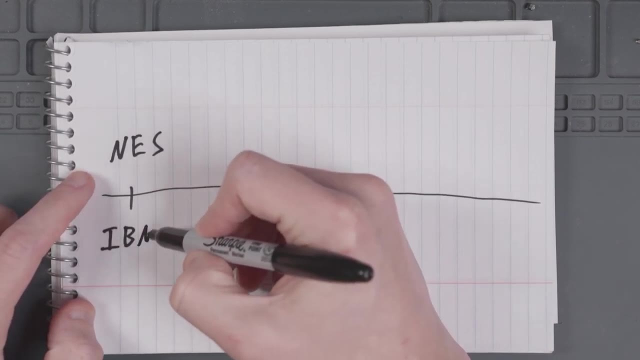 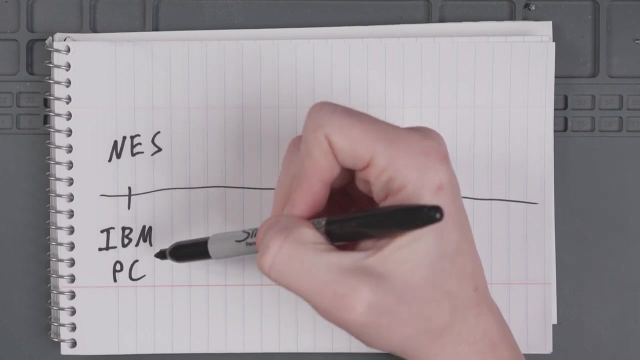 I don't know. Let's call this like 1980 something. This was like the NES, But at the same time IBM released the PC- It was around this time- And the XT, And these weren't like home computers really. 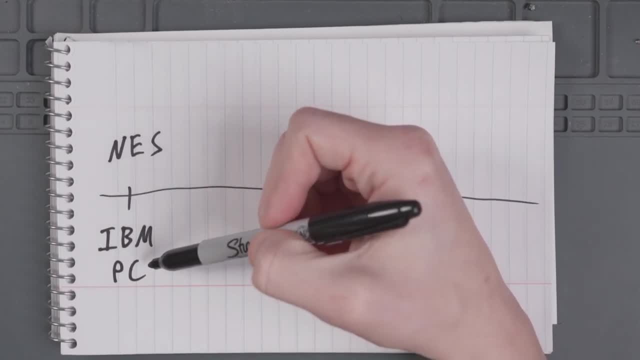 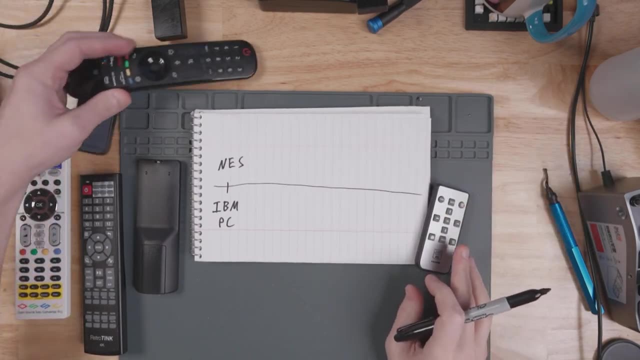 These were for people to do office work. It's a different button on those 12 remote. Oh yeah, you like my. this is my life now, Trying to keep track of all these remotes every time, every stream. So that's my life. 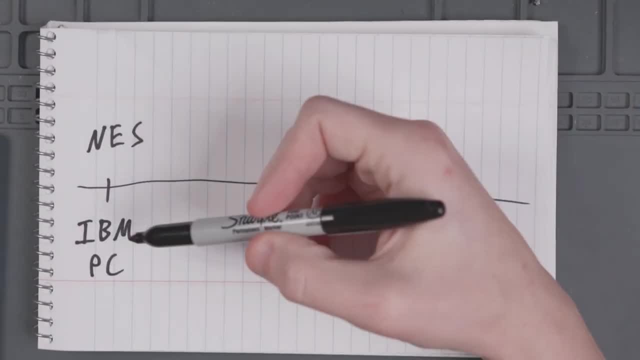 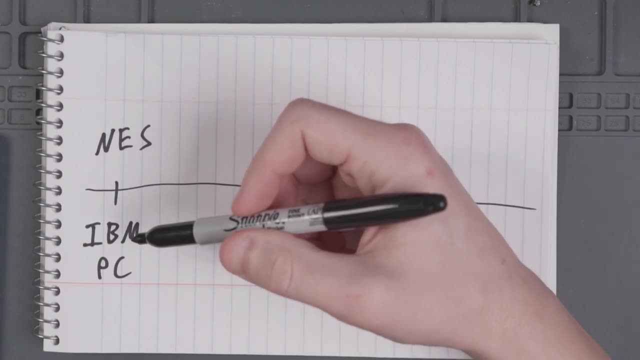 Okay, Yeah, So these weren't really. I would not call the original IBM PCs like gaming computers, right? So they were probably barely. you know, most of them were probably black and white, And so they're really for business. 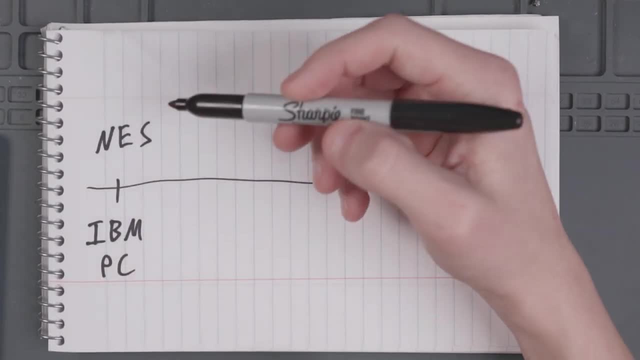 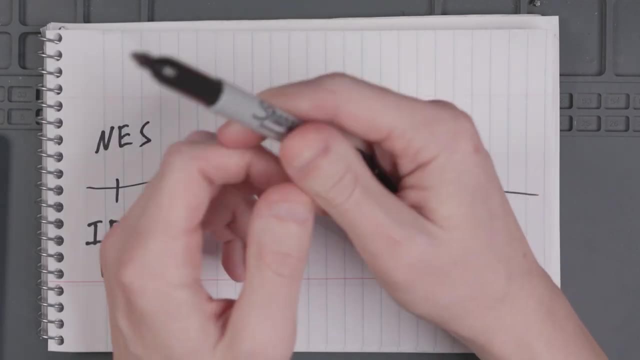 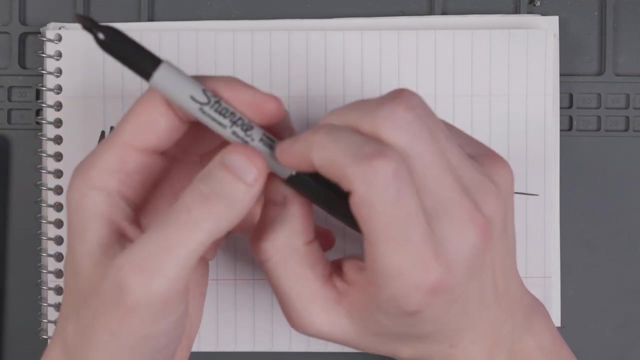 And not really for gaming. But I think kind of fast forward and you'll have to. I think maybe what's his face? APEC guy? I think he has a good, I don't know. You can also just read about the story of how. 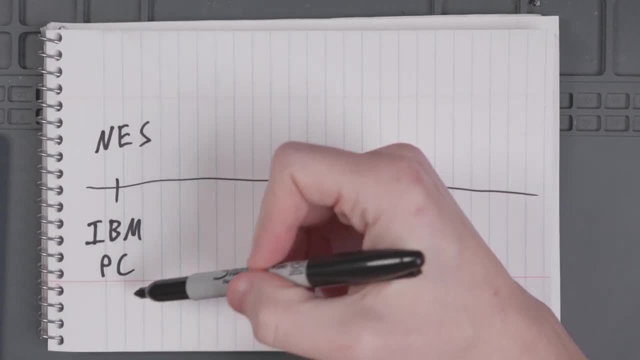 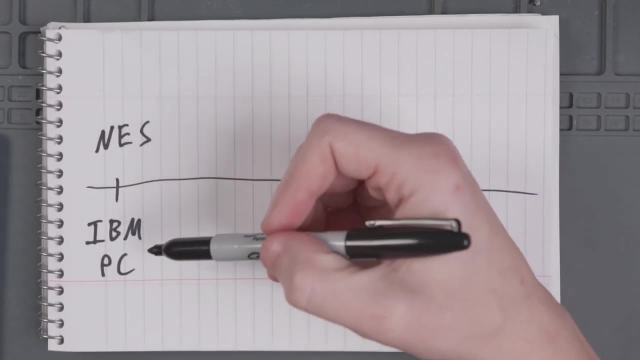 I think it was Compaq. How Compaq reverse engineered the BIOS of the IBM PCs- The IBM PCs fall- was that it used off the shelf parts. It really didn't use custom parts other than the BIOS. The BIOS was the only thing that was okay. 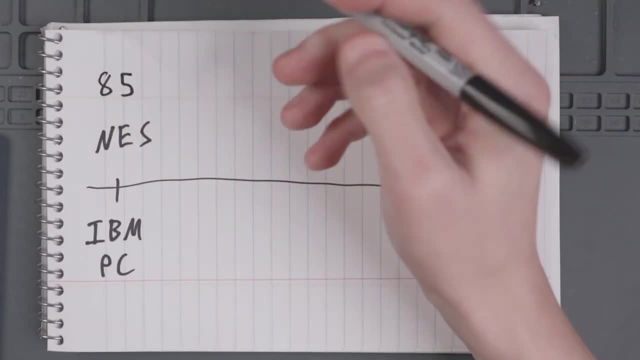 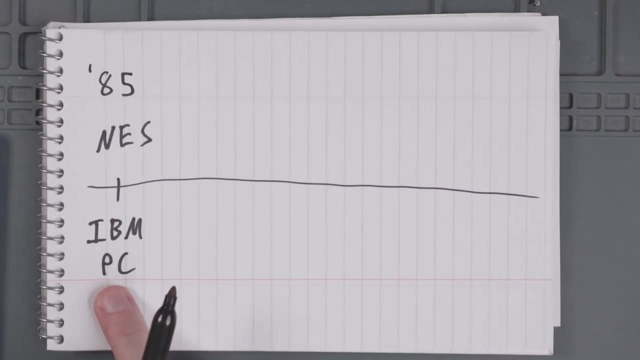 so this is like 85. The BIOS was the only thing that was proprietary, I guess, at the time. So you know, fast forward a few years and this you know. I kind of looked up what processor: the IBM PC. 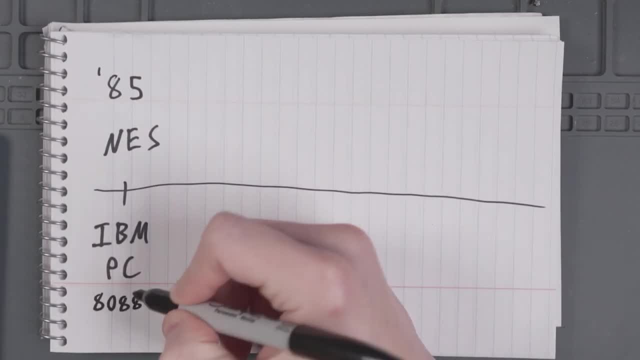 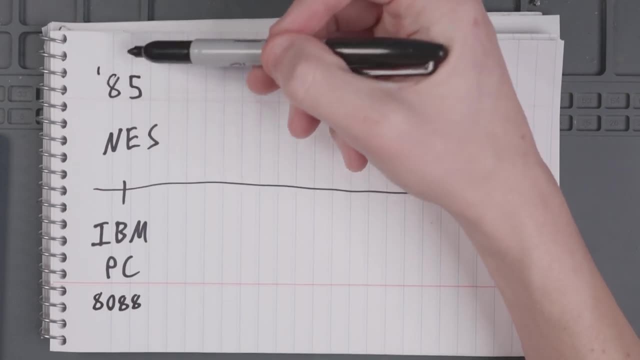 So like that would be this. I don't, I'm not a, I'm not like a CPU whiz. right, I know the like. the NES has a different style of of CPU. It doesn't, you know, it doesn't have the same kind of thing. 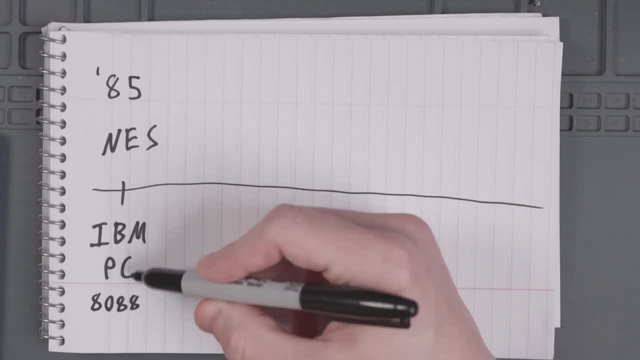 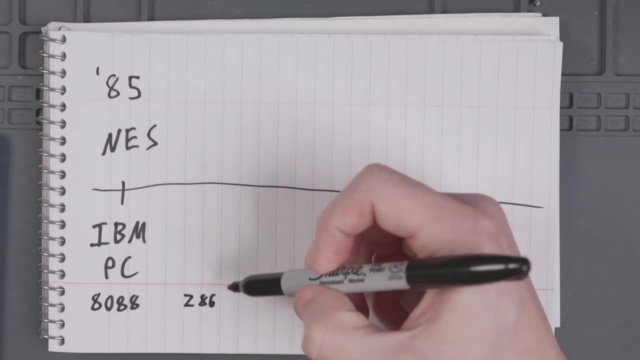 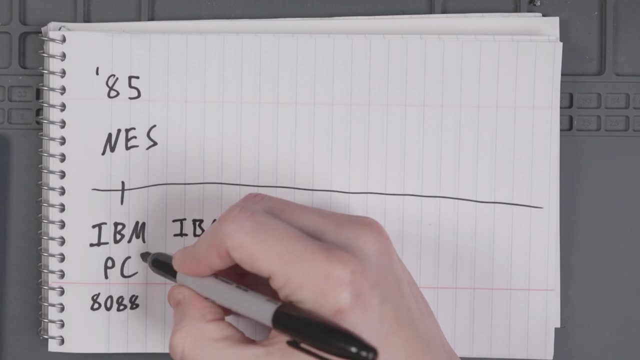 But kind of very quickly we went from you know the IBM PC to like 286 computers. I have a 286 clone machine and I have an IBM. I guess this is also the XT, because the difference between the original PC and the XT 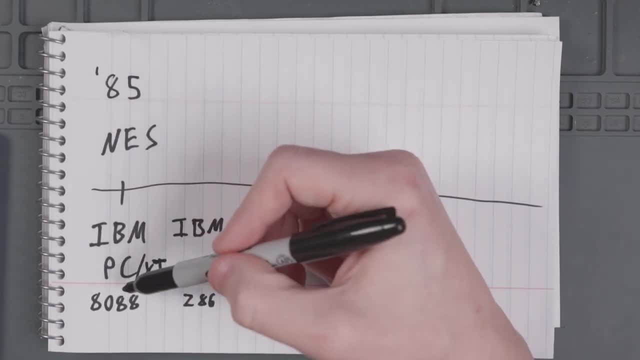 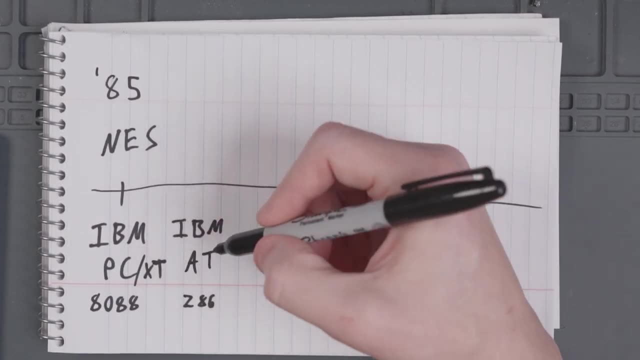 was that the XT had a hard drive built in hard drive. Otherwise you'd have the boot from DOS every single time that you loaded. So the IBM AT was the first IBM PC And I guess it's really the last. it's kind of last. 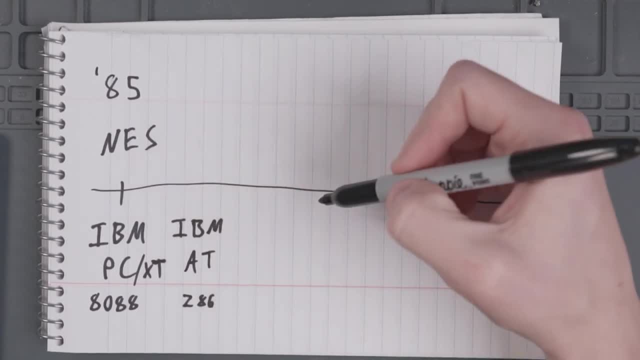 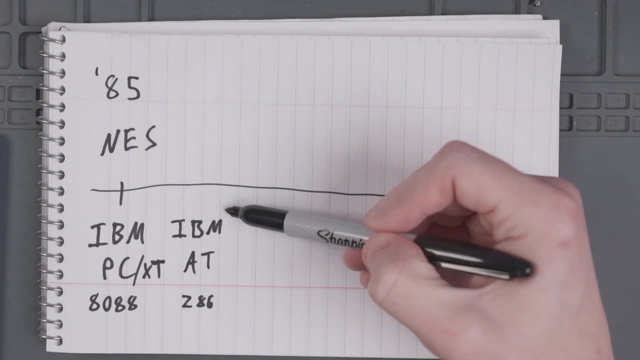 I mean, it's not, it changes. They had other lines of computers going forward, but I would say that this is where cloning kind of took over. like the same generation, the 286.. So I have a, I have a real IBM AT. 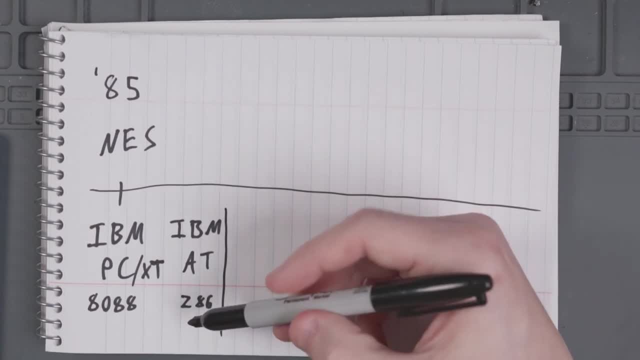 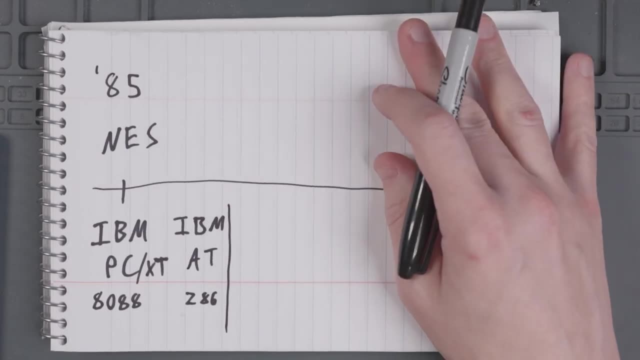 which has a 286 processor, but I also have a clone one. So as soon as you know, companies started being able to just reproduce everything, almost everything about what IBM kind of offered. it was sort of just a race to the bottom. 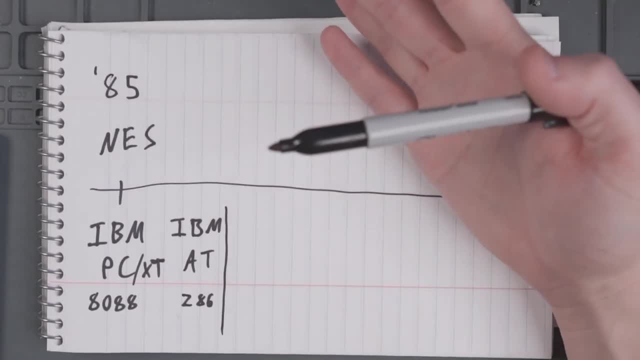 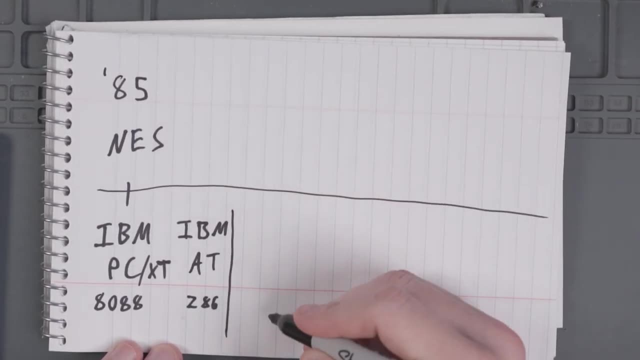 And that's how pretty much the whole most of the computer space happened, at least in North America As far as I know. I think it was pretty much this story. So then you go on to, like you know, 386, 486.. 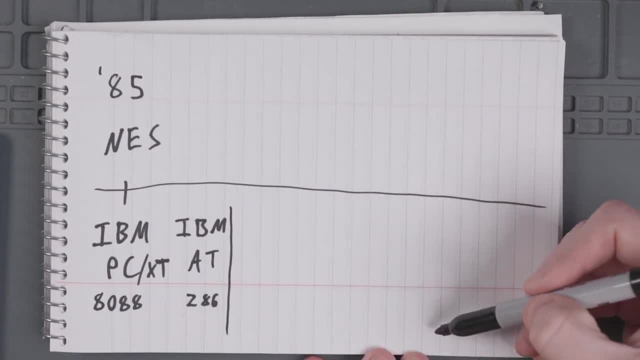 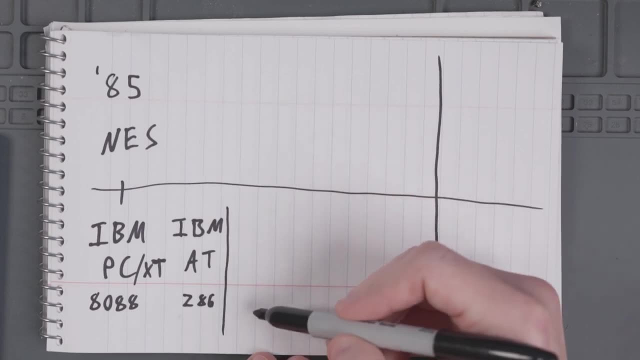 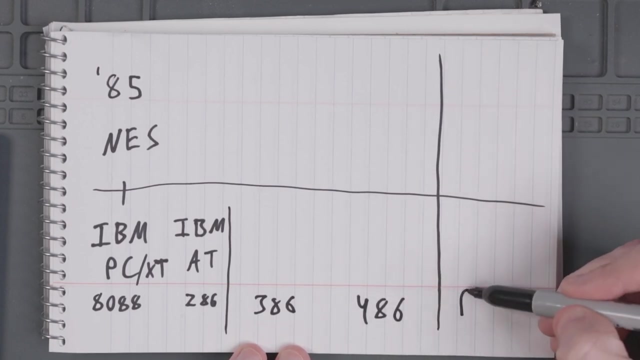 And that's, that's like, that's what I would say. I don't want to say the retro, but like, this is, like you know, 386, and then 486.. So then, this is Pentium going forward. 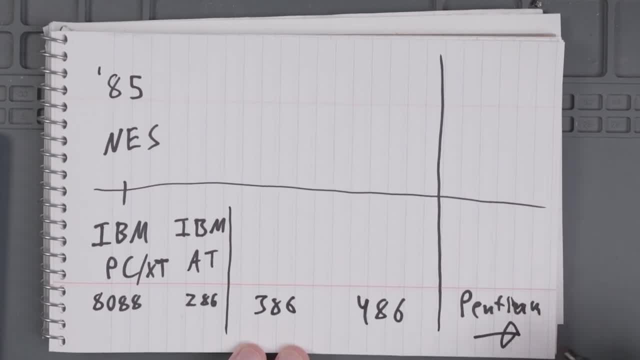 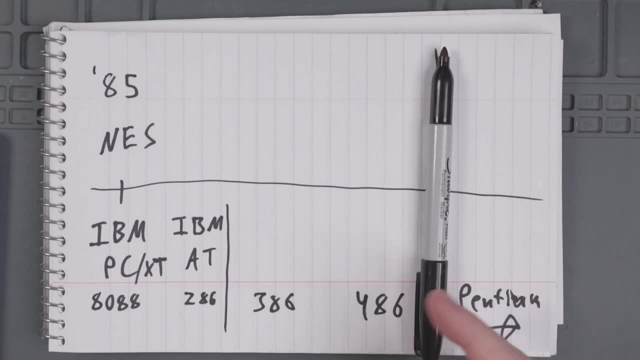 I would say that this is probably the divide. If you're interested in getting into computers, it's really difficult to get in before this because Pentium and later, I would say, if you're really, if you're at all familiar with, like Windows 98,. 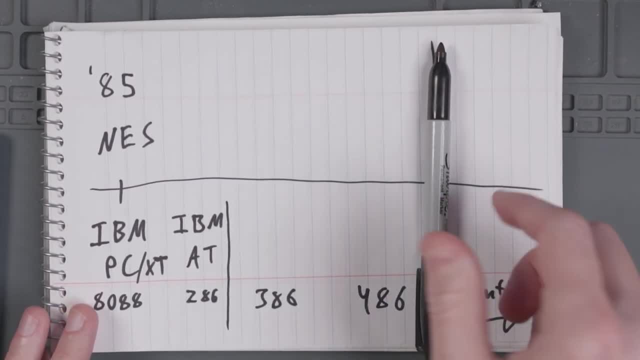 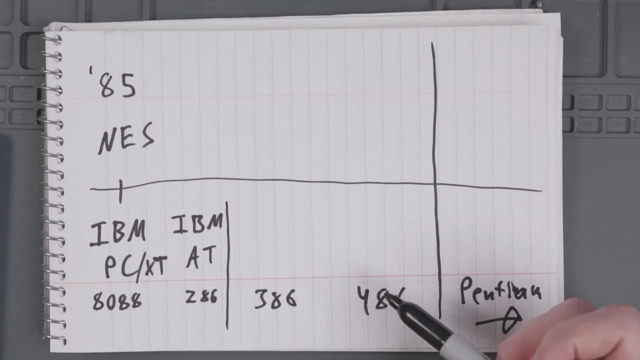 you'll be happy this way. If you go this way, you know 486, you're kind of stretching things. I don't even really know when Windows. it was probably when Windows 95 might have run on 486s, but it was really Pentium and going forward. 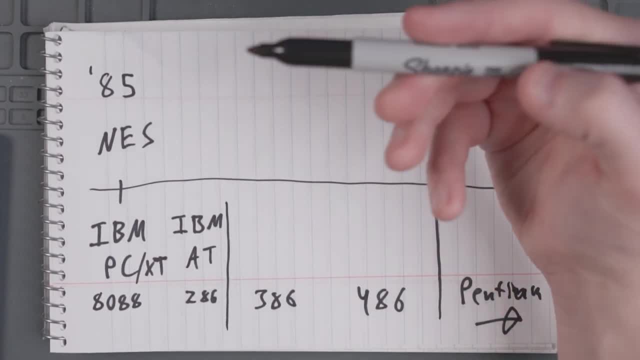 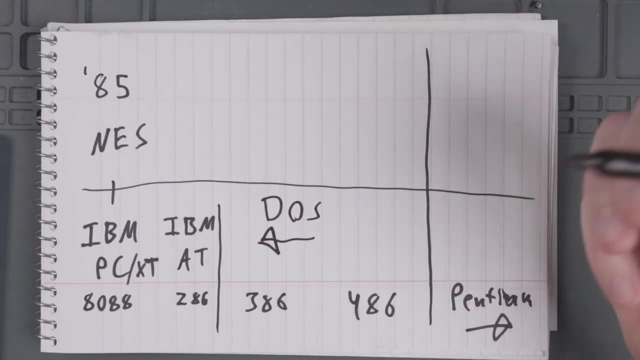 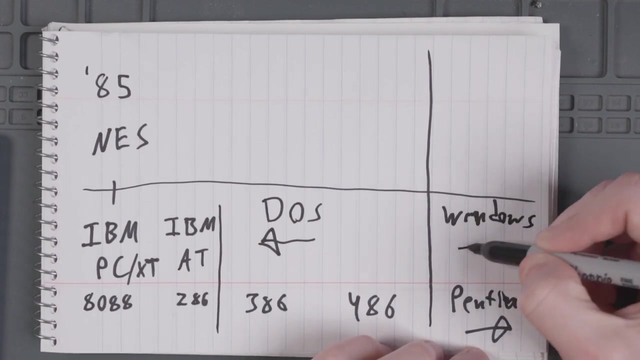 for Windows basically. So here on out was pretty much DOS. We'll just say DOS. I don't know, This is a dumb drawing And this is Windows. So as far as a gateway into playing DOS games, Pentium is great. 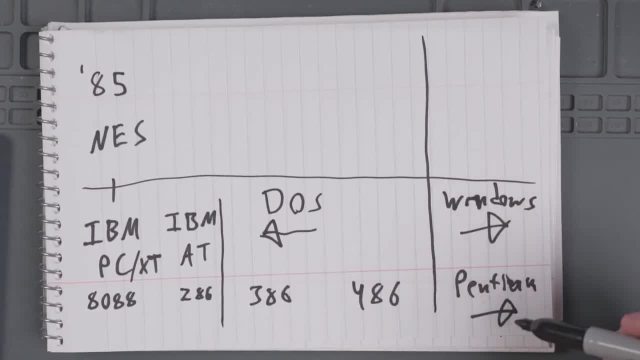 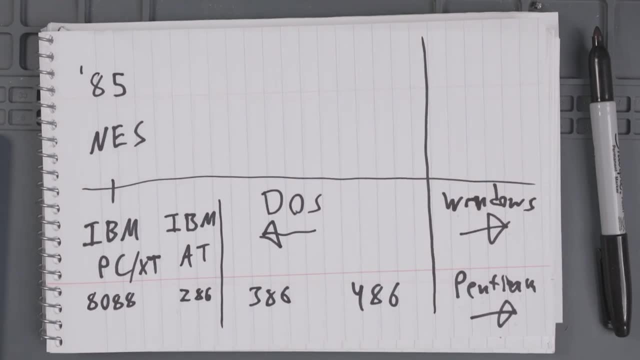 but you can still play DOS games from this generation, So like Pentium 1, and I would say probably Pentium 2.. If you're looking for something that can play the 3D games of the time, so like Quake and stuff- 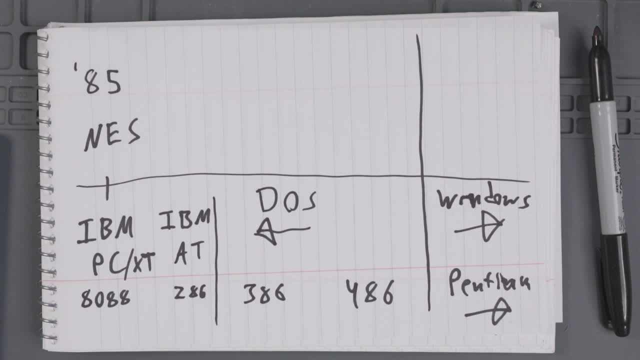 and you might have some decent compatibility with DOS games. going back, I missed the Logitech Harmony remotes. I have a Harmony, It's just yeah. I had an 8088 with dual 5.25 floppies, then upgraded to 286 with Hercules. 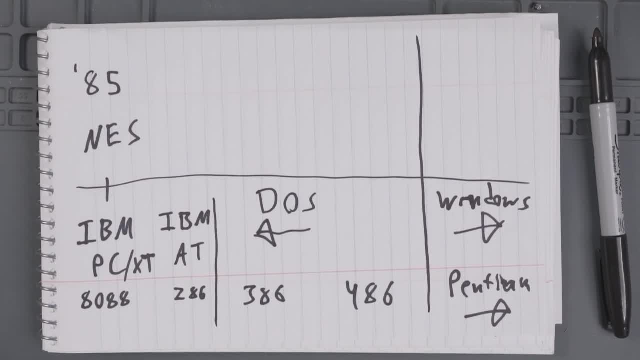 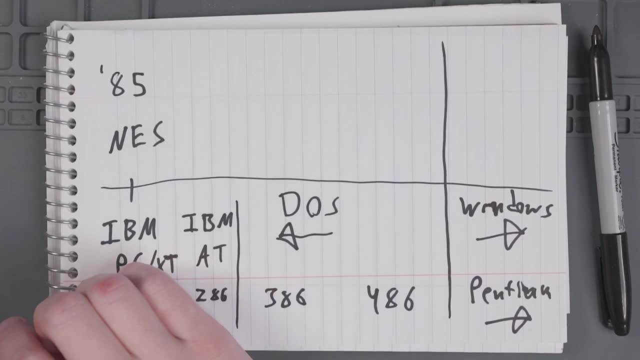 then 386.. Wow, you really went through every single iteration. Computing man. I mean I hesitate to really. I don't really call it fun anymore because parts are super expensive and there really isn't that much innovation. I suppose there is. 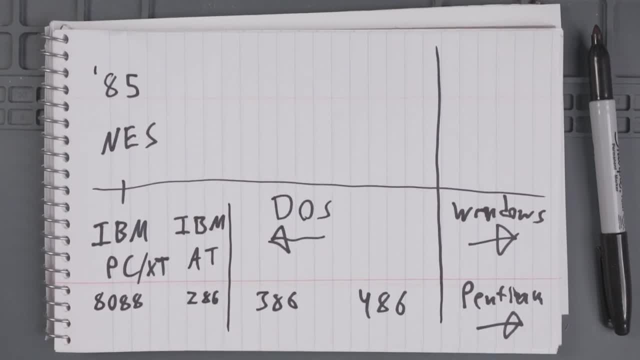 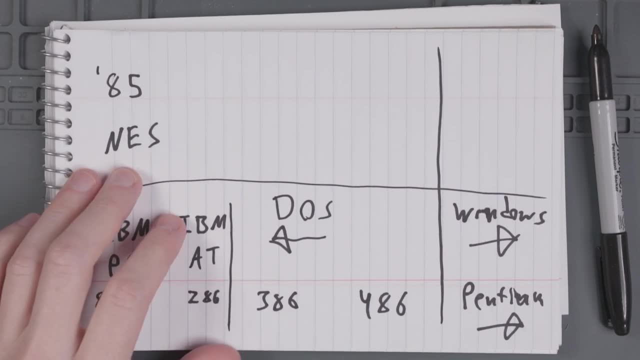 We had Ryzen and all these other super high core count PCs and stuff. but it's not like this era where everything is weird and you've got ISA and you've got PCI and you've got AGP and all these different weird connectors and things. 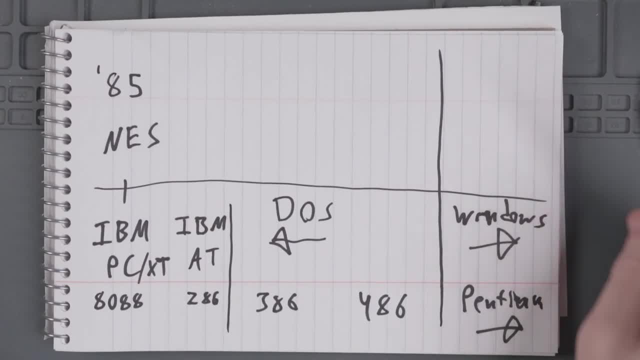 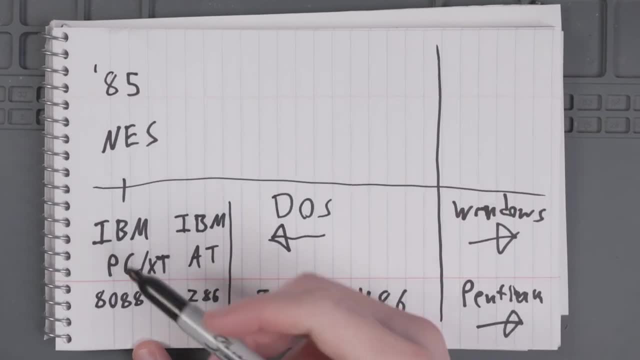 So Pentium equals x86, which is kind of another nickname for Pentium. I mean, these are all x86, basically. So the difference? I read that there is an 8086 as well, so that's the U186,. 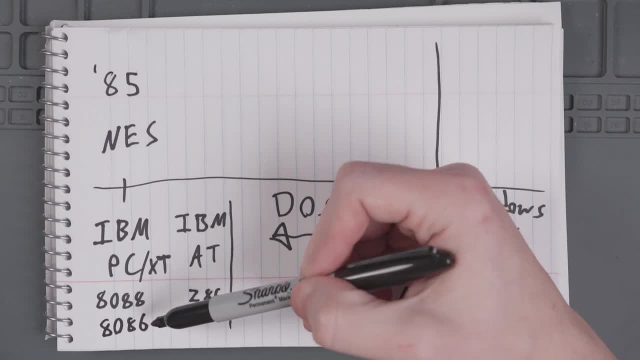 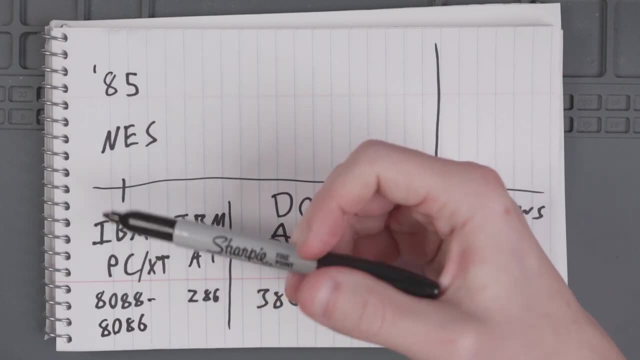 but I think the difference is the memory bus. I think the bus is higher on the 86 or something, but I think these are cheaper. So these were. they're not like cores or anything. We didn't get into multiple cores until well into. 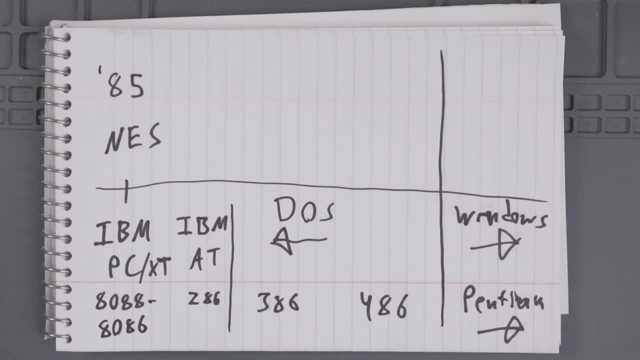 what like Pentium 4, or no, was it core? Core 2 was the first time we had multi-core. What do we have before that with Pentiums? So, technically, this is all x86 architecture, This whole. 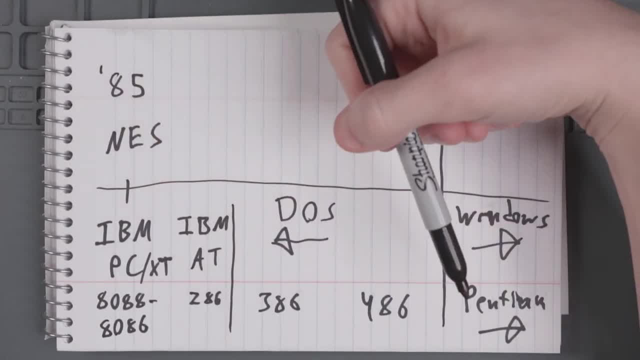 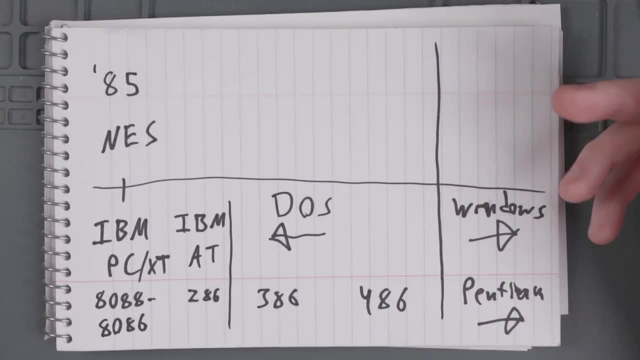 everything and kind of going forward. for the most part You have. you know you have new features, a new CPU. what do they call it? Not libraries but the- I don't know- the features of a CPU. you know. 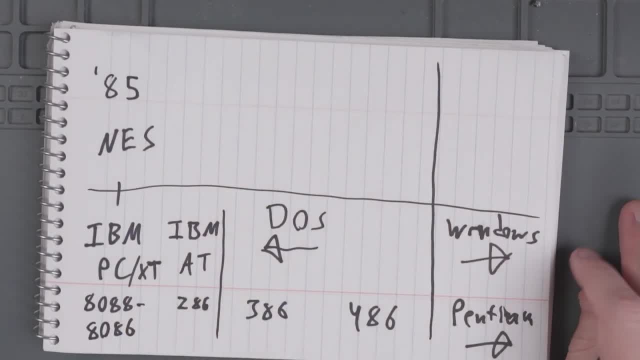 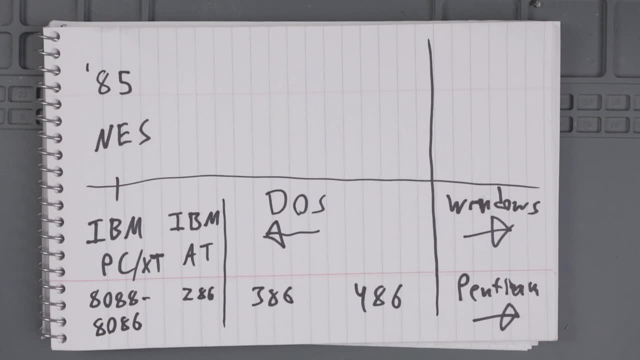 they get more and more as you go forward, so you can't really go back with newer hardware that much. but x86 is an architecture that is still in use. Yep Core Duo, I think was yeah, was in the first core. 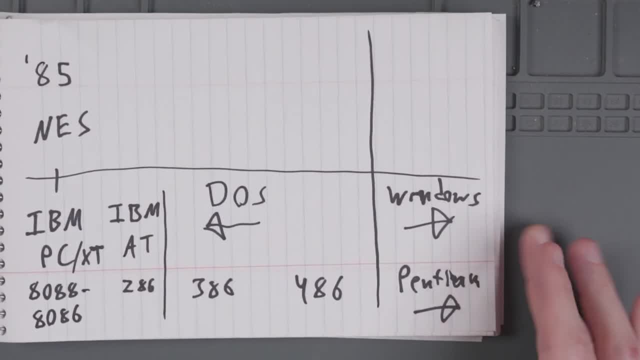 So this kind of goes up. you know, single core goes from here, and then Pentium 1, and then- if I kept the drawing over here- 2 and 3, those were really kind of more like also business class or like professional. 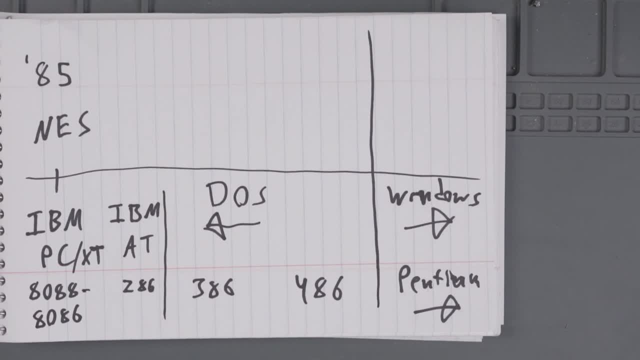 like, let's say you were at, because that was about the time when, like people would start doing like- I'm sure it was probably in the 80s- they would do what computer, like CAD, or maybe even like video, like CGI, work for video. 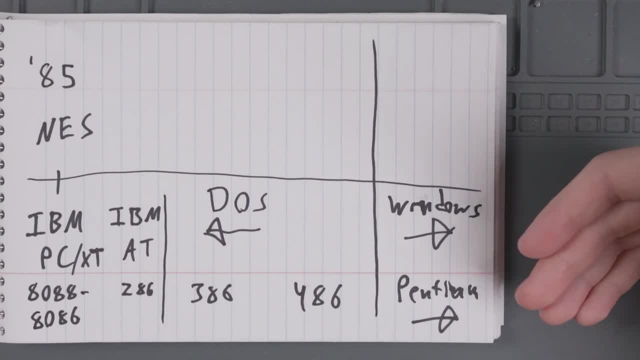 probably would be done on these kind of like higher end so you can get. you can get Pentium 2 and 3 systems that have multiple slots. so I guess, because Pentium is pretty much in slots, the Pentium 2 and 3,. 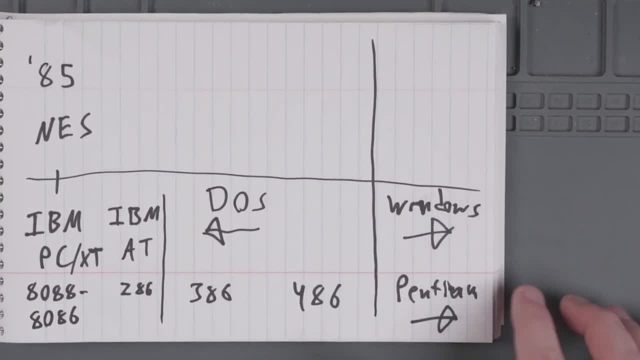 so you could get multiple CPUs, physical CPUs, in it. so that's like hardcore, like you really need really good performance was up here before Pentium 4, Pentium 4 was when things started to begin getting samey. my first computer was a Tandy Coco 2,. 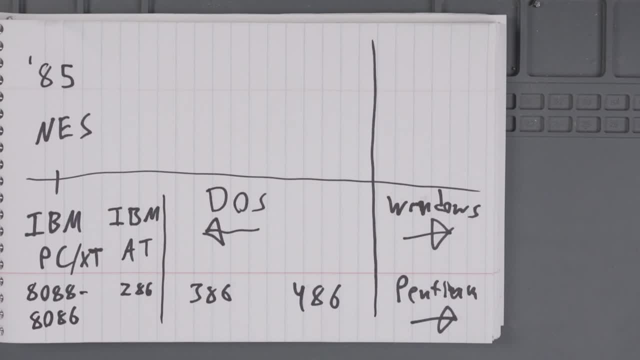 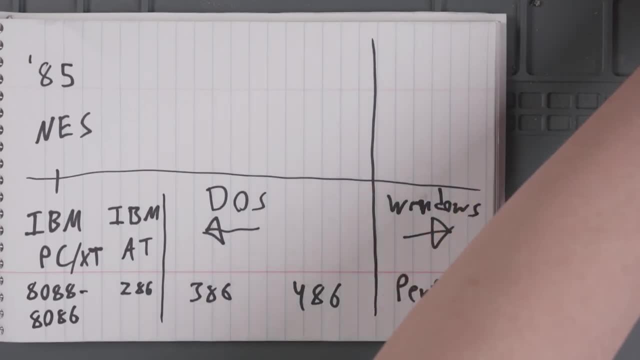 yep color computer. I would like to get a Tandy someday because I know that they have the unique sound capabilities. like games are written some- some DOS games- have a Tandy flavor. that would run on their fancy, fancy integrated sound card thing. 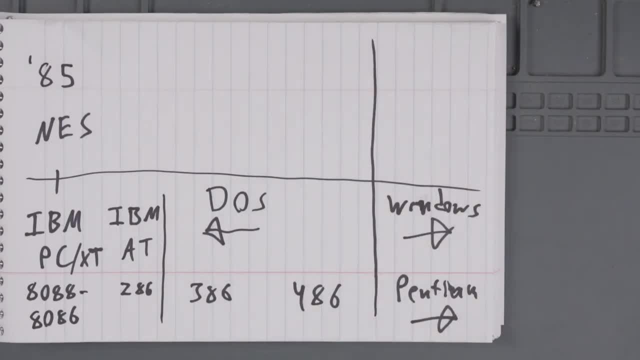 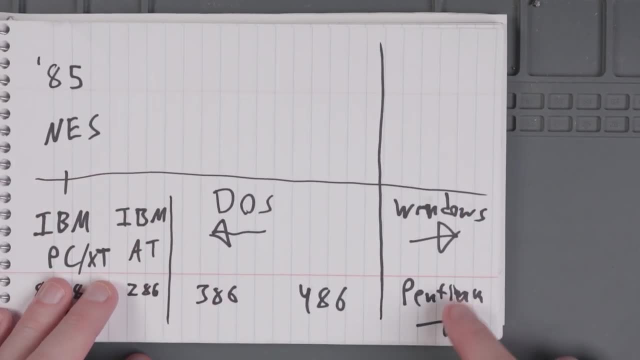 yeah, processor extensions. I guess like the, the- there's another word that I can't remember right now- whatever. so you have like MMX and stuff was around this Pentium age and yeah, so multimedia and online stuff is like this going forward. 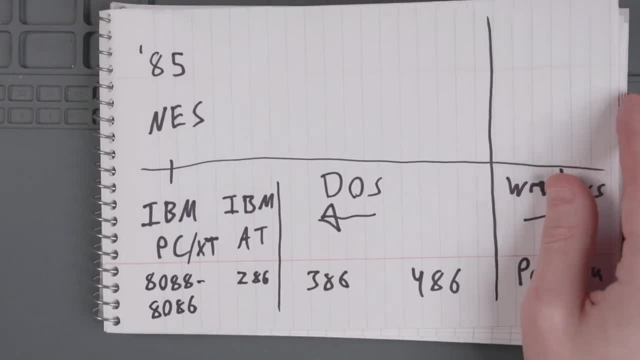 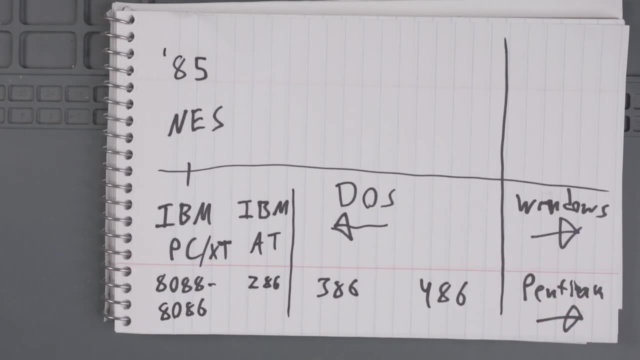 all right. so from my experience. so let's ignore the Windows and beyond. so we're in DOS land, hardcore DOS land. there's multiple different version of DOS. this particular video is not going to really cover DOS, but I just wanted. 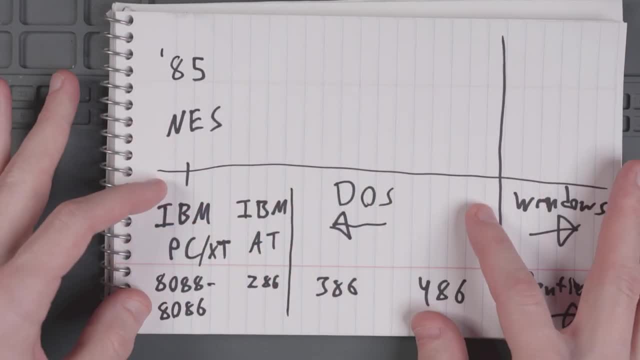 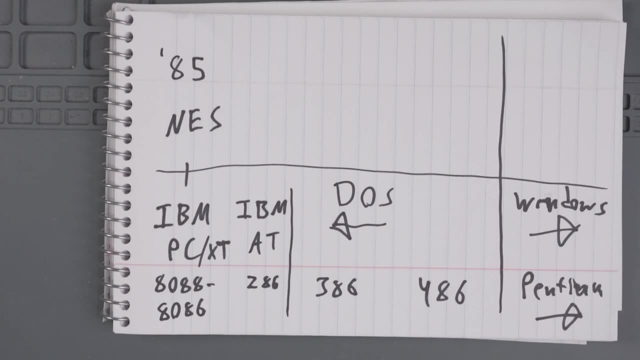 or you know how to use DOS, but I wanted to frame what, what the the importance, I guess, of the Micro 88 is. so if you've ever seen what an original IBM XT so like, let's say you wanted to go to the NES. 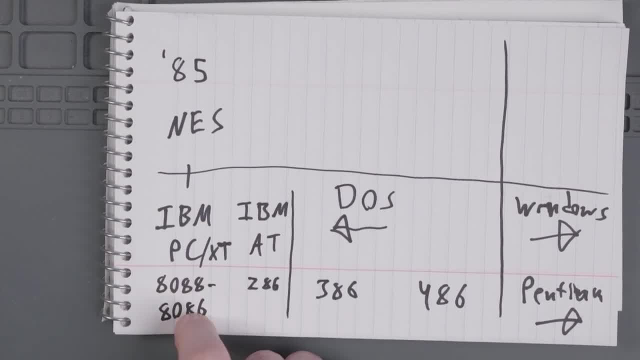 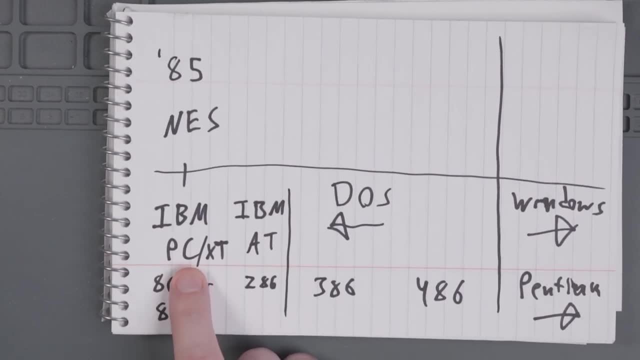 let's say NES sort of era. there were some games, right that I played King's Quest. there's a King's Quest version here, BurgerTime, there's a whole bunch of games actually, if we go to. 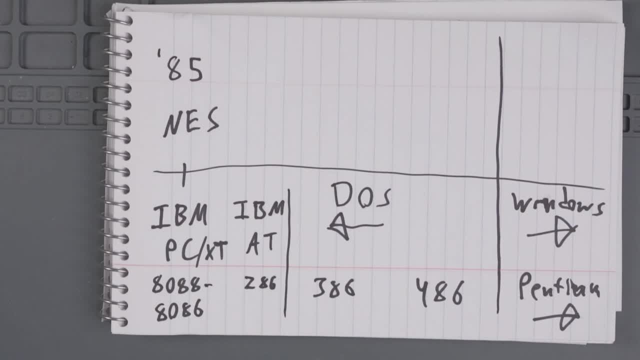 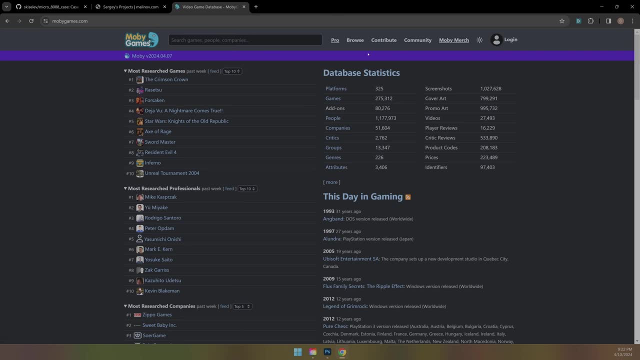 what is it? Moby Games. there's a website that has- yeah, I think it's this- this. this Moby Games website is kind of cool. then we go to browse games. I swear we're getting to the project. 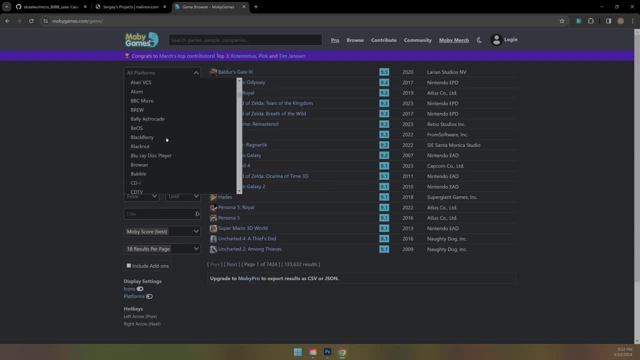 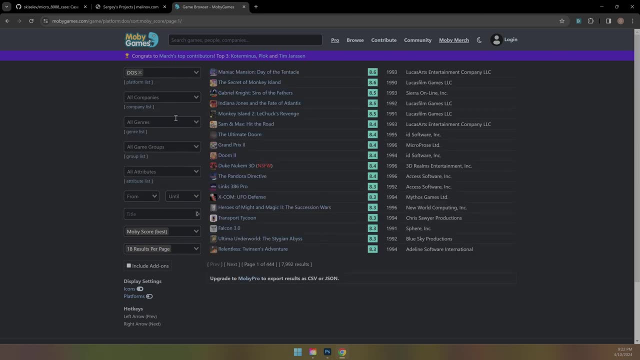 we will. and then we do platforms and then DOS, probably, or PC, DOS, DOS, and it has a cool list. you can kind of go through all of the games. I mean this is page one of 444, with 7,. 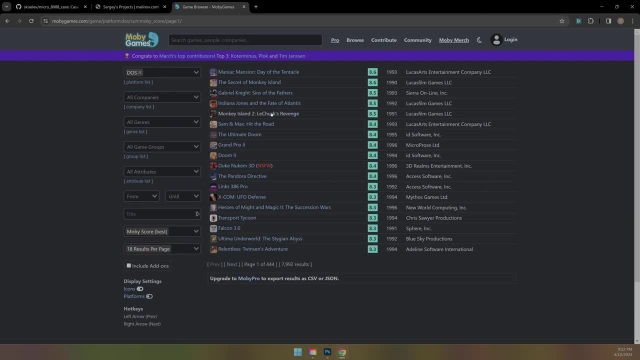 it's 8,000 titles that they have and you can kind of go like year by year almost and see what is out and what's popular. it has some some of these like I don't know. 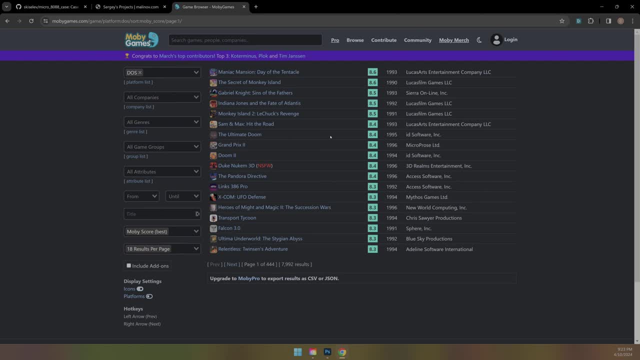 this is Moby Score. so if you're looking for like cool or new DOS games or something, this is a cool list to kind of like give you some inspiration. but we want to look around like 81,. 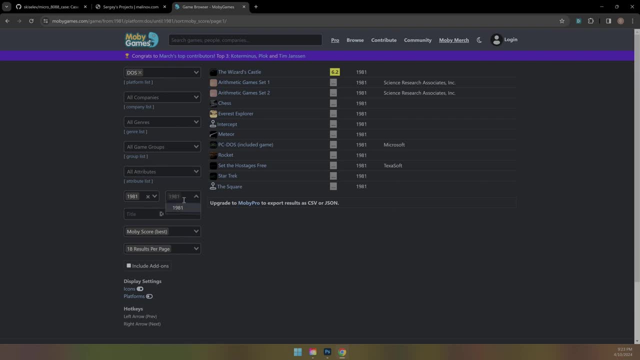 to really no get out of here. it looks like 89, what, what? what is this list? yeah, from until. oh, can you only do one way? oh, okay, here we go. so this is every game between. 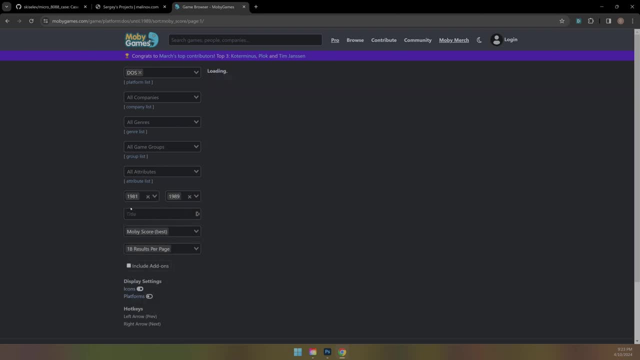 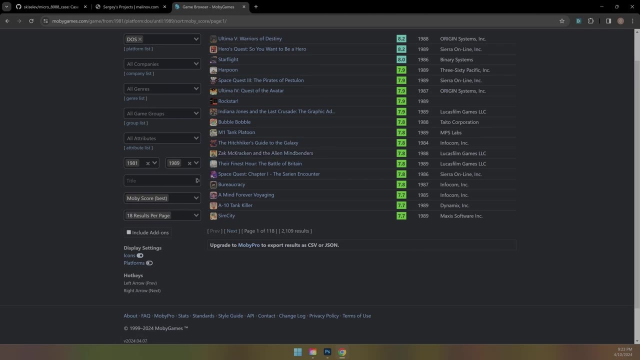 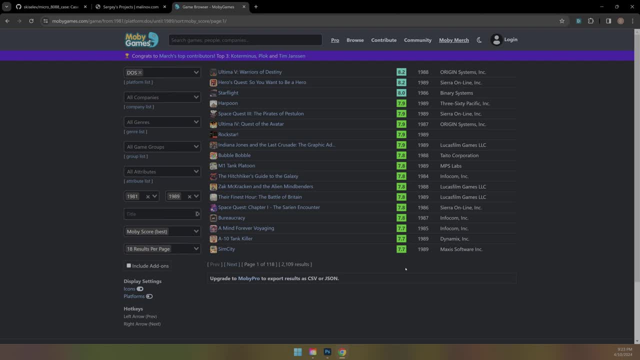 dang hey, Reventlo Tandy- yes, Tandy was Radio Shack. yep, yeah, yeah, Alterations, yeah, you're right, MMX 3D now, okay, so so what would be? 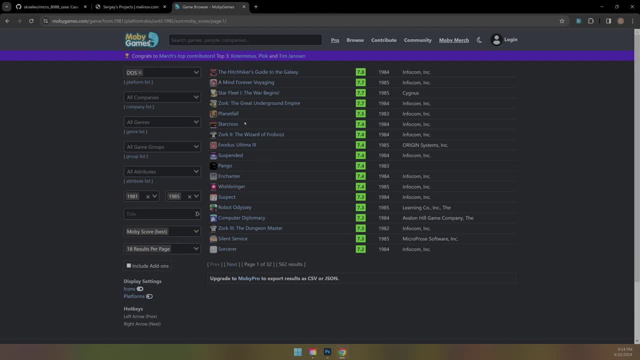 like an older game. so this is all the popular games let's get out of here. how about like 85,? was it really anything? I think Zork is also a text adventure, but like Ultima. 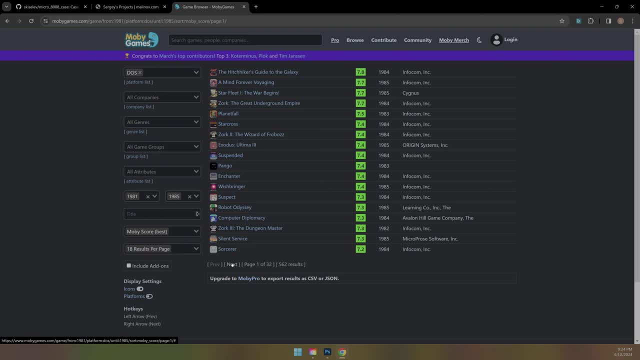 you're beginning to have. I mean, these are gonna be, like you know, the quote unquote: better games, Ancient Art of War. so there's a lot of games in this time period. right, that you know. 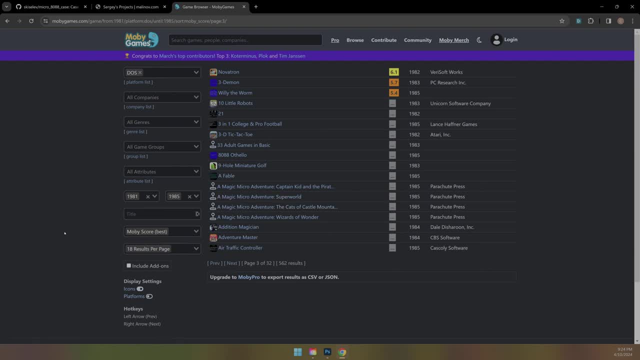 you could run DOSBox. that's a definite, definite option, but it's not. it's not the same and you don't get the experience. I feel like people that do like retro gaming stuff they like. 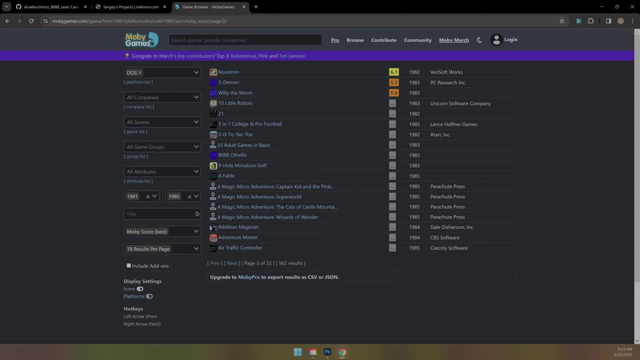 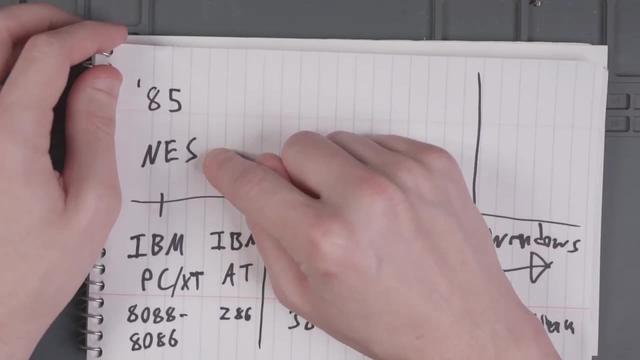 retro gaming, for that, you know, even if it's just a a little bit, even if it's just a little bit of modding or like using a scaler or something, you're physically interacting with a real console. 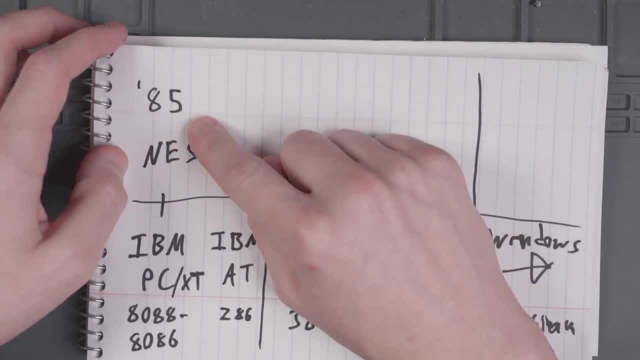 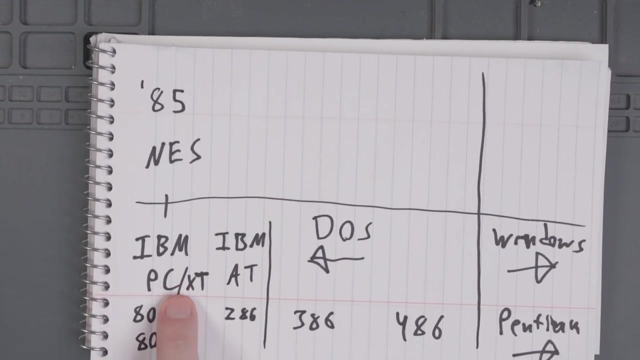 a real thing from you know, whatever 1985, um load stacker to double your drive space. uh, so, yeah. so I realize, though, if you look for an original, and so I wouldn't even recommend buying an original IBM PC. 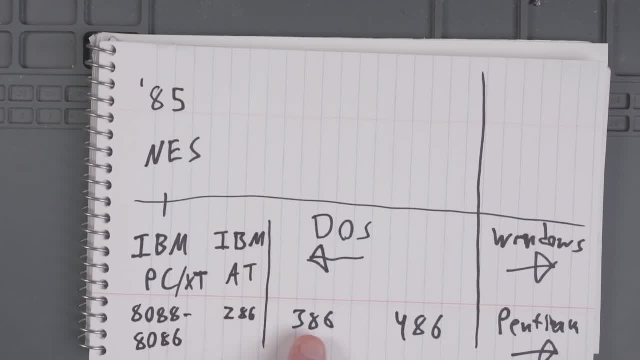 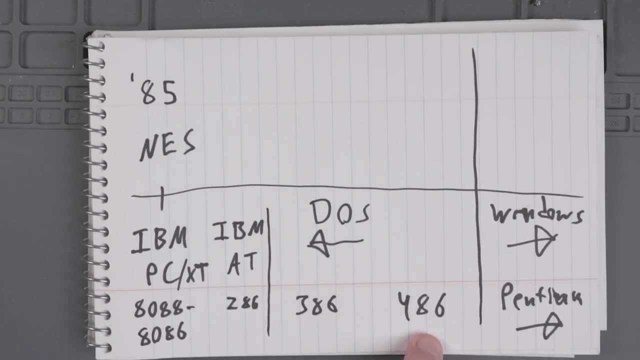 unless you were a a collector, like I barely call myself a collector- and I bought a. you know I I have the 286, so I really I bought a computer that had a 3D6, recently. 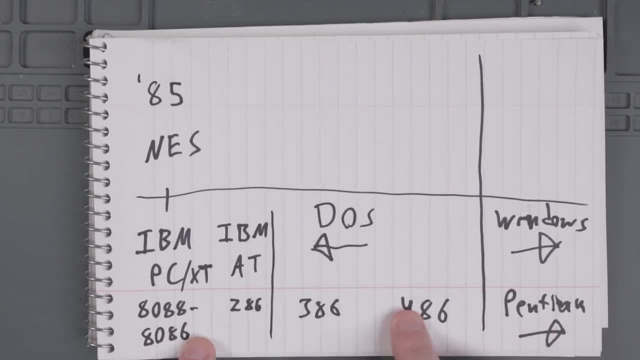 I bought one that had a 486, you know, I I had when I was a kid. I had a Pentium, so I really had to. I wanted to fill in the gaps, to kind of complete my collection. but 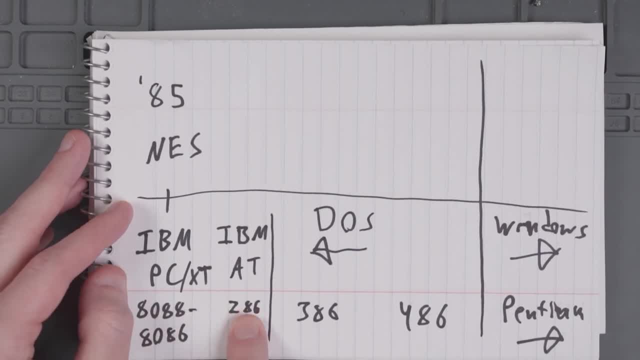 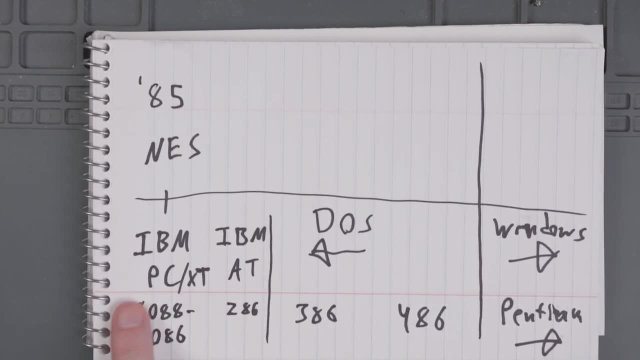 I have to admit that the capabilities of these kind of- uh like original IBM PC, this 286, in a, in a real IBM AT, the performance is still lacking. you, you, you're gonna struggle running some. 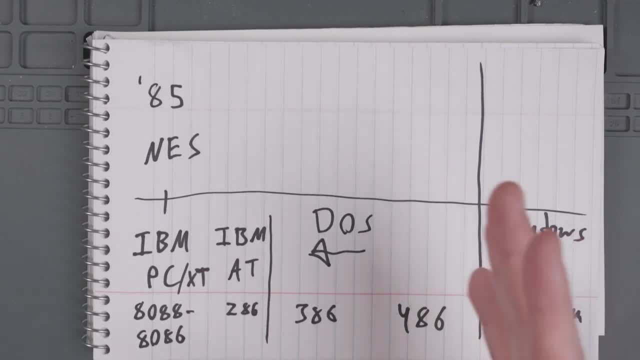 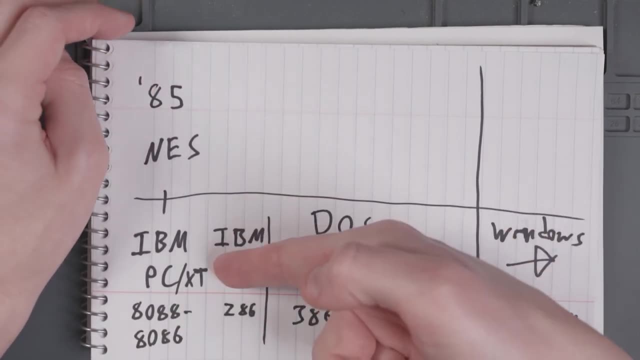 you know certain games that are hot, like 3D, that have any 3D if if at all right. so this is more for like 2D games and stuff. so I kind of relate this to. 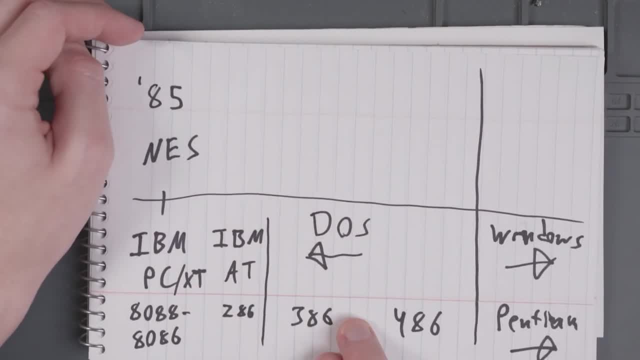 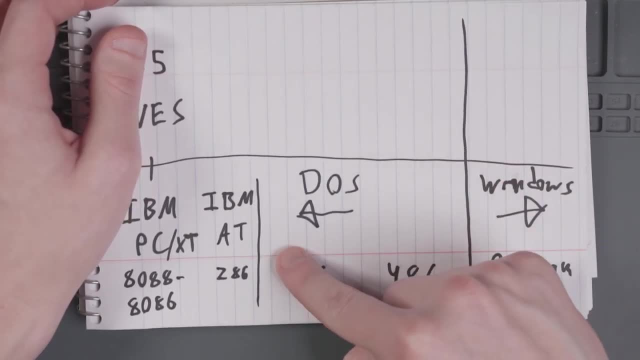 like the NES, I suppose, of this stack. um, you know, 386 is is nice. it's kind of like you know some like uh, what was that game? that driving game Stunts. 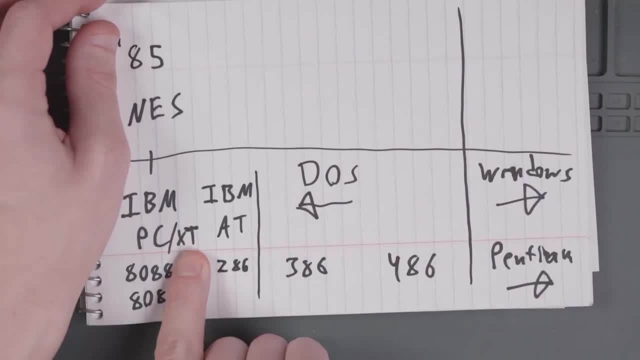 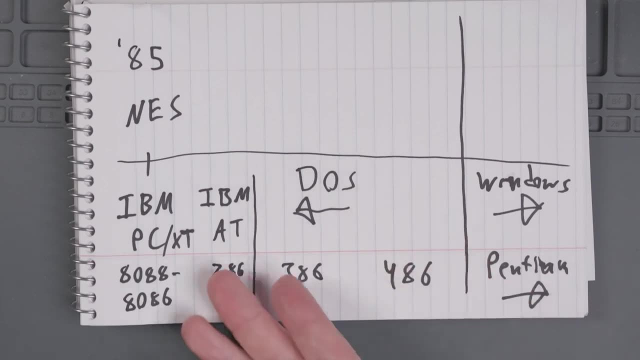 like it kind of barely runs on a 386, it really also depends on the video card that you have. but there's kind of you have limited like configurations that are are like worth doing. I you know. 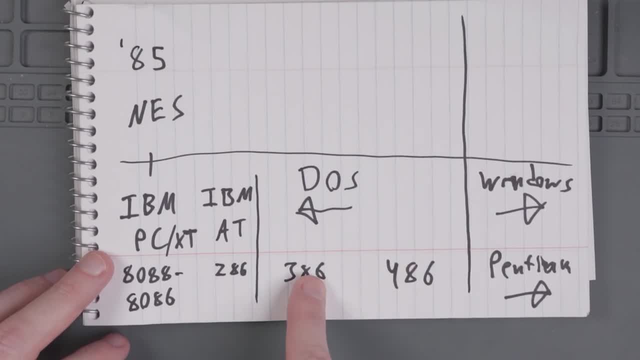 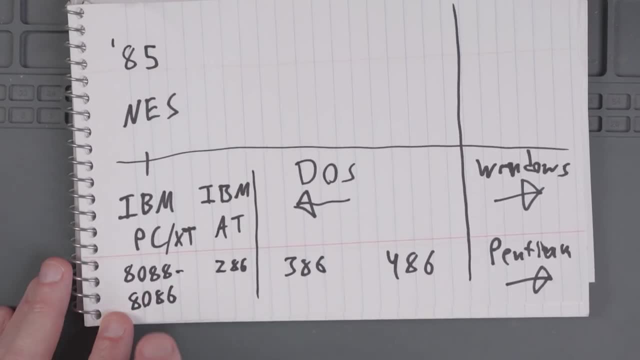 you don't put- like you wouldn't expect to put- a like a high, high-end, like VGA card that might you might have had, um you shouldn't, um you know, have it in our collection. 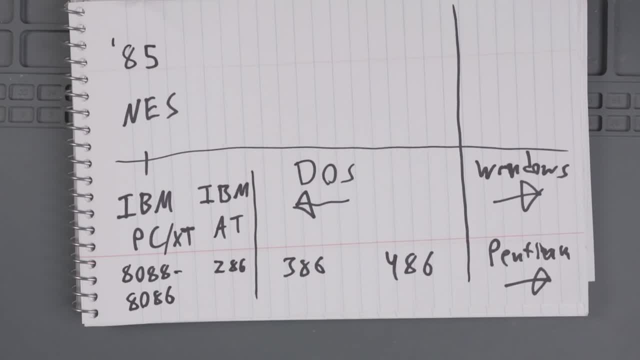 I guess, is what I'll say. so if you haven't- no, if you haven't- noticed the prices of these things, let's see, let's just go to eBay. I know this is kind of risky, not risky. 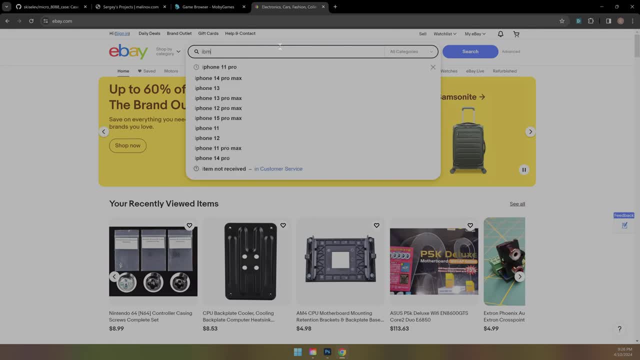 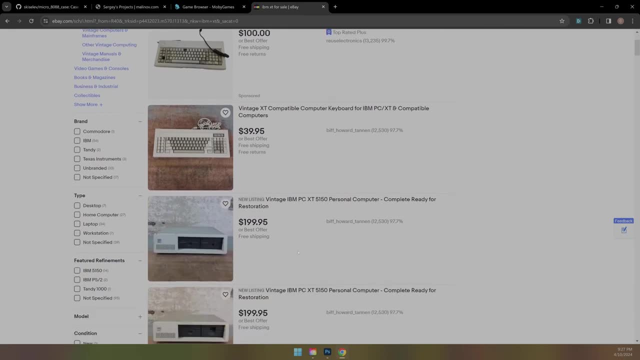 but I don't want to leak any info. so let's, let's, let's type in like IBM X, just put an XT, because the XT is the first one that had um, the first one that had a. 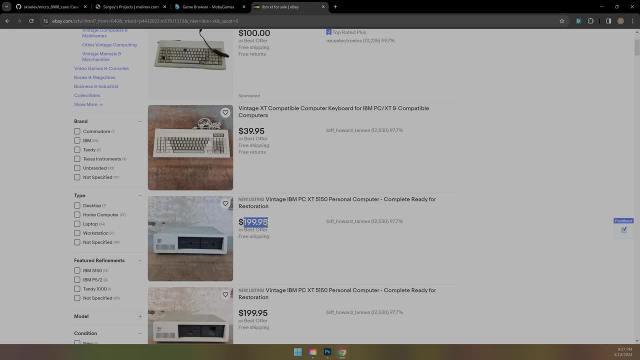 uh, I guess it's not terrible. this one looks for restoration okay, so that's actually not a terrible price. the other thing you have to know is that I, if you want to look for um the IBM PCs. 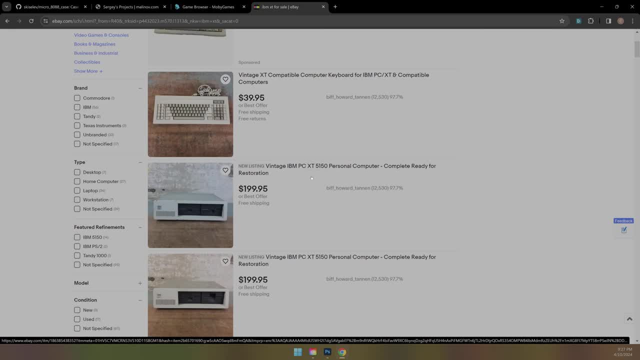 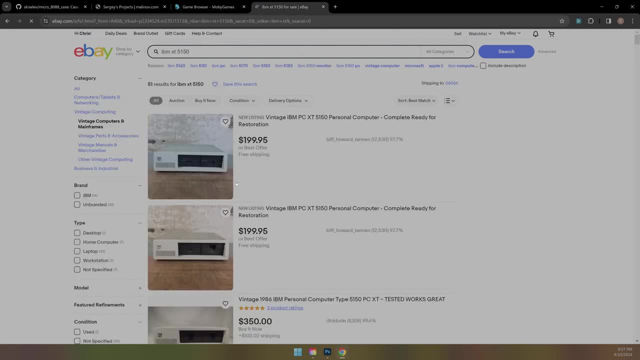 they had this uh numbering scheme. so 5150 is the XT, 5160 is the AT. so, if you wanted to, we really should put um 5150 in here, because we might get other stuff like: 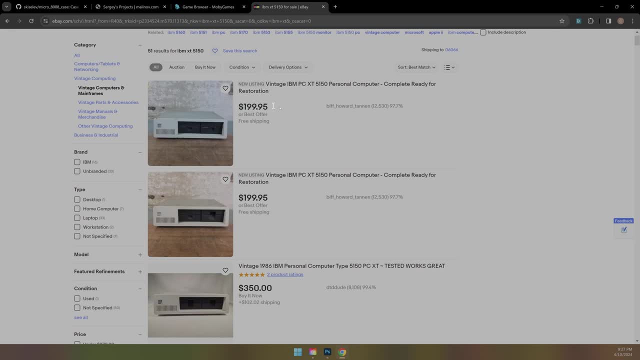 uh, stuff, I guess it's not terribly expensive. but the problem is not necessarily the expense. the problem is then you've got to: um, get it working, get all the other stuff working with it, um, and 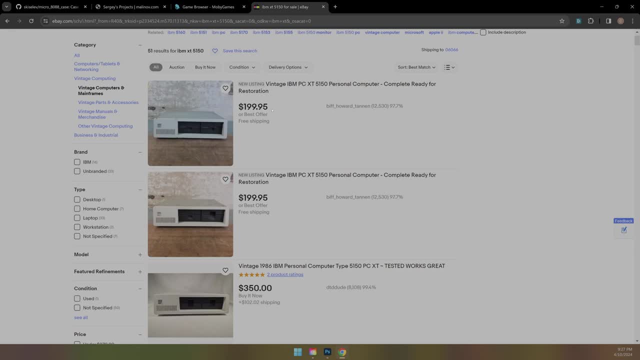 you know, if I'm being honest, I don't know, if you know I do not recommend people trying to get like MFM and like hard drive- old hard drives working, I guess, if it has floppy disks. 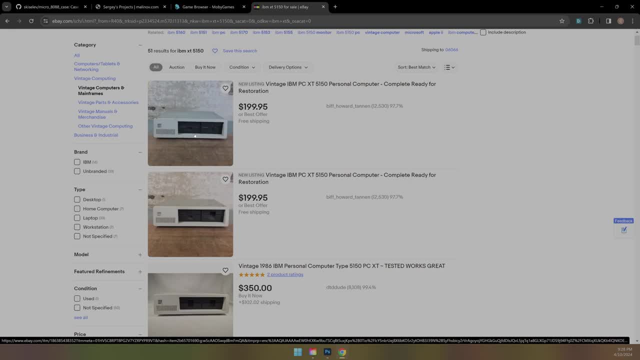 and it can't like. you bought a- let's say you bought a system and it had floppy disks, or floppy drives I mean, and it came with DOS boot up disks. I guess you could be happy with that, but I don't recommend anything. 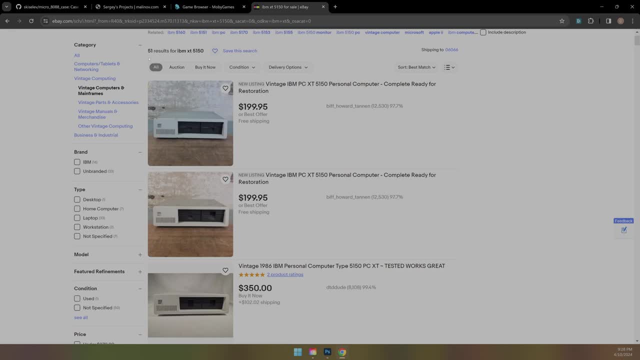 assuming all the parts work um, because really all you have to do is boot DOS. right, this? this is we're in IBM land, right? we're in IBM PC land, where you just boot DOS from. uh. 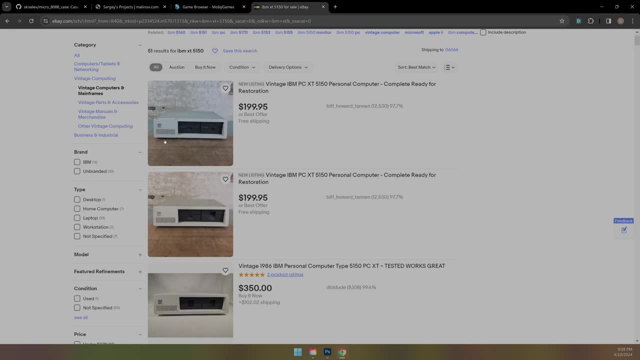 one of the drives and then switch to another floppy drive or or a hard drive or something to load your games and things from. so it's really not that complicated of a of a setup, uh. but the huge downside of these 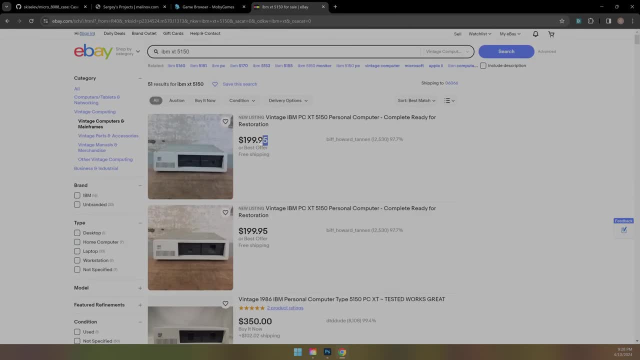 besides the price, which is not terrible, I gotta. you know it is a lot of money, but it's really uh end up being well, not with all the add-ons and things, but um, it's heavy as hell. 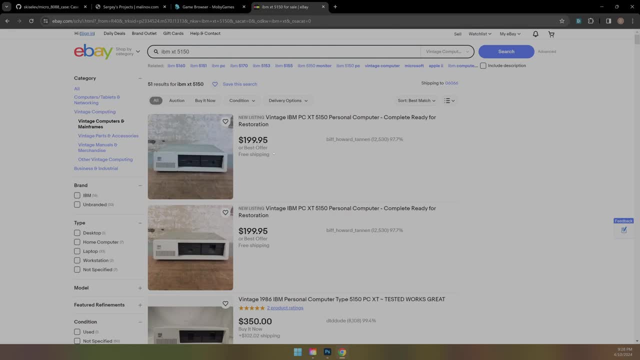 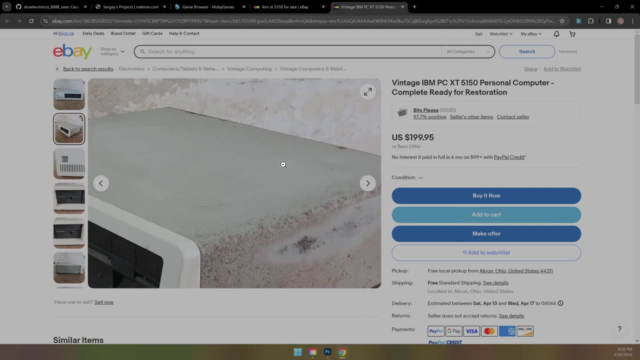 you like, if you do not wanna like, if you have no room already, then you're gonna not ever wanna buy one of these. they look, do, look cool, but they are definitely desk uh consumers. 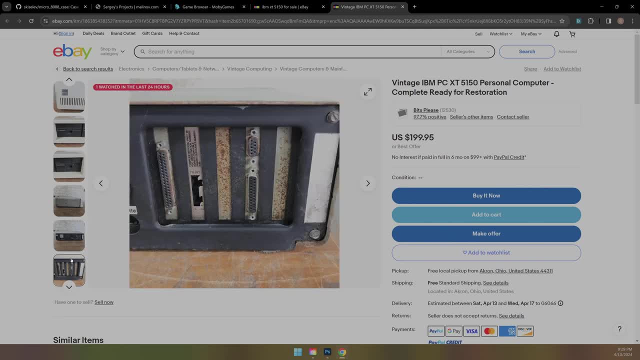 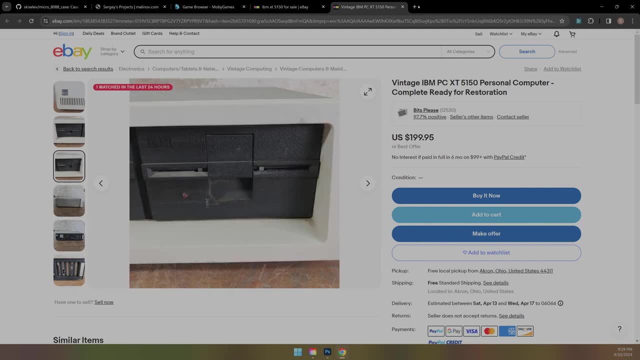 right, cause they were kinda meant for a a big CRT monitor to sit on top. so, anyways, and as I would not wanna buy this one, uh, but we want one, right, we wanna mess around with it. 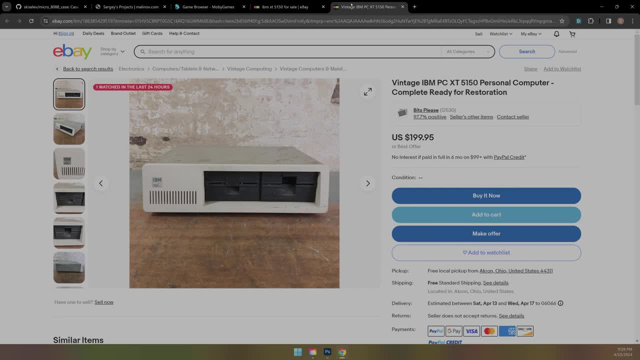 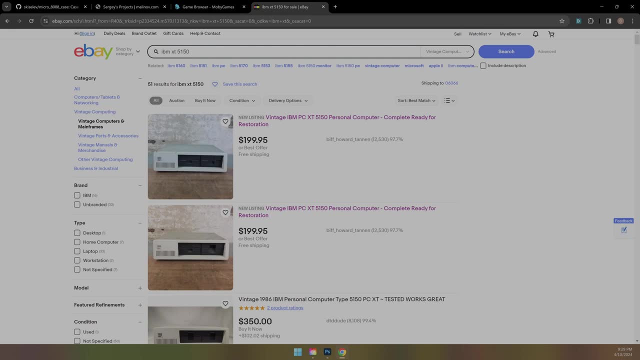 and see what the capabilities of of it are. oops, did I click the wrong button. okay, uh, alright, let me just catch up in. the all the games I've been running have been years 90 to 95,. 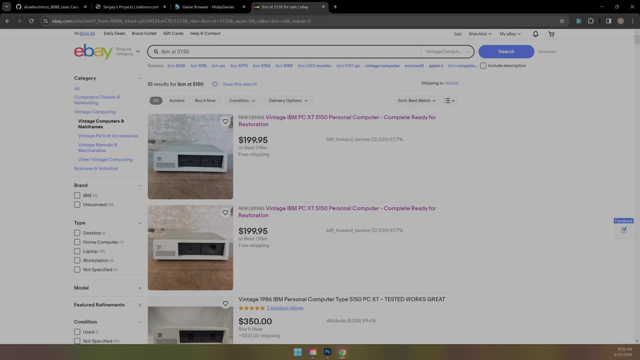 oh, on your um 46,, 2, DX 66, is I'm on, the most versatile platform for DOS games. we don't talk about cost in retro computers. well, see alterations. it the thing is. 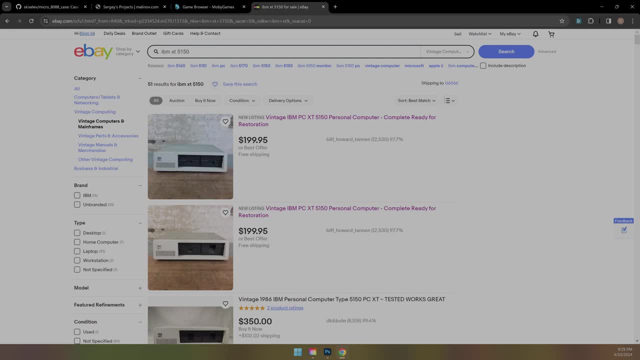 we live in such a crazy good time for open source projects, right like um people that have so all this nostalgia for these old things and that that drives even retro stuff alright, people have this nostalgia. 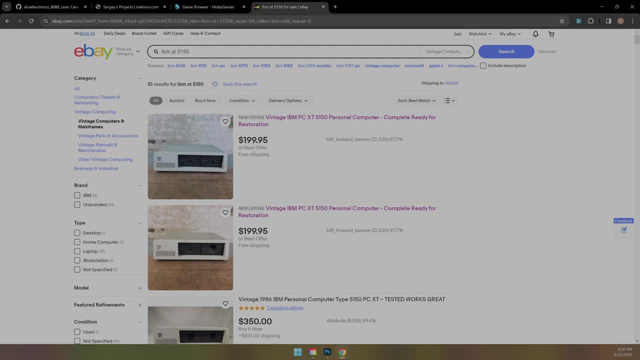 for the old stuff that they used to have when they were younger. or maybe they still have it and they wanna get the best out of it. they wanna see how they can improve it. um, for you know not. 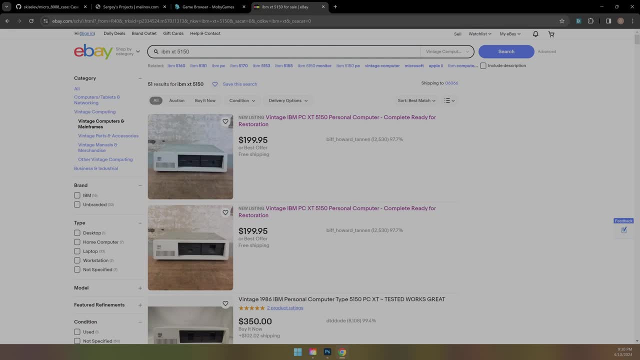 not only themselves, but you know other people. so, uh, I guess that's where this project comes in right. so imagine if you could have one of these. well, there's actually more. there's more to it. 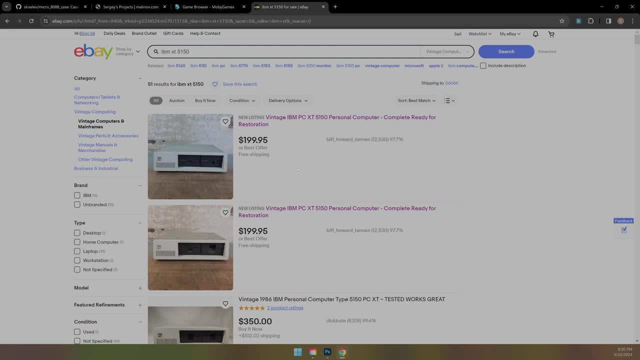 alright, I guess we'll. we'll talk about the, we'll talk about the project and then we'll um cause this? um, I guess I should've talked about this earlier, but this video is sponsored by PCBWay. 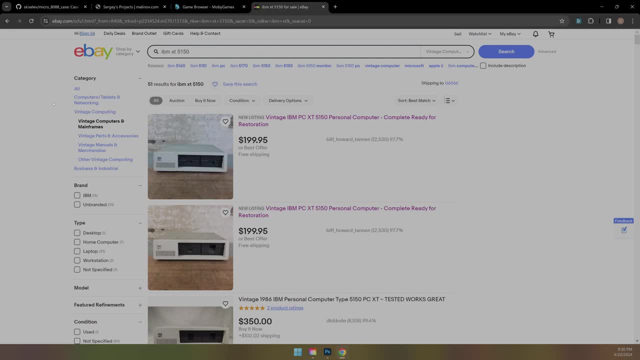 we'll kinda talk about PCBWay more in a little bit when we talk about the project, uh, but I I just wanted to say up front that this: you know, they, they um produce the PCBs that I'm gonna be using. 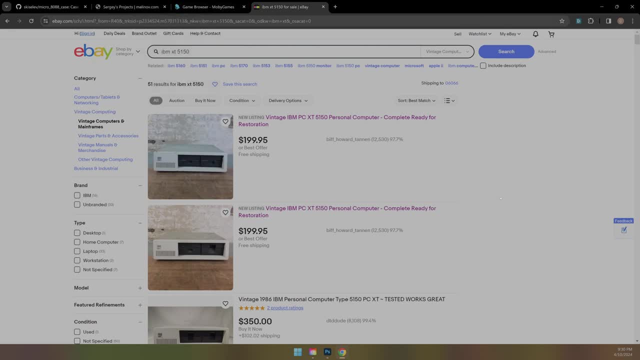 and they mailed them out to me. so, um, big shout out to them. uh, there's a link in the description if you wanna check them out. but we'll talk a little bit more about other things they can do and 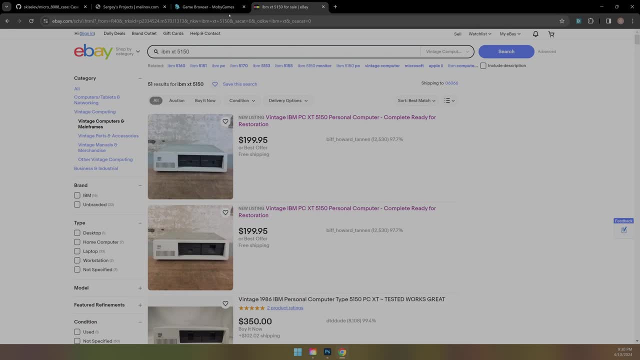 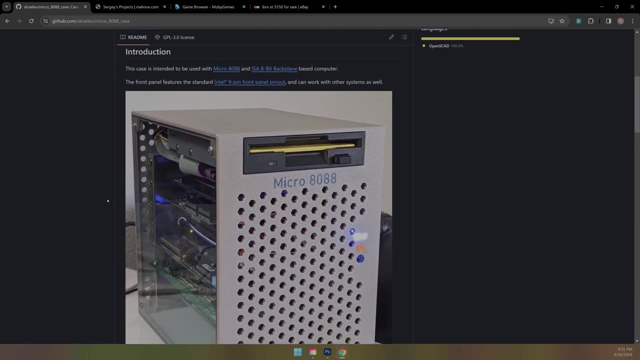 um, yeah, so we'll get back to PCBWay, but thanks anyways. uh, alright, so where's our? okay? so this project, um, we're gonna create um, a, a brand as much of. 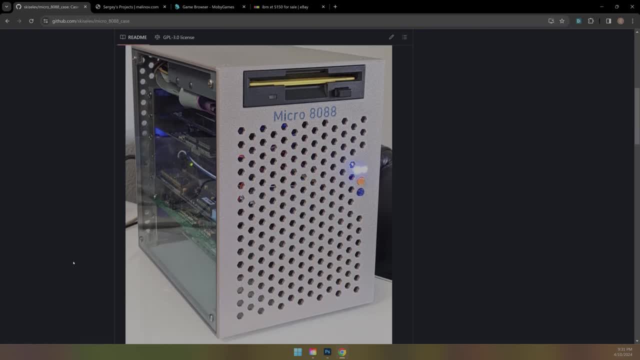 as you can call a brand new IBM PC, right, but it it's sort of like the OpenTendo in the fact that you need- you do need- original chips, some original chips, and we'll talk about what those are. 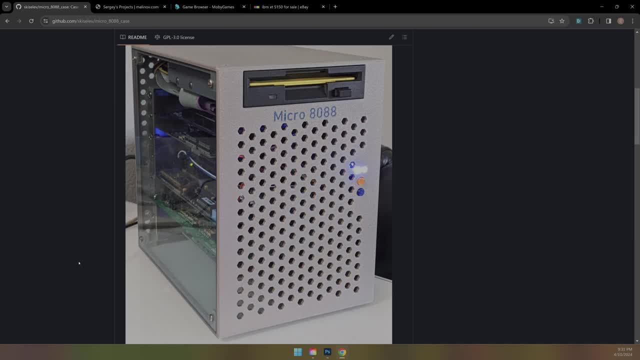 um, but for all intents and purposes, most, most of the components and the PCBs and stuff are gonna be brand new. uh, and you can even choose to not use a if you wanted to not use a flop, a real floppy drive. 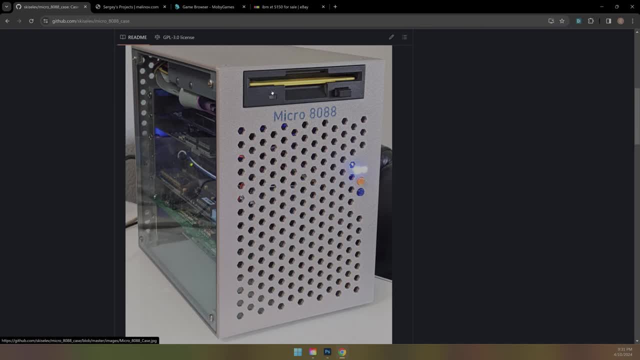 you could use OpenFlops or uh GoTek so you can have a brand new USB, uh flop- excuse me- floppy device thing which you know that's really handy for for me being able to use it. 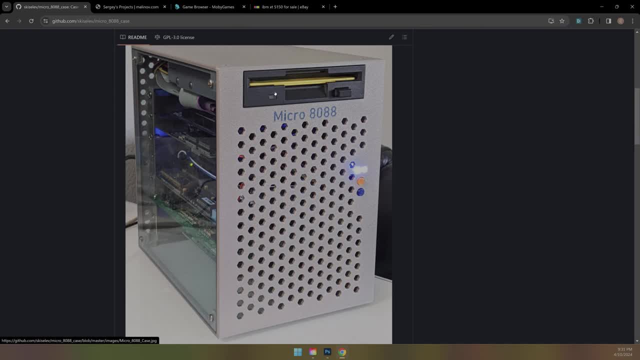 just being able to put stuff on a flop, um uh, USB drive, and then just off you go loading stuff. so definitely handy. you can jam a CF card in an XT, no problem, right, yeah, so you can modernize. 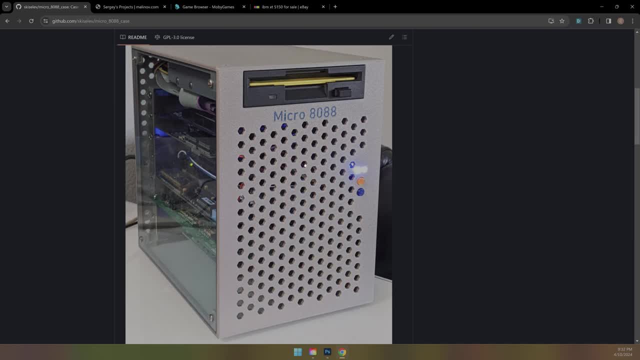 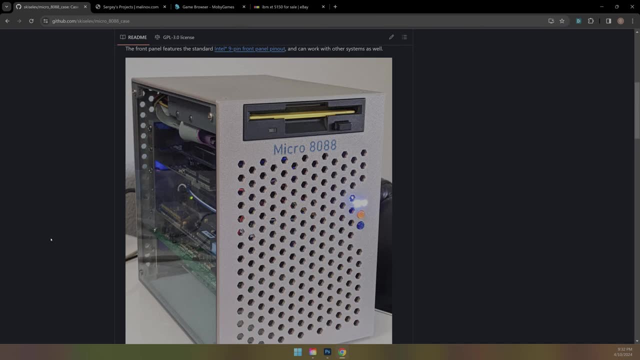 I would say um an, an original IBM. so, like I said I, I modernized my AT, I put a I. what did I do? I had to put a, an IDE uh card, into it. 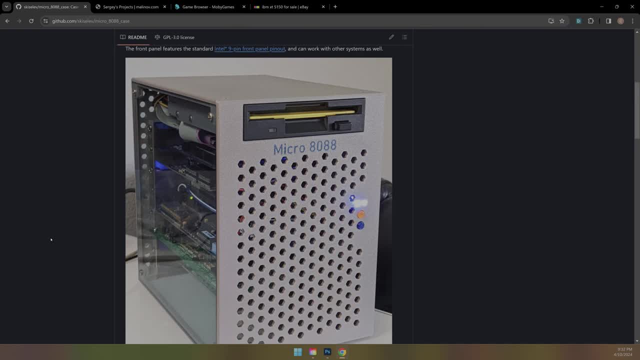 so that I could load um uh a CF to IDE card, so Compact Flash, and then I have uh an XT IDE ROM boot thing that loads the uh IBM or the XTE IDE thing. 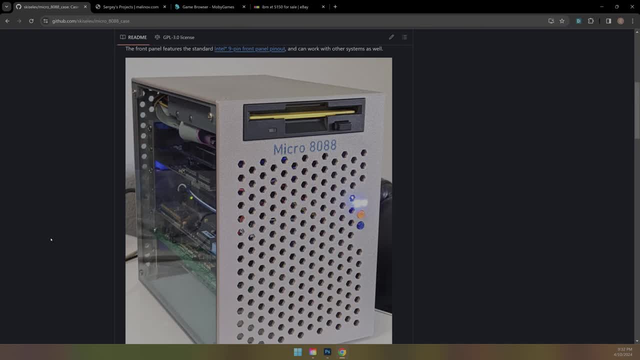 um, so that you can get large. you can, uh, DOS can actually recognize and and use large hard. uh, you know, the Compact Flash drives are a lot, probably an order of magnitude larger than any hard drive at the time. 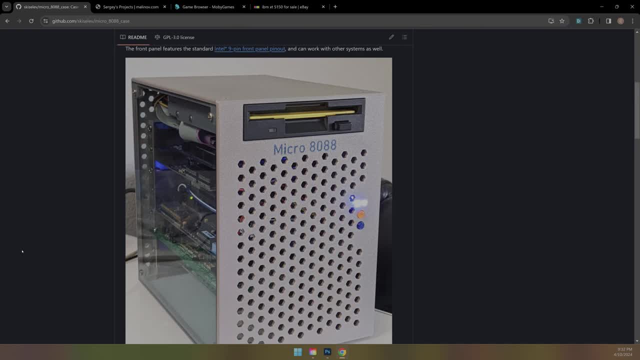 you're hoarding XT CPUs. actually, these use, these use ones that are different form factor. you'll you'll see, um yeah, because, believe it or not, I mean some, some of these, you know. 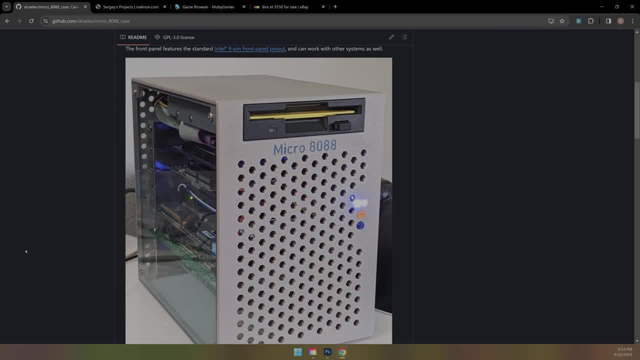 older hardware that have been remade into like embedded systems, because maybe they're you know, their systems were old and they didn't really want to upgrade, so they chose to just make new hardware using the old parts, old spec. so there's all sorts of weird. 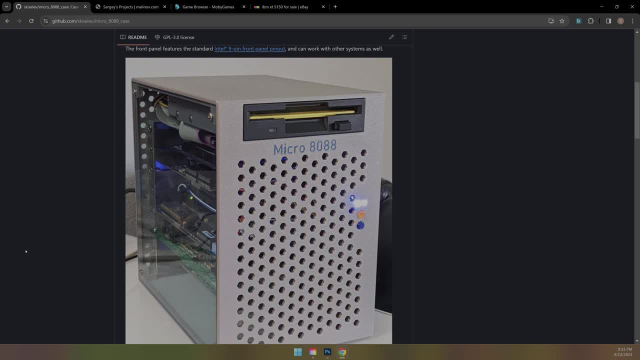 you know, entire board, PCs on a board. so that's kind of what this is, but a little bit, little bit um more string, um separated, and we'll talk about it each little part, Okay so, 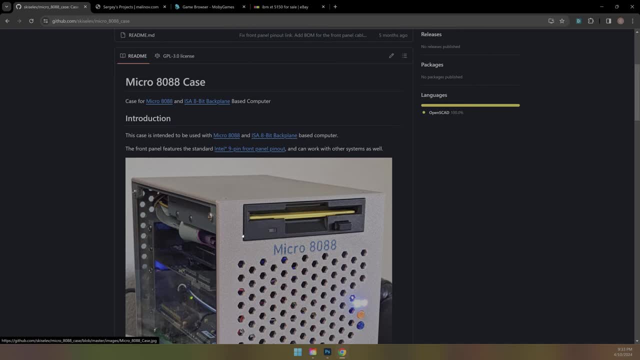 so this is a project. I suppose you already know the case. that's where we are here and this is the first thing I decided to, to just get a head, head start on. so I printed, I 3D printed the enclosure. 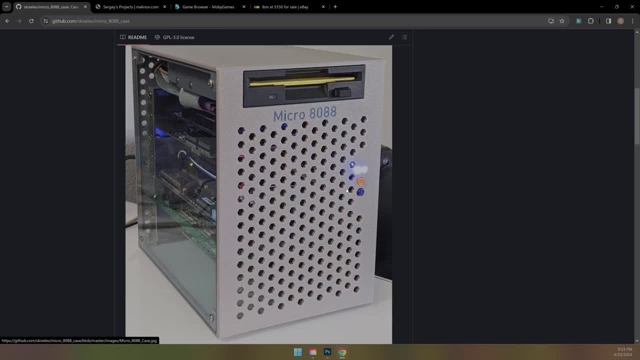 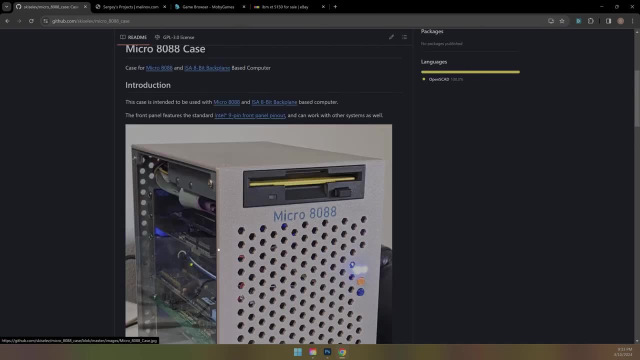 I didn't print the buttons, but there are. there is a start, I think, a power, power and restart, maybe on the front, and some LEDs, and it's got a PC speaker inside, which is kind of cool. 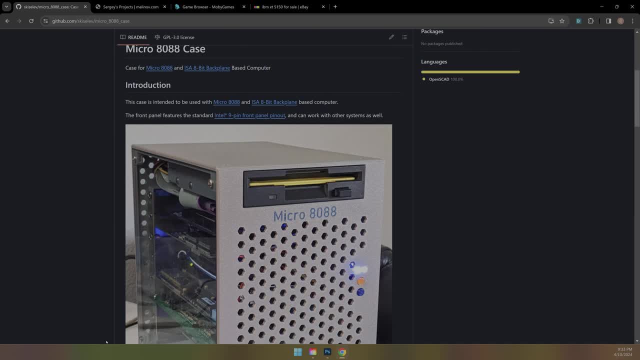 I thought someone had made a floppy hard drive emulator to network share interface. ooh, that's interesting. have I seen the throttle button? No, it's a blaster from scrap computing that allows you to slow your CPU down to play game. 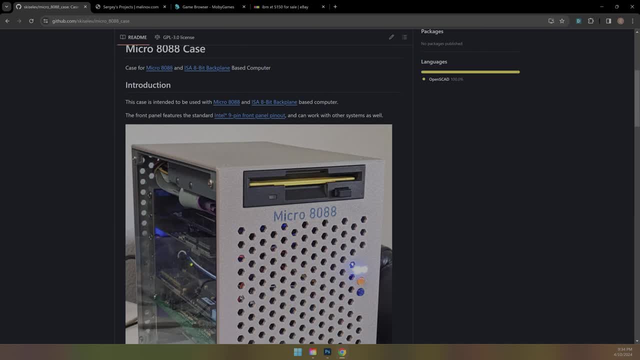 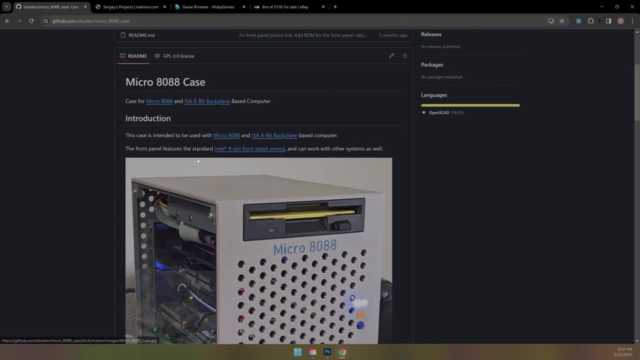 speed sensitive. that's interesting, hey, Bartleby. uh, okay, so let's talk about what um the. the two- I would say the two main parts are what we're going to work on tonight, okay. 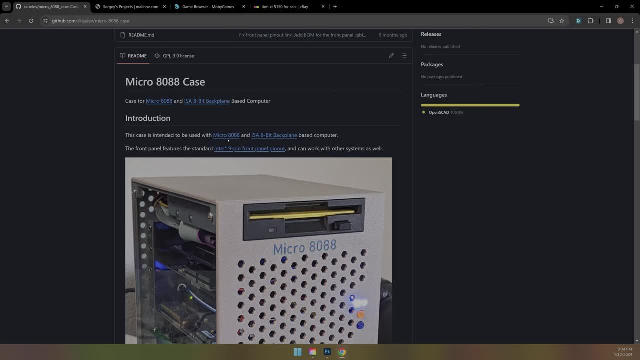 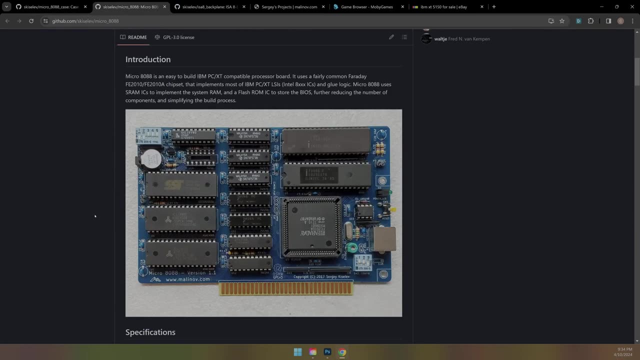 so the Micro 80, 80, the Micro 8088, is well, I will open both of these. is really this part? it's really the, the the CPU part of this whole thing, but it's more than that. 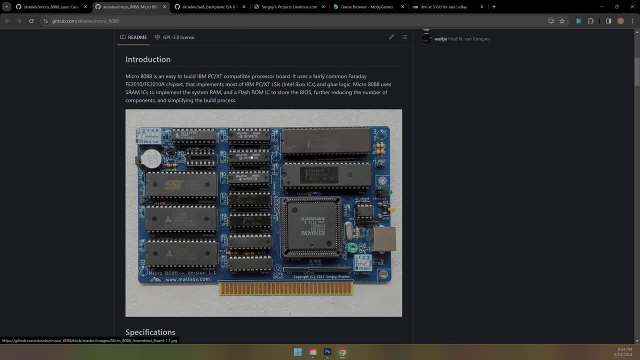 it's really. you know, it's the CPU, it's the memory, it's the boot ROM or the um, one of these? I'm not sure if it's these two things. I'm not sure what these do. 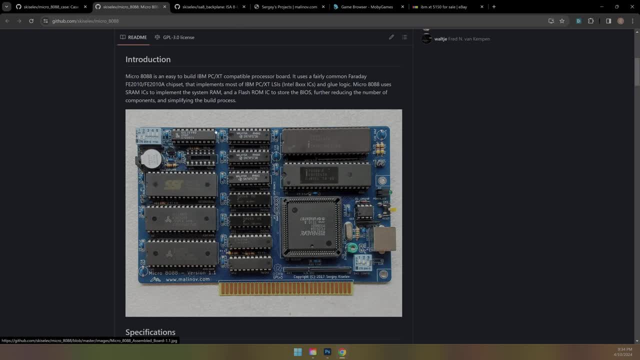 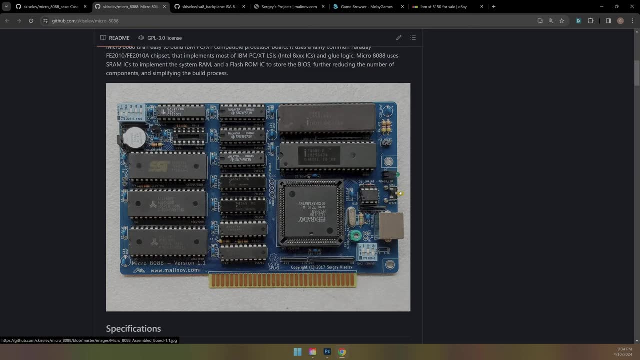 or maybe it's this. this looks more like a, a ROM and the memory and some other things you know. it has onboard, uh, PS2 for a mouse or for keyboard, I mean, and it has I guess. 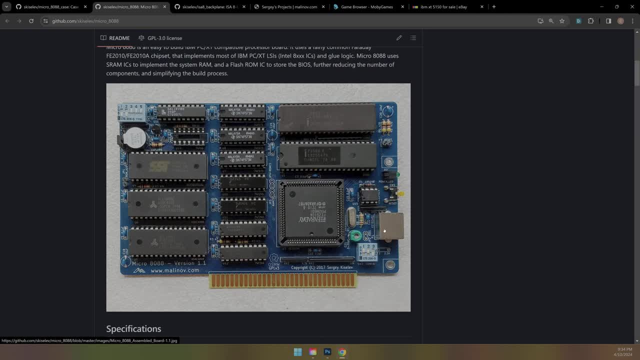 a built-in reset switch in the back. so this already is. you know. you can see the the modernness. that's a bad word, but if you have an IBM class PC like a, either a PC, 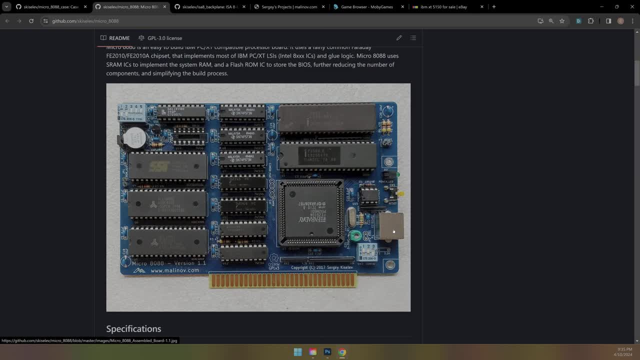 an XT or an AT, there's a chance that you're gonna have an AT connector. actually, I think the PC and the XT have a different connector too, but uh, the AT connector, the, the, the mouse AT connector, is like a. 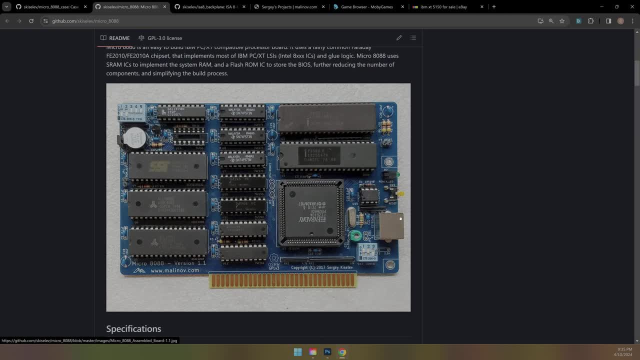 it's like a bigger port than um PS2, so the PS2 port, I think, actually does come from the IBM PS2, I think IBM anyways. so they, they like name all a lot of this stuff after. 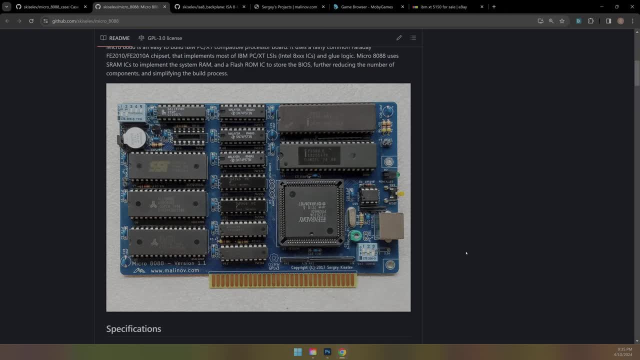 uh, IBM stuff, uh, so you can already kinda tell that this was aimed to be like. uh, um, first of all, super compact. right, it actually makes use of this, this chip here, this Faraday chip. 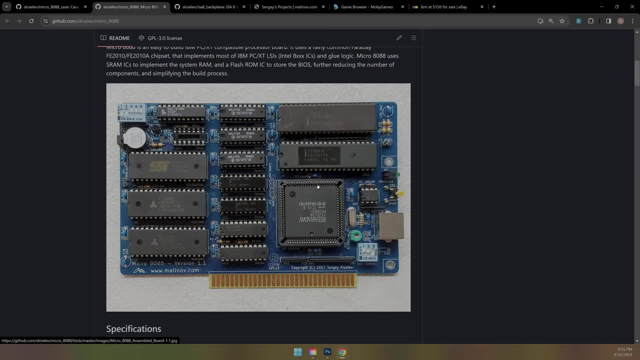 is. it's a chipset that has basically everything integrated into it. um, so it's normally, if you look at a real IBM PC or AT or XT, uh, motherboard is just stuff all over the place, right? you see a ton. 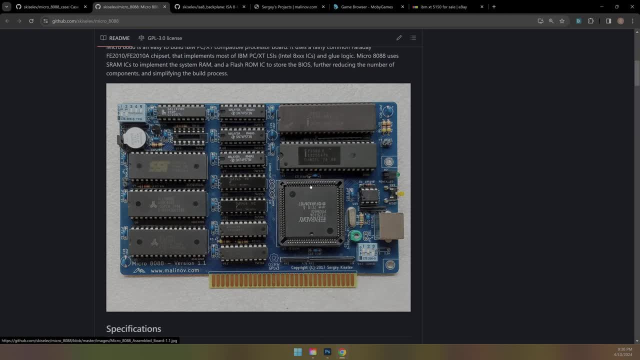 not discrete components, but you do see a lot of like logic chips and stuff on the board and you know, as computers got smaller and more manufacturers got involved- um, you know Intel and things they would start developing. 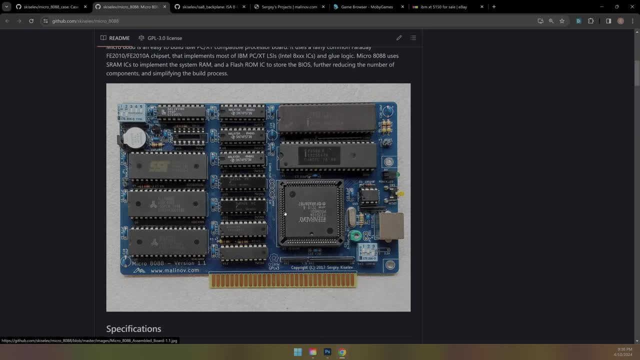 chips that would kind of accumulate a lot of the functionality into these smaller chips. so I guess they had more features inside of one chip. so this, basically this, the smallness of this project is uh. 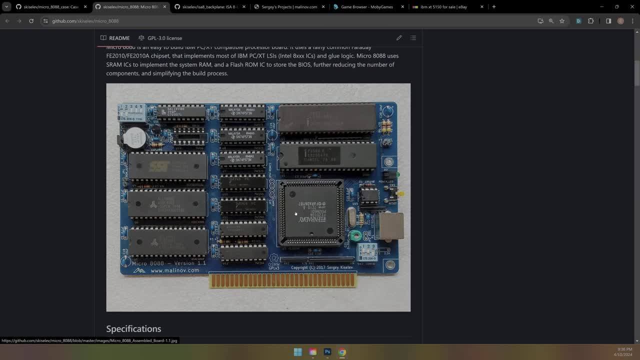 enabled by using this Faraday chipset chip. so I've got one of these and the 8088 that we've got is uh, I, this is a real one. I believe in this picture, but I have a. 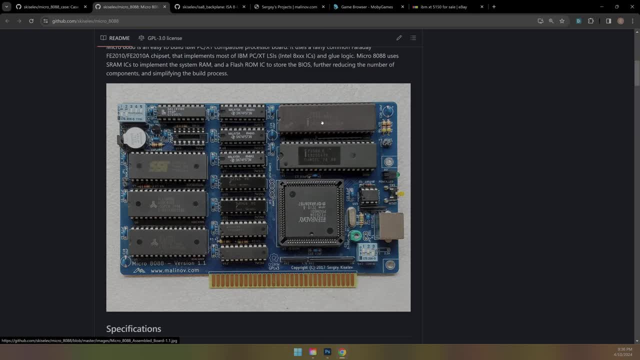 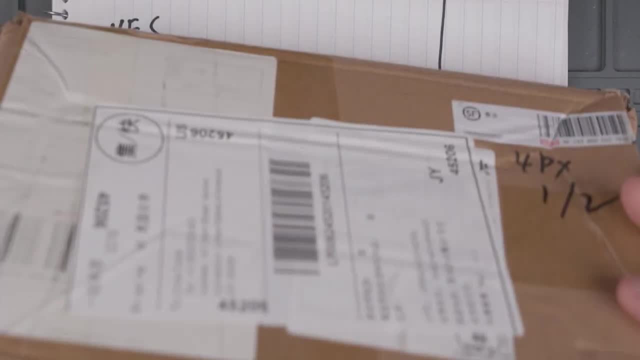 let me see, let me get my bin of parts. yes, okay, we'll look at the. we'll look at the PCBs in a second, but, um, so this is the processor that actually I think they sent me. 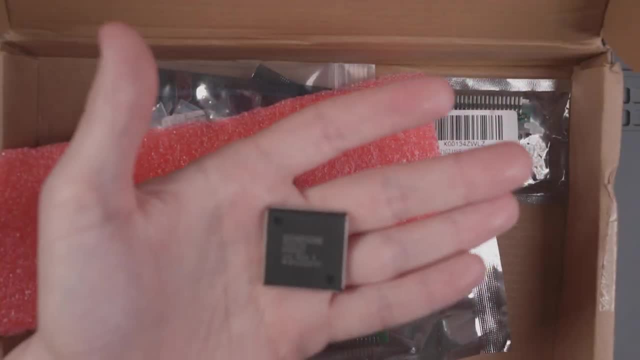 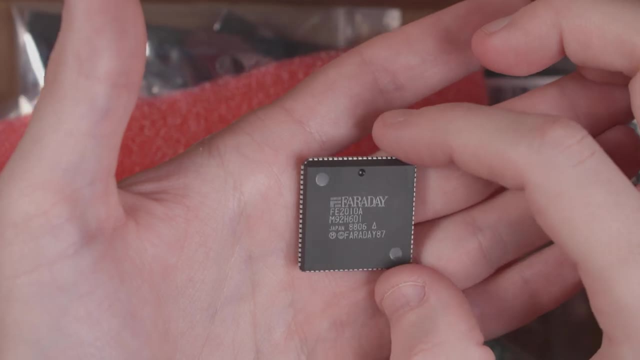 when they sent me the Faraday chip, this Faraday chip um which, if you are gonna be, you know, these are not. oh, I think that these were kind of expensive, or at least this might have been. 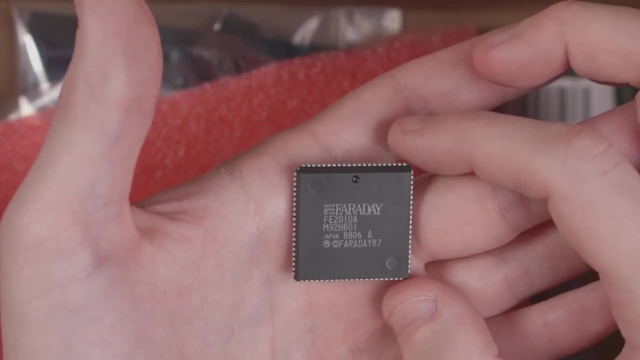 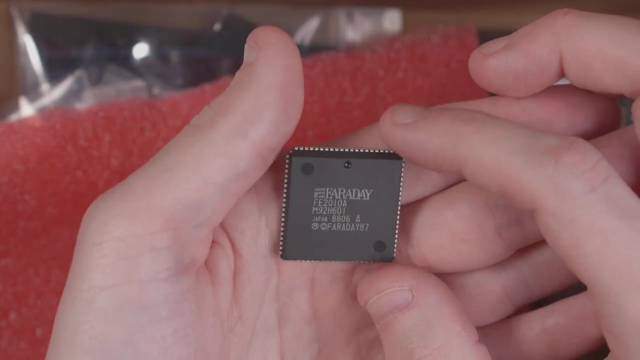 it might have been 30, or 40, or 50 bucks or something um early mice use DB9 serial. yeah, I've heard of uh. what is it called uh? so I have this, the Faraday chip. 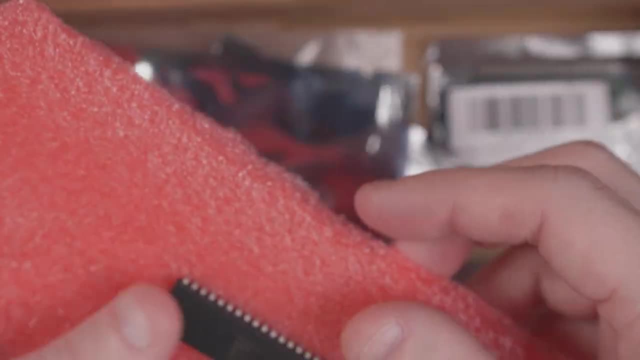 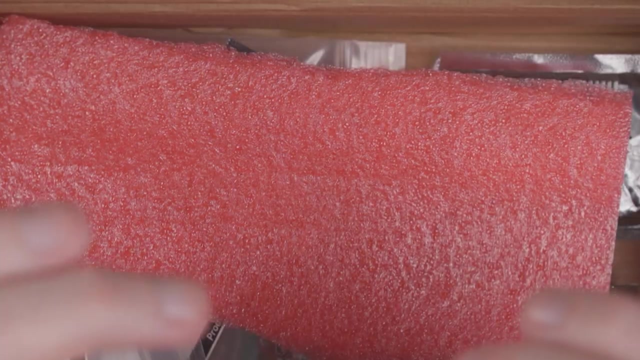 so that's kind of the most important thing that enables you to build this, I suppose. but here is a CPU. I think they sent this to me, so mine is an OKI. I hope this will work. it's an 80C88A-10,. 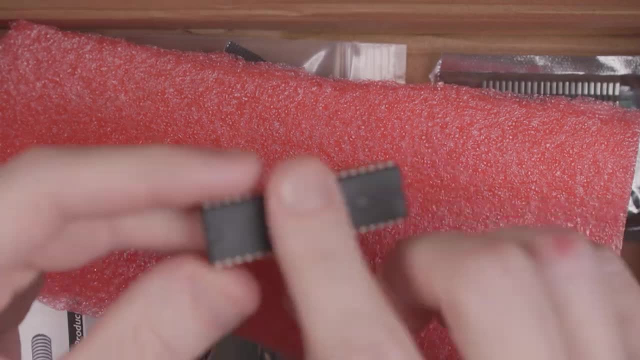 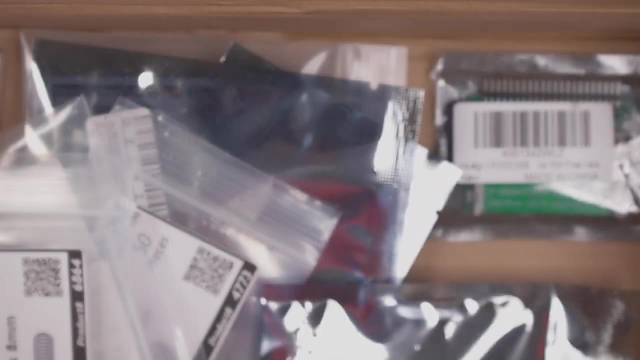 so 10 megahertz um 8088, which is faster than the like the stock, the stock clock speed on the original IBM 8,. uh, XT would have been 4, it wasn't until the 286 that they got. 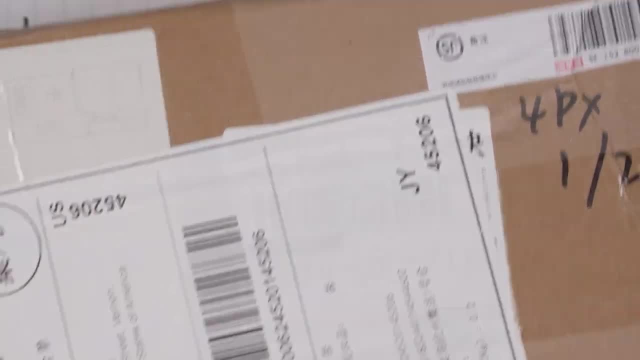 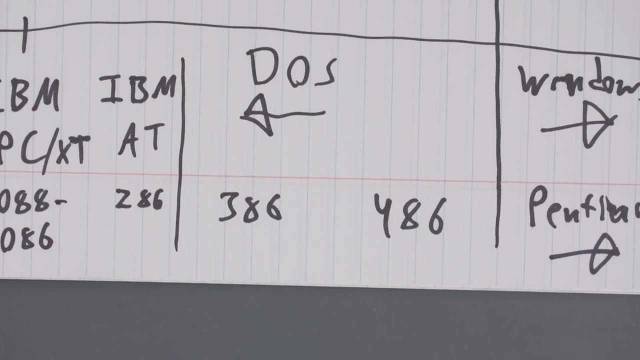 8, and 12, and stuff. oops, that might have had my name on it, rip. OK, so go back here, oops. so that is the main part, and I've got the PCB. where is it? 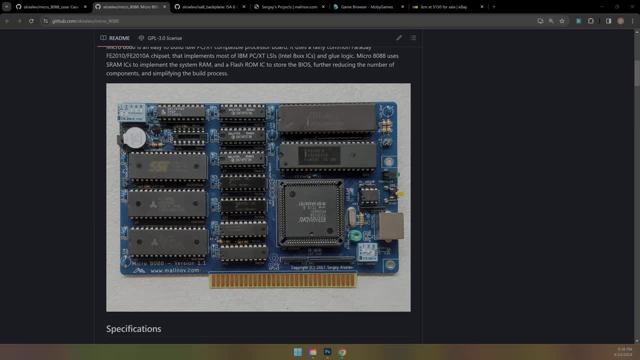 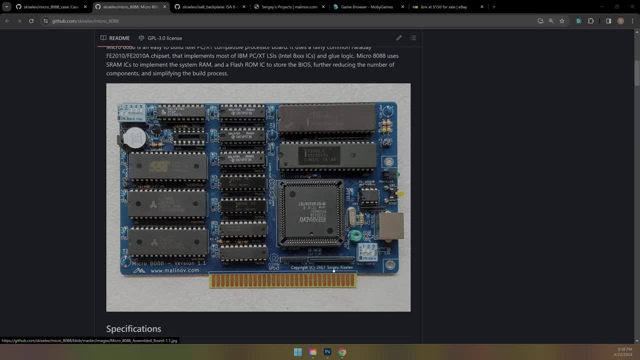 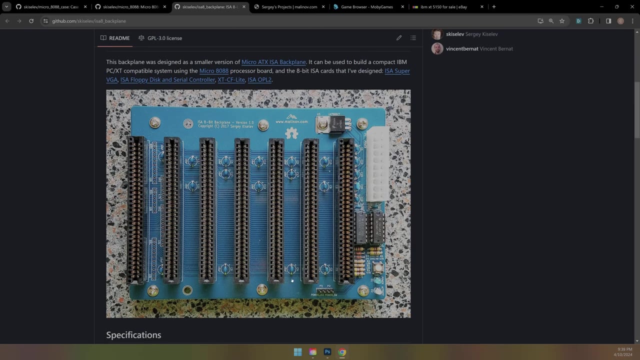 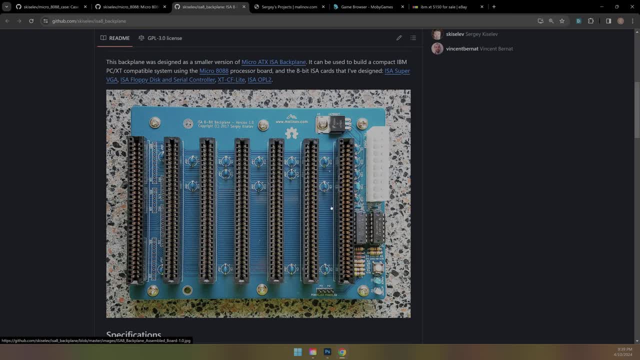 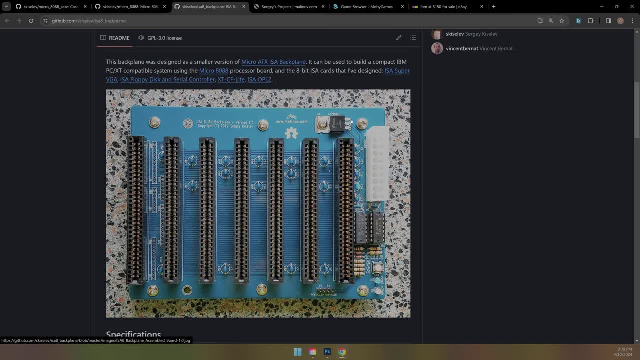 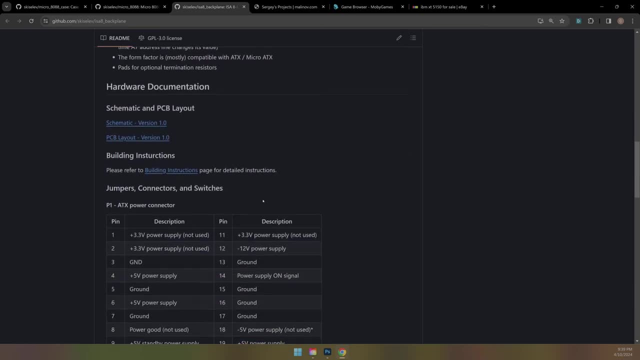 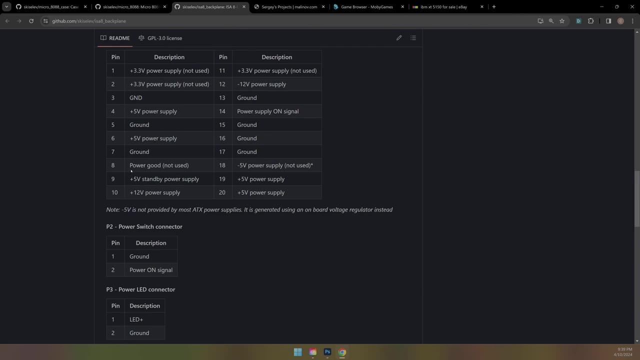 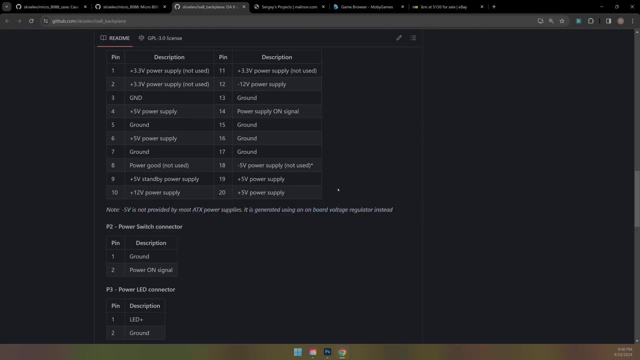 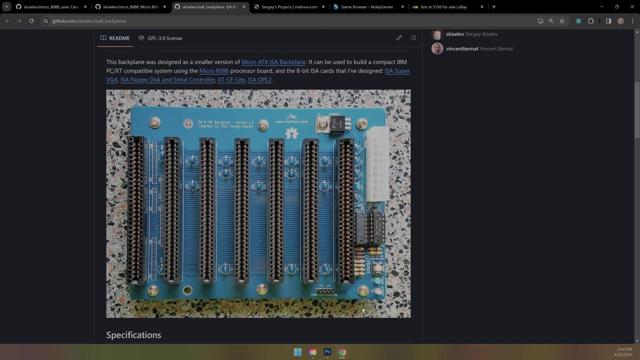 generated using an onboard voltage regulator. okay, so it looks like they're generating the negative 5 volts on the on here, maybe this thing. so this is a kind of a cool way to get all the other functions to interact with the PC. so you have a nice. this is kind of set up to use the Pico power supply, right. so 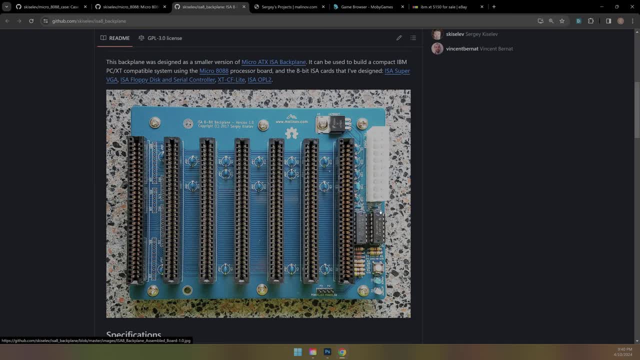 like you. there's a version of the Pico power supply that just like slots their sockets, like right into this thing, and then you have just a button that kind of goes to the outside of the case and you can just turn it on and off. so that's. 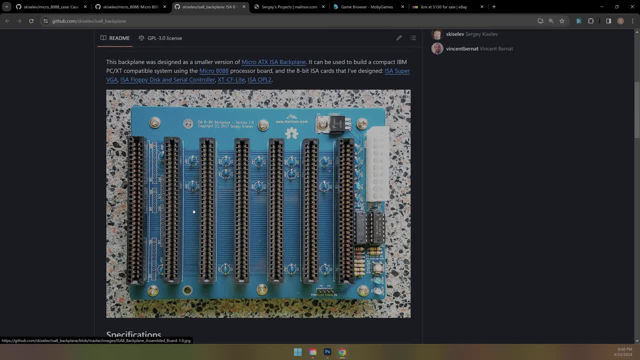 really kind of neat and you know all your other functionality would just be, it would just come from your add-on cards. so to kind of round this out, like you saw, there was that floppy, floppy drive in the front of the case, but you don't have to worry about that, you don't have to worry about that, you don't have to. 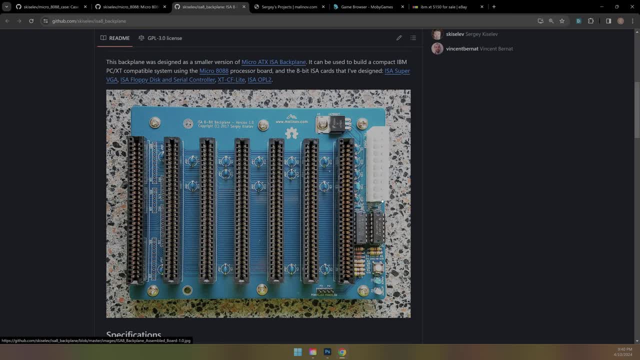 definitely want a. you would need it like some kind of a hard drive controller. well, so they're using the stack. I guess actually they're telling you here the rest of the parts, so that you know you get the micro 8088 processor board, this backplane, and then the whole rest of the project revolves around using this super. 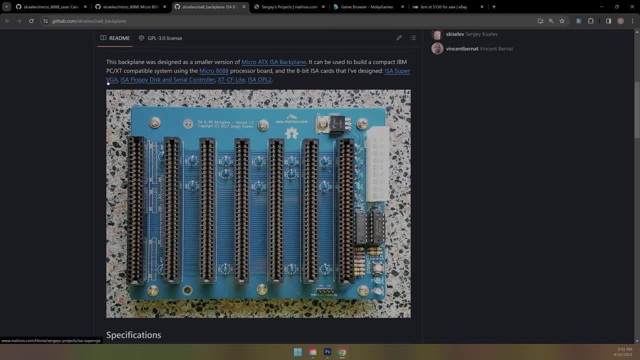 VGA, which is a, not a clone, but it's using old chips on a new board, again, kind of like the CPU board. so there's a VGA graphics card, which is nice. there's a floppy disk controller, which is what connects to the floppy drive, right? so you've got your floppy connector here. 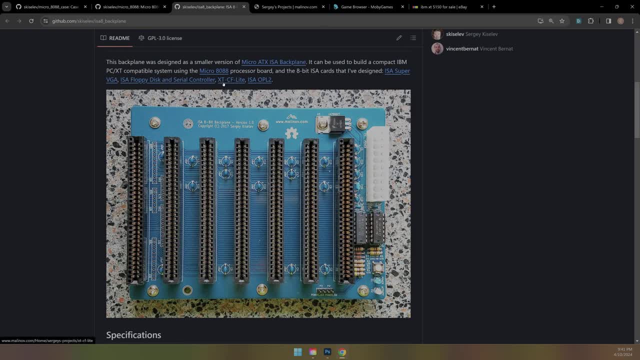 and then for a hard drive, instead of having a like a MFM card or a IDE controller or something, you would just use this XT CF light- I guess- board, so that gives you compact flash kind of in a small form factor. and then for a sound card, there's this ISA OPA card. and then for a sound card, there's this ISA OPA. 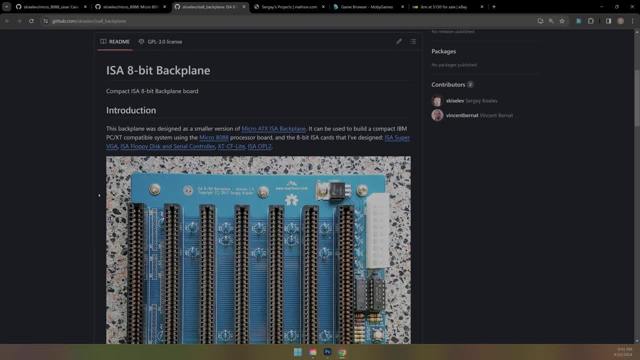 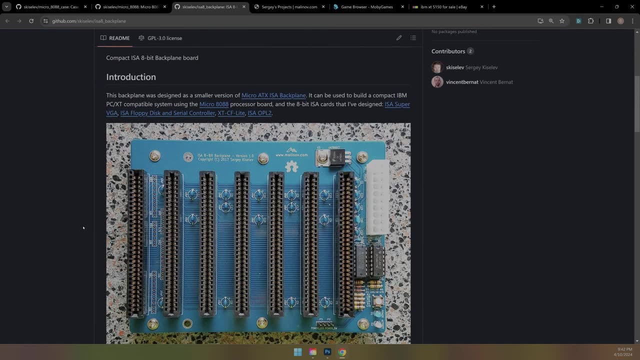 two projects. so all these, all these sub projects are all from Sergei on their on their github. so we're gonna start with these parts and, like we, probably we're definitely not going to get through the whole build. I mean, we're not gonna get through the CPU build, probably the CPU board build, but we're gonna start. I. 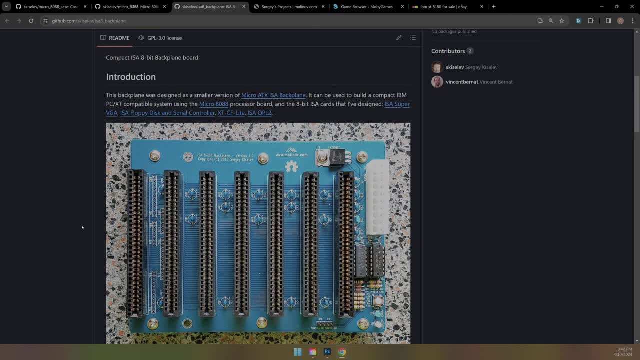 don't miss having to have ten cards to do everything. yeah well, it's funny cuz my, my, I'm like I have a lot of old computer stuff to deal with now and I'm like what's the point of having to have a new computer and I have a lot of old? 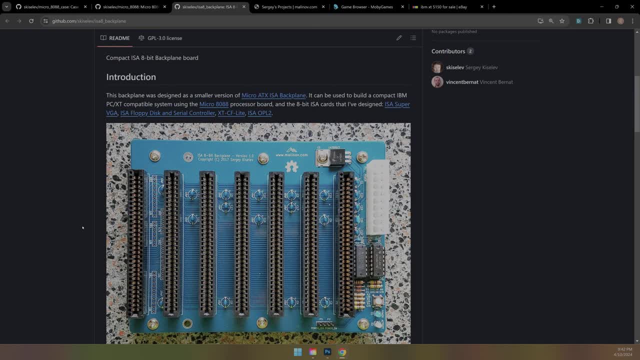 computers and I have a lot of old computers so I get to sort of like capture PC. it feels like that because I've got so many cards in this thing it's like literally there's no slots left, but yeah, but I mean that's kind of part of the fun, you know, of putting together of an old computer, is like. 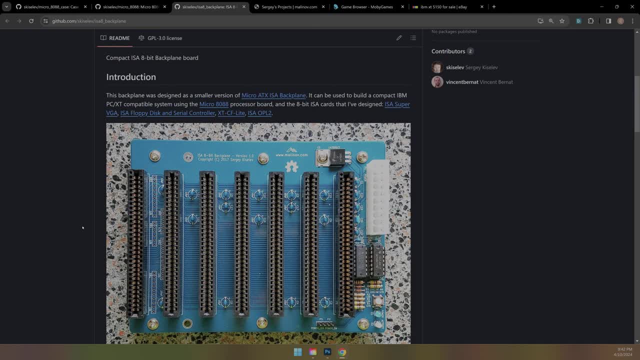 exploring what all the cards do you like? yeah, I don't know. when I was younger I was very excited about all different kinds of cards and things. yeah, I don't, I just from a less to break sort of thing if i don't know who's walking around their computers. but 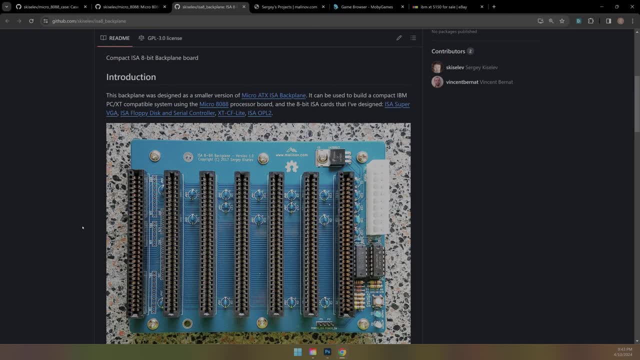 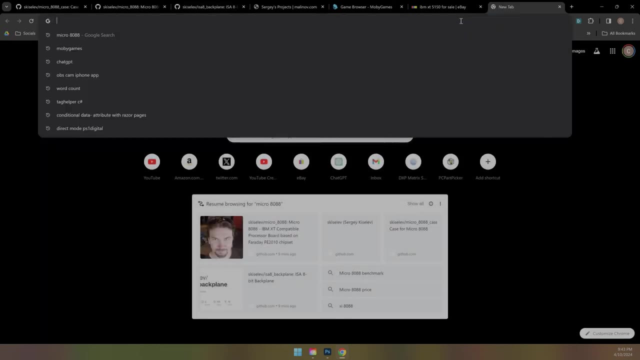 um, you know i don't mind it. you know the stuff is inside and not really visible that well, but uh, yeah, working on them is not as fun for sure, just because there's not as many things, okay. so i guess i didn't really have anything planned of what to say, uh, but i just want to. 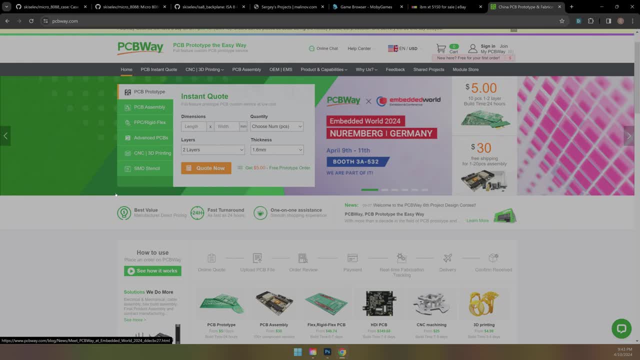 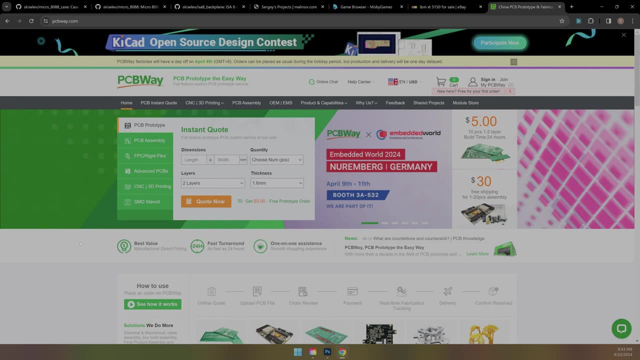 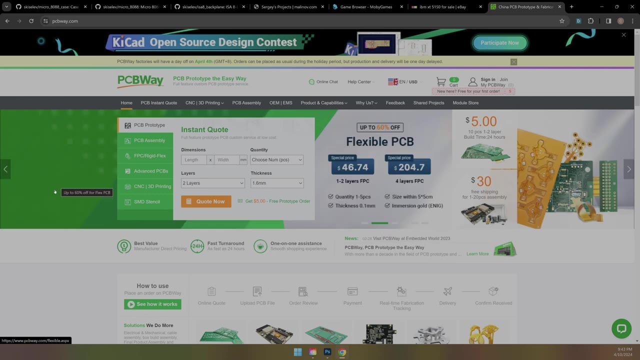 talk a little bit, i suppose, about pcb way. so this is how i where i got the boards created and, just for your information, these are well, we'll talk about, i guess, um, when we start, but they are enig. so this, these are higher price, uh, pcbs, so this is not an inexpensive project if you. 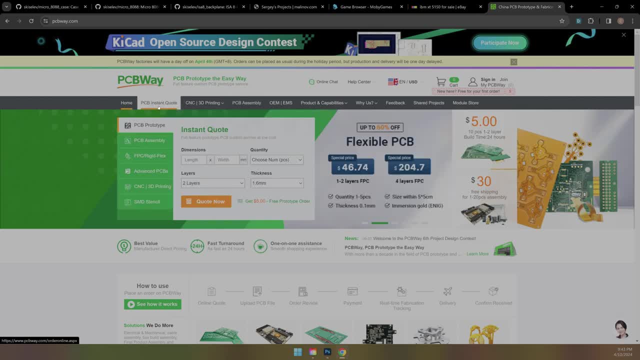 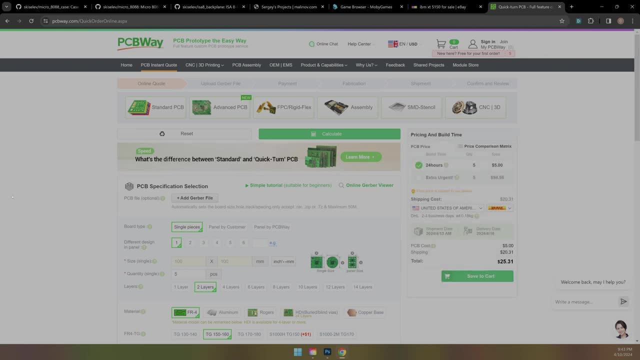 do enig. but um, yeah, what you'd have to do is you come in here and then you'd go to like quick order and then you can just upload the gerber file. so there's a bunch of gerber files for each of these projects. so to follow along with what i'm doing, you would just need. 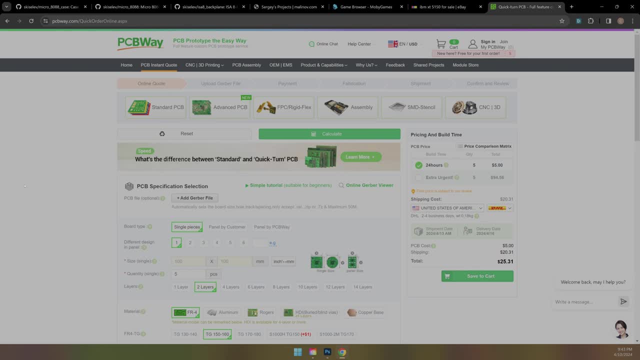 the micro 8088 one and the backplane one. i have a whole bunch of other things um that i'm gonna like. i have a pc power supply, like a, just a atx power supply that i'm going to use to power it up. so i'm not going to worry like i'm not going to get that far. i'm going to do it in chunks, i guess. so 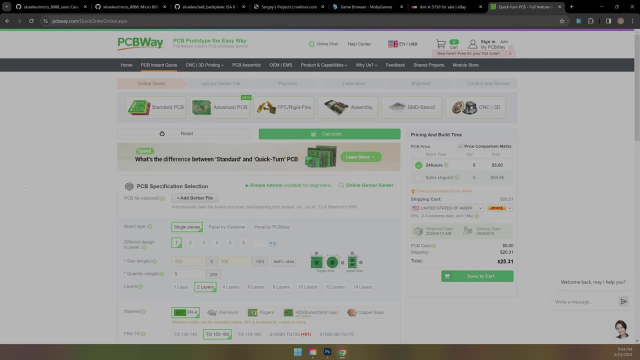 like in the future i'll do the the video card and the sound card and the ibm or the xt ide card and everything. so i'm going to do everything from that list but, um, just kind of piecemeal and use, you know, test the computer with what i've got. 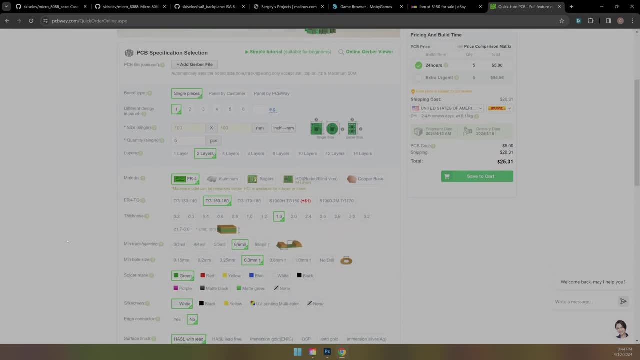 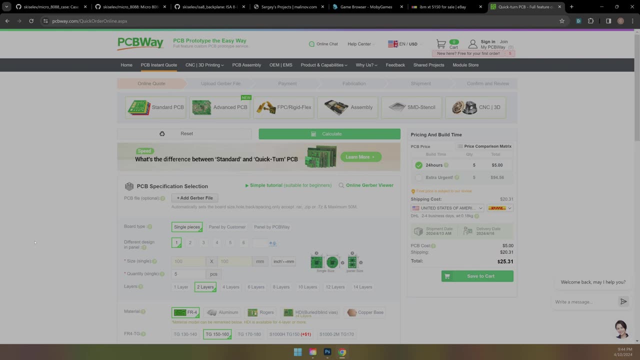 already. uh, so i- you know, i'm not sure how familiar like. so i i guess for a long time i've been kind of trying to get people to be more interested in building projects, right, like actually ordering the pcbs and stuff and soldering stuff, especially things that are um hand solderable, like i've done. 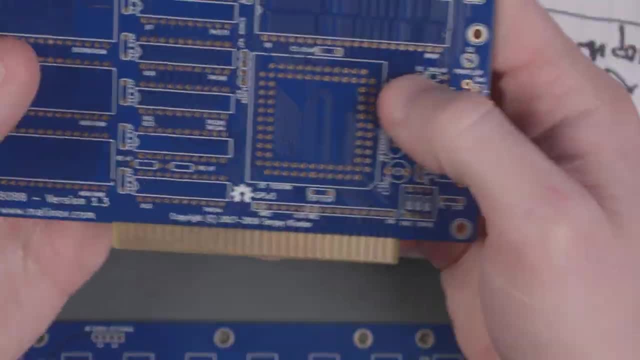 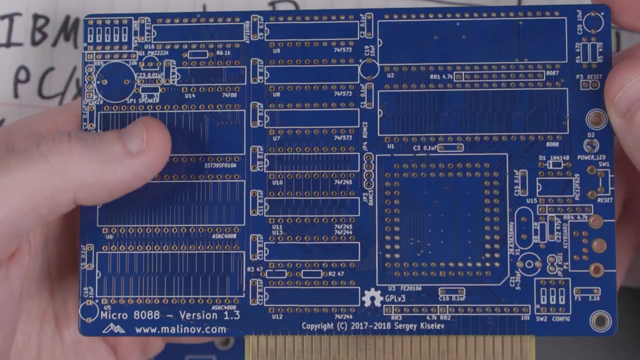 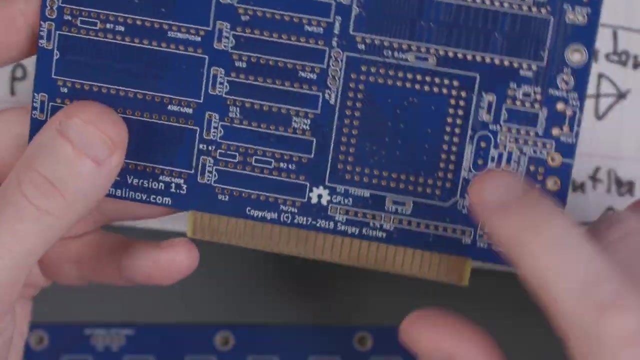 a bunch of projects that have been kind of a nightmare, but this is mostly through hole solder, or actually it's all through hole soldering. so this is a very- i i wouldn't say brand new- friendly, but it's pretty new friendly right. i mean, i don't you know, especially if you get the um enig boards. i mean, these are pretty. 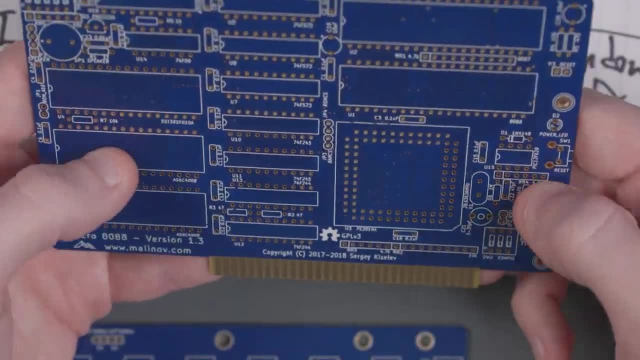 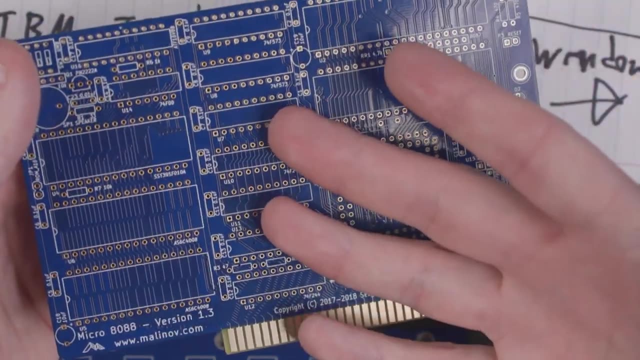 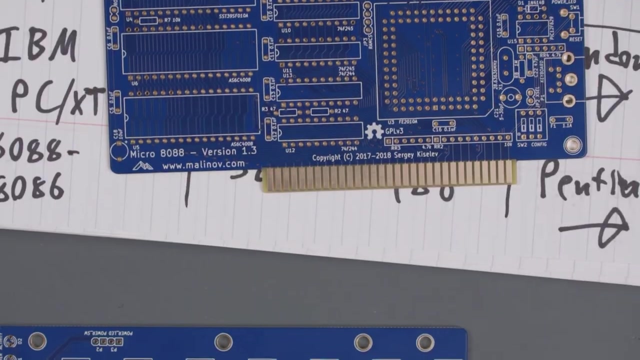 these, these pcb way. pcbs are pretty durable, so, uh, they'll might. they'll take some heat abuse. i suppose the parts themselves, like the old parts, might not, but the good part about this project is 98 of it is all is new components, so it's really not that bad. um, so, yeah, uh, i guess. 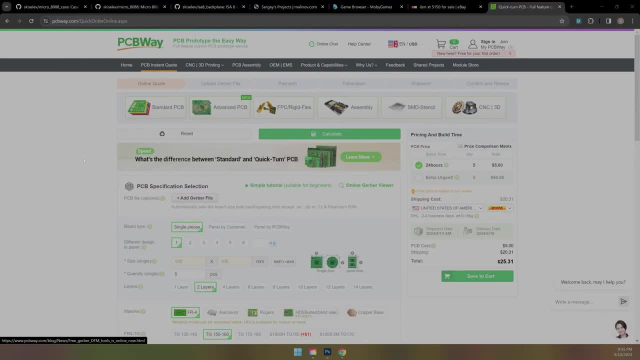 we'll talk about before we move on. um pcb away. does do other things besides just make pcbs. or you know they have a pcb assembling, um setup also, which i haven't really explored yet but because i always like to do it myself. but you know, i might have to try it with the um, i don't know some some. 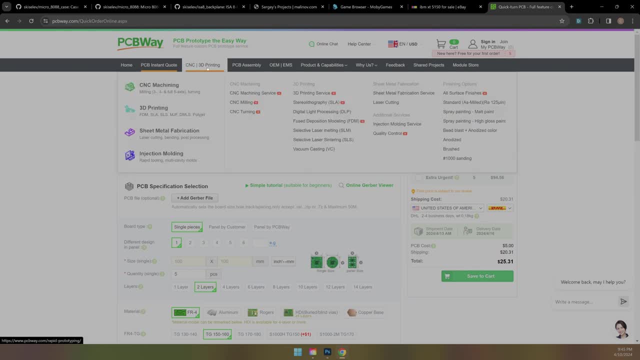 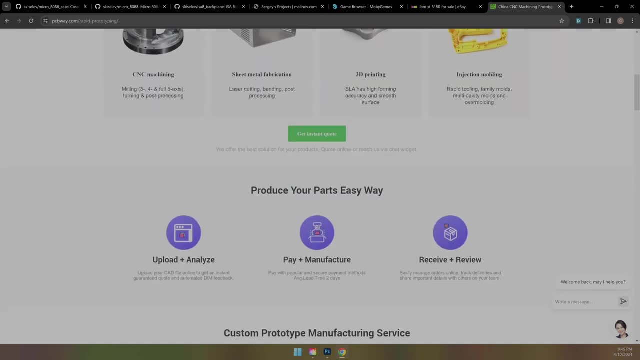 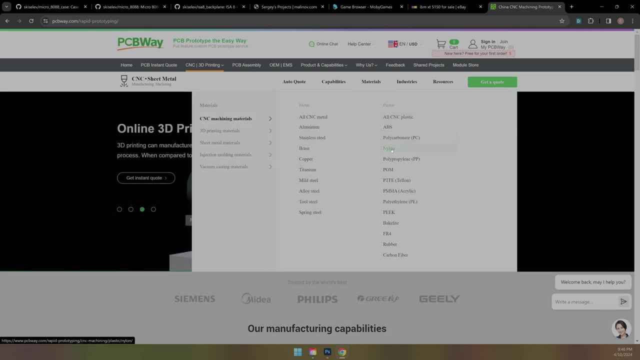 pcb assembly stuff, but their other main stuff is they do 3d printing and not just normal 3d printing, you know, like pla stuff, the kind of big, big ticket i stuff. i guess let's see where's our. uh, i can't see underneath that. the things that i like that they could do are: they can do nylon, but they only. 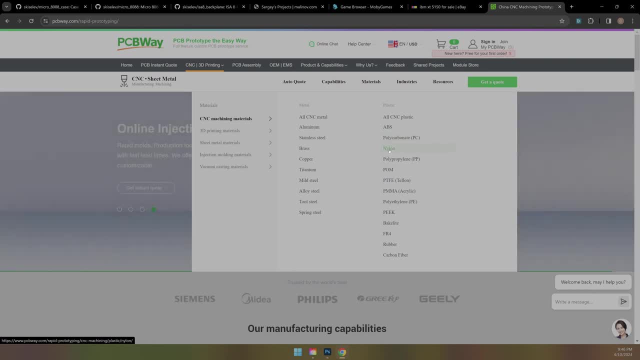 have one type of nylon, but that would be like if you ever saw my ashita, my black ashita case that i made once upon a time, or i had made for me once upon a time, that was nylon, so that's nylon. and the other one is: uh, where is it? what is it called? 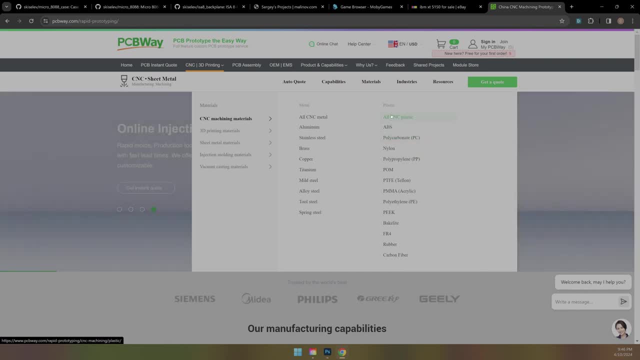 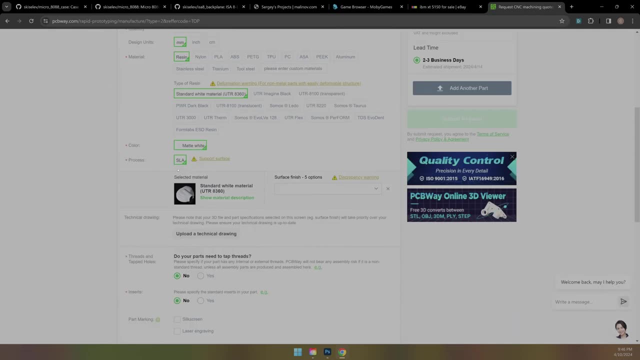 oh, i guess it wouldn't be cnc, what i'm in the wrong thing. oh whoops, they do cnc work too. that's what i was on the uh utr, the translucent, um, where is it? the transparent one? that's what. that's what it is, this clear resin, which is what i use to have them, uh, make the ashita shell. 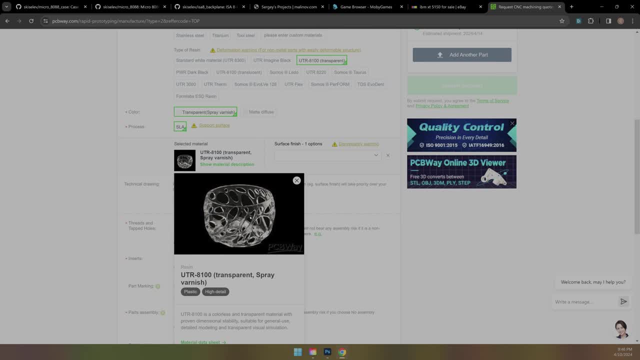 so this is kind of a cool way you can get like pretty see-through, like if you're, if you're making something like a game boy or something and you want it to be completely transparent, like they do a nice job with this. so, um, that's you know. so besides making pcbs, they can also do 3d printing. 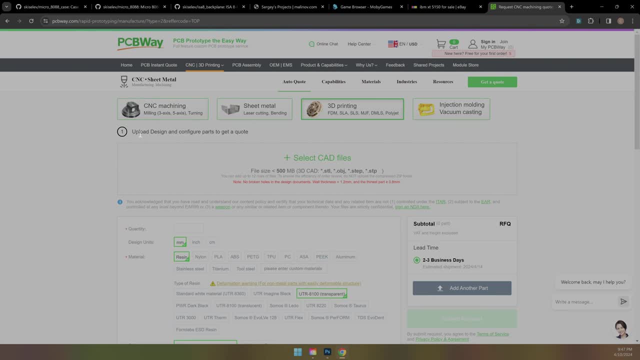 and and sort of like sophisticated 3d printing stuff and cnc machining, and they even do some injection molding stuff. but i don't really know much about that. but that's just the capabilities of your creator. you want to check them out? uh, okay, sorry, all right, so that's pretty much enough about pcba, but thank you again for for them sponsoring. 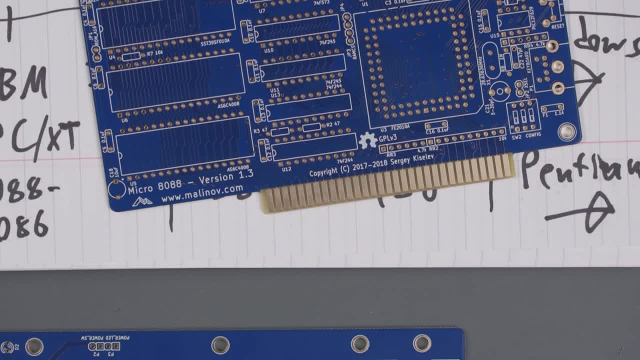 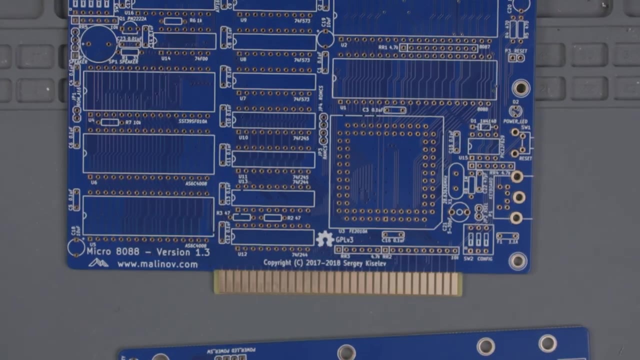 this video and this project. so, yeah, let's talk about our sponsor. yeah, let him cook. uh, we will let you in on all our raid shadow. yeah, right, yeah, you guys should wait for my raid shadow legends sponsorship. it's gonna be great. no, just kidding. hey, i don't mind the the pcba sponsorship because i know you know. 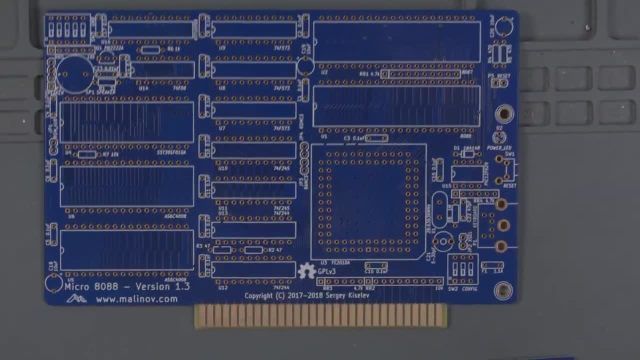 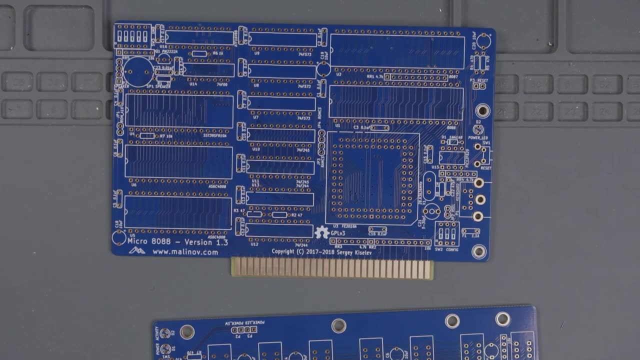 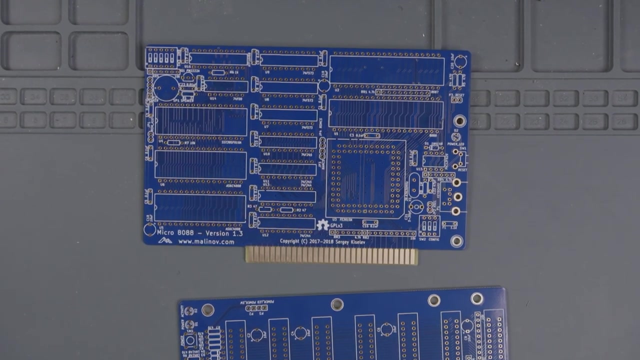 it is a pretty good sponsor to have if you enjoy building pcb projects. so and they, they for- you know this is kind of like off the record- they do seem to sponsor a lot of independent people, so kind of you know kudos to them because it's, you know, my, at least my- experience has been very pretty much hands. 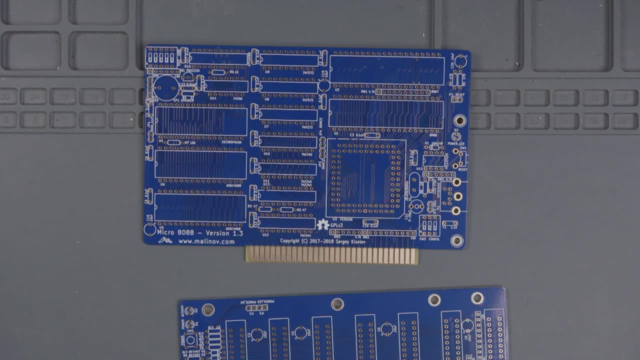 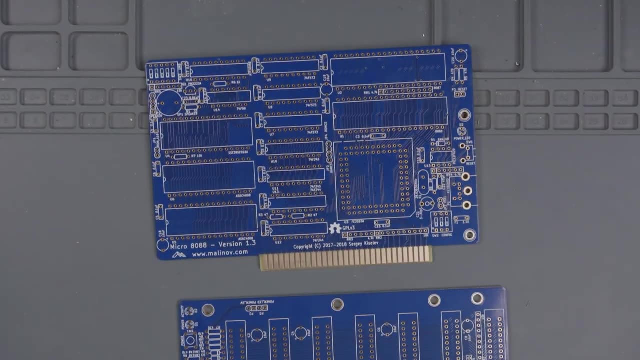 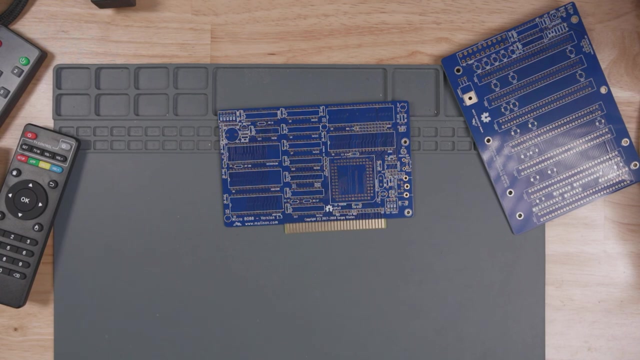 off. right, it's up to the creator to be to be creative as far as how they do sponsors and things, and, um, yeah, they seem to like to support people, which is cool. all right, so let's just shut up and get started. oh, i didn't even mention the giant. oh, yes, okay, before we actually start, i do want to mention this in: 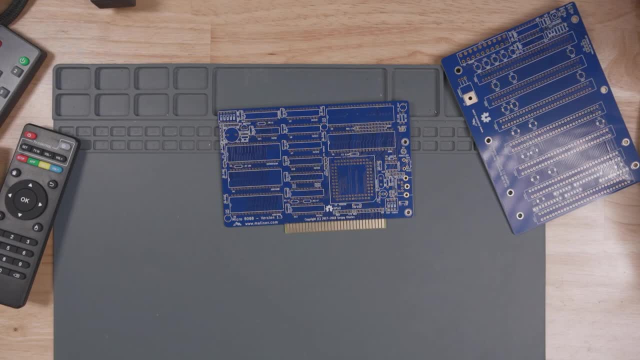 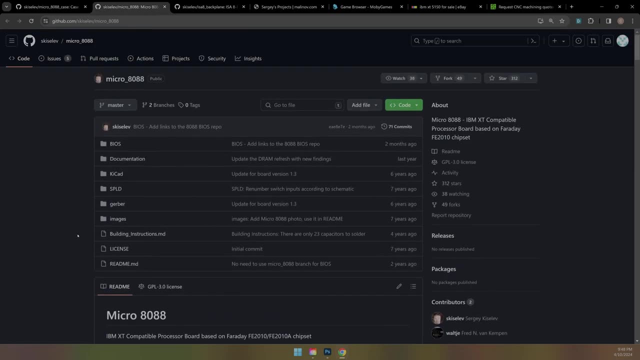 case somebody else is working on this project. i do want to talk about um, not pcbway again. i want to talk about the bill of materials, because the bill of materials is a kind of a pain in the butt for this project and the backplane, and i'm imagining all the other ones too. so, unfortunately, 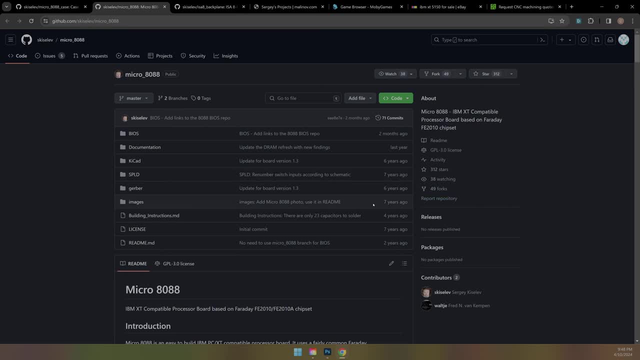 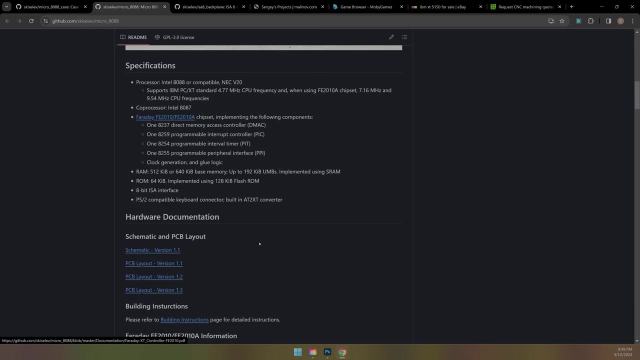 this project was built, or was created, to support people, because i've been very interested in the created a while ago. The copyright date on my board here is from 2018.. So while this is a brand new making of that board, the project is kind of old There is so basically along. 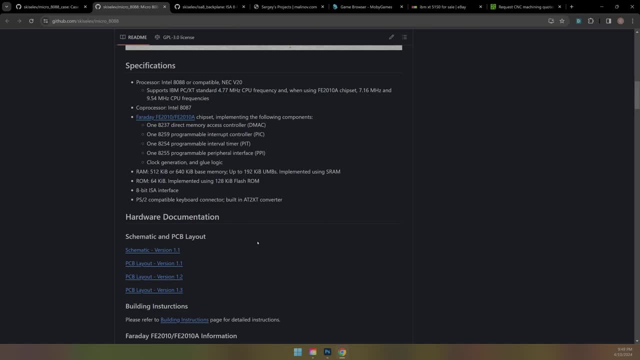 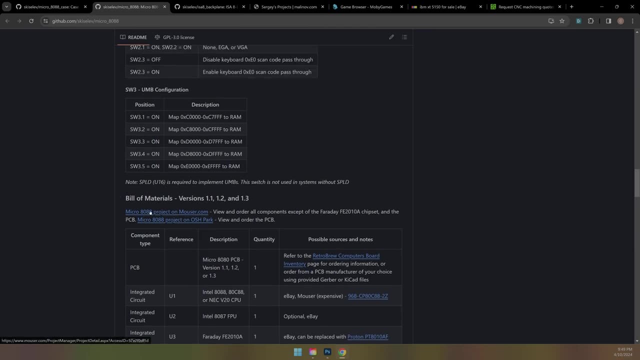 with. along with having someone like PCBWay build or make the PCB for you, you also have to get the build material stuff, which they kind of made it nice and easy. There is a link toward the middle of the page that says you know, micro 88,, 80,, 88. I'm never going. 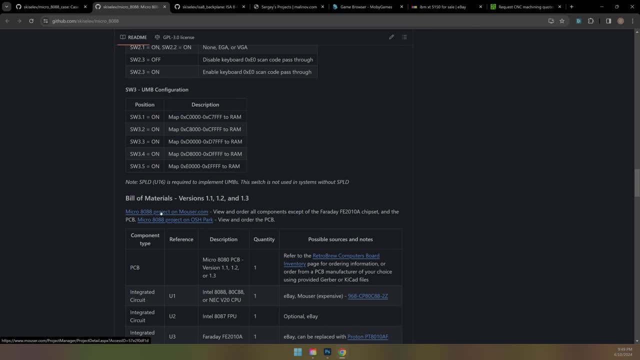 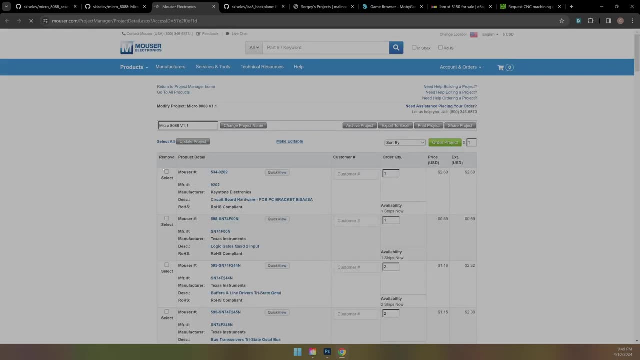 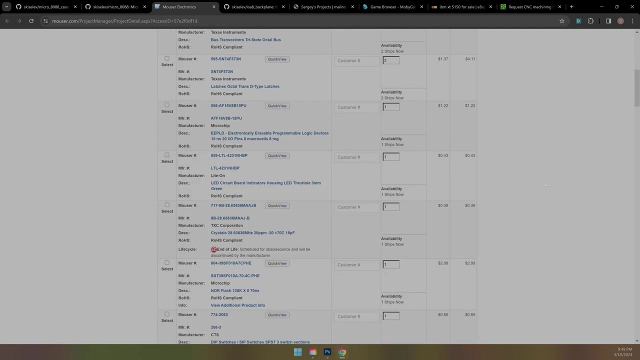 to be able to say that right, Micro 80, 88 project on Mouser. So if we click that it actually will try to pull up a cart and the cart has you know. so this is like a saved cart that Sergey or somebody else had put together. But the problem is you know some. 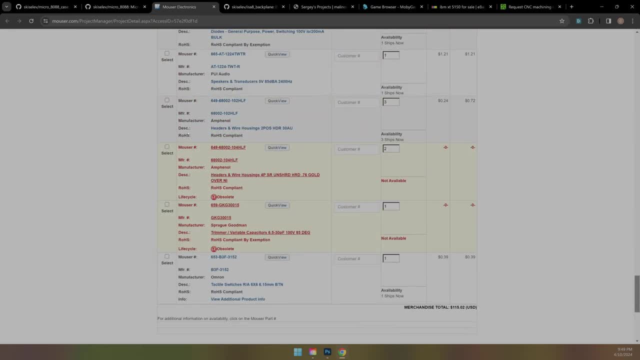 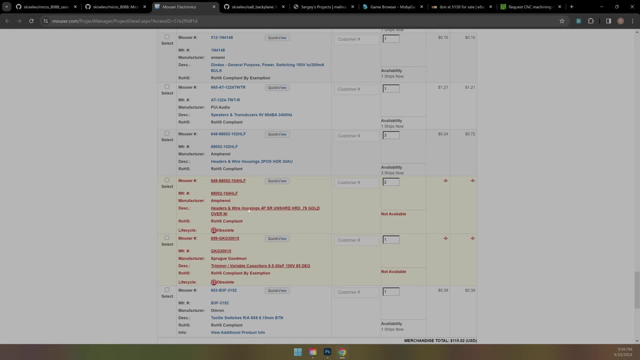 things on here might be backordered, or these parts here There are actually end of life or obsolete, at least from this manufacturer. I think this one is just pin headers, which is fine. You can just use any other pin headers. as far as I know, It does say that you're hard gold, but I don't really think you need hard gold. 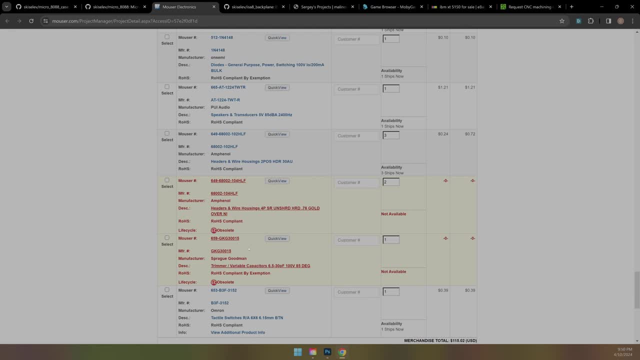 pin headers. but you know, and this, this trimmer pot or trimmer cap, which I just found it by Googling this or putting this into DigiKey. So, essentially, if you're going to be building this project and and you know you're building this and you're building the back plane, you're 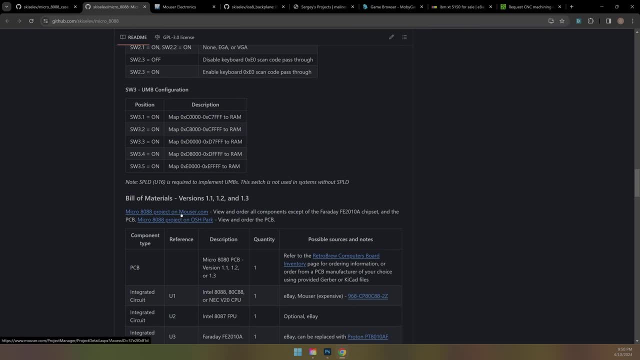 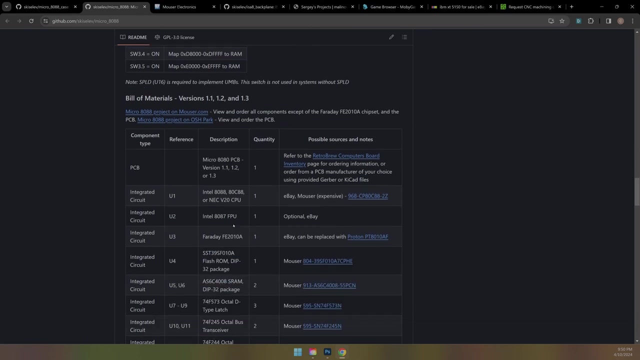 going to need a lot of things. So I do recommend opening these Mouser project lists, but then you're going to have to kind of search around either. I was able to get everything from well. I had to buy the Faraday chip on eBay and then they gave me a. I didn't buy the 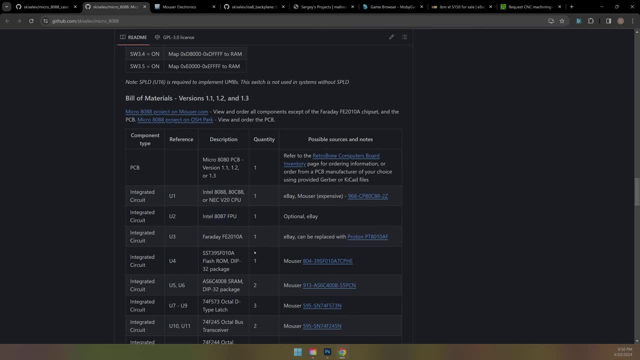 FPU. so that's something that maybe I could do in the future. but I had to buy the Faraday chip on eBay. So here's the list for that And I bought. well, actually, they gave me an ADC, ADC 88 CPU in that Faraday order. I didn't. I don't think I ordered one, So that was eBay. 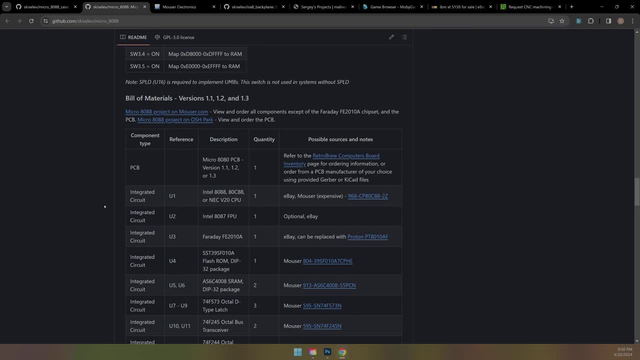 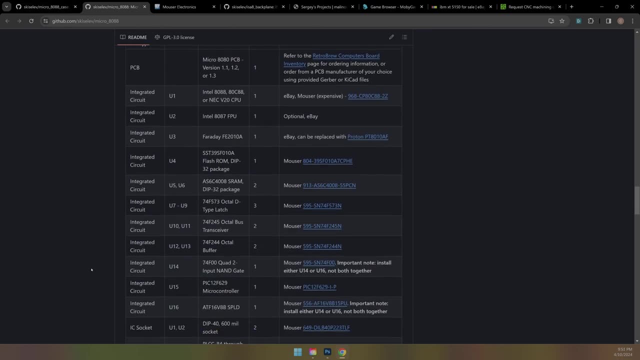 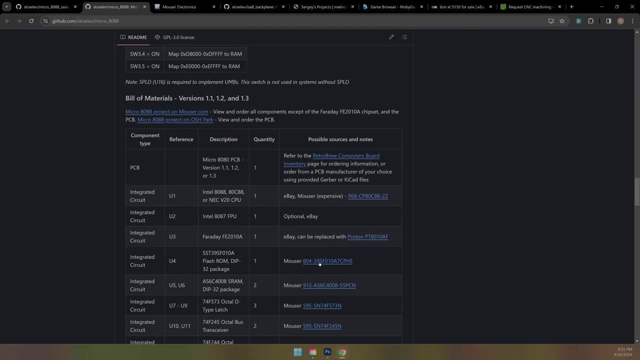 and then everything else I was able to get from either Mouser or DigiKey. So it's possible to get everything new. But it's just a little bit of a manual labor which kind of stinks, because all the part numbers here are listed in with Mouser's, whatever their inventory. 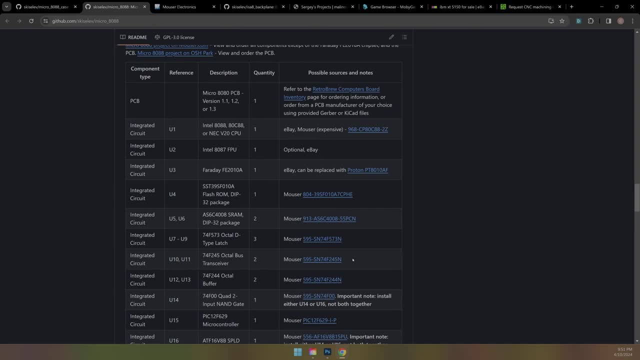 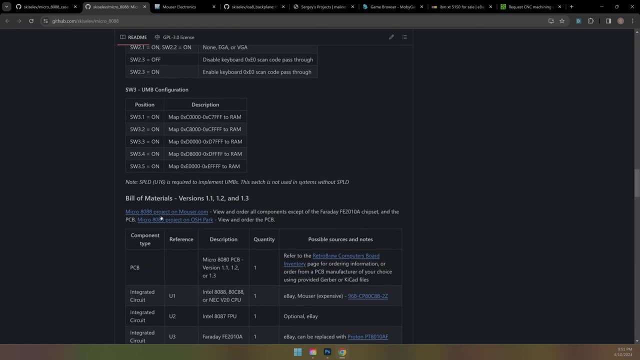 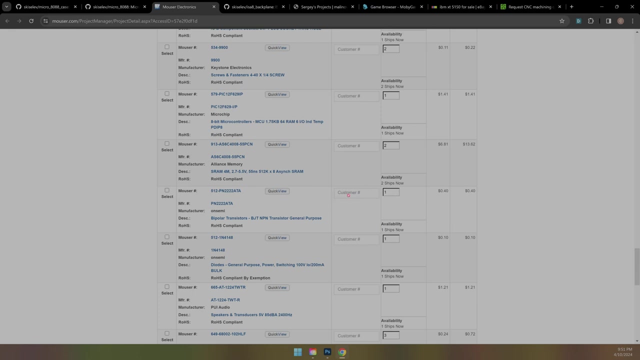 tag thing. So yeah, Yeah. So it's a little bit of a pain. I also, also, when you open the Mouser thing, it doesn't load. it doesn't load customer customer reference designators into this at all, So you'll have. 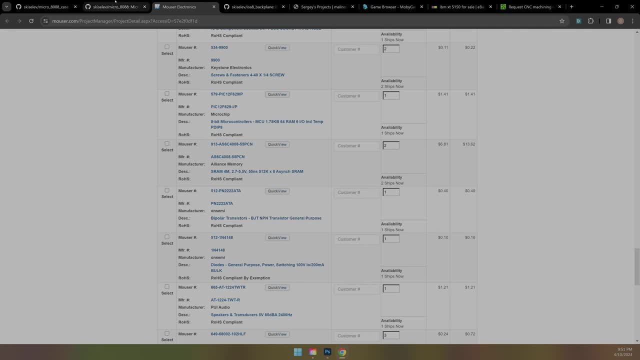 to add those also. So you know, I I sort of wish that it was a nicer. I don't know, I don't know what the better way is. I know now you can do like Octopart, whatever, and 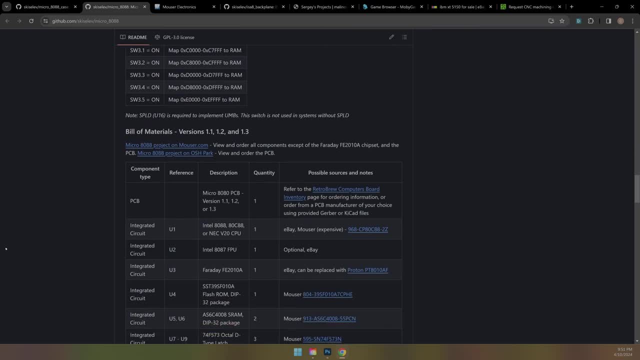 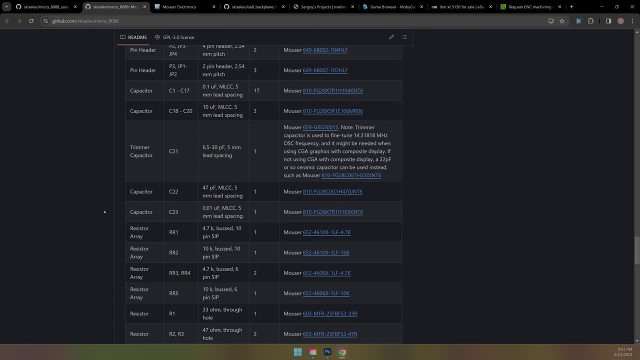 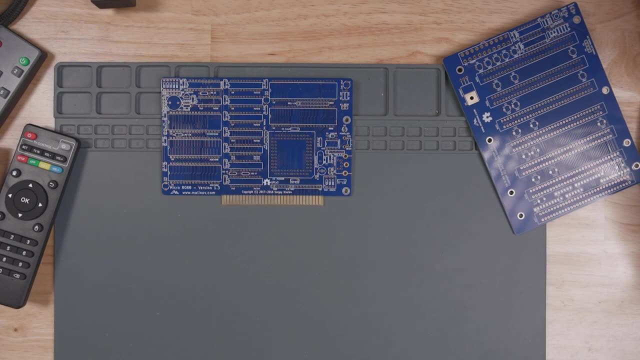 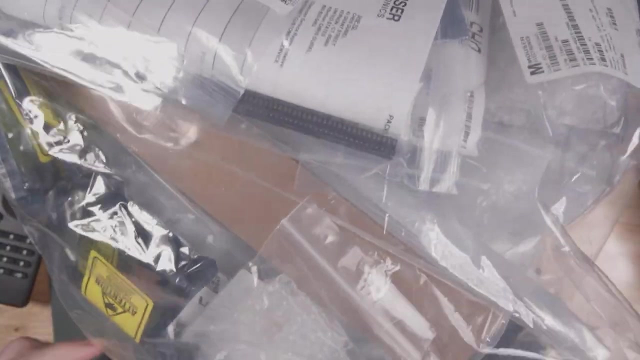 Yeah, I'm glad that there is a list and I'm glad that it's nicely listed here, but it's a little bit of manual labor to get all the parts and stuff together, But at the end of that we ended up getting a giant sack. This is actually the biggest batch of stuff I've ever gotten. 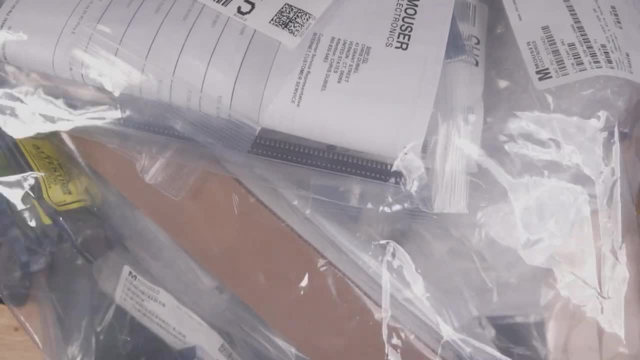 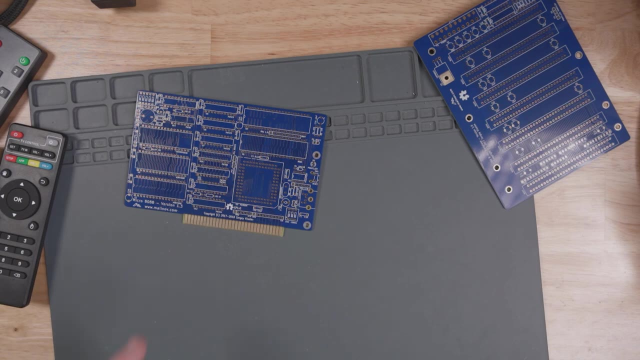 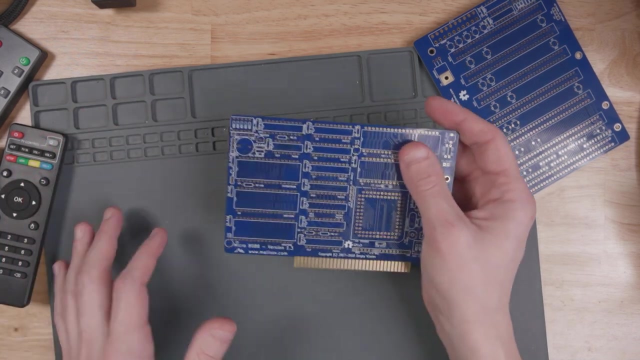 It's kind of like too big to see. It's falling apart. And I have another little thing from from Digikey. So all my parts for both this, this for the micro 8088 main board and the back plane, all in this bag. so let's get started. and one of the cool things about this whole project is most. 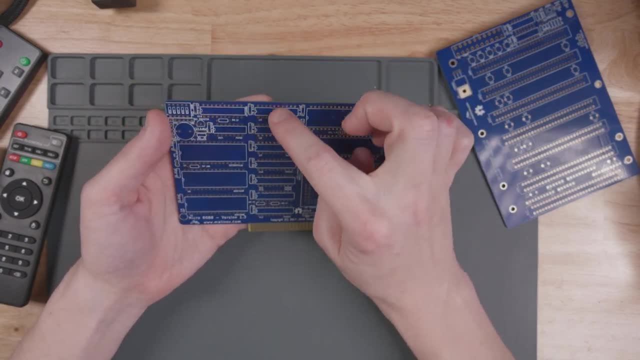 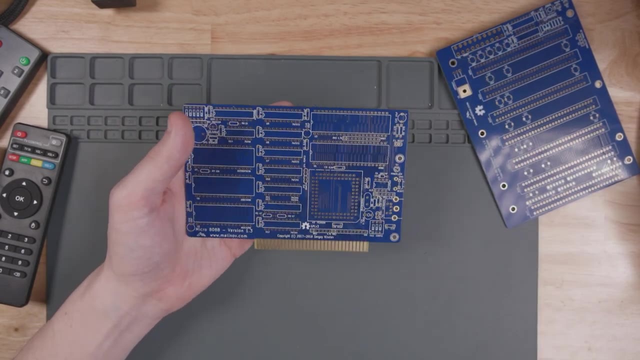 of these chips- most of the big chips I suppose, and even the memory ones here they all use. I think they all have sockets which are included in the bomb so that the sockets do make the the project pricey. you can kind of not really tell in this picture. oh, I'm not showing the picture you can. 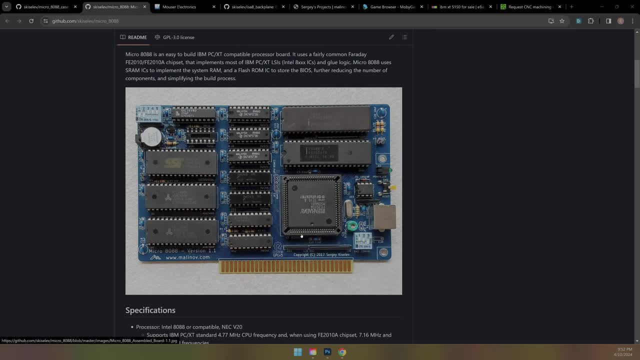 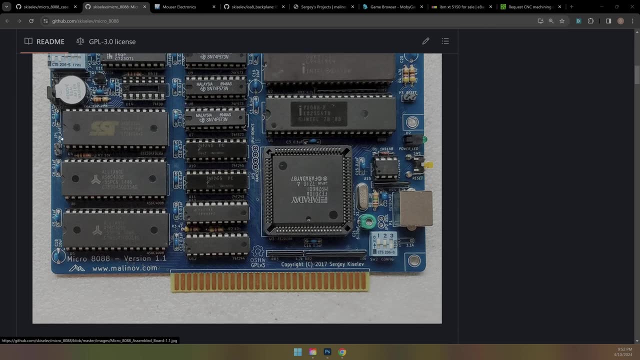 kind of not really tell in the picture, but I think they're all in sockets. well, at least this chip here is obviously in a socket, but like the memory is in a socket, these chips down here and sockets the CPU and the this is in a socket, so it's kind of a cool if you ever need to replace anything. 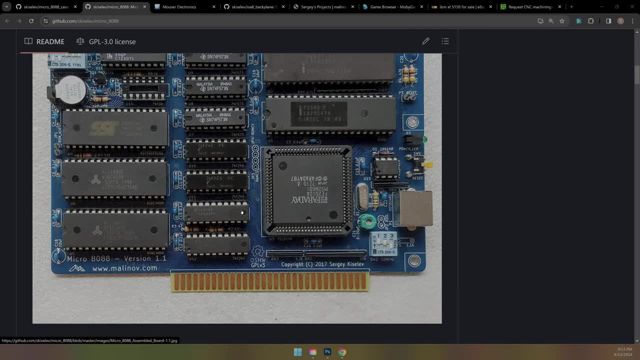 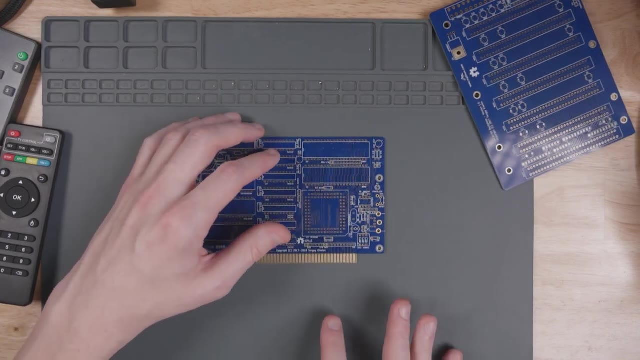 it's kind of all ready to go for you. back in college I had to build an 8088 and a breadboard. huh, well, I know like Ben Ben eater. isn't Ben eater doing that, making a I um breadboard? is it an 80, 80, 88? I don't remember if that's what he was doing, but that's a fascinating. 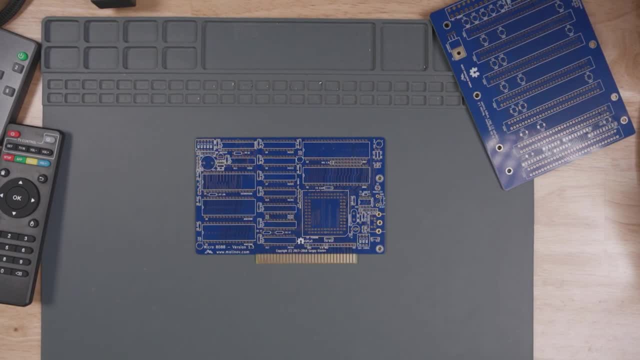 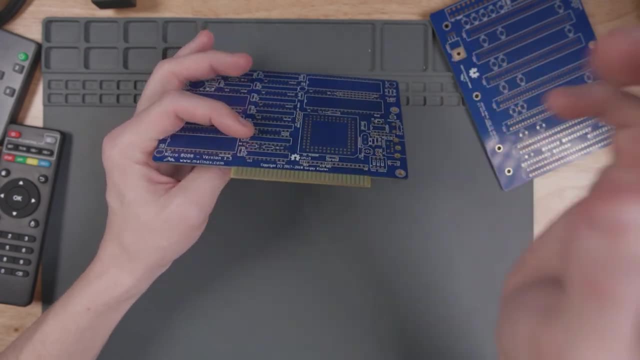 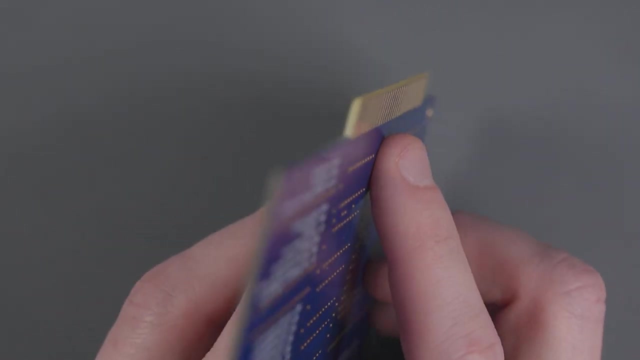 um series by Ben eater. hmm, also another thing I guess I should mention is: uh, I forgot to have them bevel PCB way. bevel the edge, um, at this cart edge. there's an option in the settings where you can say: like the cart edge, 45 degree bevel, which is what an ISA, uh, the ISA standard, needs. but I 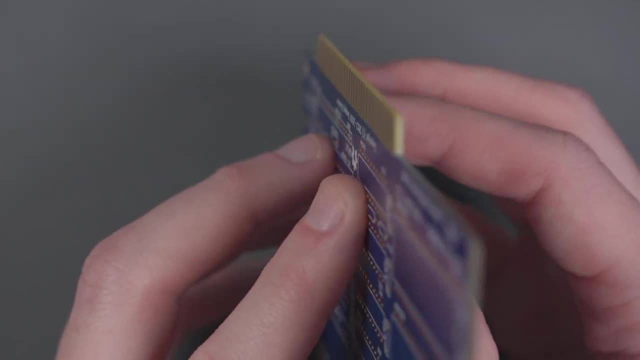 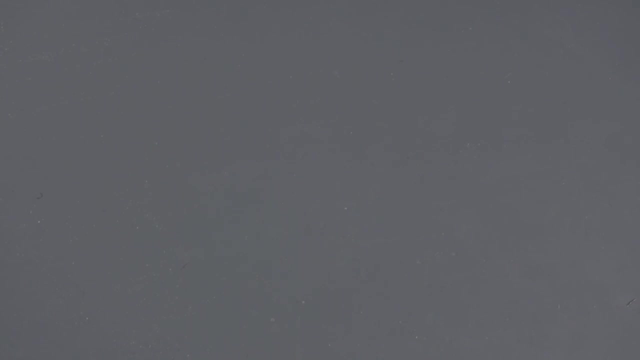 probably way too big for what I needed it, but I ended up buying this metal file right. so I had this metal file. it's huge. it's like at least a foot um, which is way overkill, I think, for this, and actually it kind of hurt, um, I think a little bit, because I kind of over. 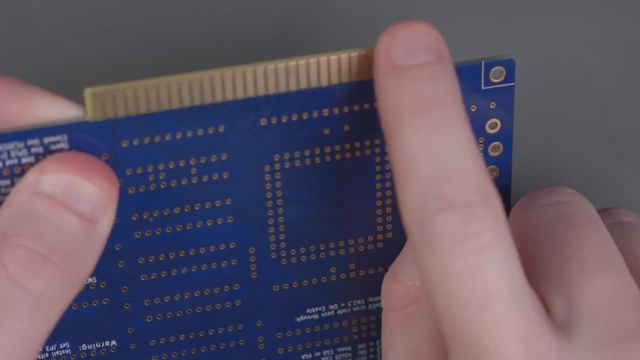 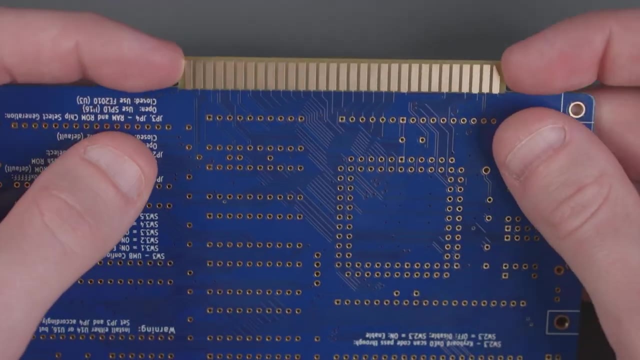 I over uh file down the edges on the edge I think it'll be fine. I'm just gonna send it and doesn't work, i'm gonna have to transfer everything to a new pcb. but you know it's fine. uh, oh, it's a 6502, got it. that's what the ben ben eater one, but i mean, either way, that's fascinating, he's going. 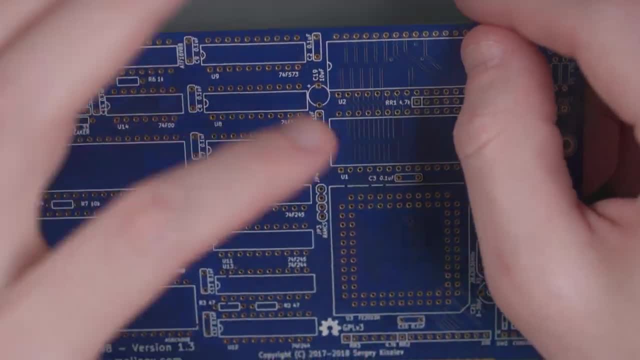 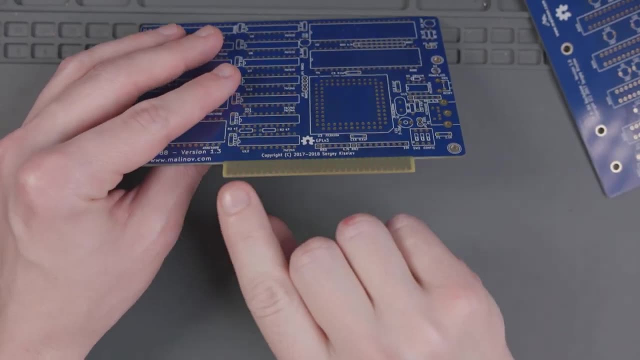 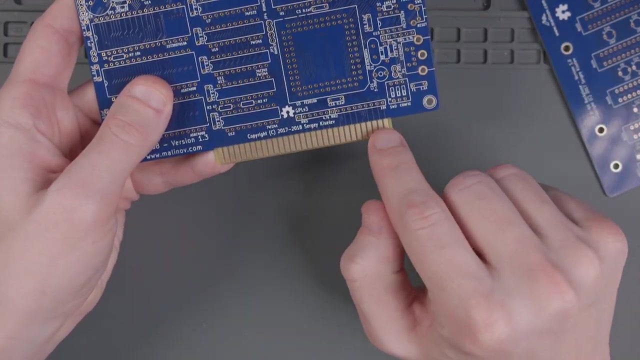 through all the steps of making it all work. um, so i did use a, a file, metal file- but i also used high grit sandpaper because it's, even with the metal file, which made a nice, well debatably straight edge. uh, it's going to leave um burrs on the metal, so like if this is, if you're, you know. 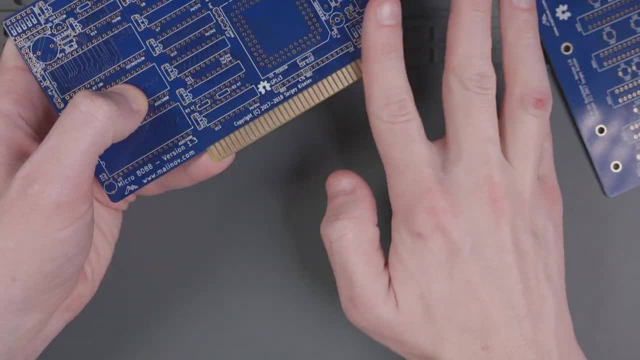 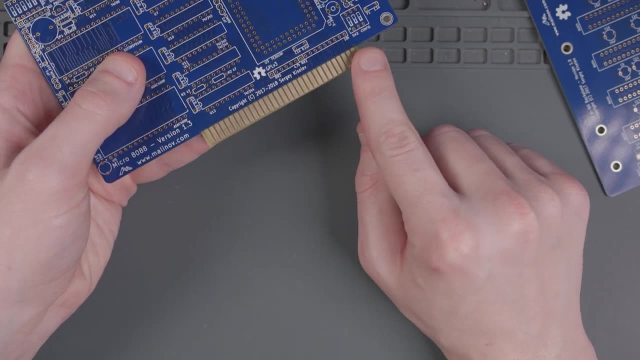 i'm using enig here, so this is kind of like harder- slightly harder- gold than the um hassle or whatever the normal uh finishes it will leave berms here on the edge or burrs, so you'll have to take some fine sandpaper like a thousand grit or whatever. i did i think it was like 1200 grit. 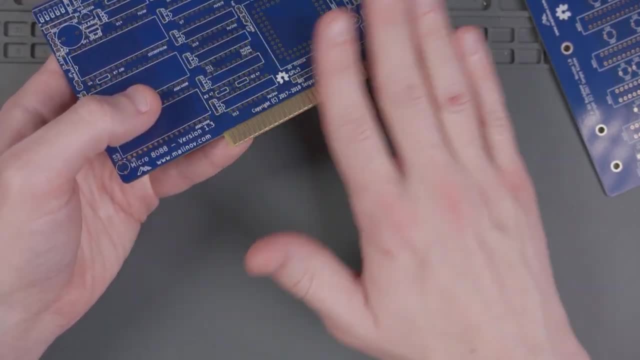 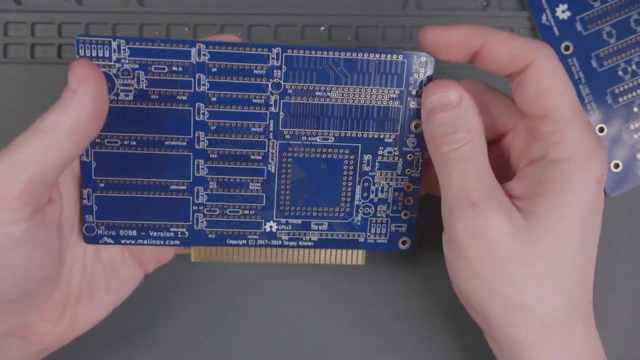 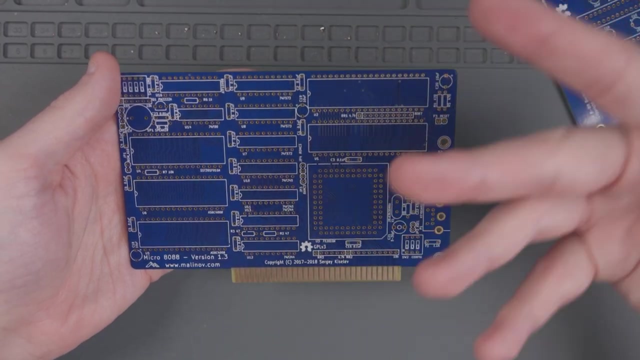 or something so like: hit it with some high grit afterward to get the burrs down, otherwise i don't know what it's going to do and you get in the socket. so i think these are pretty clean, uh. but because everything is in a socket, i kind of have to be strategic and how to assemble the whole thing. normally what i like to. 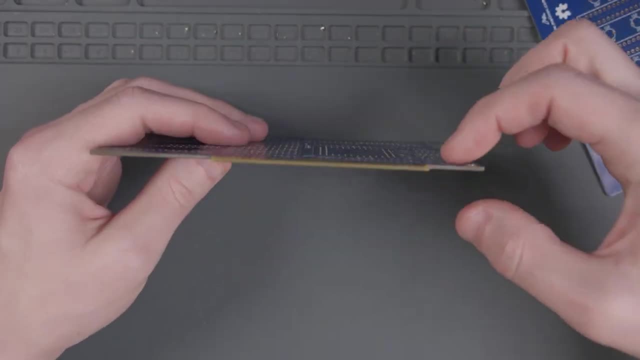 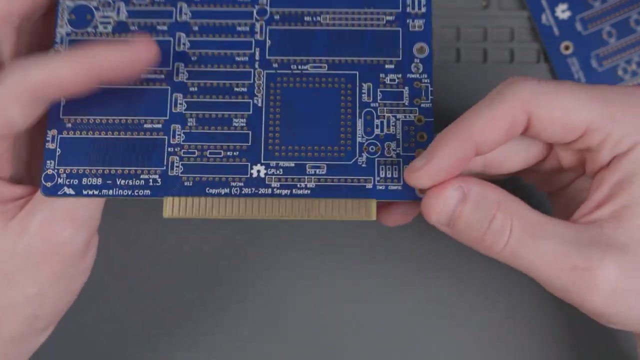 do is go from the flattest component and go higher. so like like resistors and capacitors and things like through hole ones are pretty small, so that's probably what i'll start with. um, probably not a fun stream, but um, yeah, you know. then you work your way up to the uh. 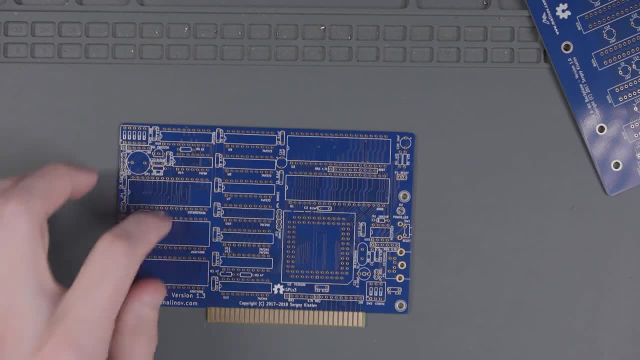 um, the taller things and, and you know, we get pretty quickly to the sockets. so there's a guy that's making an entire pc and vga and audio and all sorts of stuff. yeah, i think that's that's ben eater. yep, he's following a book. to be fair, it's not him, you know he's not. uh, 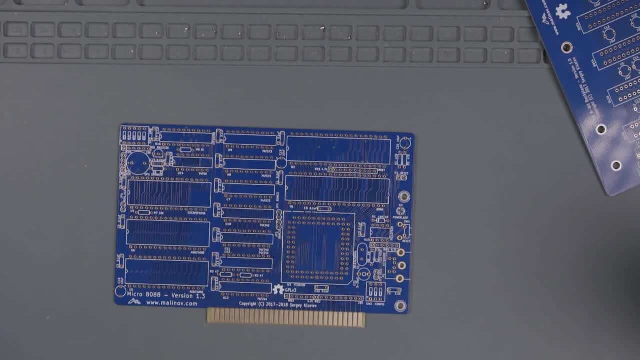 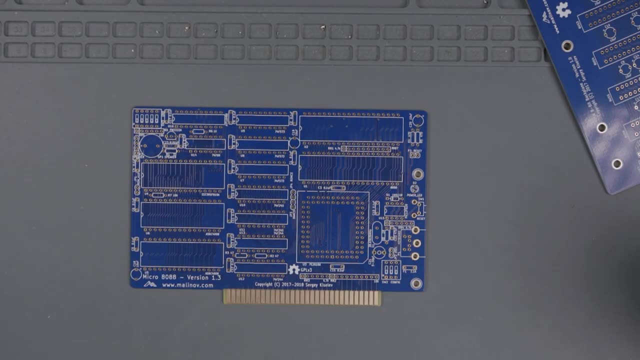 grant. you know he is making the, the kits that people can buy, but he's following a and and he's writing all the programming. so he's doing all that stuff. but he's all right, let's let's shut up and talk. all right, let's shut up and talk. all right, let's shut up and talk. all right, let's shut up and talk. 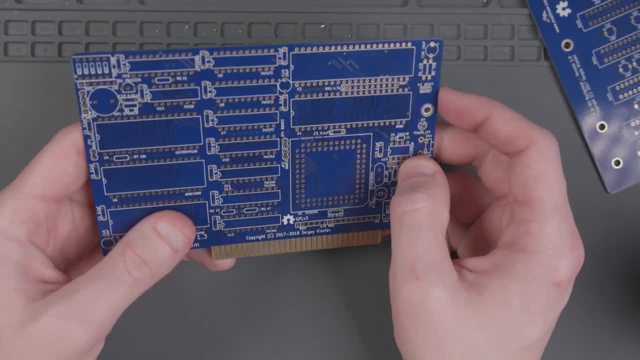 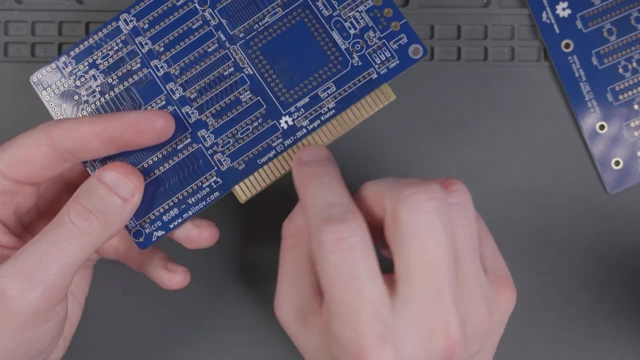 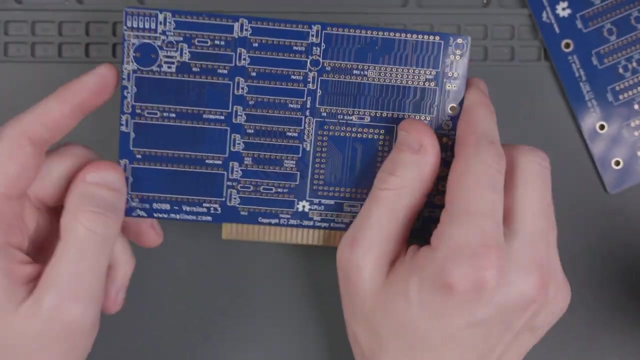 shut up and work. um, i don't know where do we start. you kind of ignore the bevel, unless you're going to be. yeah, that's true, i just, you know, i just wanted to test it really. um, even, you know, even the flat bottom would have been probably, would have been fine. but you know, if i'm going to build this, i 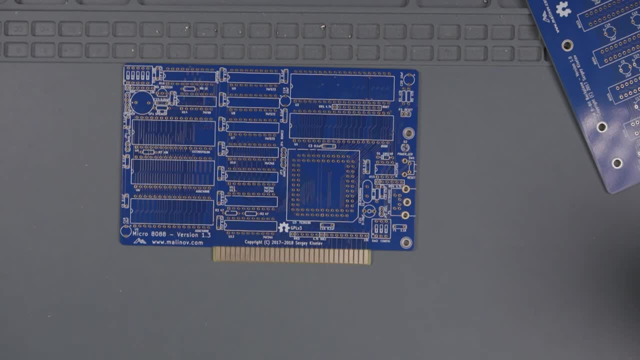 might as well take the the 30 seconds it took to to bevel that. but you know, or now i have, uh, you know, all the tools and stuff for the future, you know. so, all right, i don't know where do i start. i guess let's try to pull out the. 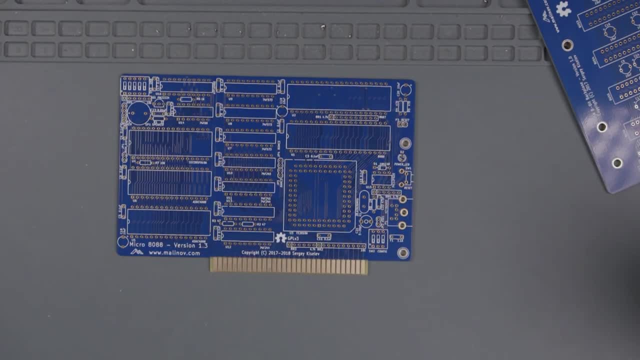 the capacitors. i know this isn't a fun capacitor installing stream, but um, we gotta start somewhere. rr2 oh resistor arrays. okay, now this is the worst part is when you're just starting, because all of the parts are like all mixed up and you haven't organized anything yet. 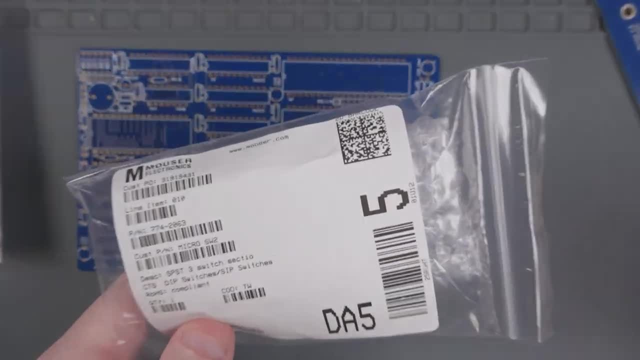 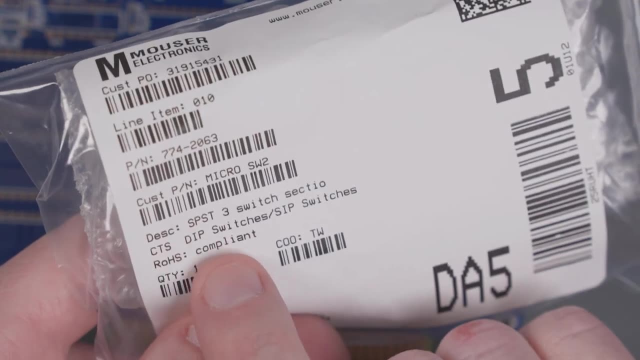 so i made sure to put, because all the parts for both the micro88 88 i just keep adding, i keep adding 80, 88s to the end of it, so this keeps getting longer and longer. i made sure not just to put the reference designator of the project but also what project. 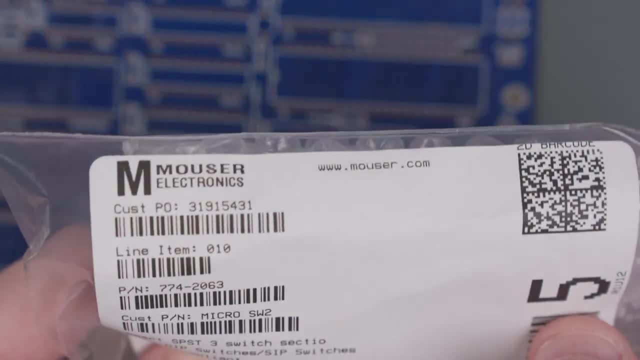 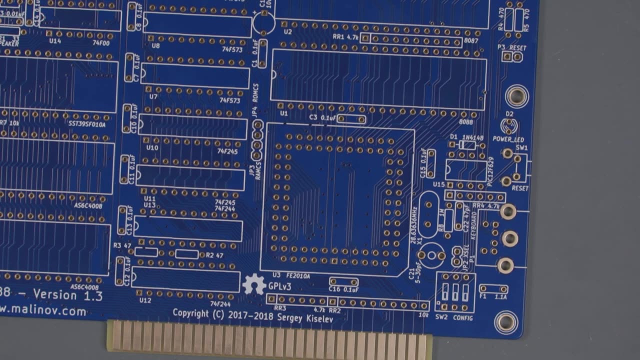 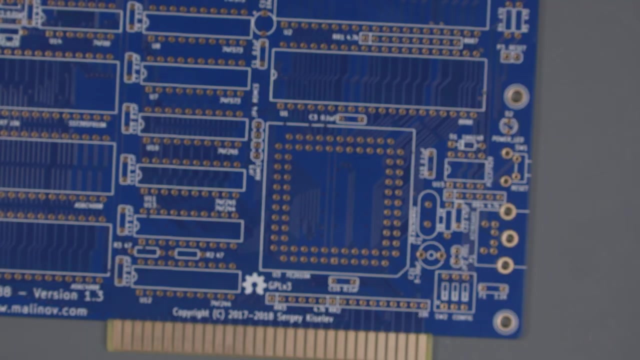 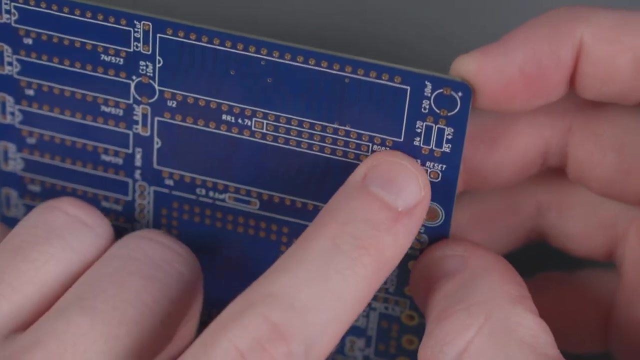 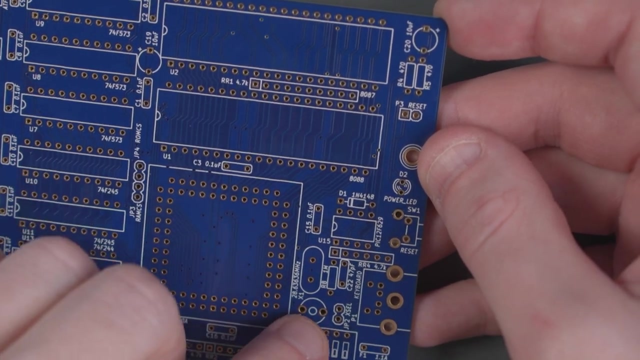 it was in. so this is for. this is switch. two for the micro um 8088 build versus the. uh, oh, this might be resistors. okay, so this is r2. well, we got a bag out, so let's see, this is what r2 and r3, which is i see r4 and r5. uh, i'm not gonna bust out the um, the microscope. 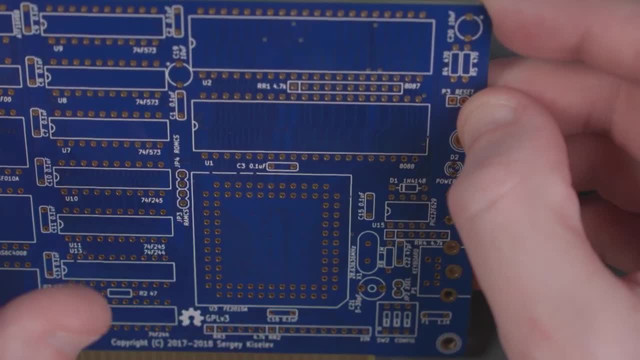 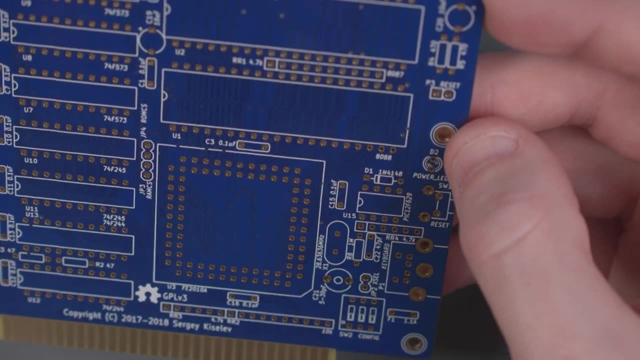 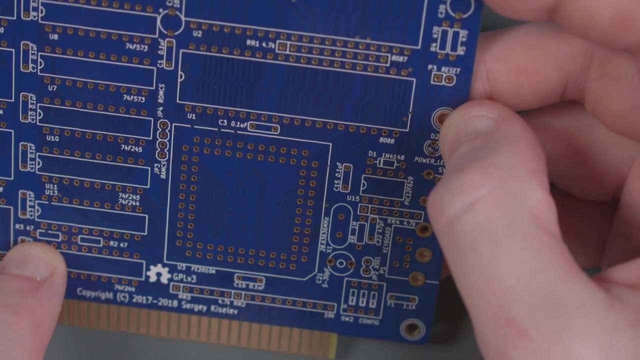 but yeah, um. well, i see the resistor arrays r1. this is also. this is always like the- oh, this is the sz2, ok, and the r3, um, so this is the r2 and r3. i'm gonna say this was r2 and r3. 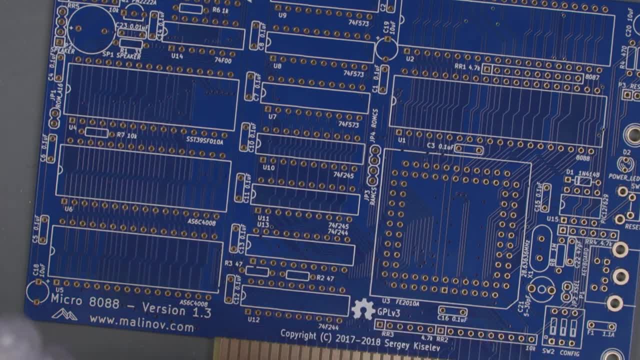 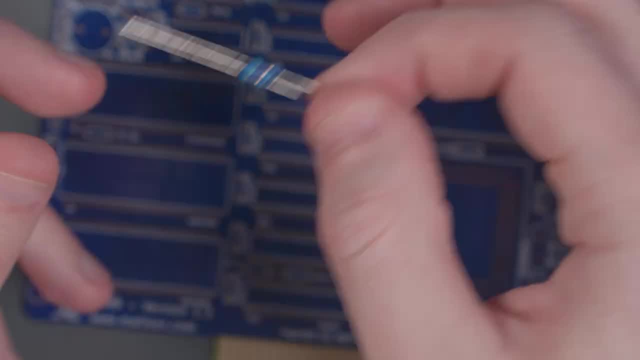 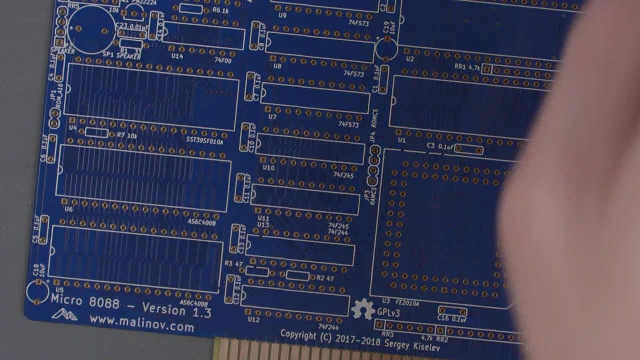 okay. so r2 and r3: okay, 47 ohms jobbies got it. i do kind of think that it's wasteful, you know, to to buy prod. you know i don't love buying components like this, you know, i would rather have a giant stockpile. 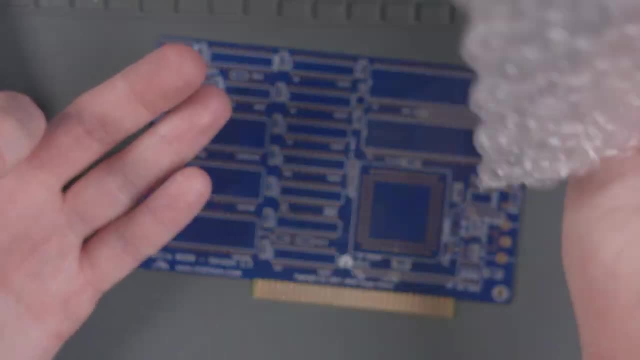 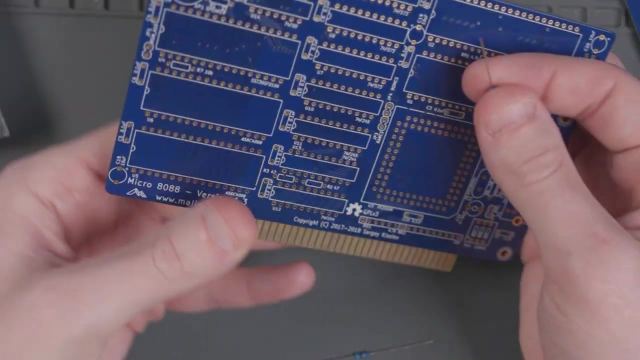 trying to say is: i don't love having all this trash left over. i mean, i try to reuse it as much as possible. if you were, if you've ever gotten something from me in the mail, you know that i try to reuse stuff. um, resistors don't really matter which way you go, but uh, you know i wish. 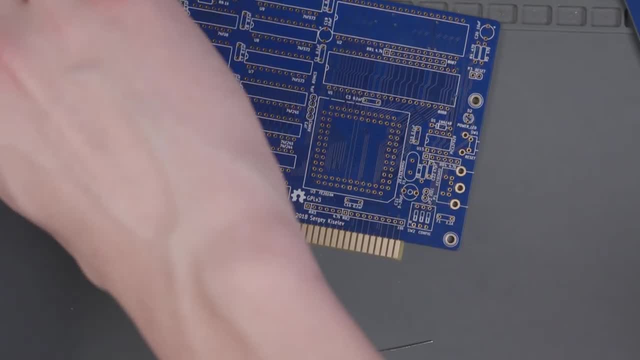 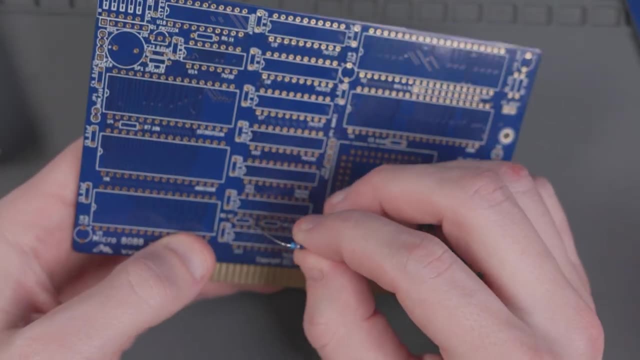 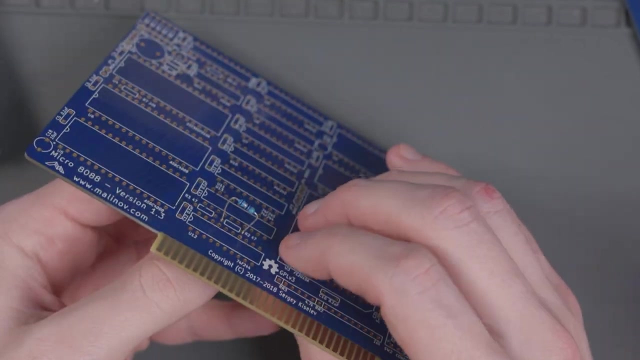 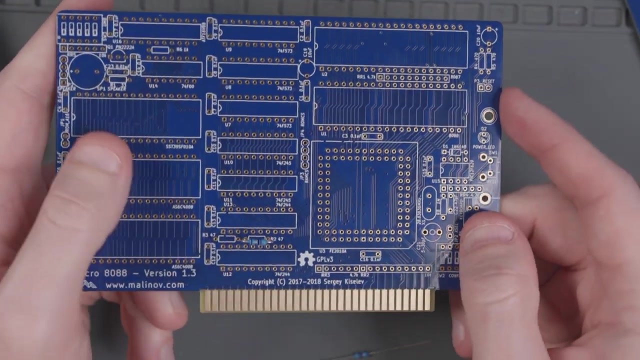 i had a fancy resistor bender thing. i just try to bend them whatever close enough and then send them on. send them on home. oh boy, they're like tiny. they like really want you to jam these resistors in there. oh boy, who, who's who's doing this and it's super tight. let me see what does the picture? 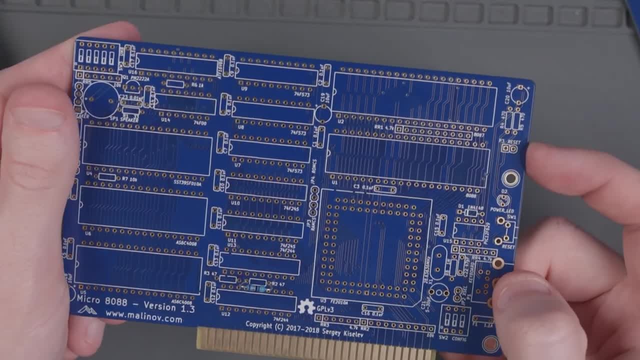 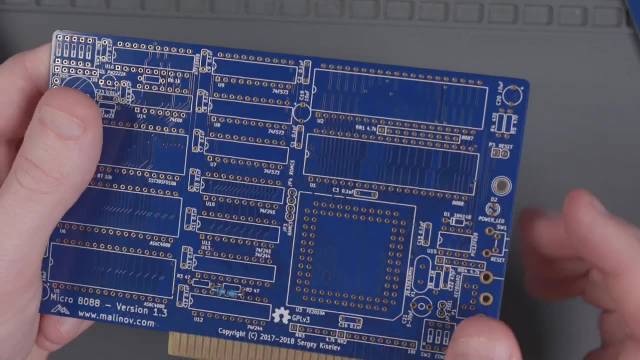 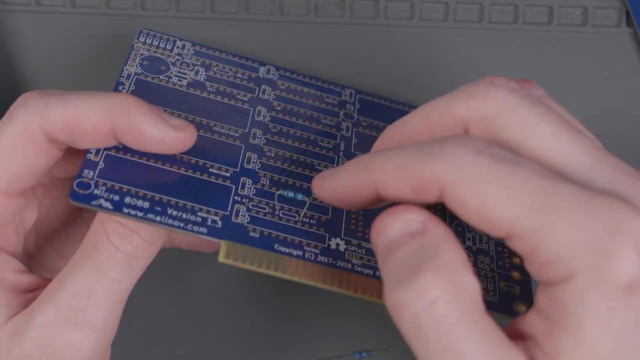 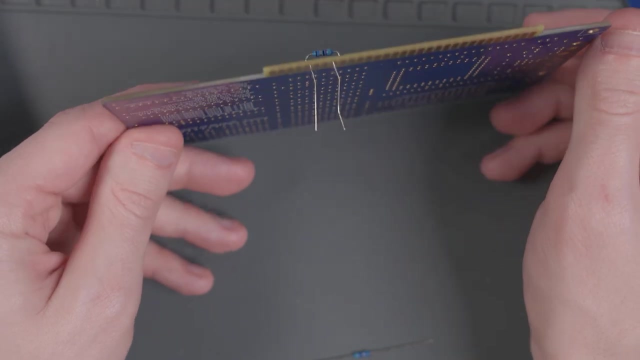 look like: um well, wow, okay, they're like really slapping it in there. i don't know, man, that seems kind of sus. um, i don't really want to bend it. i can 3d printer bender, i should, i should, uh, do that, but i don't know what you do in. 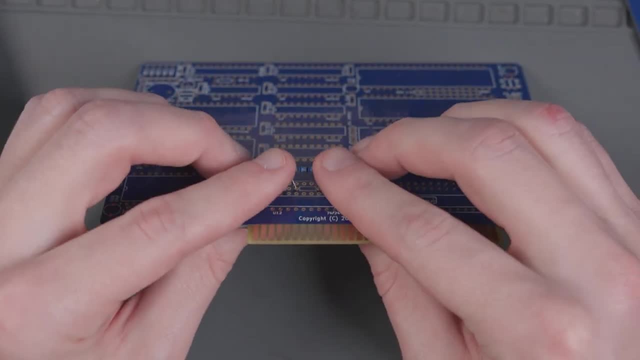 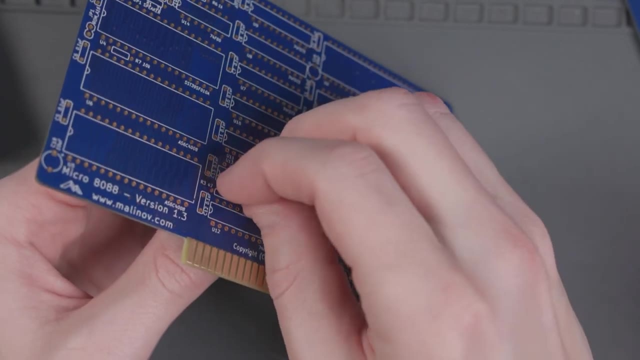 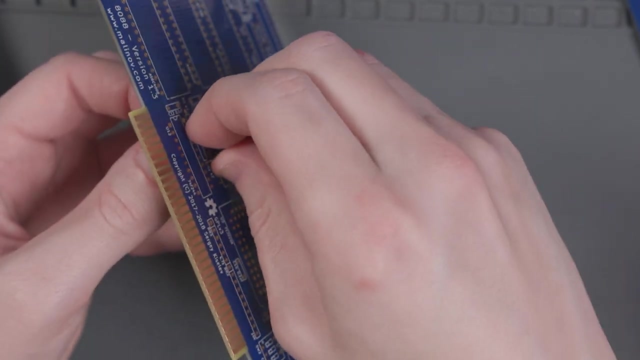 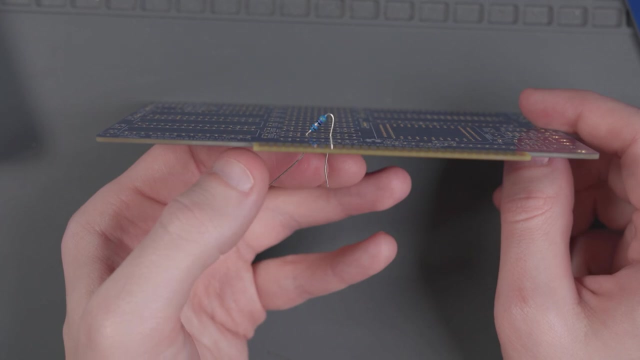 this circumstance, like you really can't bend these any smaller than they are. uh well, you know what i should do. i should probably. maybe i'll wait because i know you can do. i know you can do this. this is probably what i'll end up doing. um, i know you can do like that and that that looks pretty clean, so i'll probably end up doing. 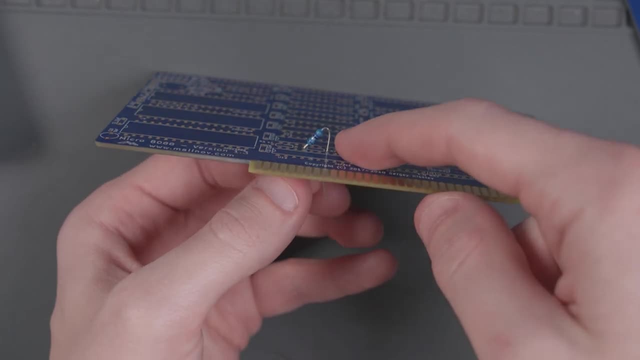 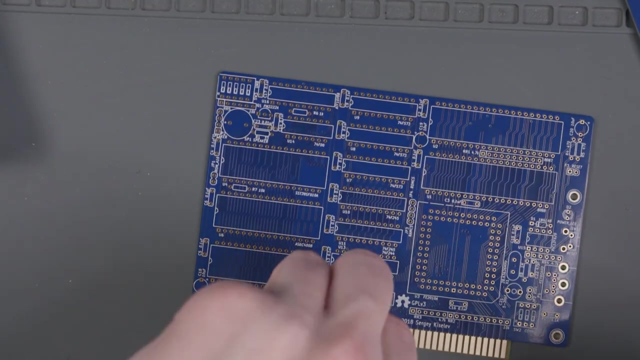 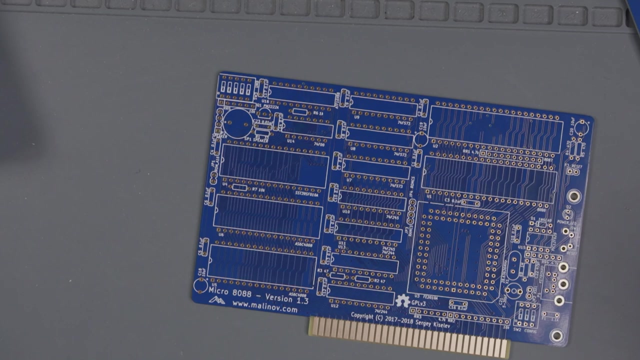 that, but i'm not going to do it yet because obviously that's that breaks our rule. okay, all right. well, that was. i have a feeling that all of these, these surface, all these resistors and capacitors are going to be the same issue. is there something that i'm missing? 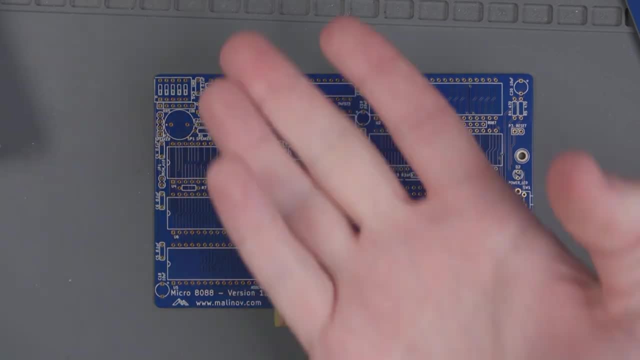 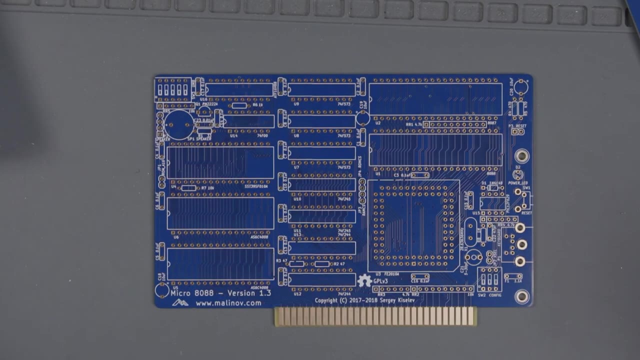 i've never encountered that, or it's super. maybe i bought the wrong type of um. that's. the only other thing i can think of is maybe i bought the wrong. uh, i know you could probably get smaller ones than that. okay, so this is a nope, not the right thing. just reach it in the bag for some more stuff. 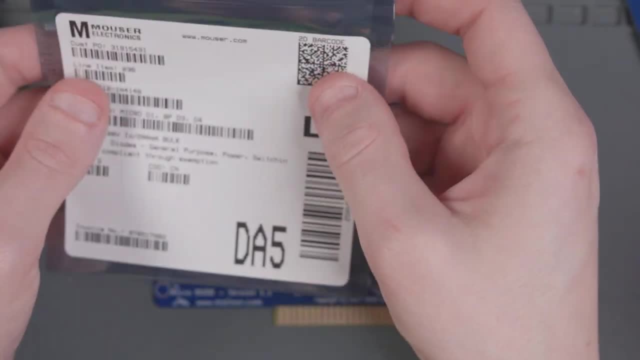 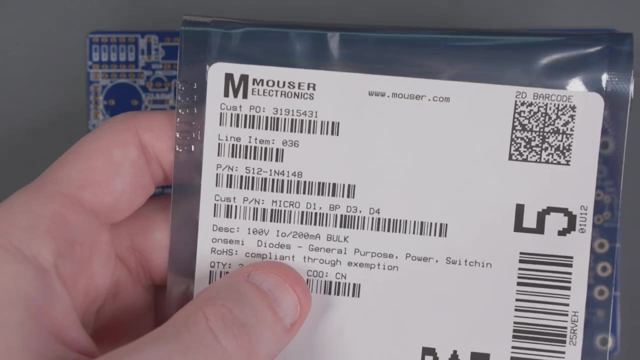 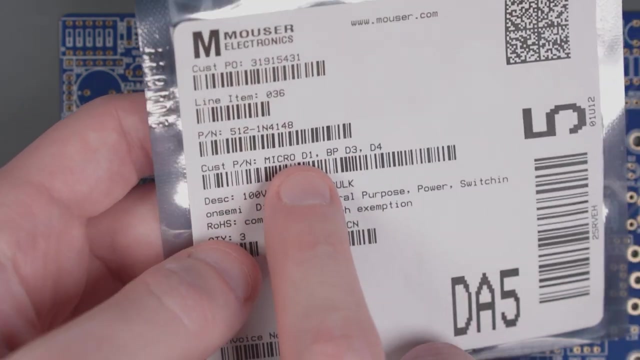 what is this? diodes? okay, these diodes are probably pretty small. okay, so this is d1. oh, so, yeah to. to differentiate between the, the micro and the micro project and the backplane, i put bp for backplane, so i can. i gotta get one d1 diode. 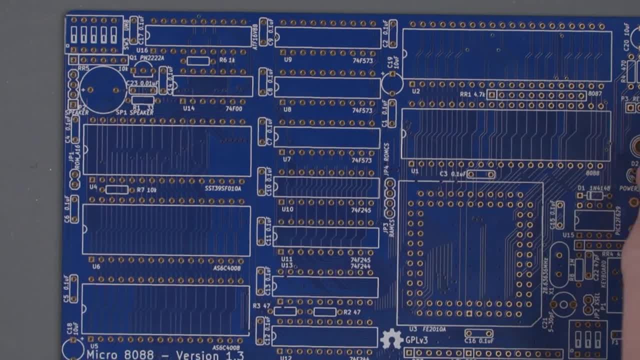 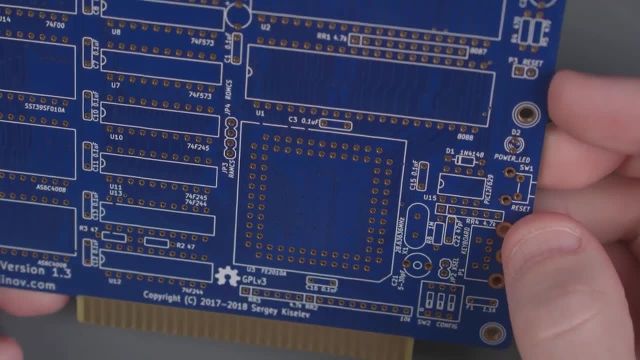 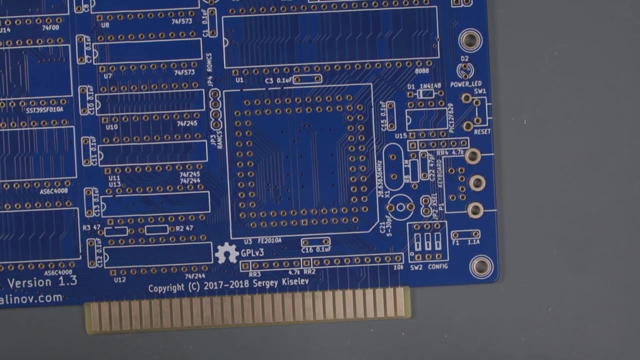 and we gotta find it. where's d1, these ones? there it is found it. yeah sweet and uh, diodes are directional, so when i get one out, oh yeah. i was kind of ranting about the bags, the amount of bags, yeah, i don't like the fact that. 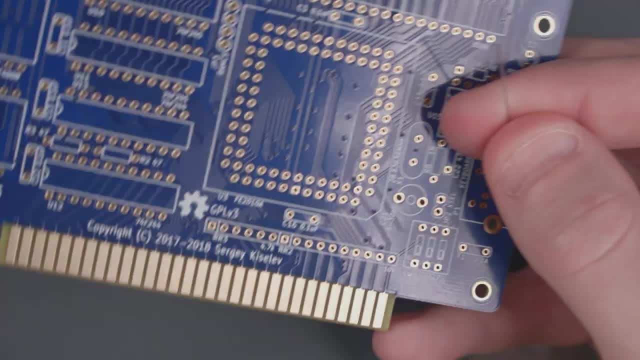 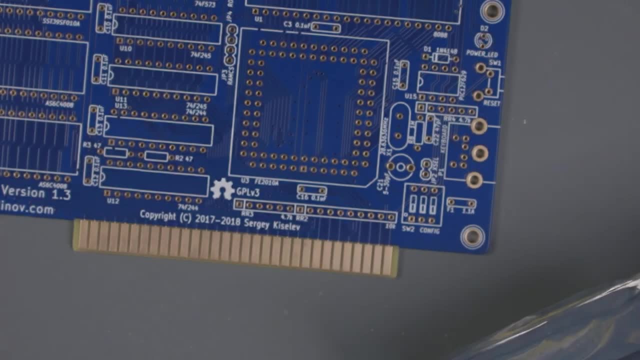 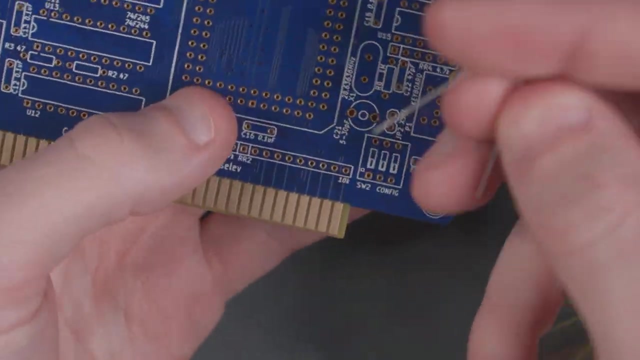 that i have to buy so many, that it comes in so many packages when you buy a project. but i don't really see, you know, unless somebody made the like sold kits. i guess that's a good way to do it, but somebody's got to do the. do that, take the time to do that, uh, okay, so diodes on one end, they. 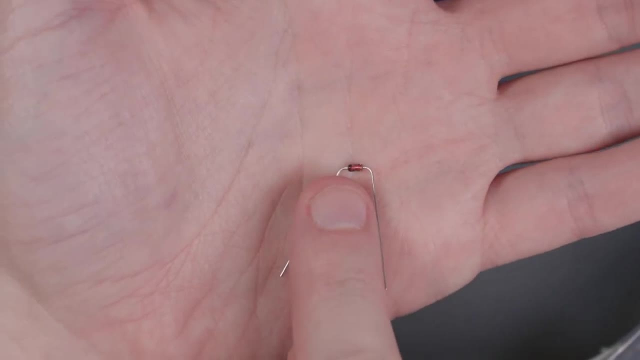 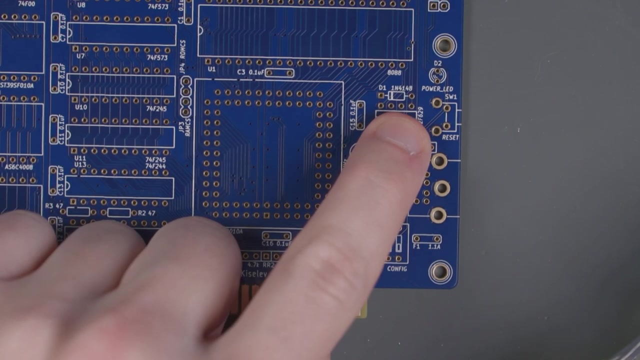 have a lot of different types of diodes. they have a lot of different types of diodes. they have a lot of a little black line. in this case it's on the left, and on the board there should be board markings. so in this case, um, there's a line on the left side there, so you just put the. 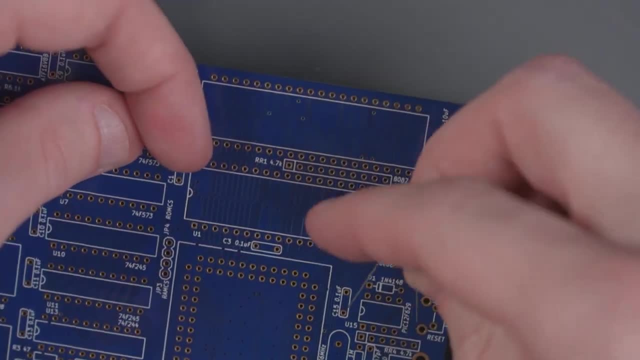 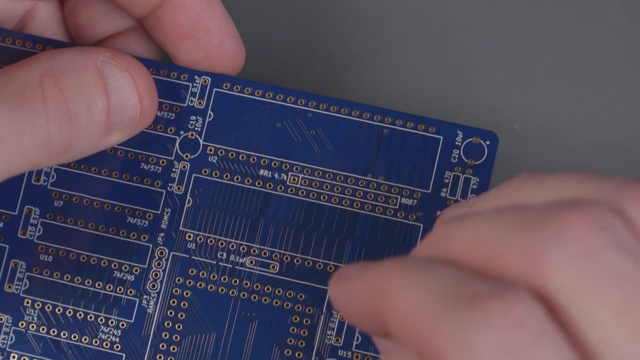 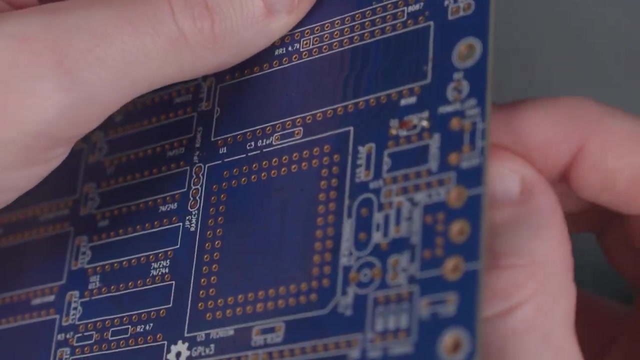 black line to the white on the diagram. wow, it's only been an hour and i'm just getting the first component soldered. that's right. see, this makes sense for it to be really flat or really narrow, like that, right, the resistor thing is kind of i don't know how to feel about that. all right, first component going in. 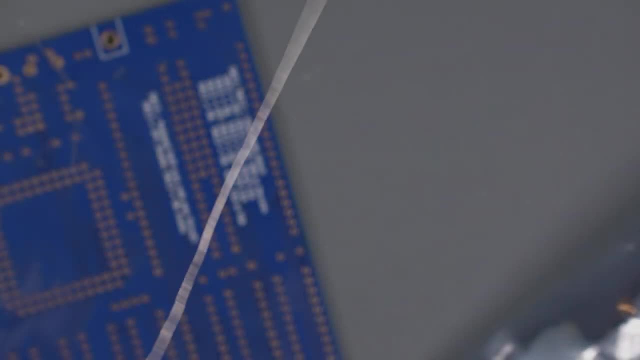 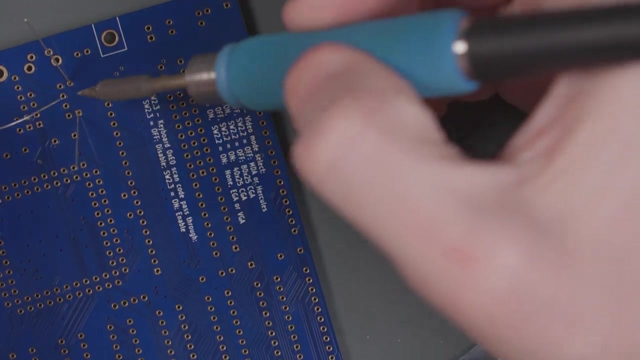 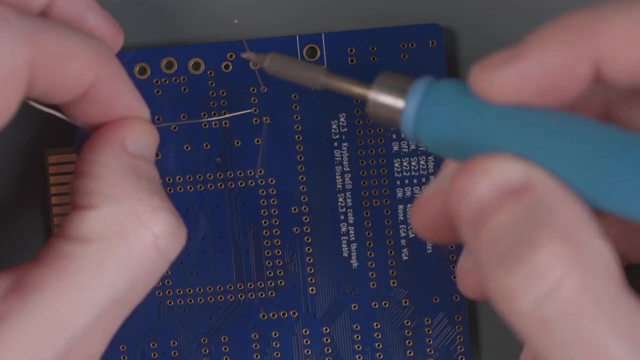 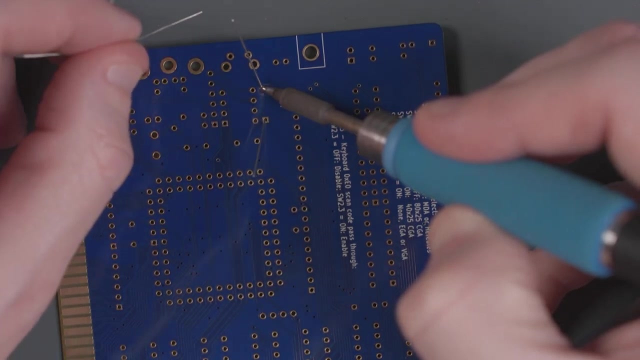 where's my solder? there it is. oh, let me turn down my temperature. don't need 380 for this. um. now i guess it is kind of interesting to know that enig has this type of coating. this, like brass coating, is little bit more heat in, like it needs more heat, I guess, to make a good joint. 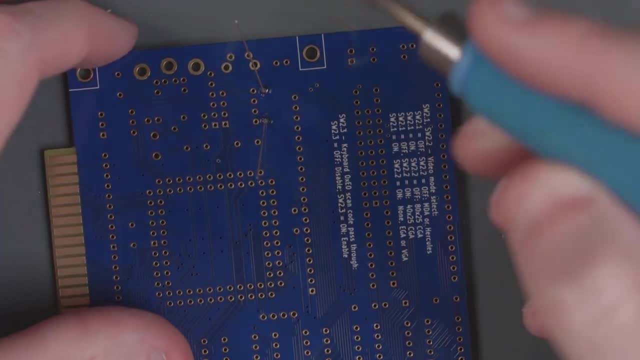 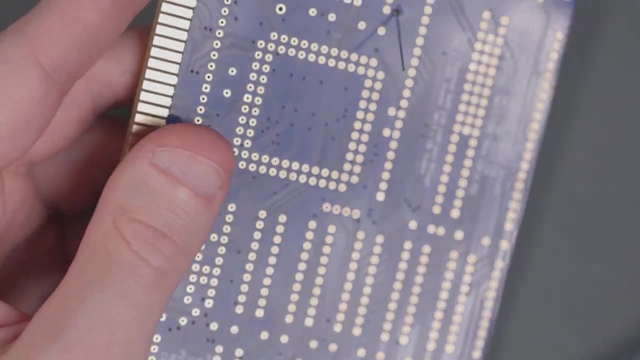 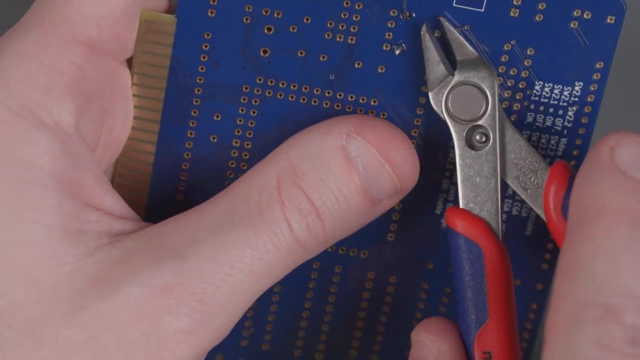 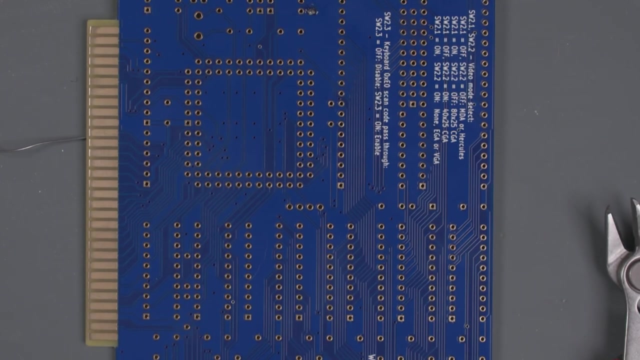 like you need to hold the part, you need to hold the weld. I find that you need to hold it longer than with hassle. so that's just a kind of a side note. but you know, just a tip that I've learned and I always keep my little parts where. 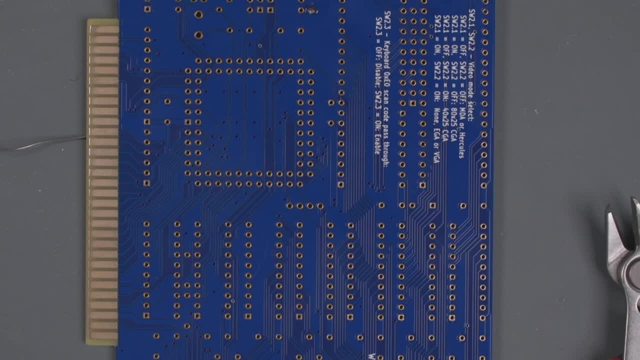 the heck. I just except for that one, that one's gone on the floor, rip. I try to keep my component clippings because those are, you know, not a million of them, but you know you have a little stockpile of them because those are good for. 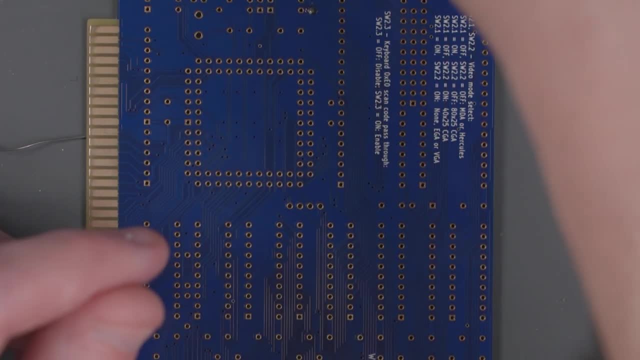 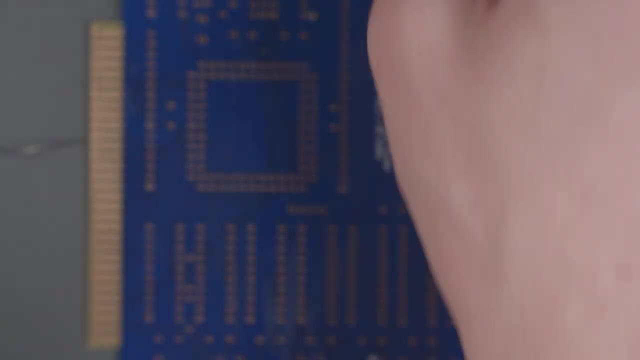 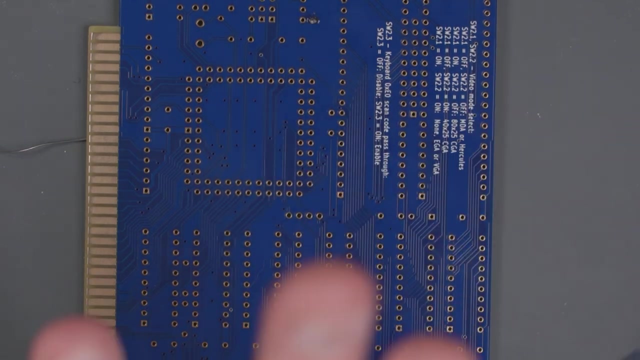 repairing. if you have, I don't know- you need to repair a wire or something that needs really stiff- oh, stiff wire or something, then these are good for that. seems like the bomb has larger resistors and it's supposed to. ah, interesting. well, that's okay, I'll do the bendy thing. I think that'll be fine. I. 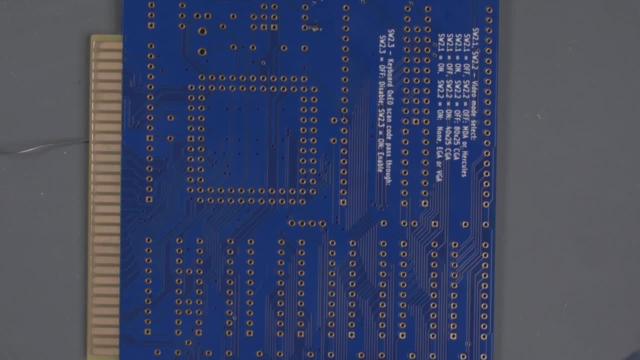 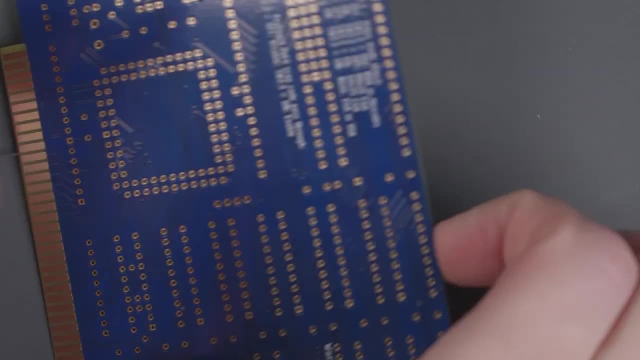 hope that'll be fine. they're kind of tucked away in those dang. then what? what resistors and capacitors is supposed to have? hmm, that's interesting. they don't look different. they look the same size as the ones that I have. I guess they just jammed them in there and they're not going to be able to do anything. 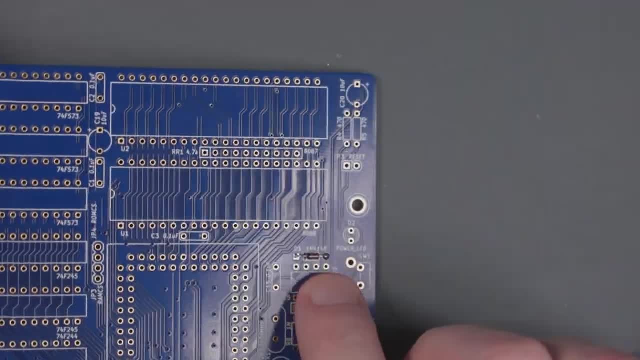 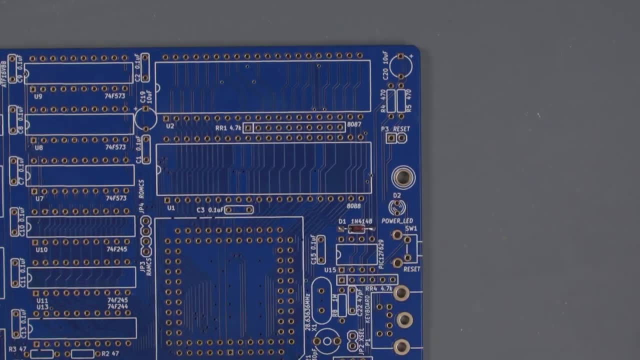 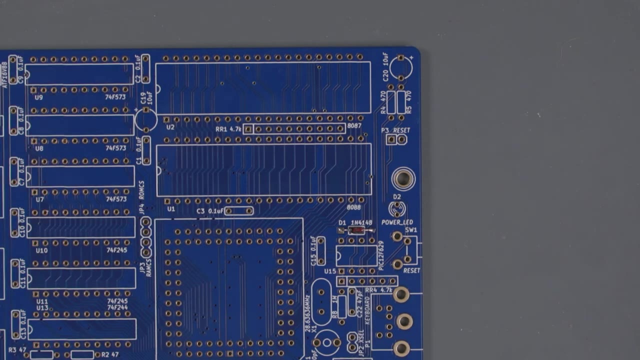 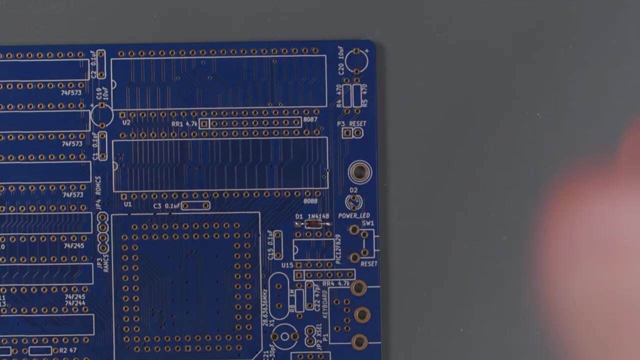 somehow. all right, that's the first component, ray. let's dig through and find some more. okay, that one's just kind of out our one, where be our one? oh, we saw that already, didn't me? so you know I got to make this kind of a little bit easier. I don't always use. 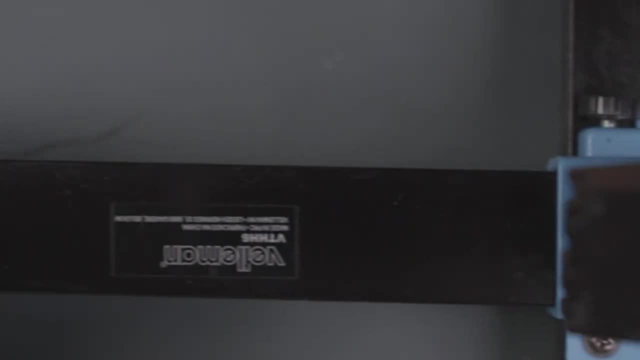 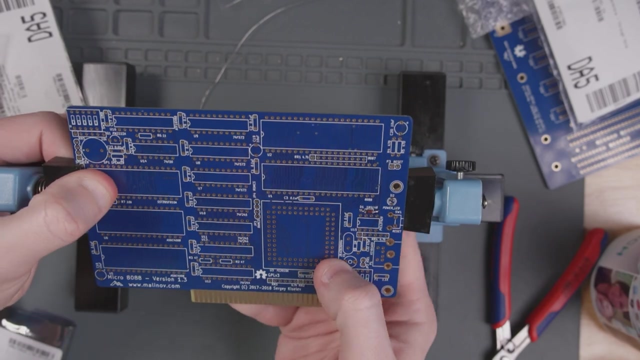 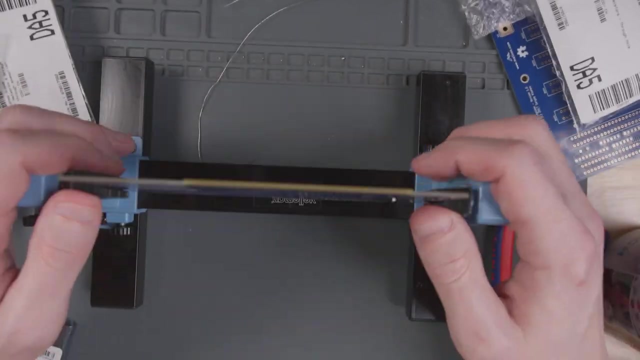 this. but i have this PCB clamp thing here. just you know, you kind of like put a board in it and it got has little spraying thingy so that you can just kind of like put it in there. now you can flip it over pretty easy. so well, I don't. 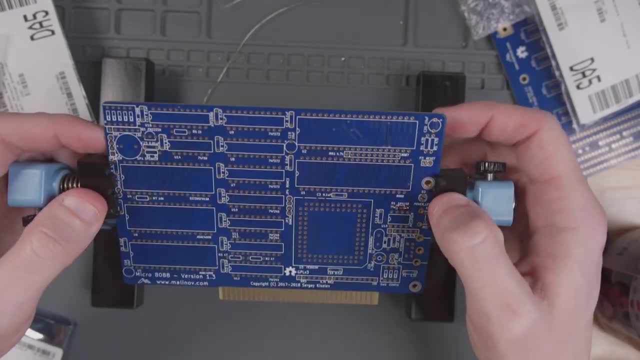 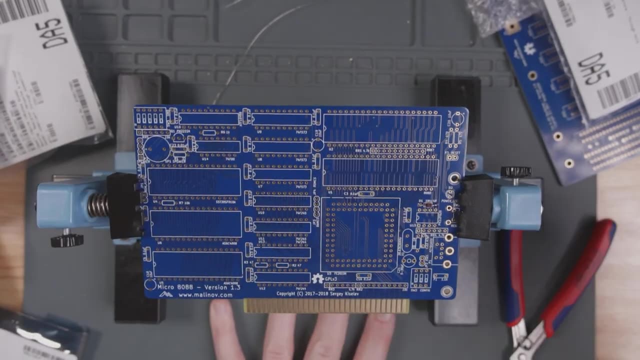 know, check that out right, see it works. I don't think I've used it that much, but it, you know it does kind of get in the way of the components on the side, but at least we can- i don't know, we'll figure it out- move my t out of the way, get out of here, okay. 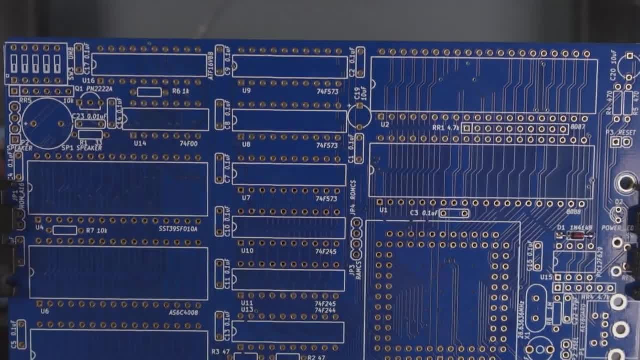 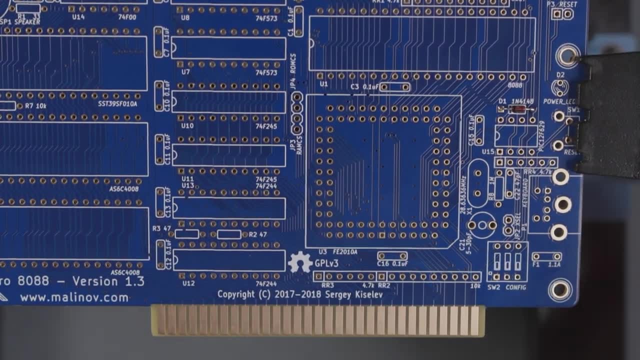 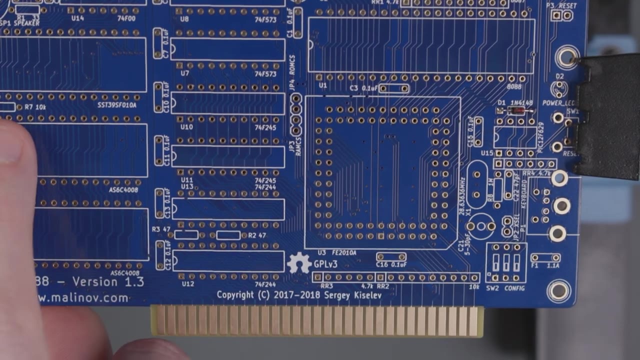 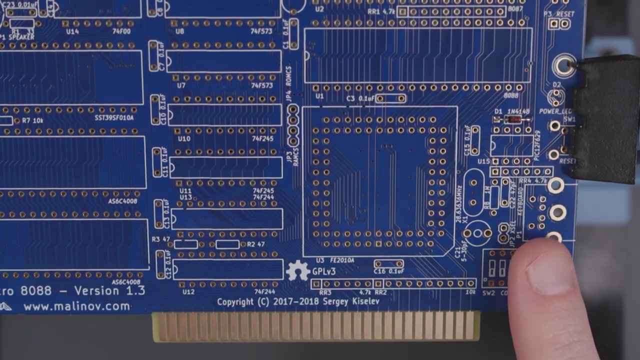 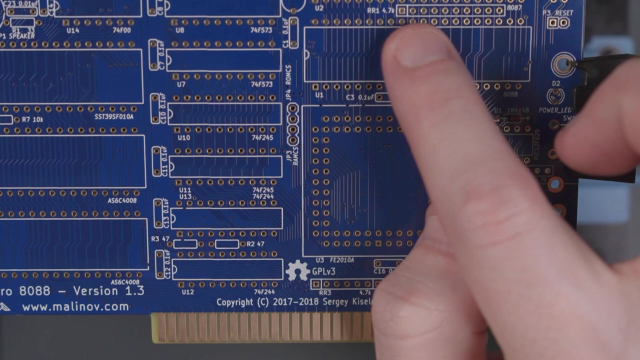 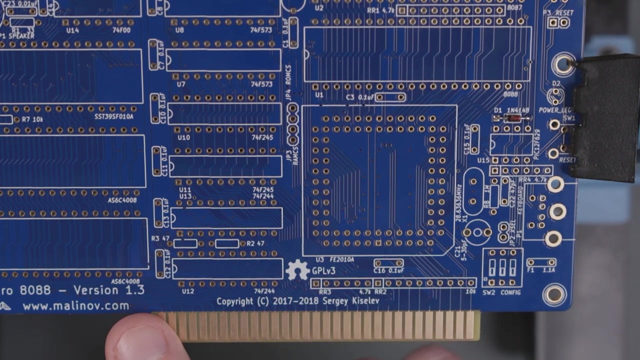 now we can go back in. all right, what are we looking for? r1, r3- oh, that was this one. r7, r6- see, those capacitors are at the edge. switch r4, r5, resistor array one: f1. come on, i'm gonna need to bring my- uh, my air conditioners up in my room soon, because it's. 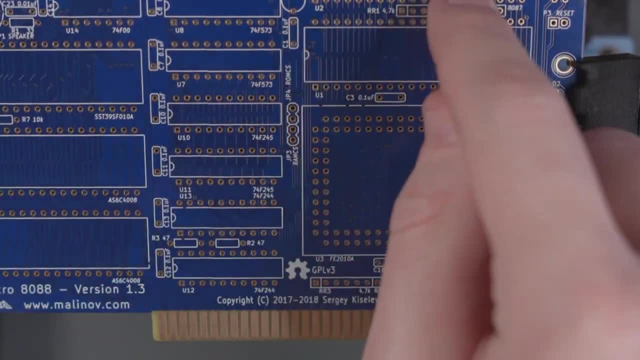 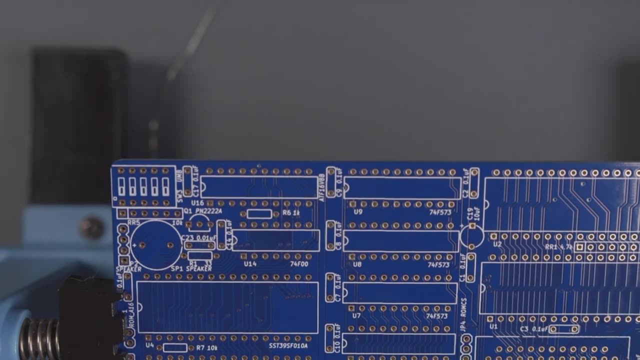 getting hot and i can't handle it. well, this is, this is annoying. where the heck is? r1, oh, r1, okay, it's up here. uh, well, um, it looks kind of um not hard to get to, but like, see, this is what i'm talking about. 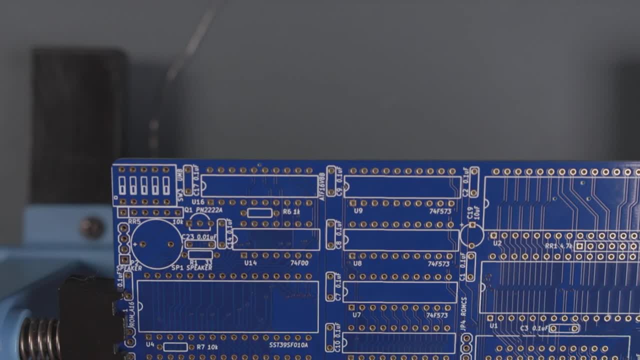 this is where my hose comes in, so that's all right. so that's what i'm dying to do is really подготов you for thisイ. this entire bag is for one resistor. I know it's kind of my bad for ordering it that way, but it is very wasteful it'd be. yeah, maybe I should think about making. 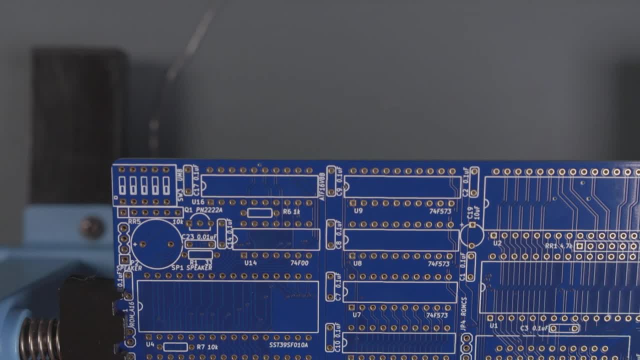 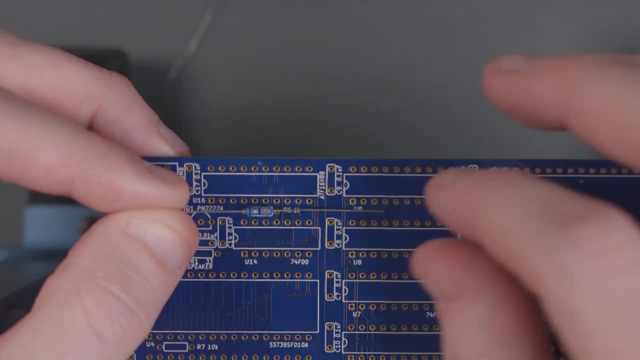 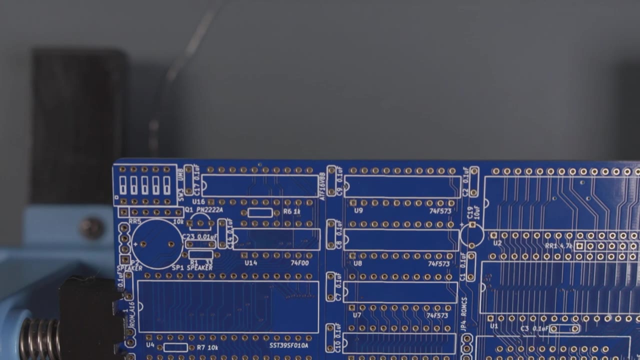 kits for these kind of open source projects. that'd be kind of cool. all right, let's see. is this one gonna give us a hard time too? probably. it's like barely the right size. I mean either that or they. they really just jammed these in there. that's a possibility. all right, I'm gonna hold off on that one too, because 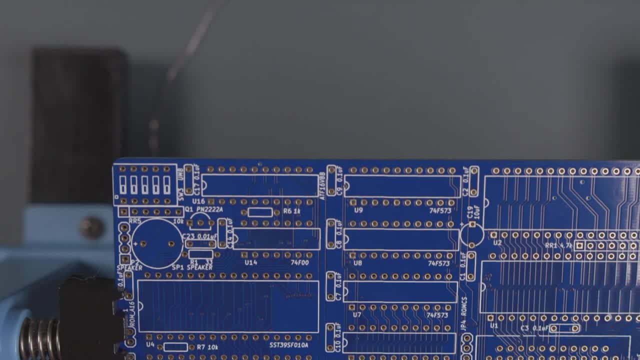 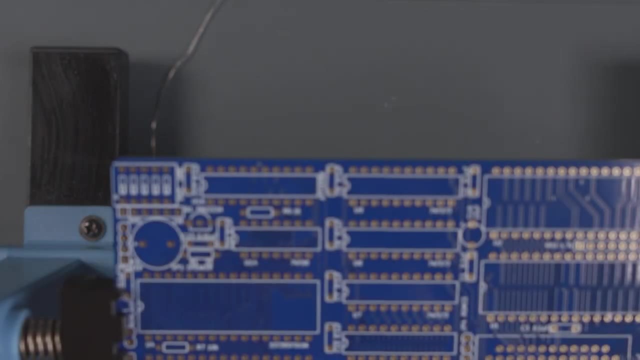 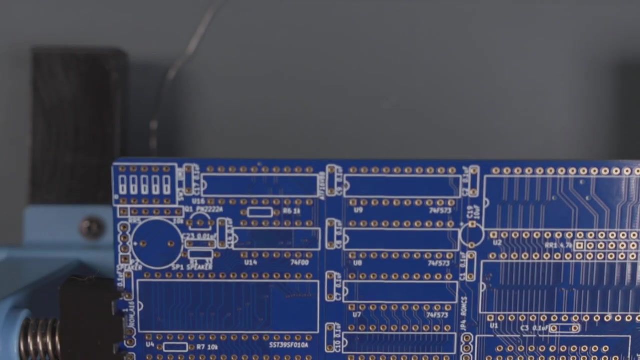 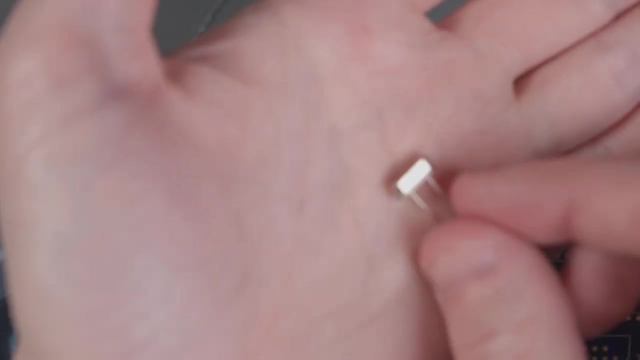 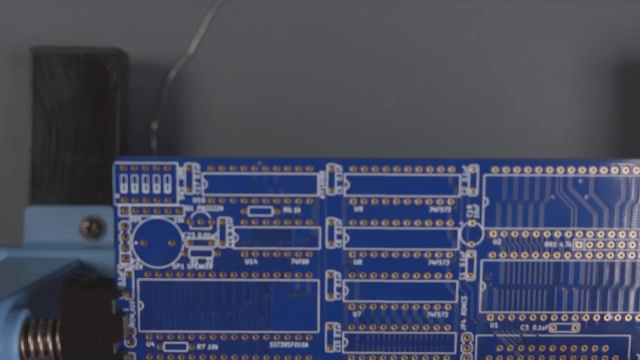 yeah, they're just kind of big. get rid of some bags, though. that's good, all right. next, grabbing from the pile x1. that is the the clock. the clock for the crystal. I mean, let's see, that should be super duper high, right? well, I don't know, it's not super high, and clocks are also not a clock, crystals are. 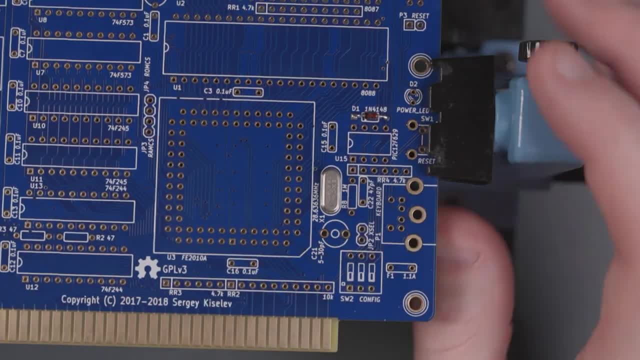 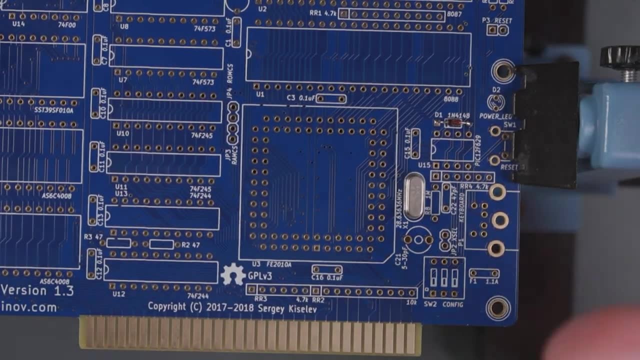 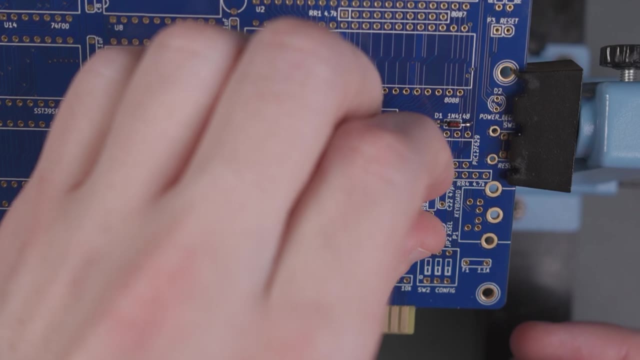 also not directional. I don't know. is that low enough? probably? I mean, they're really the next step up is what? and I'm not super concerned, I just. I'm more concerned about making sure that everything is as flat on the board as possible. so let's just do this while we have it. I don't think the clock goes in. 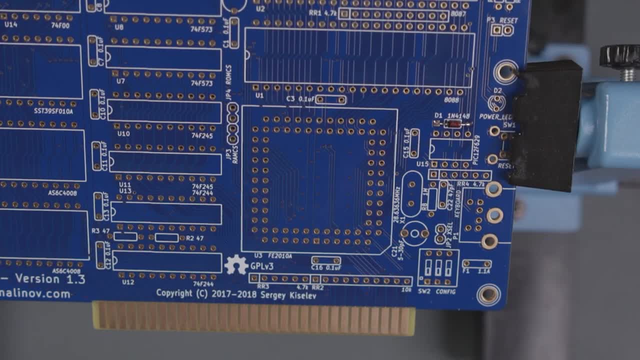 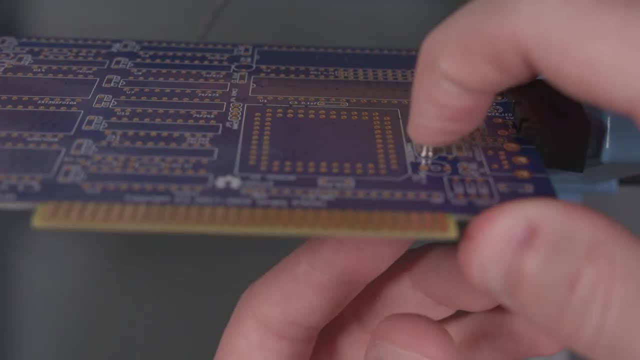 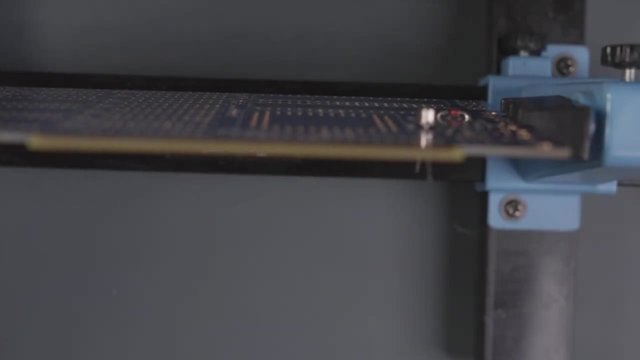 any specific way. there's no markings or anything for direction on or on the board, so I think it just goes in. so then I'm gonna like spread the legs a little bit like that, just to kind of, and then you know, I'm not really super sure that that's like. 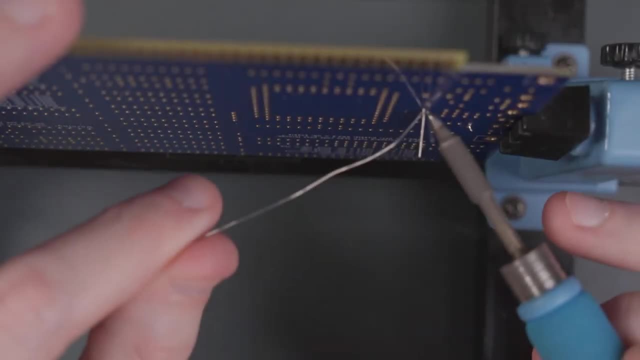 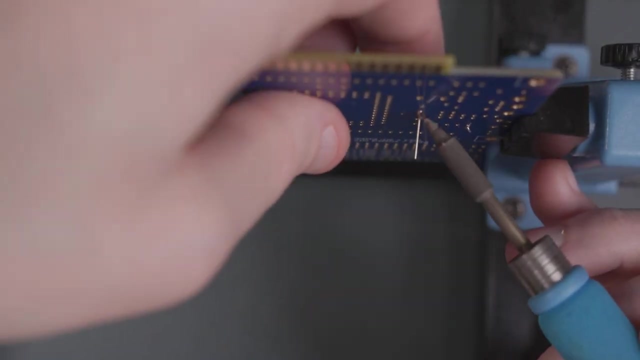 flat it's. I know it's not flat, so I'm gonna just tack one side, wait for it to cool a tiny bit and then, using my hand, just kind of push down against the piece. okay, and then, when it's cool down again, you can let go. 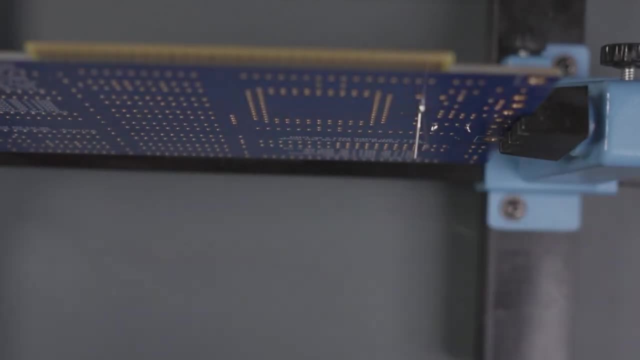 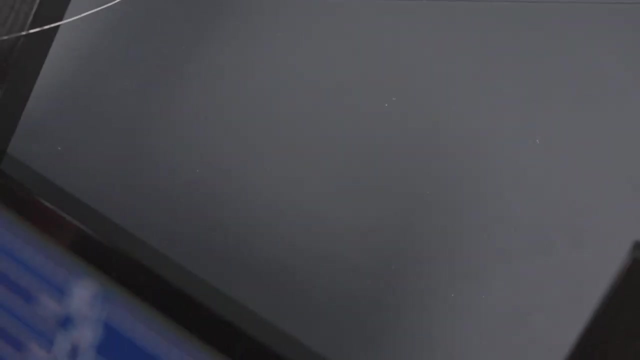 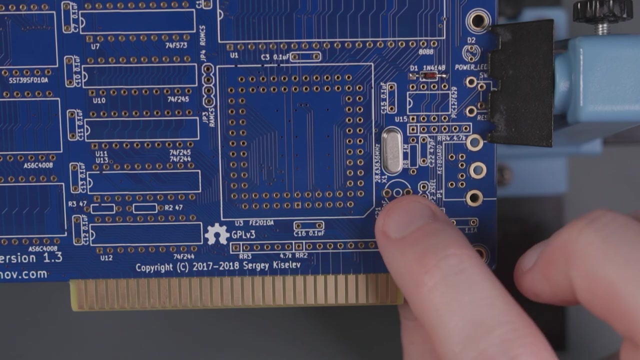 OK, cool, that's clock. let's see. what is a set. what is it twenty-eight? oh, this is not the clock crystal for the computer. I don't think this is the well. maybe it is that are. now it could be, because I know this. this is a. 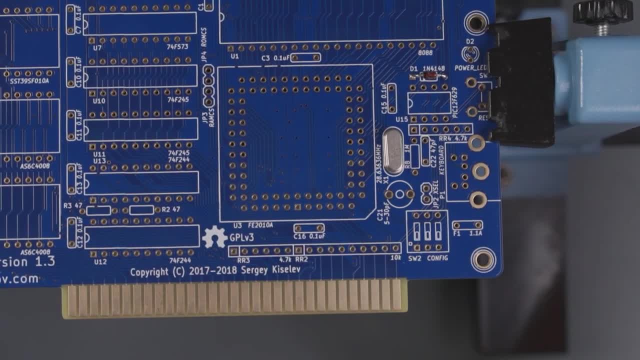 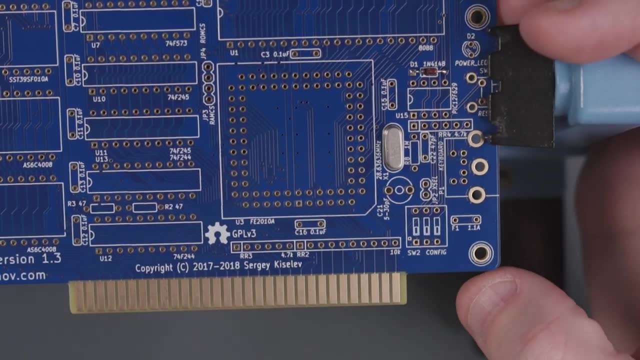 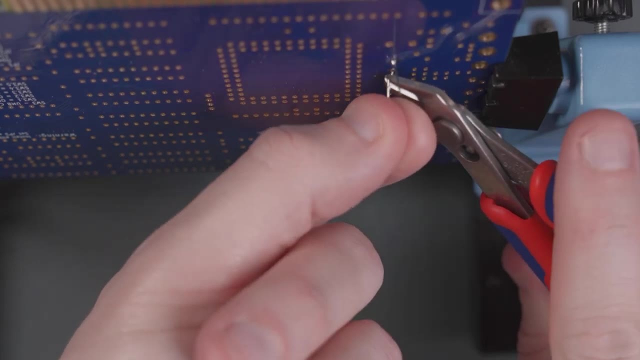 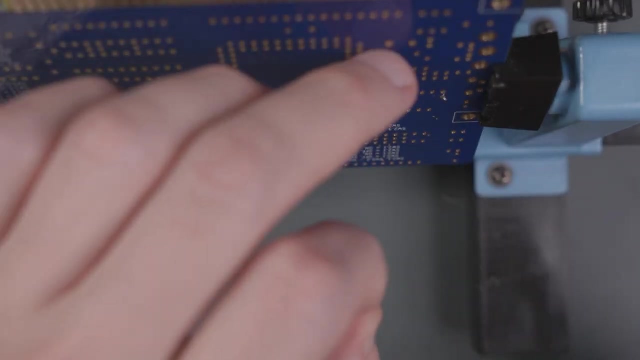 potentiometer here, or a capacity potentiometer, something like a variable capacitor or something that you can adjust for us from the point of coming to the world, the NTSC frequency or something like that. so I think it has to do with it's either NTSC clock or the CPU clock. I'm not sure about that. okay, 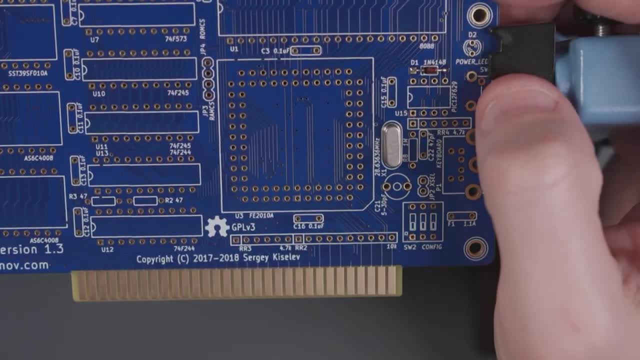 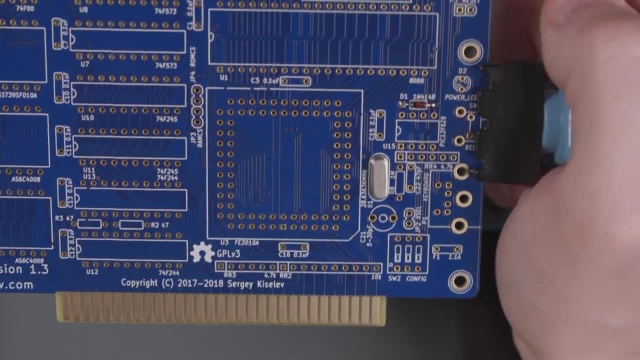 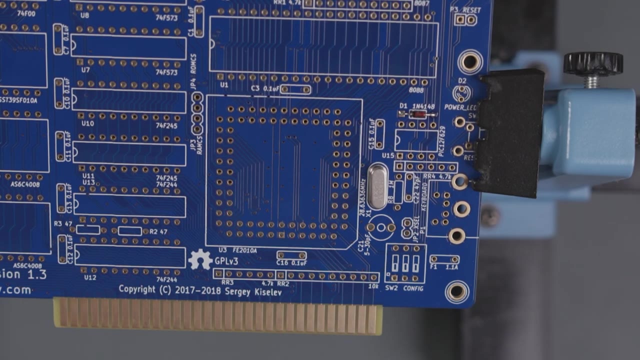 clock should matter, okay, there you always order a bunch of time, so I'll have leftovers for other projects. yeah, see, I do that and then I leave them in the bags. then I never do anything with them again, so I don't know. yeah, you're right in theory. that's a good way to do it. okay, so we finished a single bag, ah. 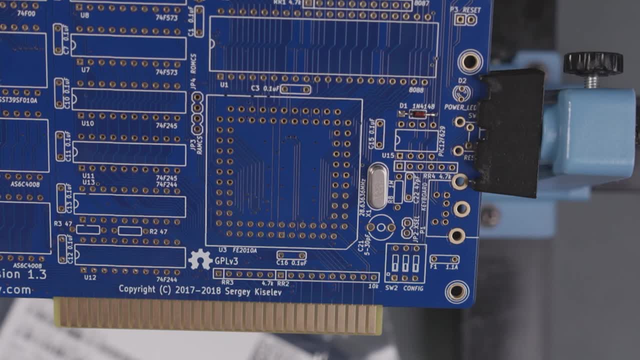 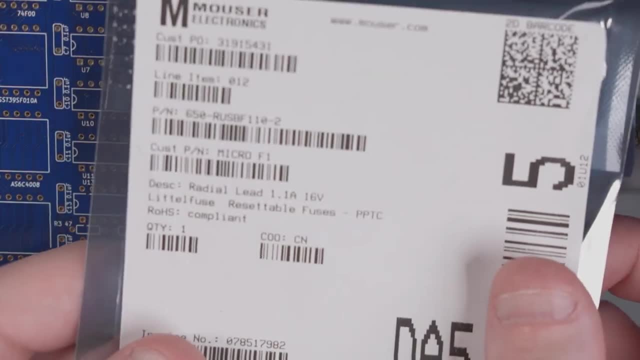 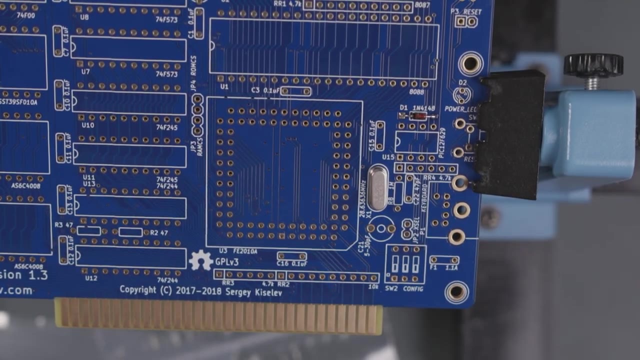 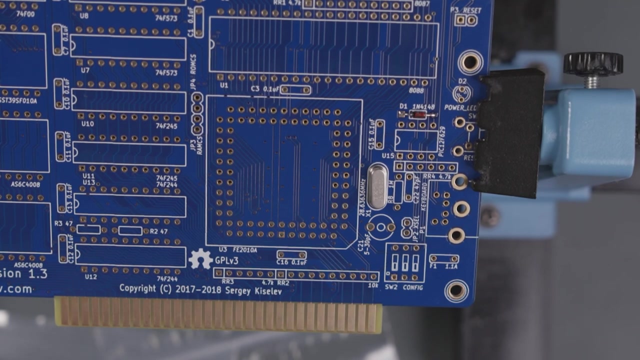 okay, I have to make sure not to lose any of these parts that I have open. okay, all right. next let's see. this is f1, which is a resettable fuse, apparently. oh, and it goes down here in the corner, all right, let's see what this looks like, this tall, tall boy. oh, my god, yo dog look. 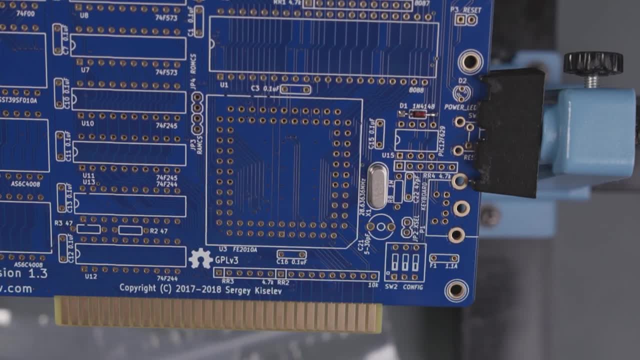 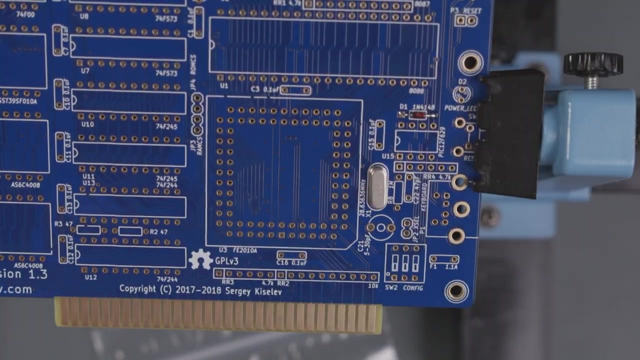 how huge this is. well, I guess that's not going on yet. that is very tall, but that's fine. it'll join our sky-high resistors later. perhaps I'll come back back later. oh, this was oh C 23. okay, we're kind of getting into capacitor land. I'm making a. 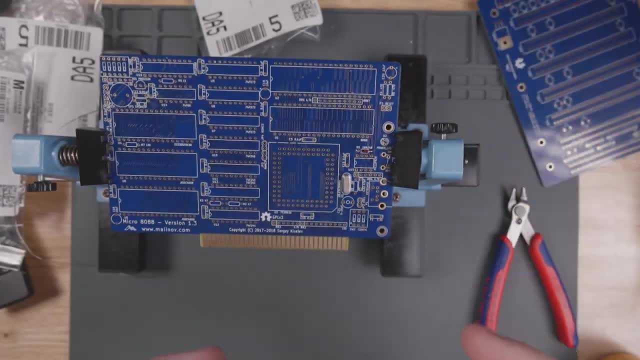 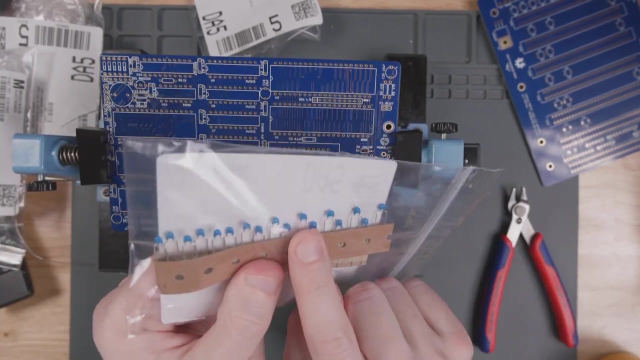 pile of the, the discrete components over there, like the capacitors and resistors and stuff that's probably going to be next after the damn well, maybe some of the dip switches, probably, and the sockets for all the chips. ok, so these are a bunch of more capacitors in there. 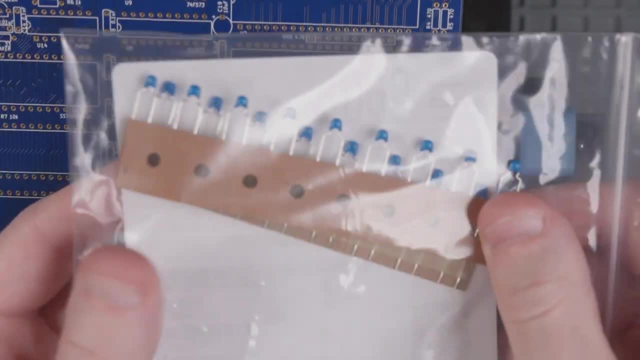 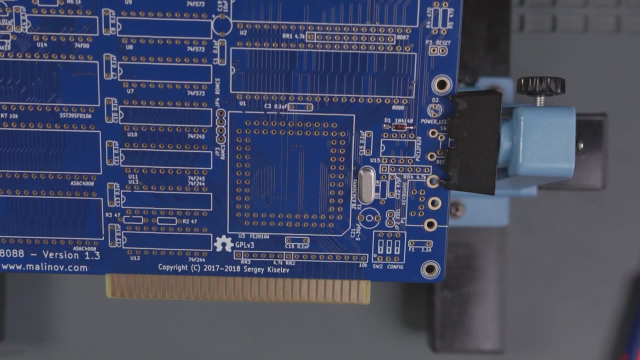 They're kind of tall so I'm not going to start there, But I'm putting them in a specific pile. All the other big parts and stuff I'm putting them in a different pile. Okay, U10 and U11.. Okay, those are chips. 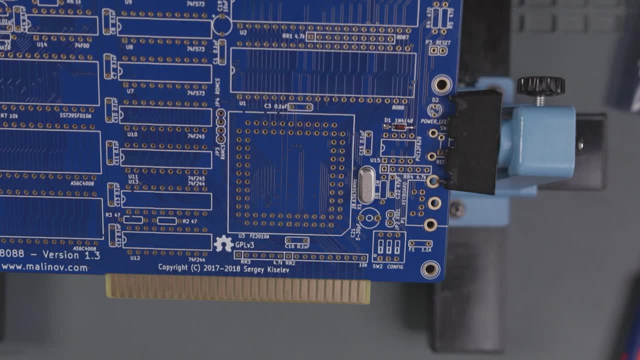 So I'm going to make a. I guess I'll have to make a different pile. My gosh, my desk is Rip my desk for, like the next week, It's going to be a mess. Okay, now we have. 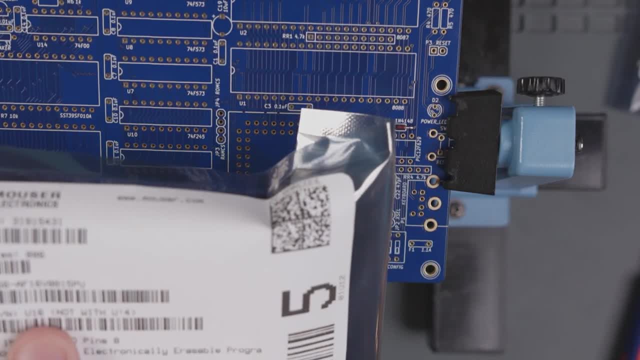 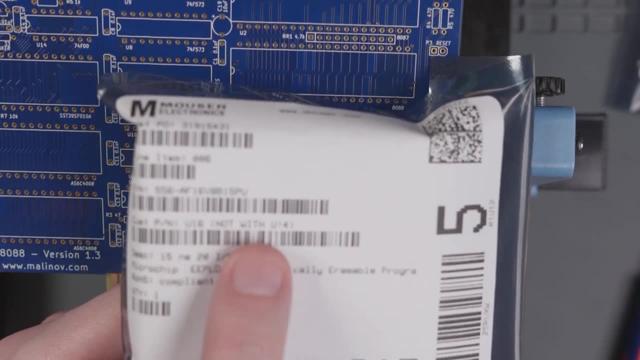 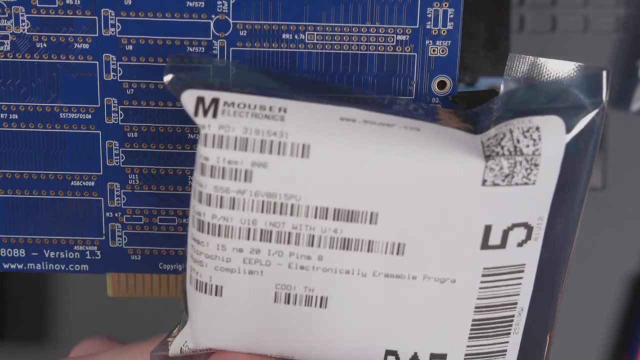 We have U16. Okay, so this is a chip. So Okay, we'll have to read. There's a footnote here. See how I wrote, not with U14? I guess I put U exclamation mark, for There's an alternative path you can do, depending on what you want to do. 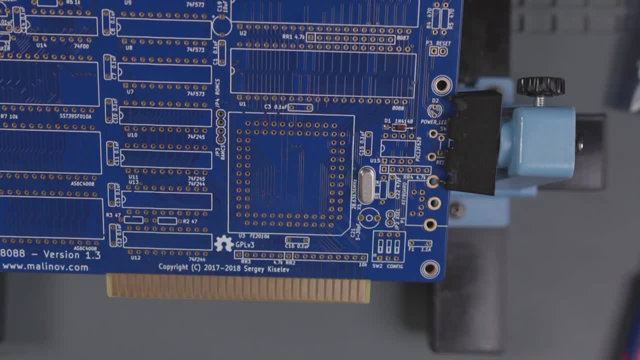 But we have to read that. there's a note in the repository that we need to come back to. All right, so I got more, More resistor arrays. I've got an LED That might be kind of short. I'll wait and do that with the resistors. 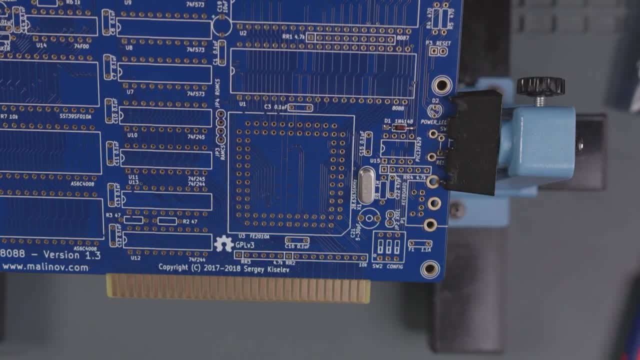 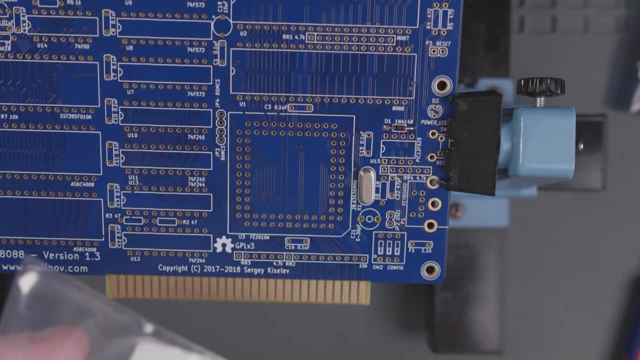 More capacitors, More capacitors. We might be getting there sooner than I thought. Okay, P3.. What is P3?? Oh, Okay, so these are little pin headers, so that's fine. They're kind of tall, so we'll wait. 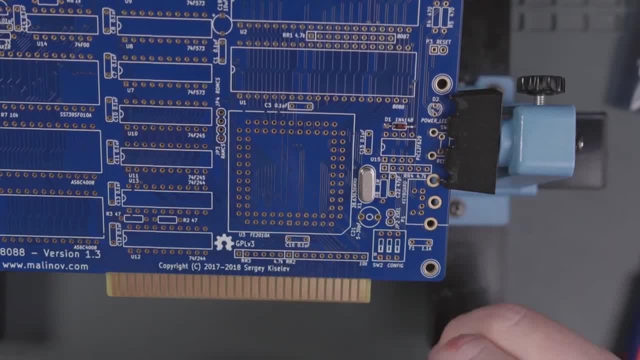 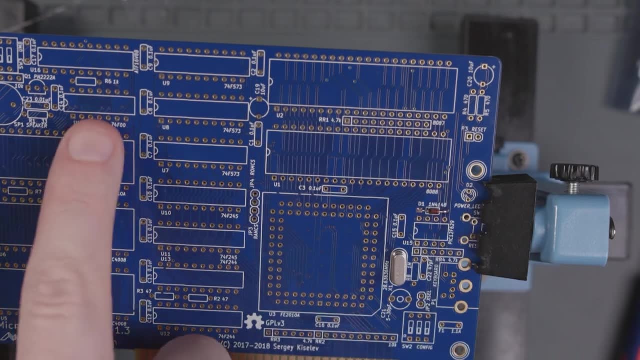 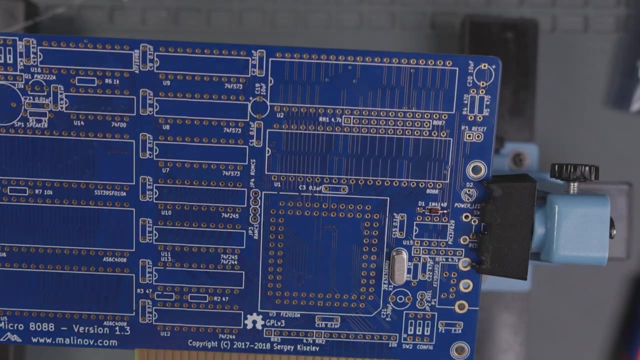 R6.. I feel like this is going to be another R situation. Yeah, it's up here, But I believe it's probably going to be the same kind of deal where it's too big for its hole. So we'll wait on that. 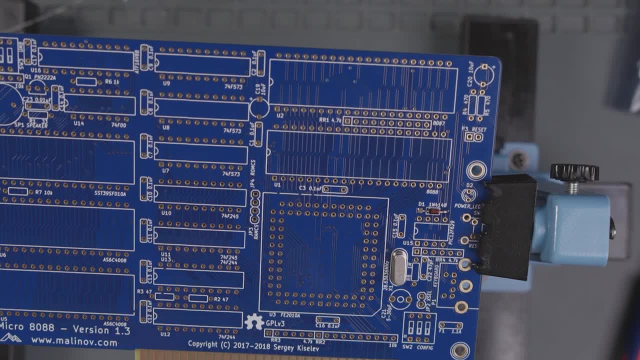 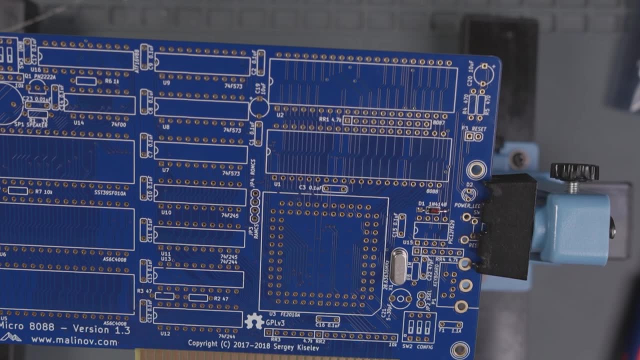 I guess I don't know What's next, What's the next level of things? I guess we can look at the switches. Maybe the resistor arrays might be low. This is, Ah, this is all the ISA. car edge- excuse me, car edge- connectors are in this big long box. 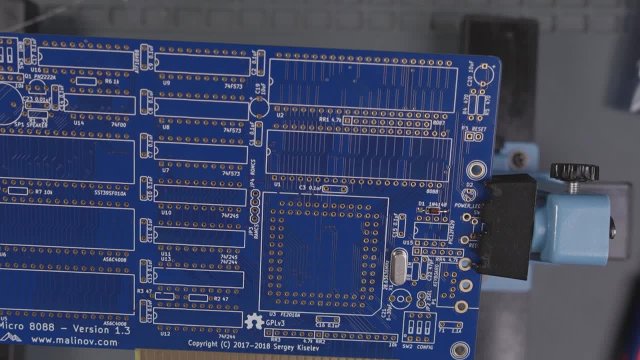 So I don't even need that yet. Won't need that until Well, actually, you know what? I have another bag. Let me check the Mouser bag. What's in my Mouser bag, Or my DigiKey bag, I mean? 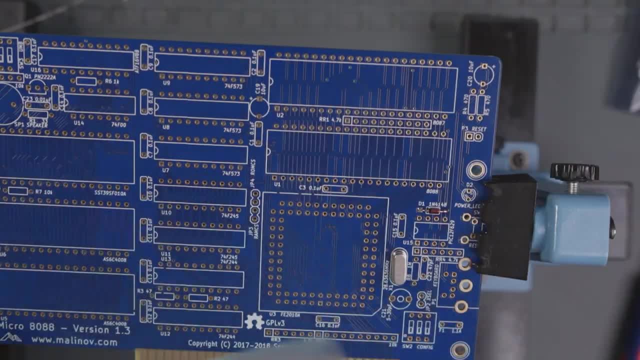 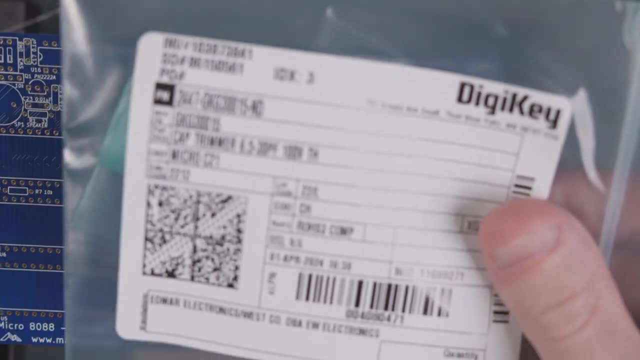 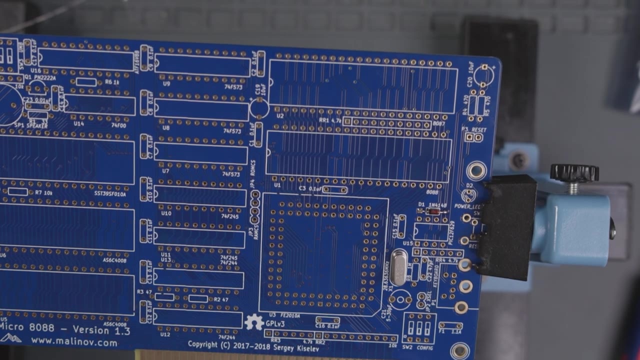 Just more caps, More and more caps. Oh, this is that trimmer pot. the trimmer cap Is a potentiometer, a capacitor, or is it a resistor? I thought it was always a resistor. More resistor arrays, so that's cool. 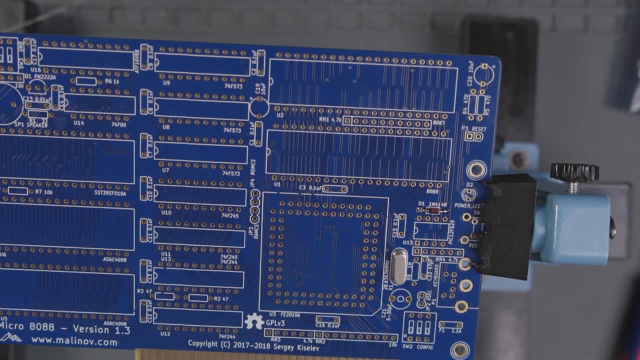 We're getting there, All right. I really want to get to the, Not the chips. I want to get the chip holders. Oh, here they are. All right, Let's see how tall these are, because this might be our next step. 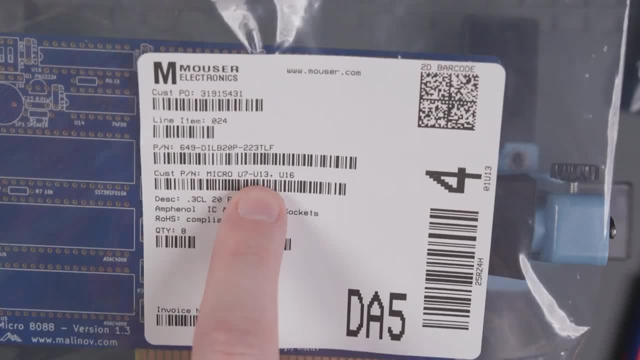 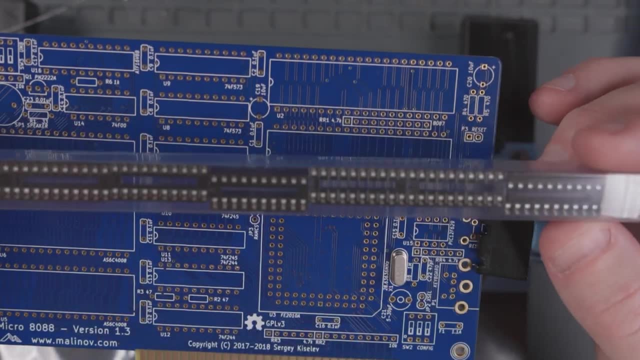 So this is what This is: U7 to U13 and U16.. And these are nice sockets. They're double wipe ones, which means that there's metal on both sides: There's metal on the inside and the outside, so that's kind of cool. 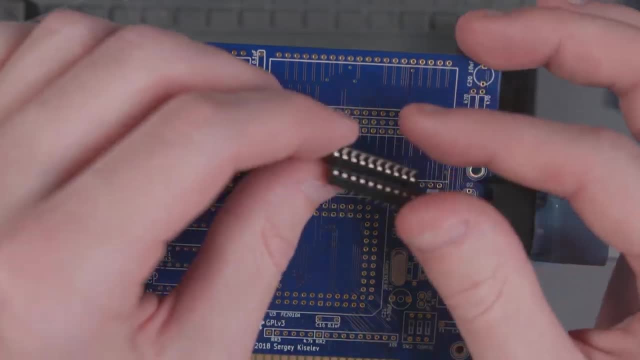 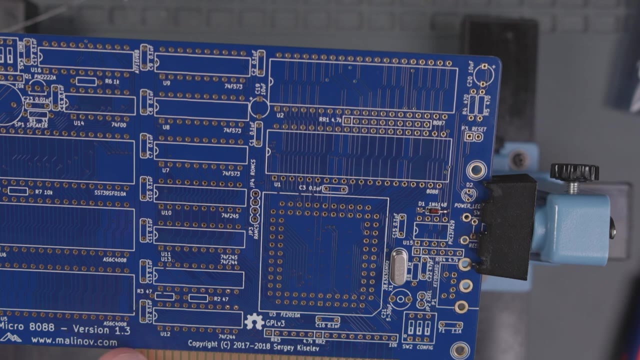 So let's start with these, because I don't think we're going to get any other discrete components lower than that, unfortunately. Yeah, These capacitors are all kind of high And the resistors we have to do that weird thing with it. 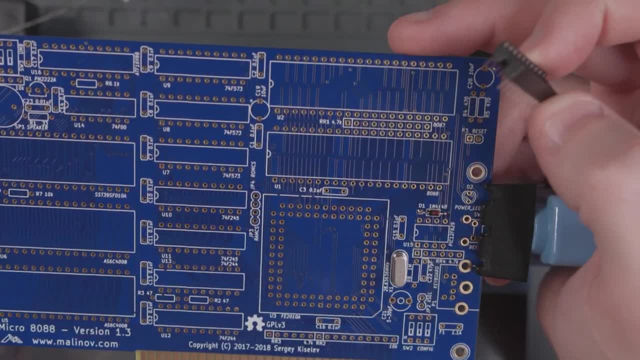 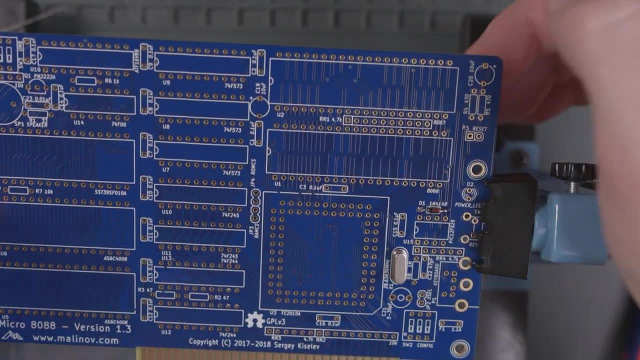 So we'll just come back. Maybe the It doesn't really matter, because the reason why you do the low to high is so that you can flip the board over. But I'm using this weird thing anyways. It doesn't really matter, Okay. 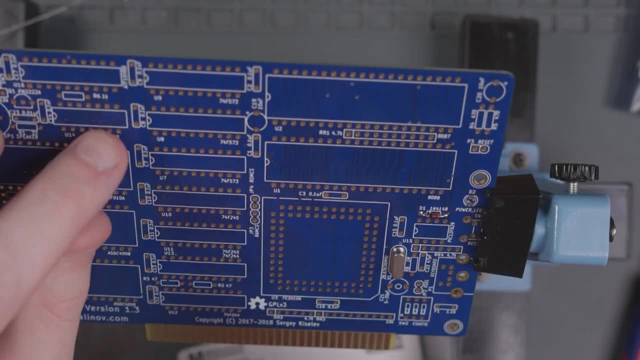 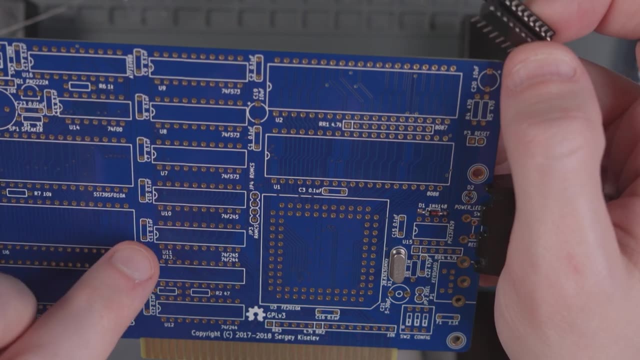 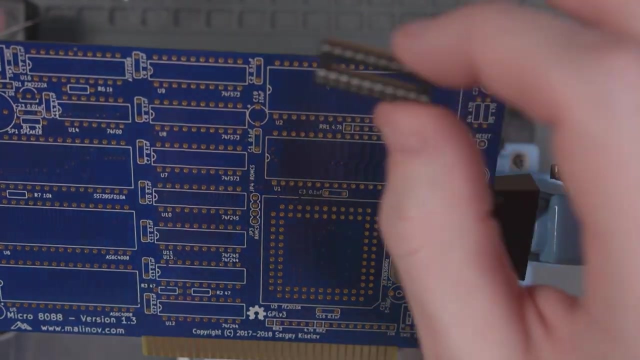 So these sockets go on U7 to U3.. Okay, So we got some kind of a weird layout here, So U7., U8., U9., U10., U11., U13. And U12.. So the names of the parts are kind of out of order, but it seems like it goes U7 through U13. 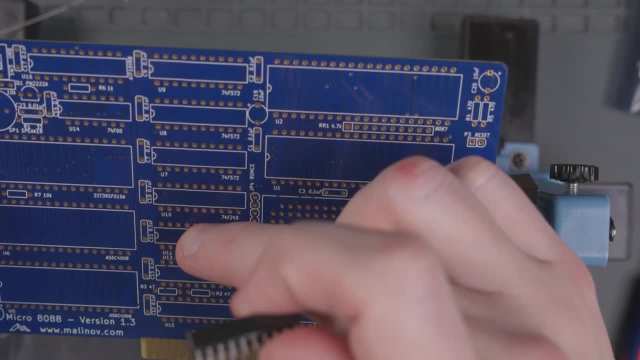 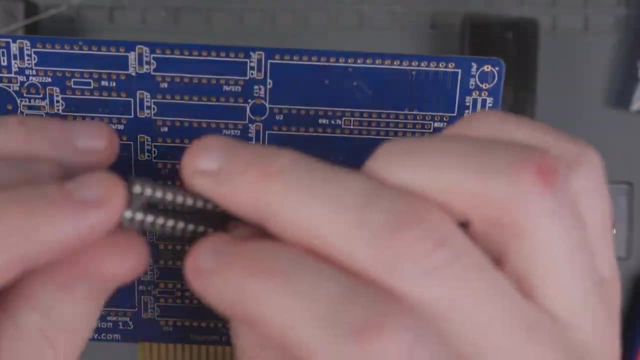 So that's U7,, U8,, U9,, U10,, 11,, 12, and 13.. And U16 up here. So you want to make sure there's a These. I think this must be the ramp. 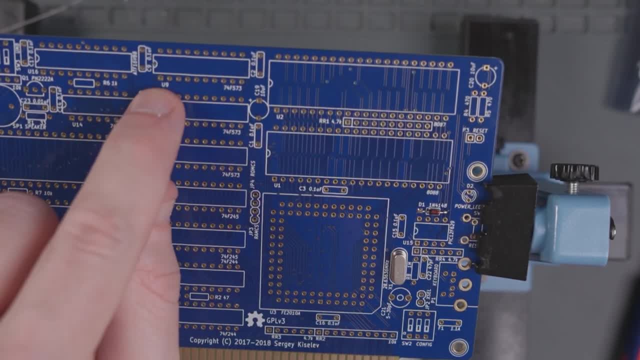 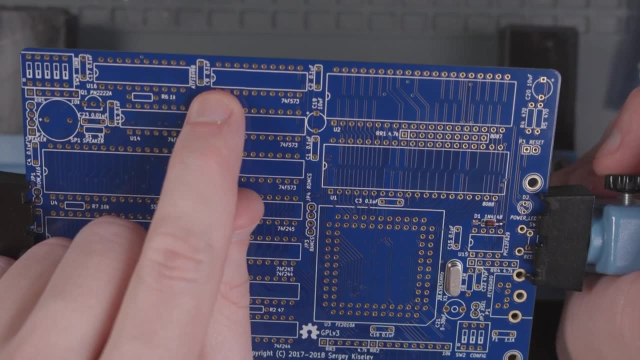 But like all these larger sort of dip package chips, they are directionals. There is a little moon, or half moon, I guess, or moon. There is an eclipse on our PCB. That is kind of like the That is also going to be on the chip that goes in there. 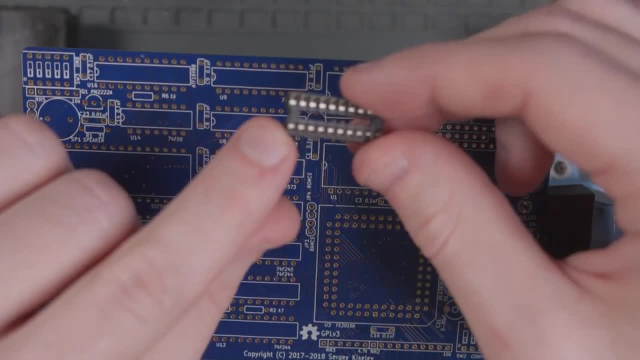 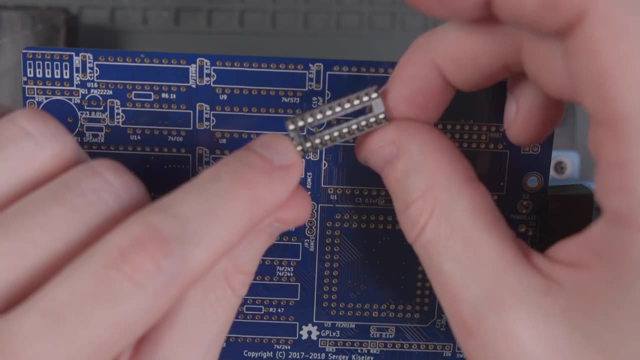 And it's also on the socket. So there's a little thing, a little half moon on one side, but it's not on the other side. You can see that. So that goes in like that. Now, with these it's going to be kind of hard. 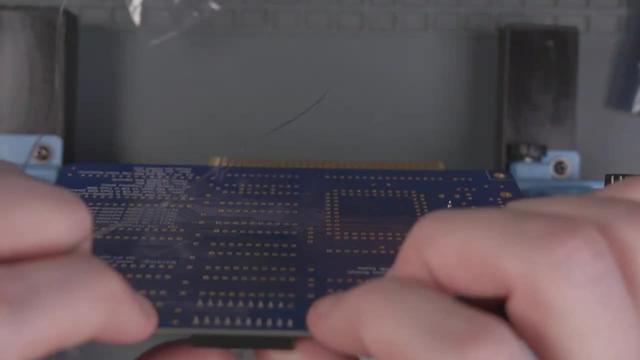 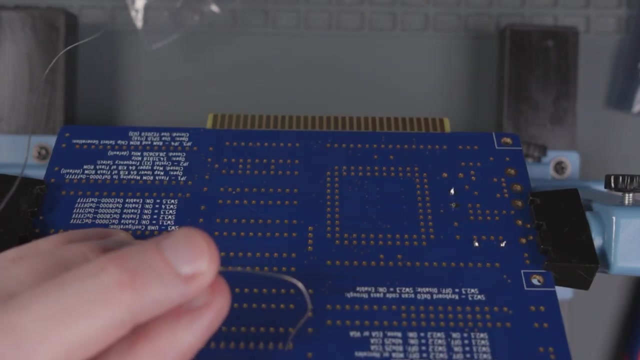 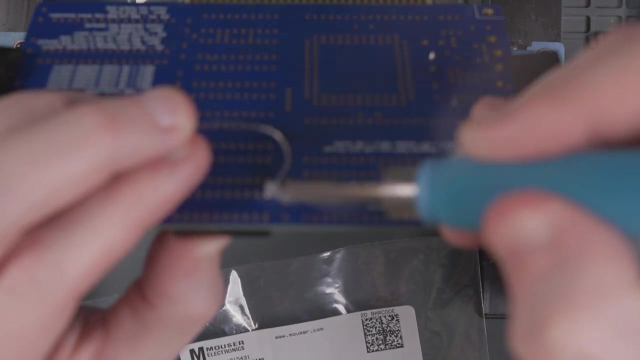 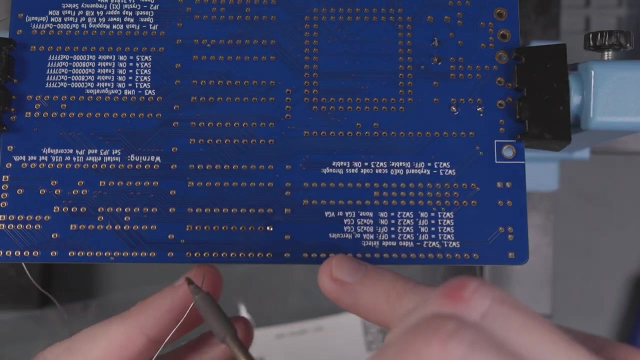 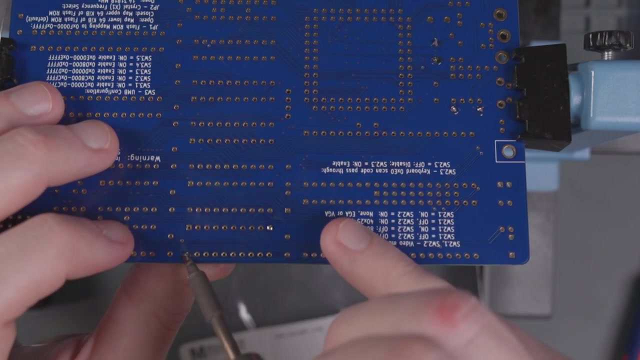 Let me see, I guess I can do this. Having this holder thing kind of makes it a little easier, Okay. So get one on one side And then one on the other side, And then push up and heat it up again, Okay. 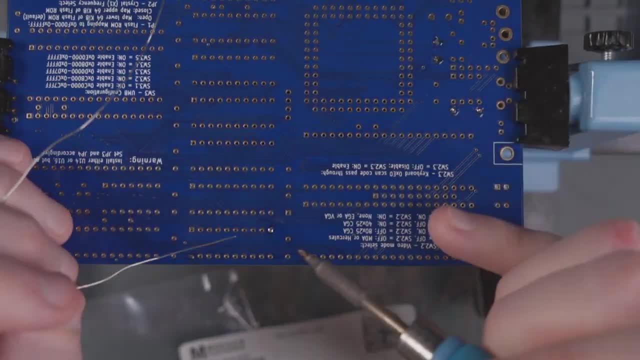 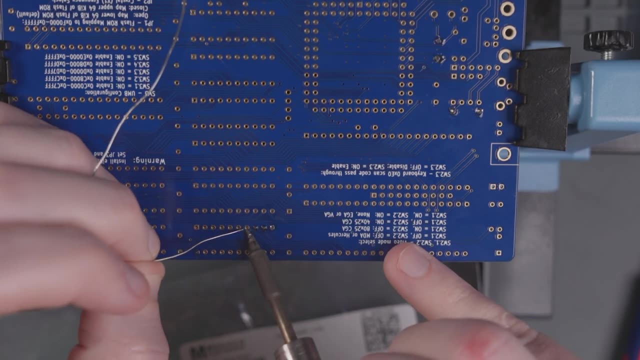 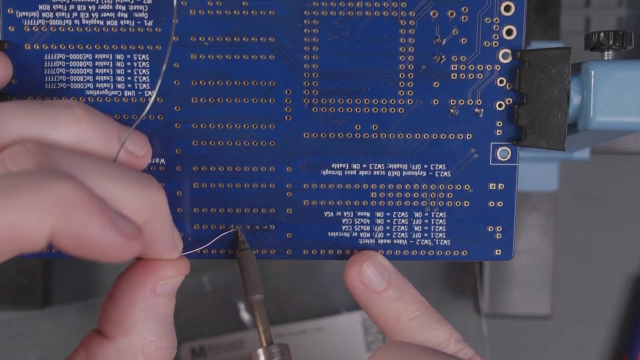 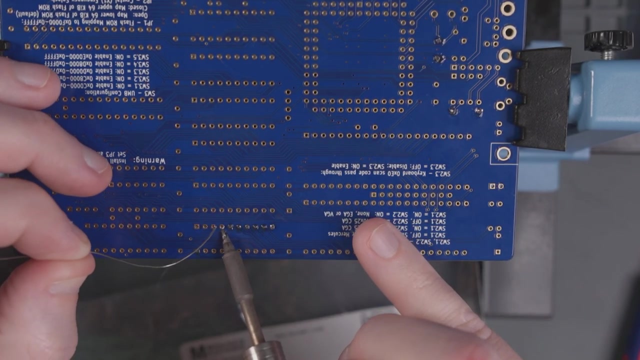 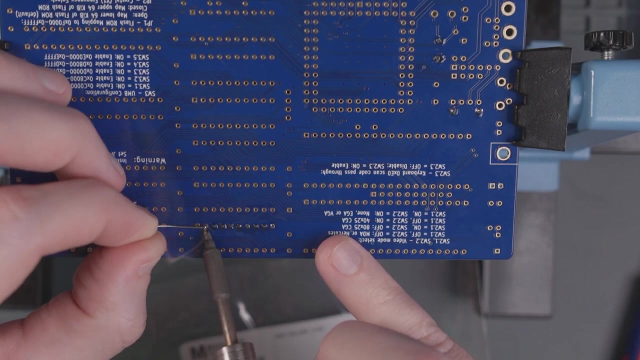 All right, So once you have one on either side, then you can just do all of them. I guess I should do some drag soldering, but Okay, This is kind of getting wobbly And you do this. That should be fine. 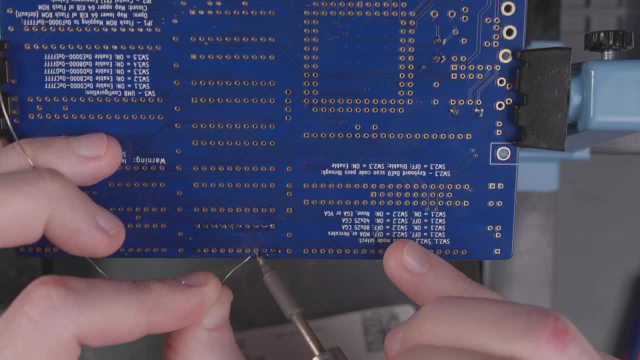 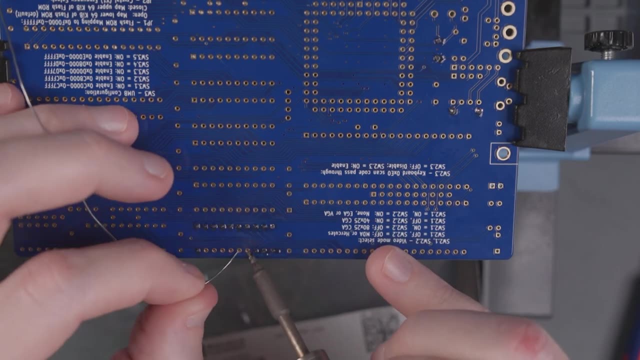 Okay, so now you got a Ave d'Ordine in here, So I just lift this toward me, Okay. Okay, There, it is All right. All right, There we go. All right, There we go, All right. 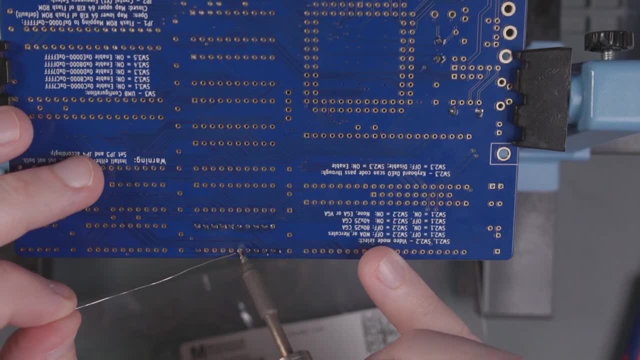 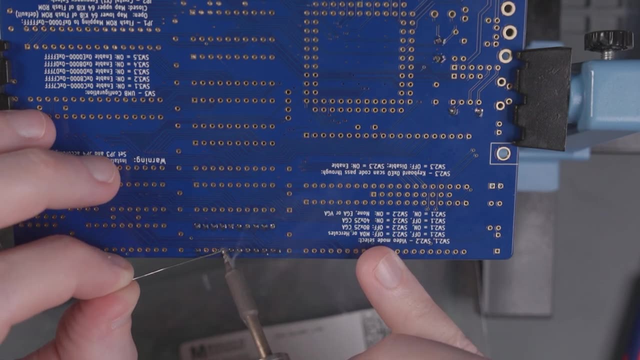 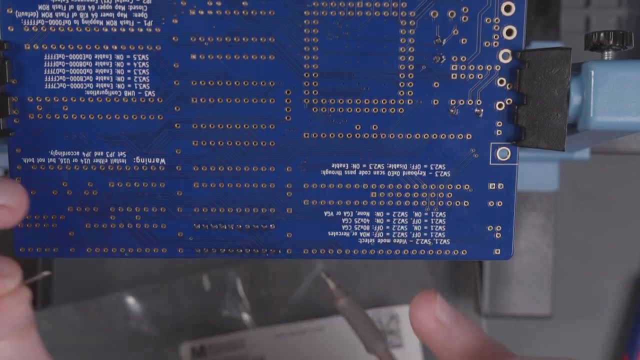 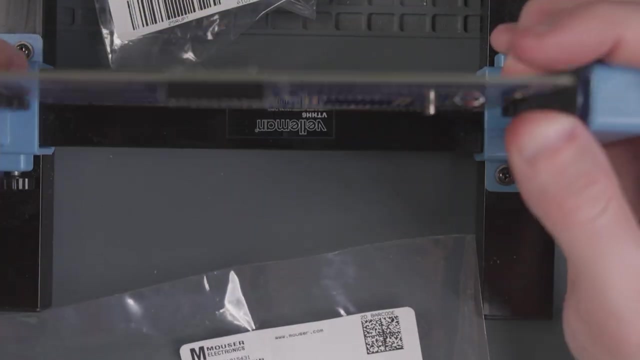 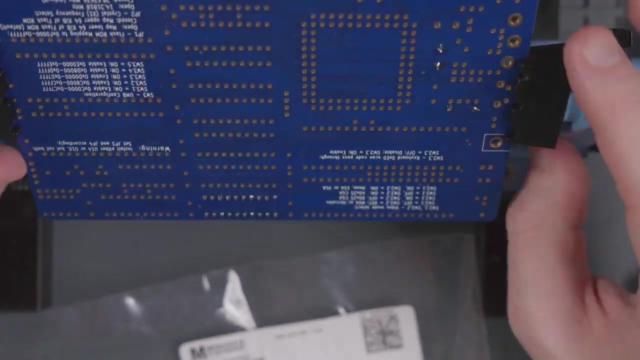 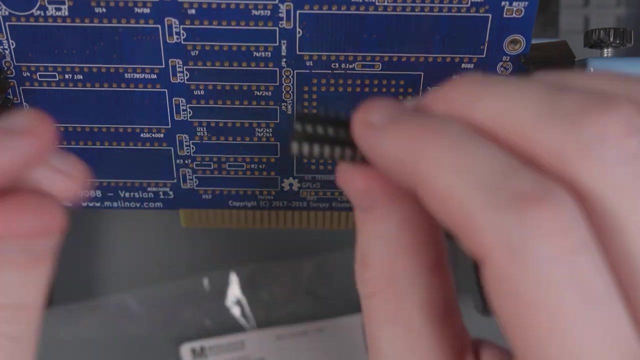 All right, Anybody playing anything fun, Playing any fun games, Watching any good TV- Alright, one down, a thousand more to go. Well, not like literally a thousand, but there are many on this project. Alright, let's keep on trucking. 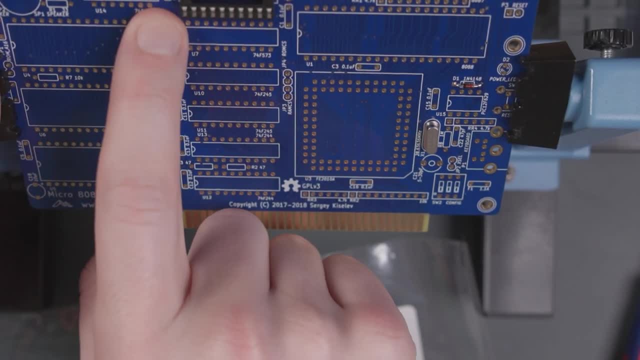 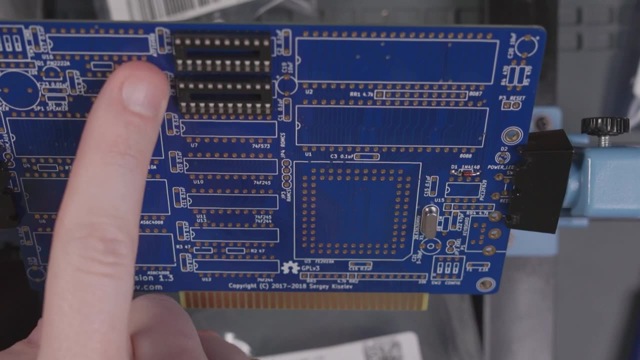 Yeah, I don't think we're going to be in trouble when we go back to solder the capacitors which are kind of like in here, Because I don't know you're going to be doing your soldering on the bottom anyways. 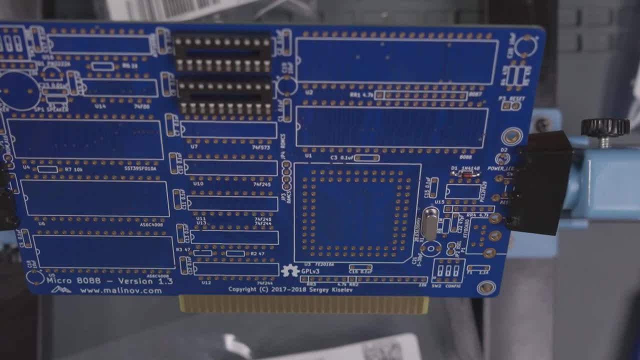 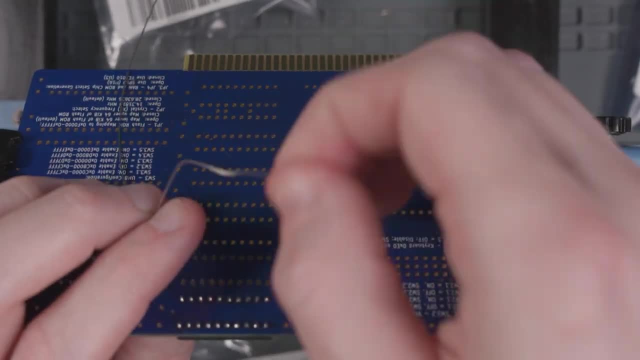 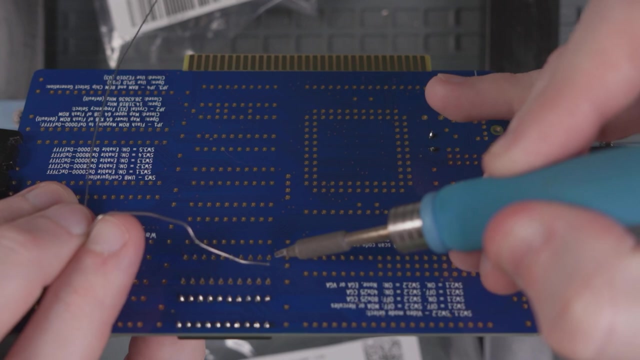 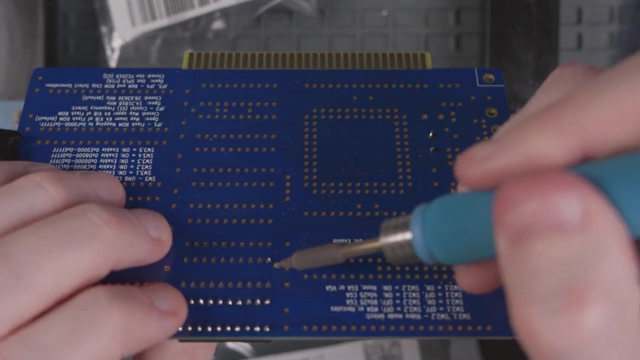 So I don't really think that things are going to get in the way, but I don't know. We're going to find out. I watched, we watched all three Crocodile Dundee movies, my girlfriend and I. It has been a long time since I watched them. 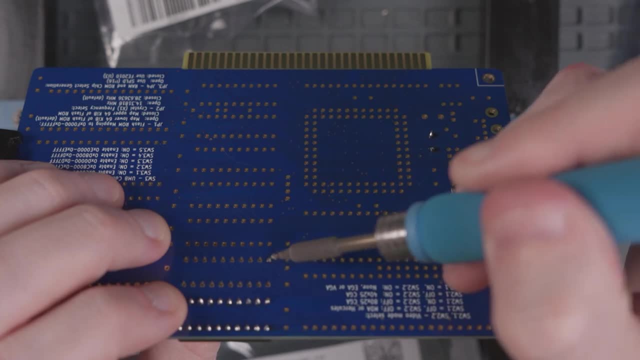 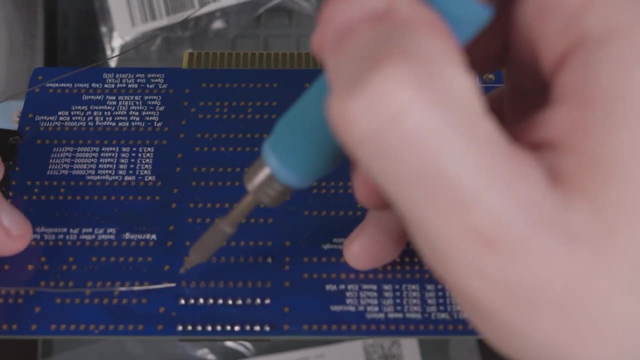 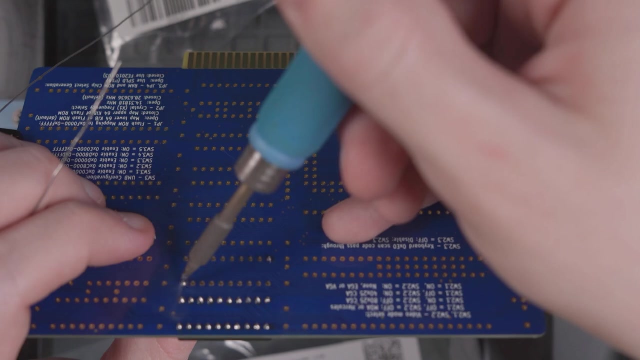 My dad really likes those kind of movies And I remember watching with him When I was younger. But like, I hope this is not like child abuse or anything, But I remember there's the part where in the first one where, like there's this guy doing cocaine or something. 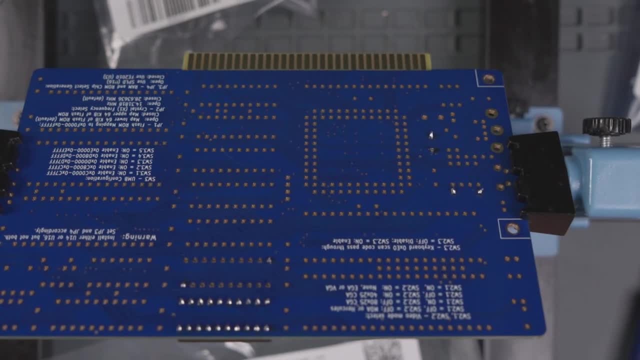 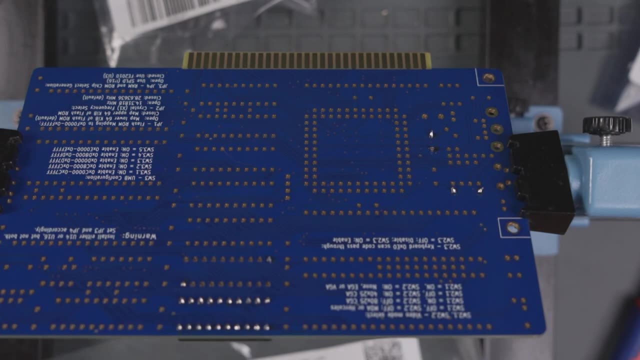 He's got a bag of cocaine And Dundee thinks it's some kind of like sick remedy or something that he wants to do. So he like dumps it all into a. he like dumps boiling water into a bowl and like dumps all the cocaine into the bowl. He like wastes this guy, like hundreds of dollars of cocaine on this guy. So I remember that distinctly, remember that one random scene And that's in the first movie. So pretty funny. And you know, I think the first one is better than the other ones. 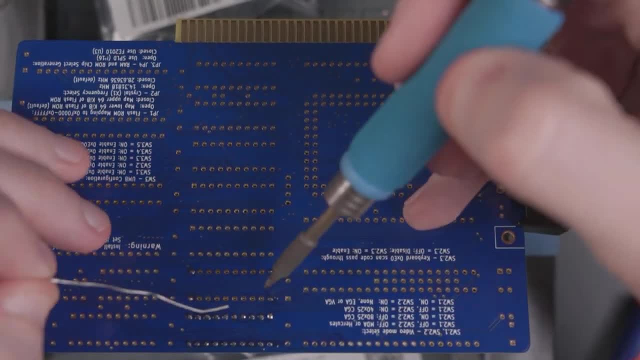 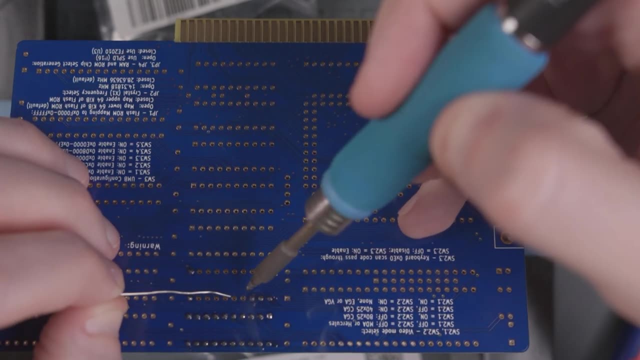 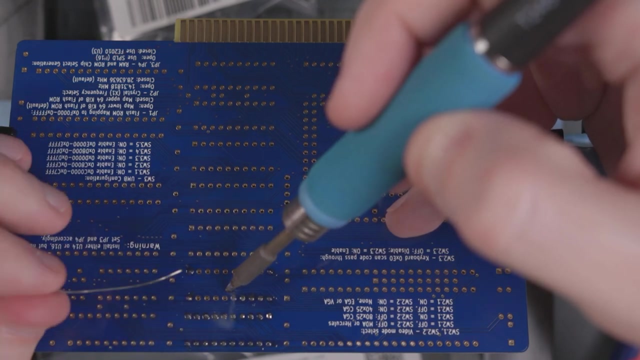 Started playing Phantasy Star for the Master System. I think I uh, I played the. I tried playing the one. uh, on the Genesis, Is that one of the earlier ones Or is that like three or four or something? Um, cause, those games are kind of like I, I, I wanted to get into them. 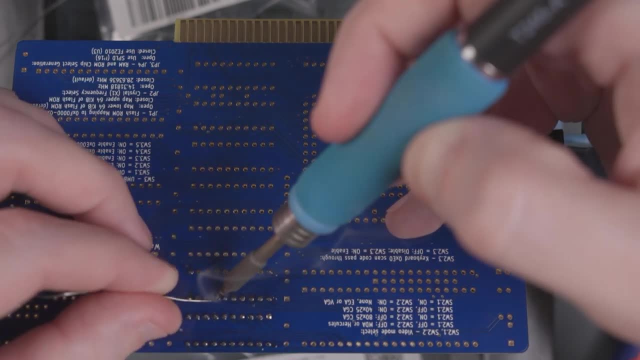 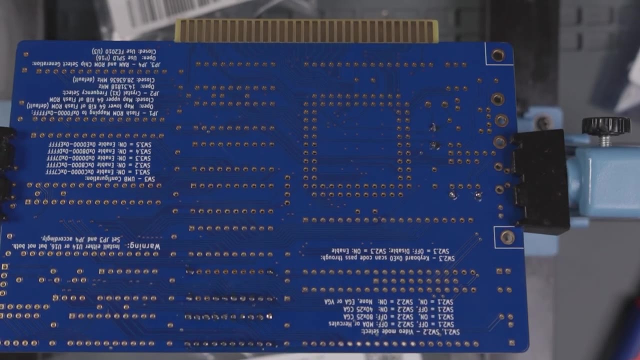 But like I don't know Something about those kind of games, um, I couldn't really get into it for some reason- Not in a bad way, It's just I don't know. That's like one of those series that is going on forever. 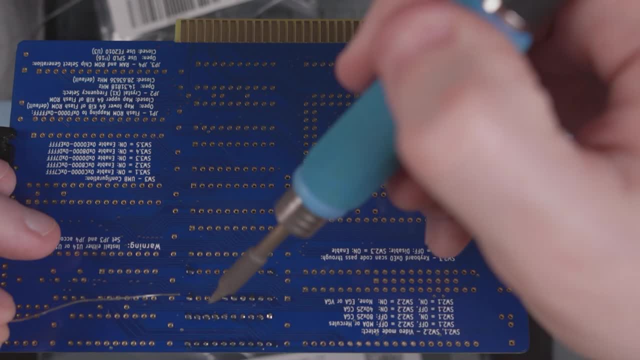 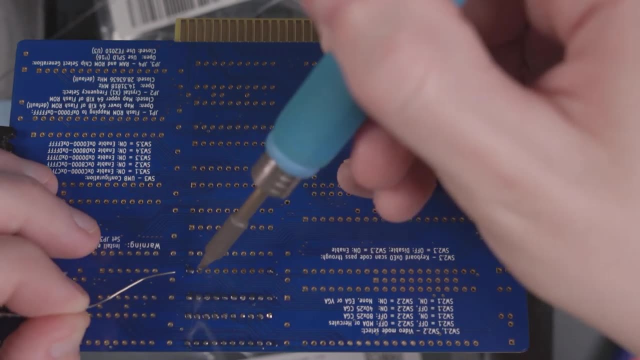 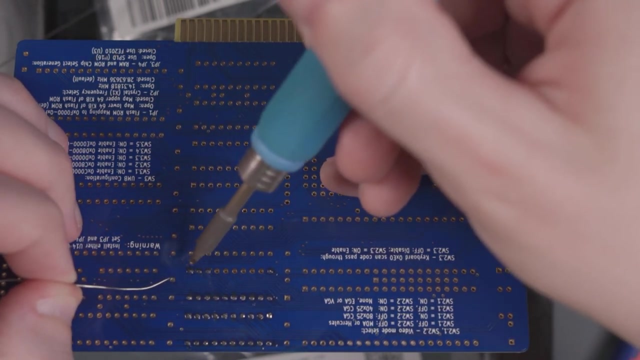 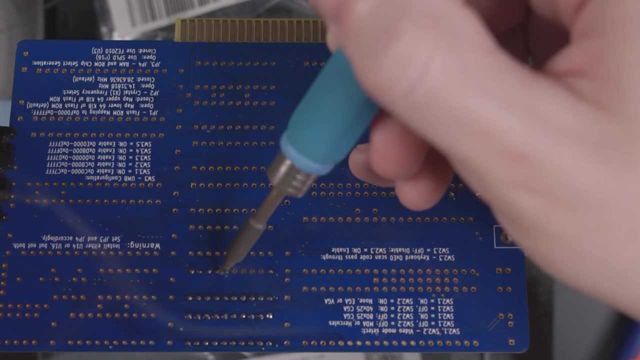 And so I figured I would try it. But It's crazy how more, how less people watch this, Or how many more, how many fewer people watch this over the Morph streams. This is what I actually do. No, I don't know. 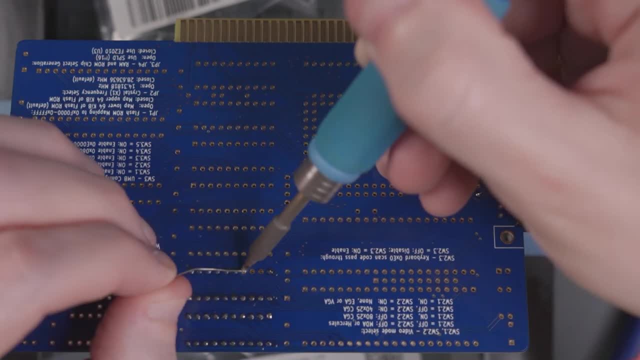 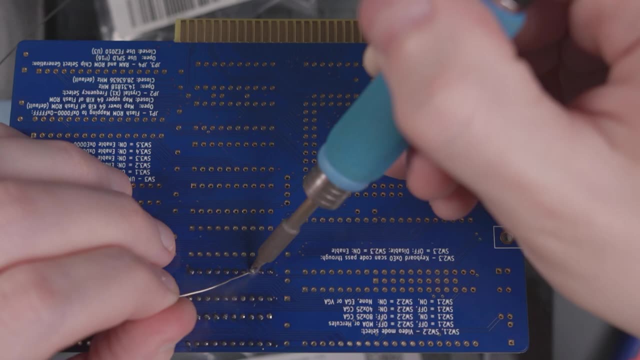 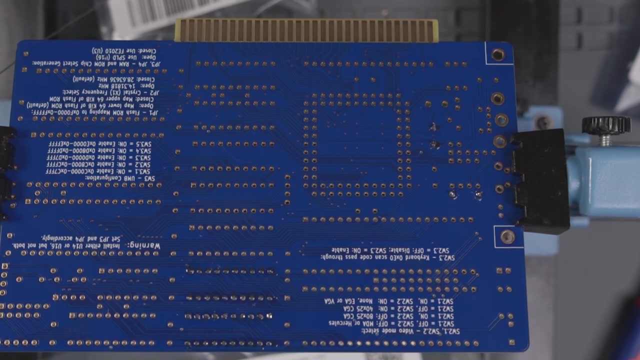 It's fine, I think you know I don't like. you know I do everything. You know I try to be interested in everything. See ya, zombie geek. I've got the stream going while packing PicoGus boards up to I, I, uh, Ian, I, I need to just. 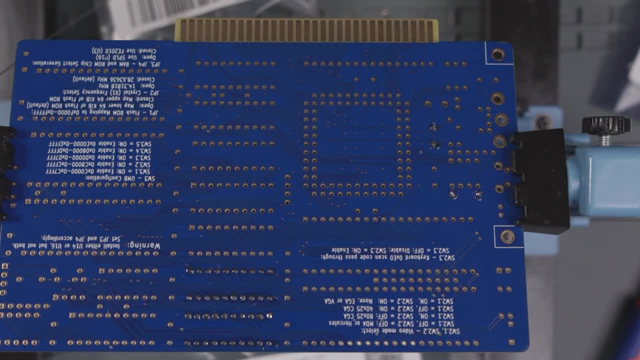 buy one of the PicoGus 2.0s, I think. if I have, well, I say this out loud, but if I have one of the boards, it might make it easier for me to diagnose the one I built. 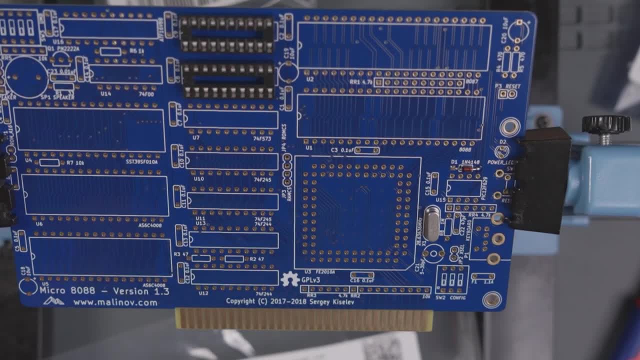 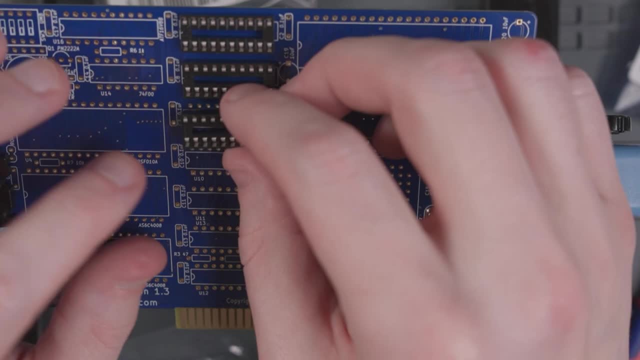 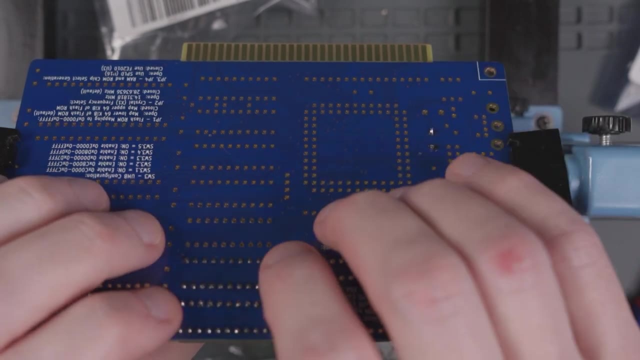 Um, but I just haven't had time. Like you know, I bought a whole- uh, I bought a whole um hot plate so that I could try to redo the parts, but it's just a lot to manage, Um, and I gotta like I'm really jealous of people who have the technical know-how. 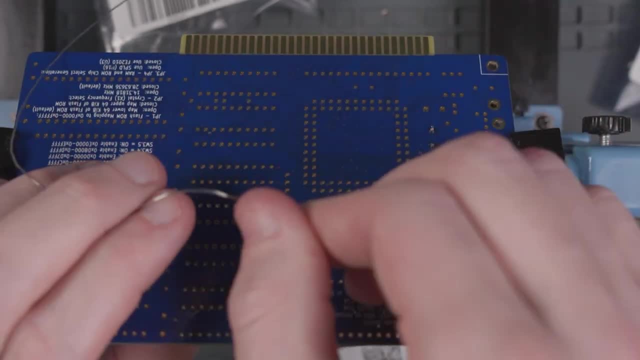 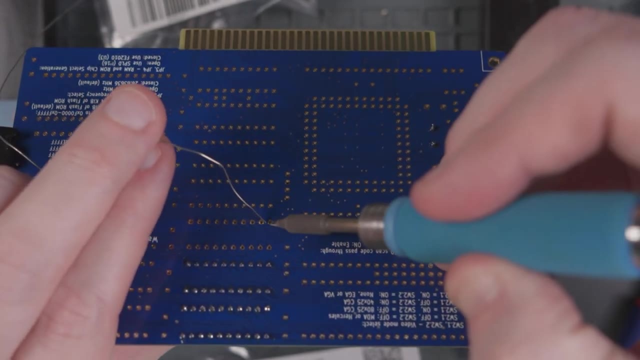 to like look at a schematic and be able to figure out problems and stuff, But that's which is weird, Cause you would think that I would be good at that. But I just like building them. I like you know, taking a person's project, their open source project- and making it real. 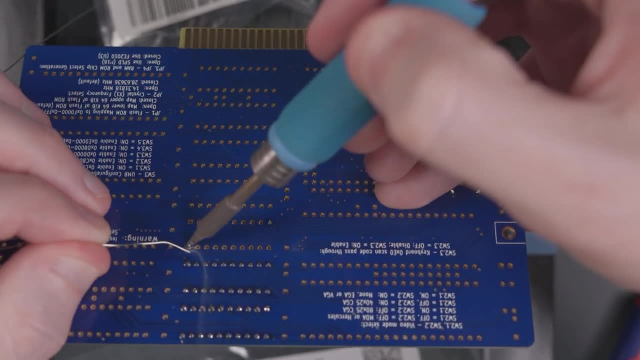 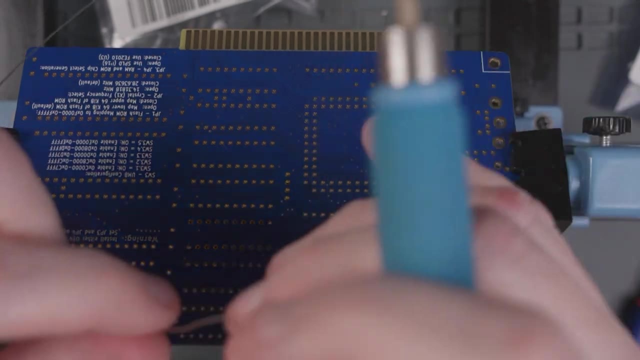 instead of it just kind of living on GitHub, and not in a bad way, I just mean, like I find it fascinating that somebody you know put all this effort into building, designing a product and all they had to do was put it on GitHub. and then I 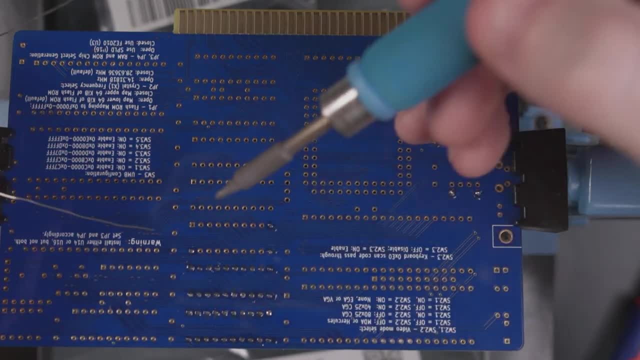 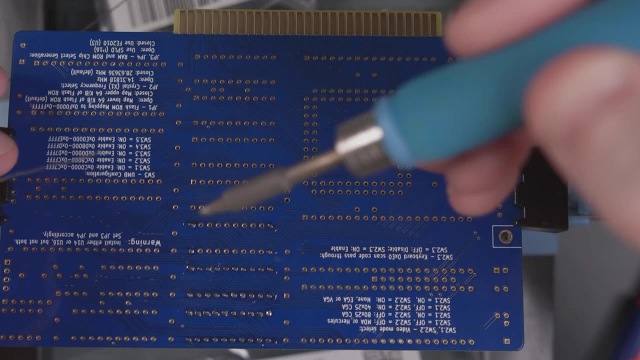 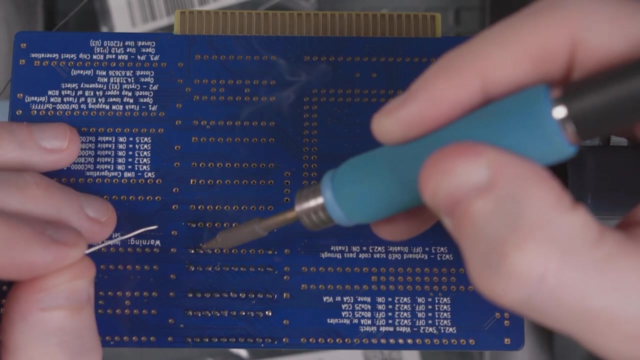 can make it myself. That to me still, every time I build a project that blows my mind That it's It's how as easy as it is to build new stuff without having to have that much technical knowledge. So that is why I'm kind of I want people to be interested about um. I would love to. 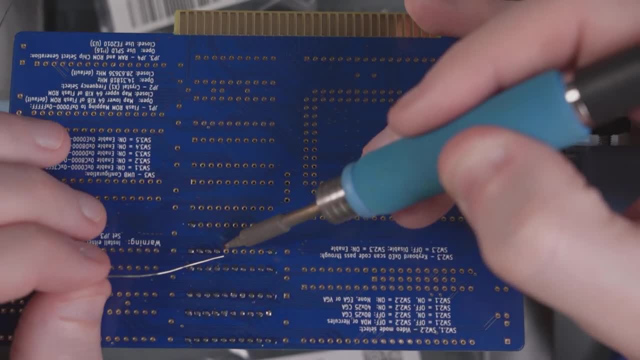 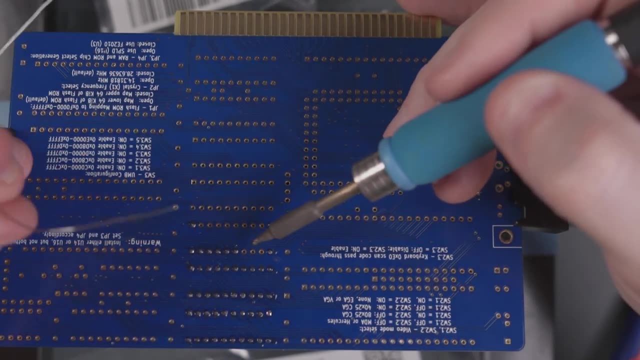 see this kind of a project for the for the newer CPU is like a two 86 version and three 86, like with 16 bit, um, or even like PCI, like you can get 32 bit. you know like I. 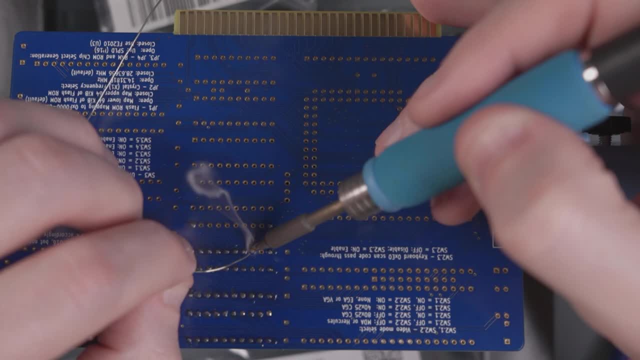 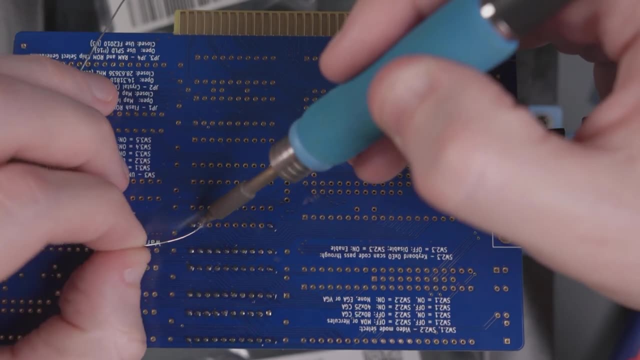 know that gets increasingly more complicated and stuff and boring Speeds and bus speeds and stuff have to matter, you know. so you can't, you have to have a well-designed layout and stuff, but still I mean it's, it's taking something that is. 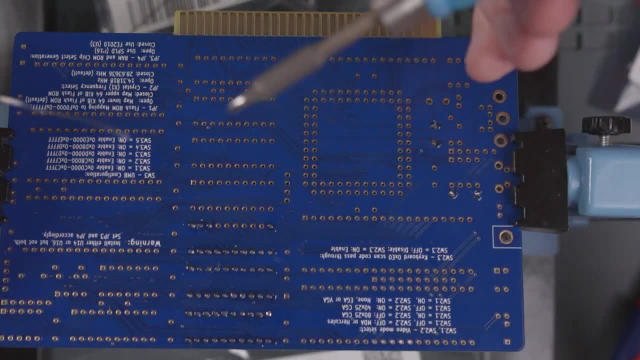 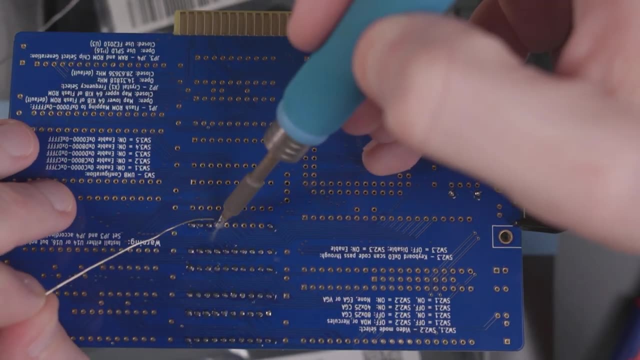 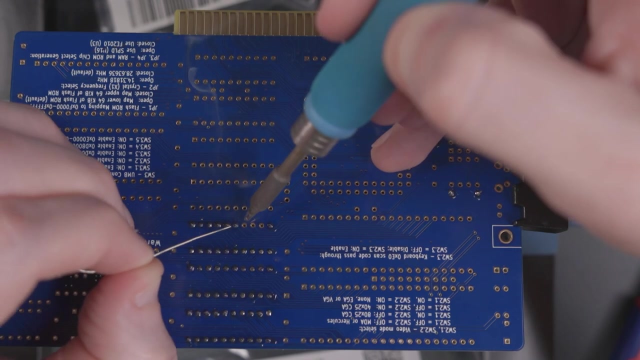 largely inaccessible and expensive, which is, you know, big old computers that are in various states of repair. uh to you know, uh, a unified project that kind of many people can use And have like a baseline configuration that they can just assemble. 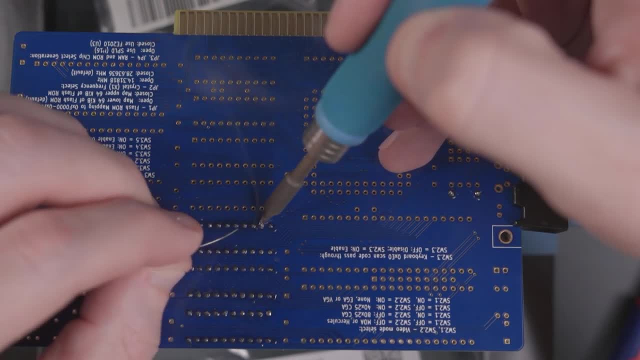 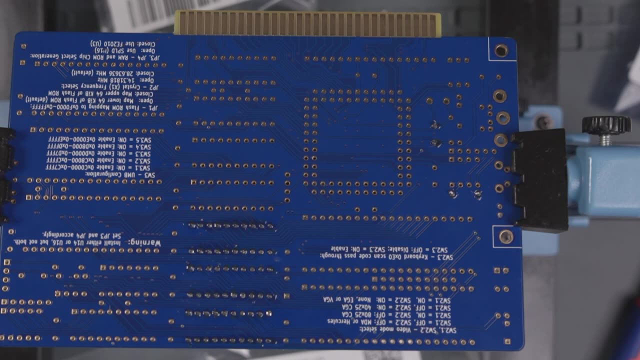 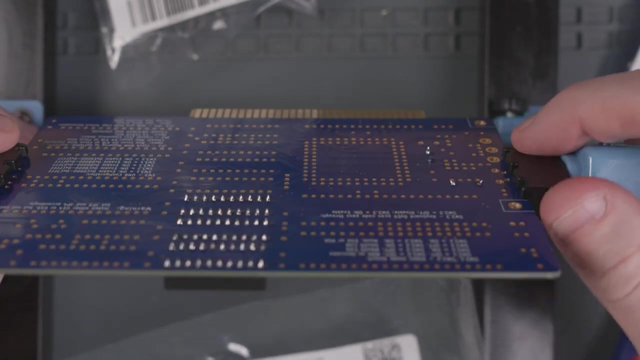 So that's kind of what I'm hoping: that this project will be. like a cool IBM PC class computer, It's a super tough thing to troubleshoot, especially with those- uh, those QFN parts. I mean, on paper they don't seem hard to to solder, which is why I was so gung ho about. 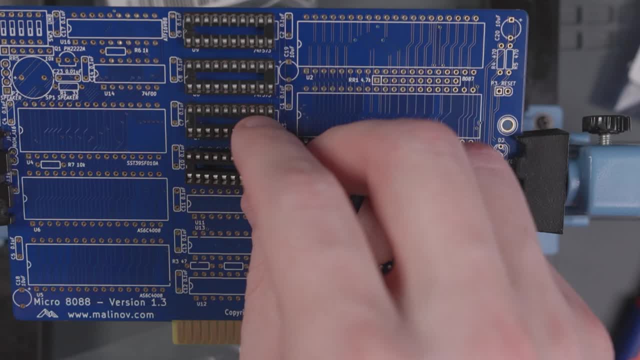 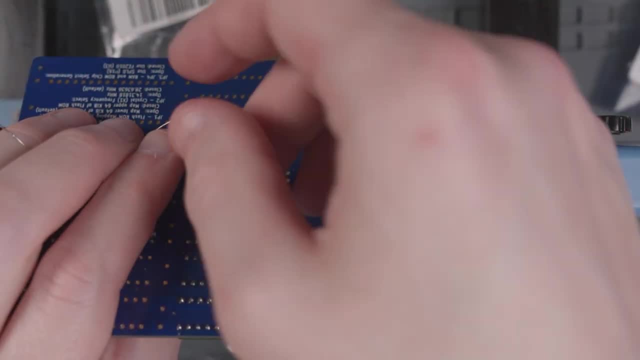 it, It's hard, It's not, it's not simple, Or, you know, there might be some, some amount of luck. uh, because I've seen a whole bunch of videos where people solder them on and then they don't like um test them in the. 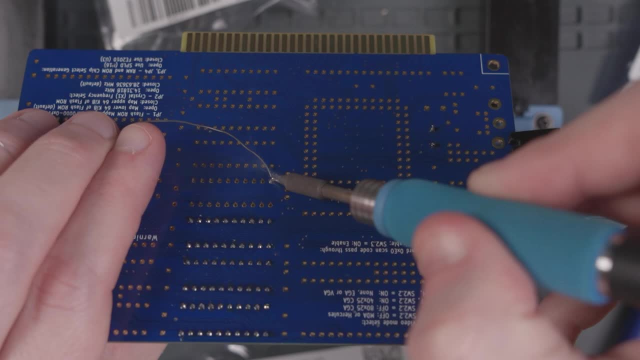 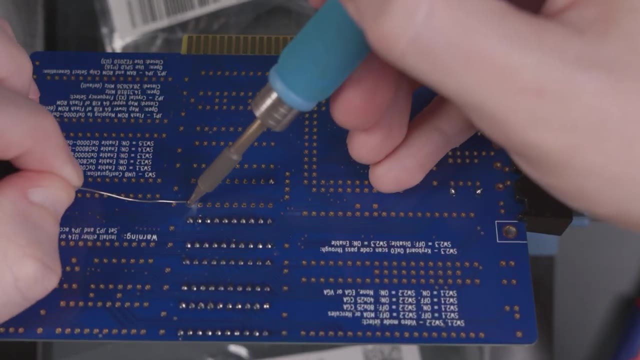 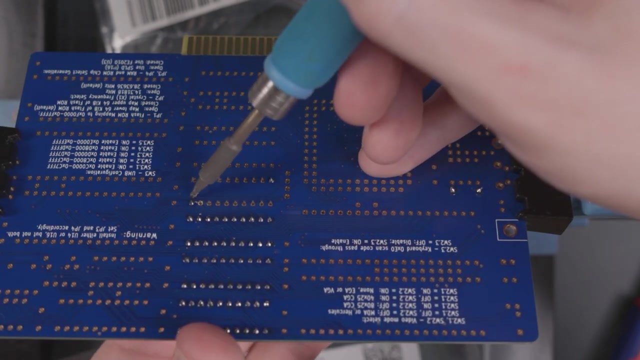 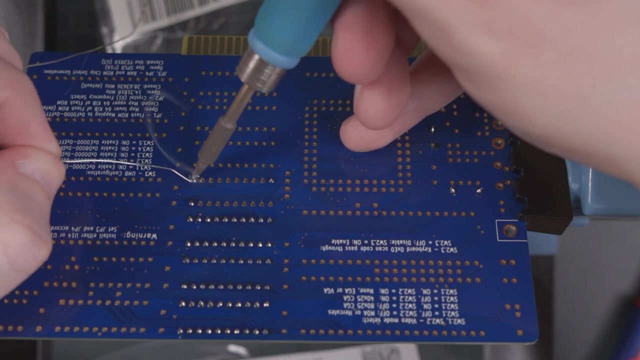 video Like. so I'm not sure people actually. you know I'm sure somebody out there is soldering them. well, but it's not as straightforward as it seems. But now I've got a hot plate, so that probably would have helped me before. 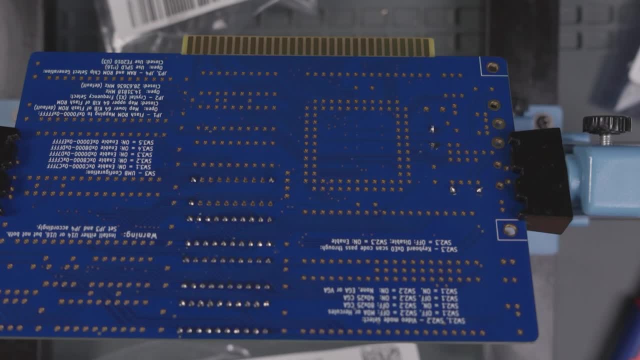 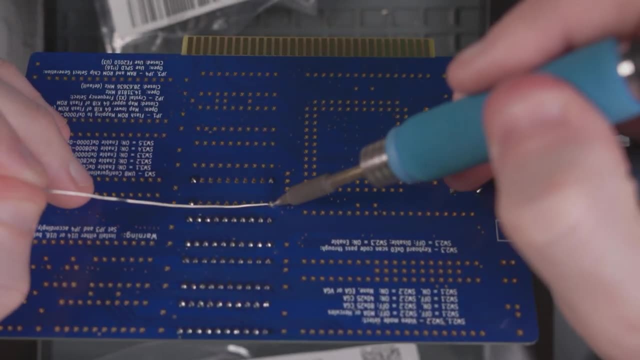 I did watch the uh Adrian's mail call today too, about the picogus too. It got me excited. I didn't realize that the the sound blaster functionality was out. now I've heard I knew that it was coming in a beta or it was in beta. 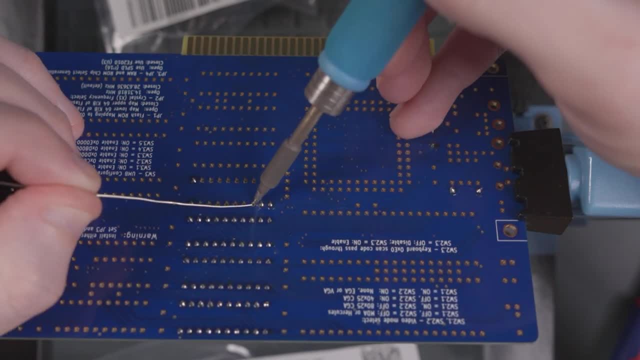 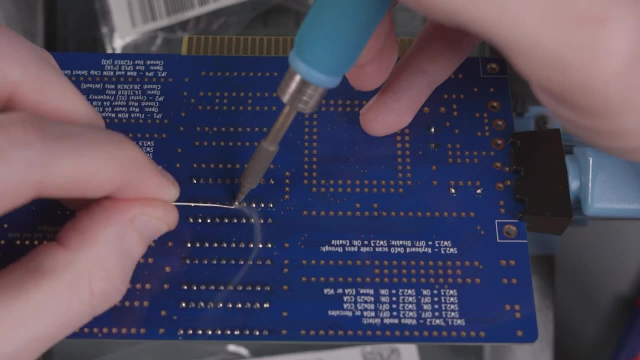 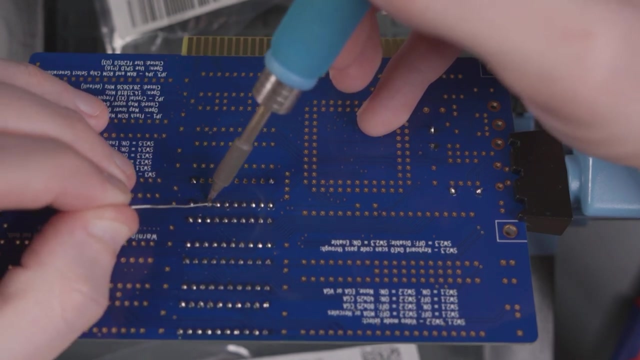 So that'd be very exciting. I don't know if an IBM AT or, uh, yeah, XT, I mean- can really take advantage of any of the sound, uh, sound blaster functionality, But I think it's cool because what doesn't sound blaster also have ad lib, kind of as. 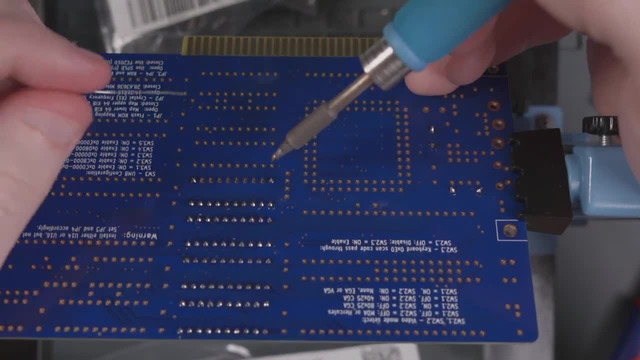 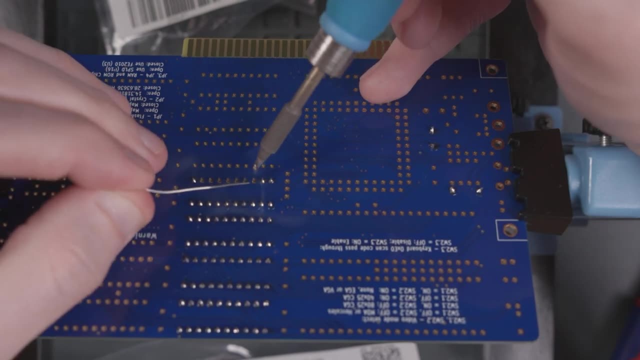 a backup. So that'd be a cool double. um, it did. it did have ad lib uh emulation before, but I mean it's cool. It's nice to be able to have it set in sound blaster mode and then at you kind of get ad. 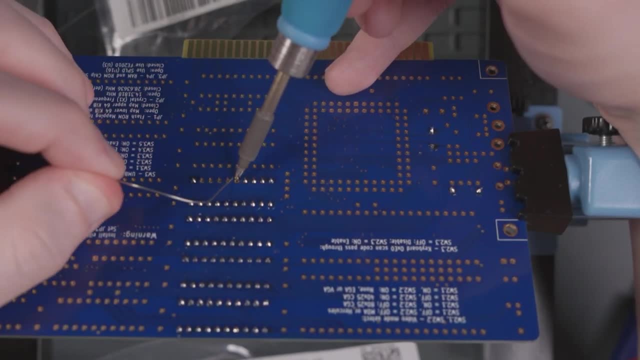 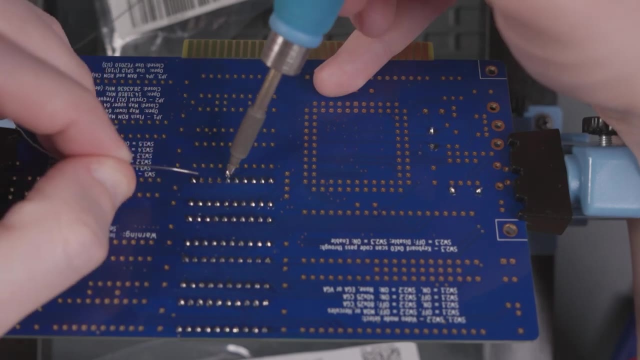 lib without having to change the config, which is kind of cool. So that that is like a now it's like a must have card, assuming it works well. You know, I saw Adrian's works. you know, seem to work well. 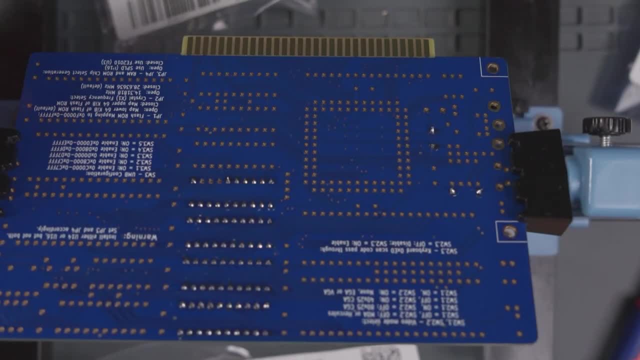 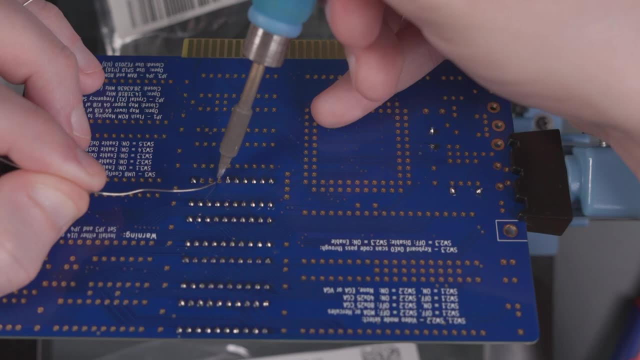 He had it running with some sound- um, not MIDI, but some kind of thing- And uh, it sounded pretty good. So now it's like a that's like a must have if you're getting into to, I mean even. 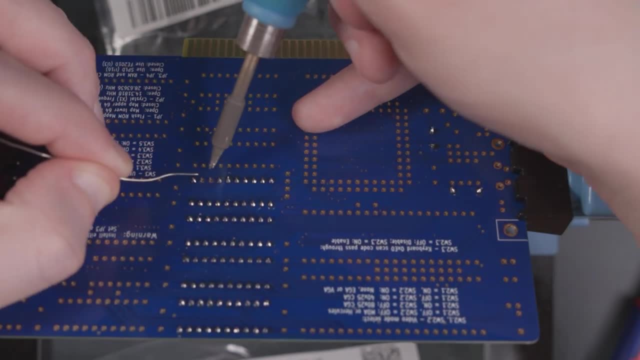 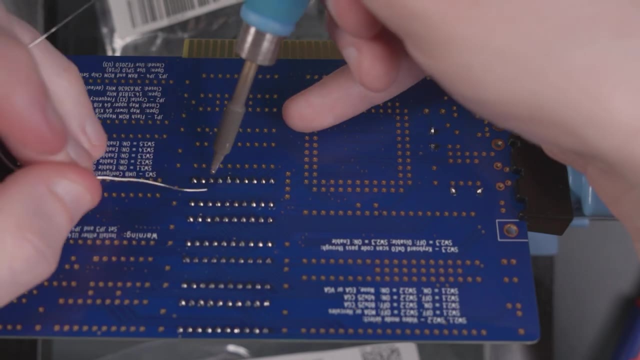 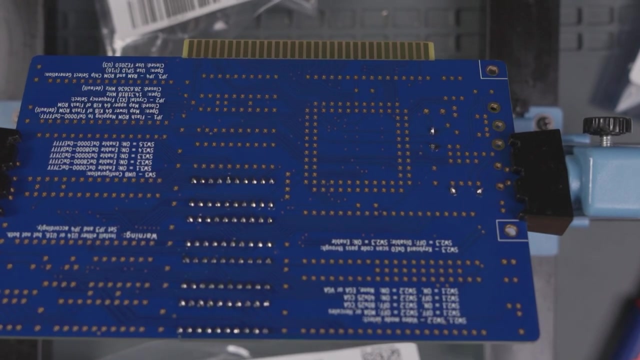 if you're, even if you've got one already like uh I I still personally liked the sound of what is it called Like wavetable kind of sounds, Cause that was my first computer, had a- um, my first computer, that gateway machine had. 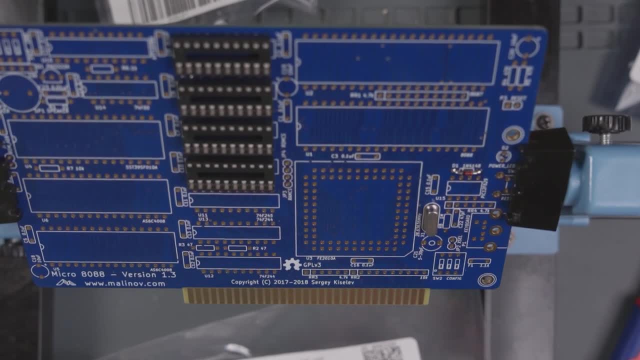 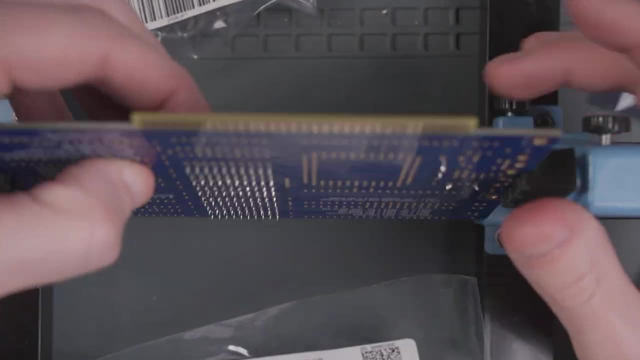 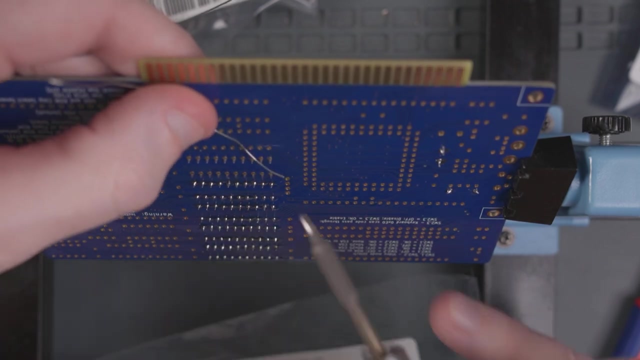 a uh soundscape card which is kind of like a sound blaster clone, but it had the wavetable support, So it had some built in wave sounds and that's how I remember doom sounding, Not not like a sound blaster. 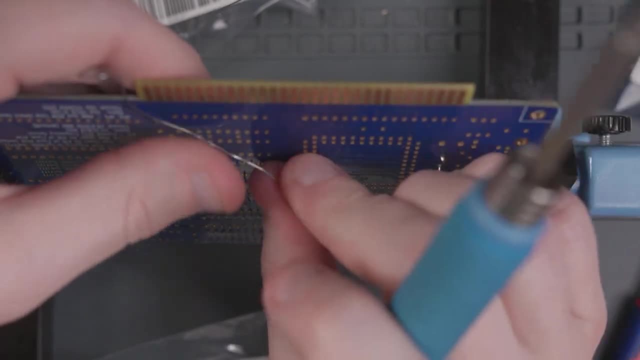 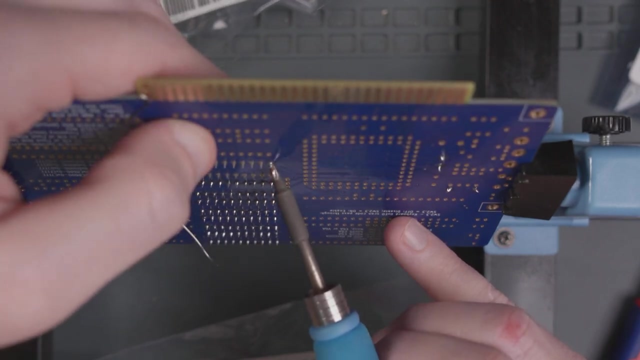 So I imagine a lot of people probably when you first played doom you might've played it on a sound blaster, but I played it when I put first played it was with a wavetable setup, So it sounds a lot better in my opinion, but probably more authentic for it to be a sound. 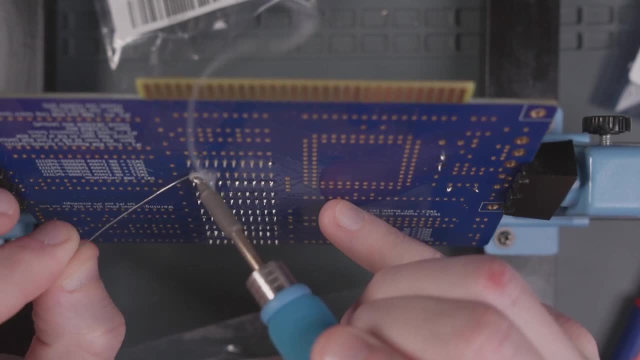 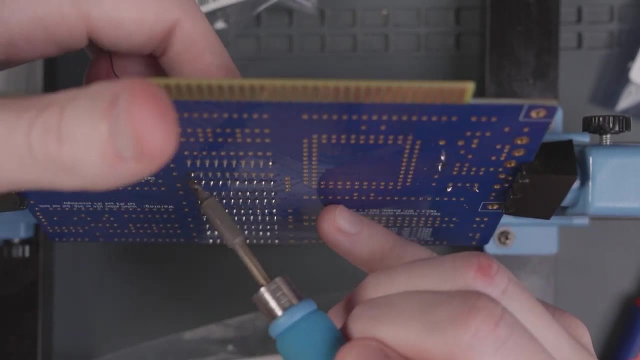 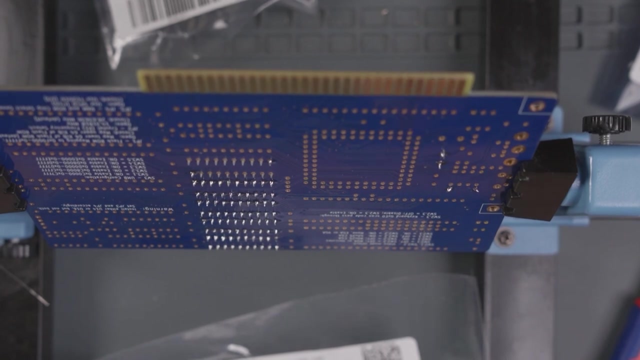 blaster for that Good old doom Doom music sound blaster includes ad lib and sonic soundscape. Those sounded really good. Yeah, I don't know why, Like they were like an OEM brand, but I guess gateway really knew what the hell they were. 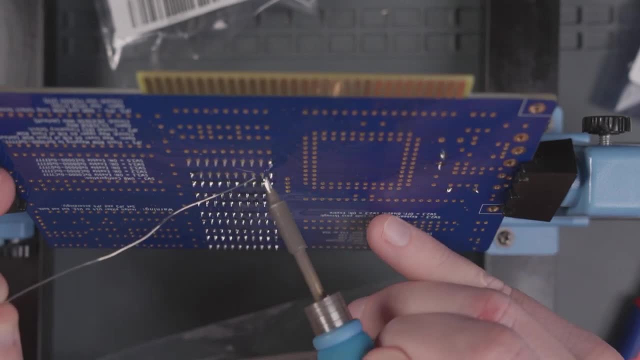 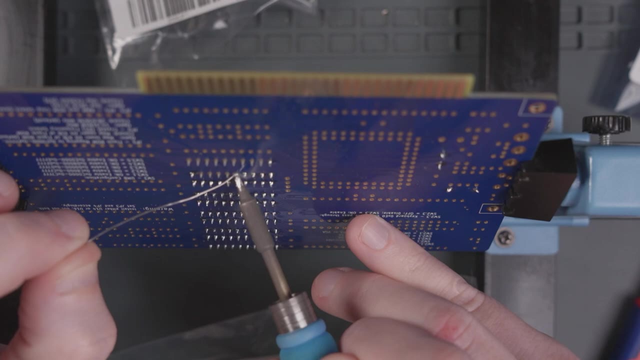 doing back then? Cause those, those machines, you know they sold them for a pretty long time- Like there's a lot of different Pentium, you know those Pentium towers- Uh, my dad's that even had a Pentium pro which was basically the beginnings of Pentium. 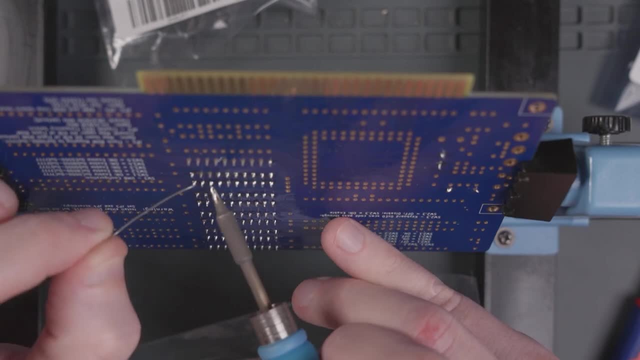 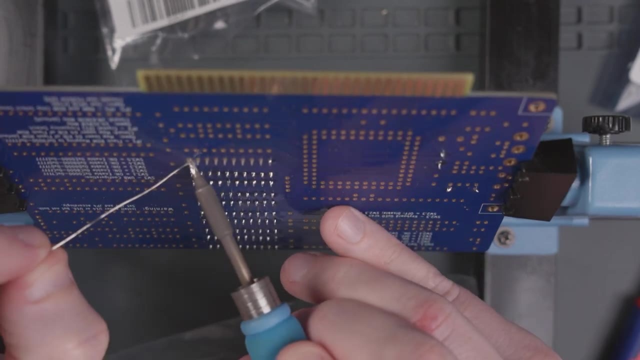 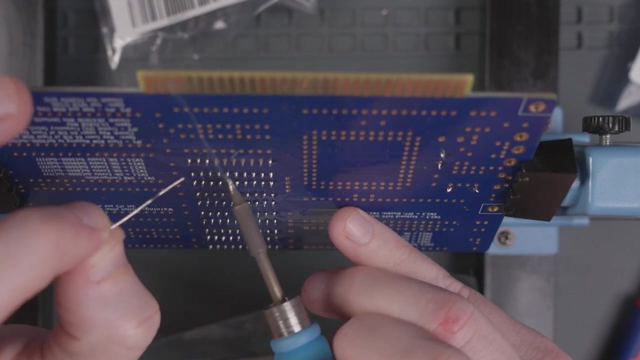 two, Pentium pro and Pentium two, kind of share some architecture uh, which differs from the Pentium one. but um, yeah, so it was a pretty. it was a 200 megahertz machine at the time, where you know Pentiums could be a hundred, one 33,, one 66.. 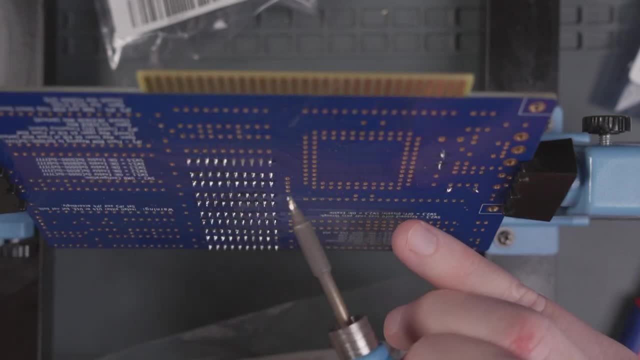 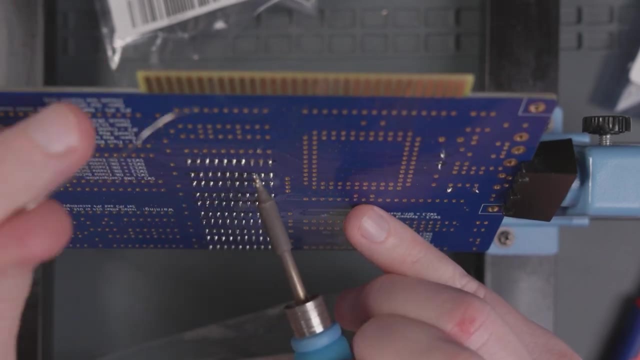 So 200 is is kind of on the high side of Pentiums, Uh. so so things like playing doom was a breeze. I mean, I had never really played quake at the time, but um, I it would probably be. 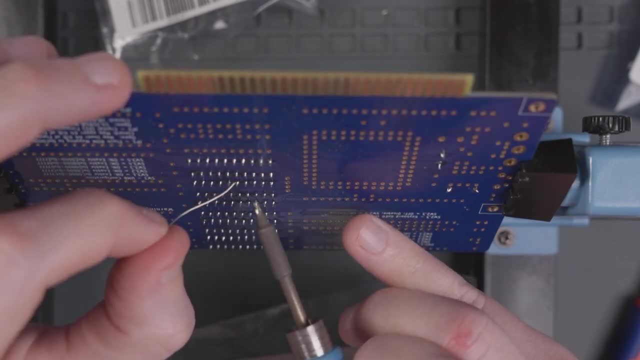 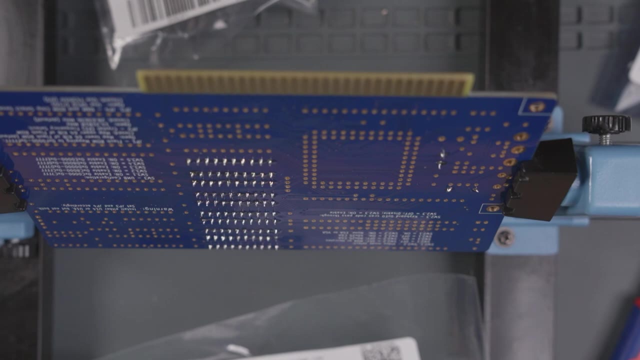 limited by the. I had it had a what, actually I'm not sure what, the one, my specific one that my dad had, but I had the. uh, what is it called? Uh, shoot, I can't. I can't remember the graphics card that I had. 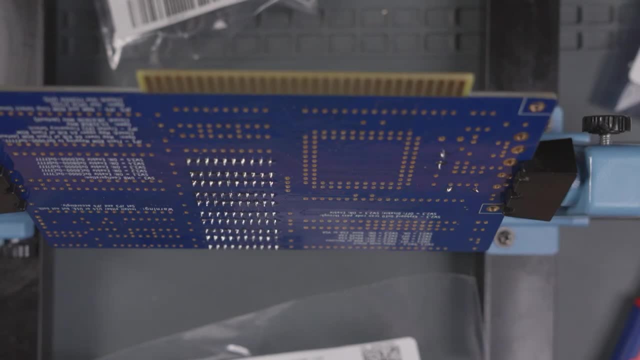 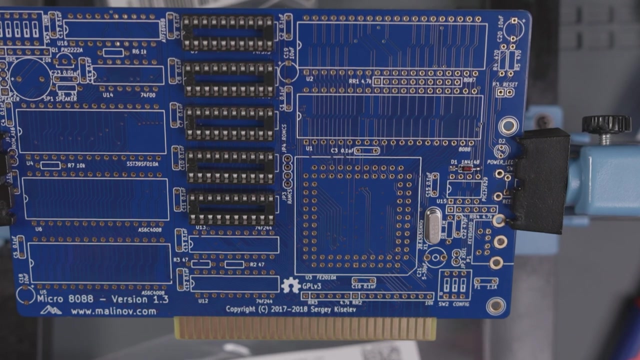 It was that name brand that I had. It was the same brand that I don't, that I never really had heard of before. So the M, I think Mm Matrox, millennium, That's what I'm trying to think of. 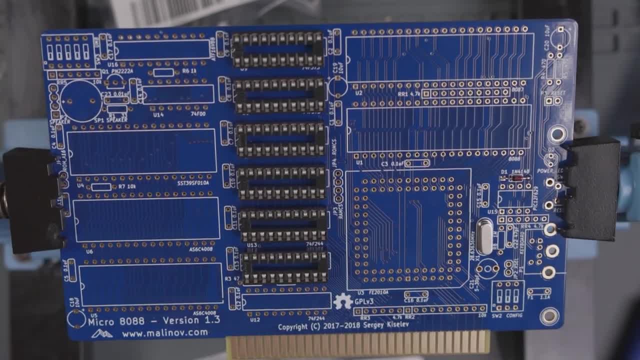 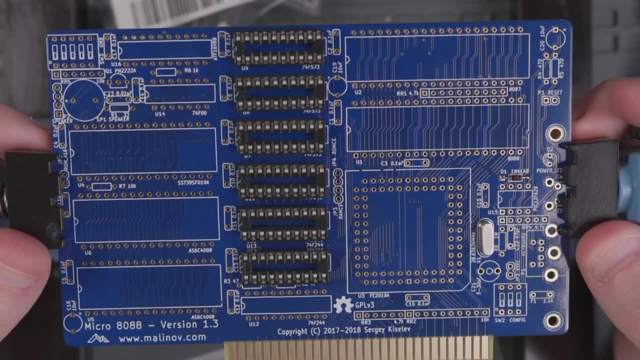 Well, this is pretty much what it's going to be for the rest of the stream. Um, but I think I will do. I'll populate all everything between now and probably Sunday. I, if I have time, maybe we'll do like the the the tail end of it. 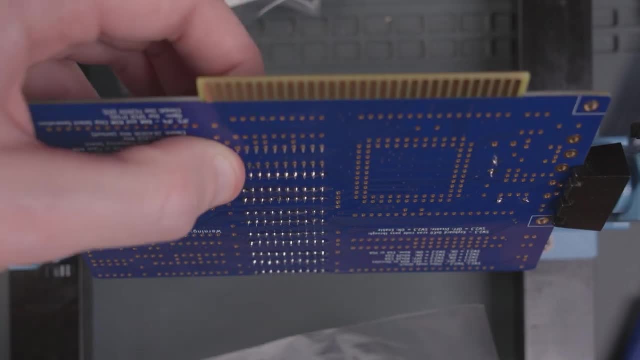 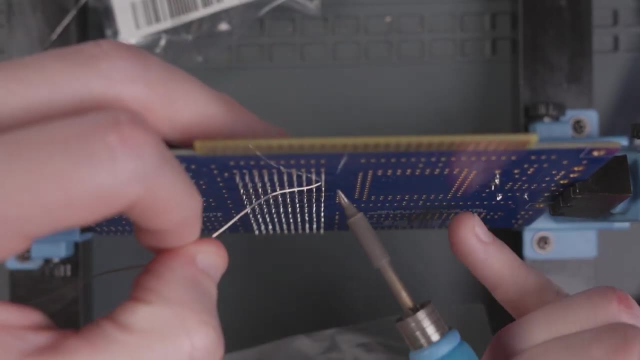 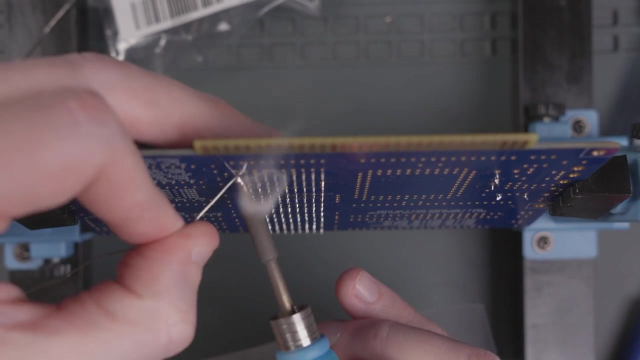 Cause I think people are probably more interested in the scaler stuff. but I I gotta get this project done And, like I said, I really hope that this project would be a cool way for people to be, you know, learn more about how to solder um and then have a super cool working IBM. uh. 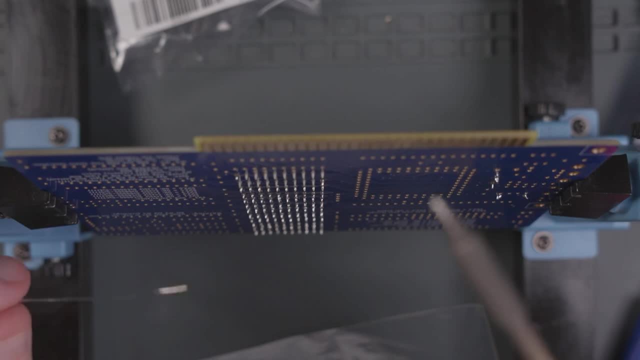 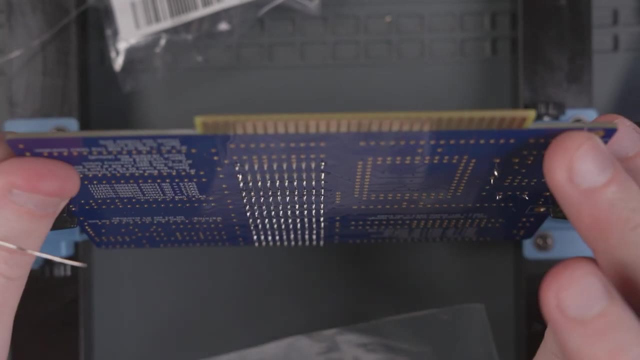 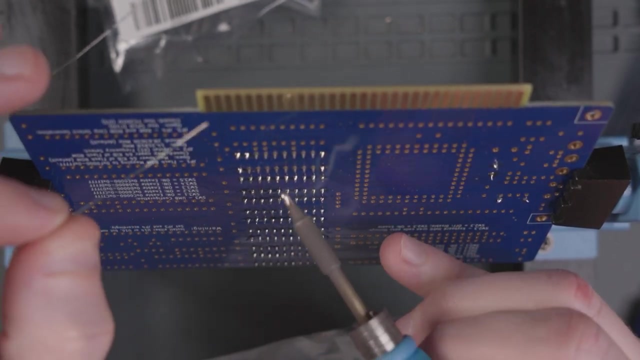 PC That's, it doesn't take up a lot of space. So that's kind of a cool um double whammy in my opinion. So, uh, I'll be setting it all up and then the following stream, or I'll be, I'll be. 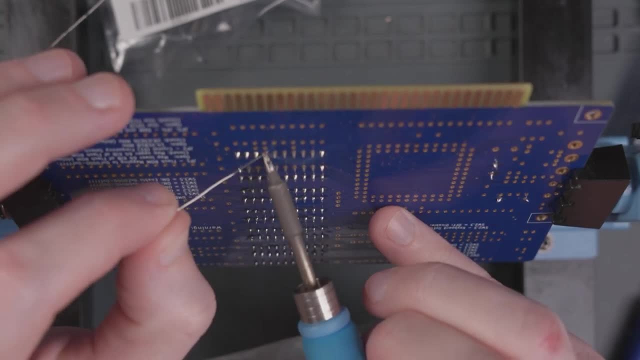 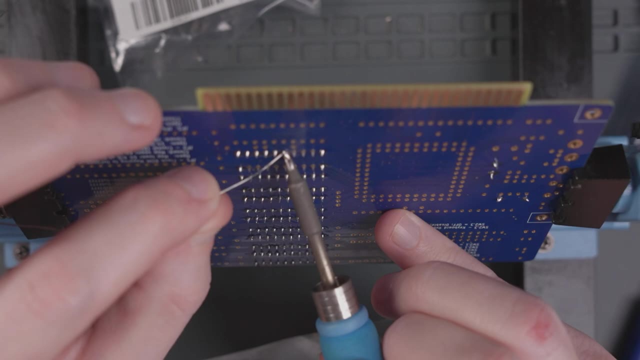 populating the boards, probably before the next stream. Then the next stream will be trying to turn it on for the first time. So I have a. I have a ATX power supply. I have. I guess we could just use floppy for the boot. 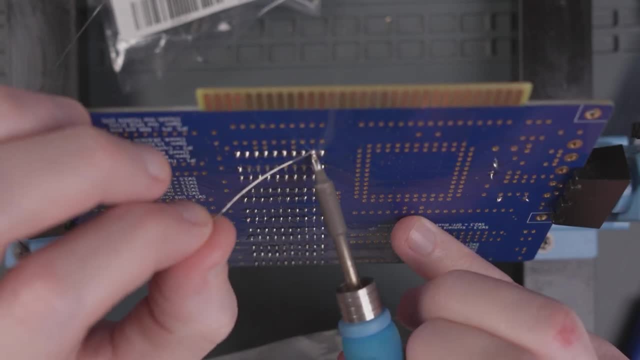 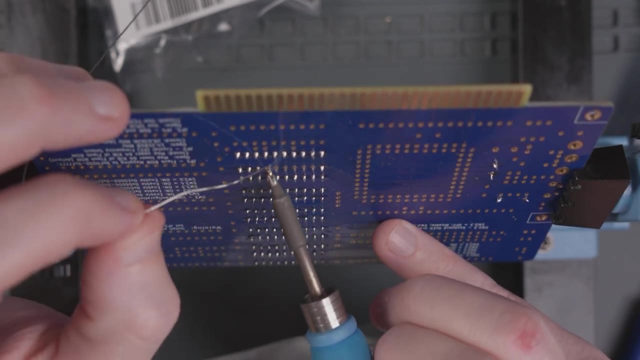 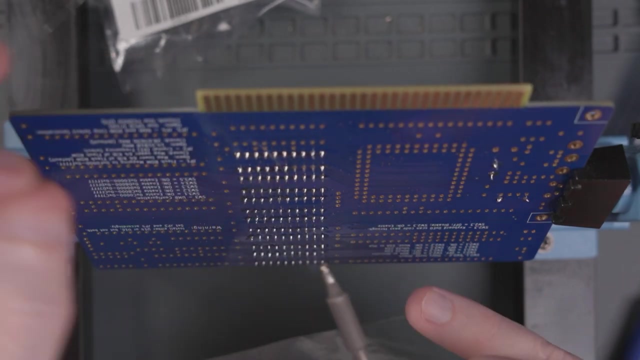 Just, You don't need it. We don't need a, uh, a hard drive in the beginning, just to test that it works, And, uh, a VGA graphics card. Um, eventually we will be building the, the graphics card for this bill, for this project. 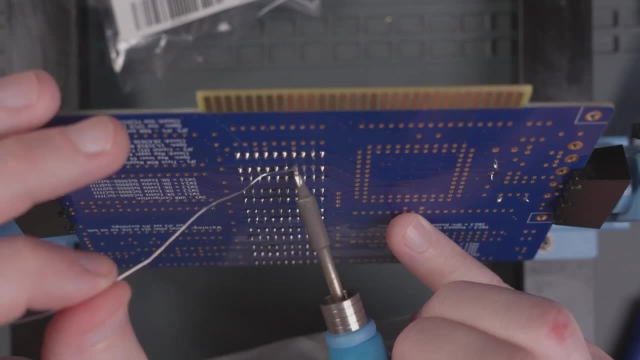 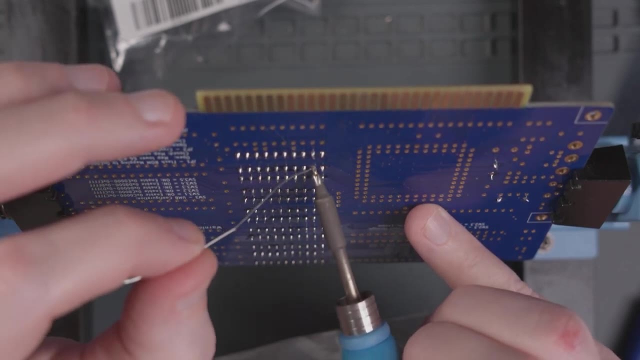 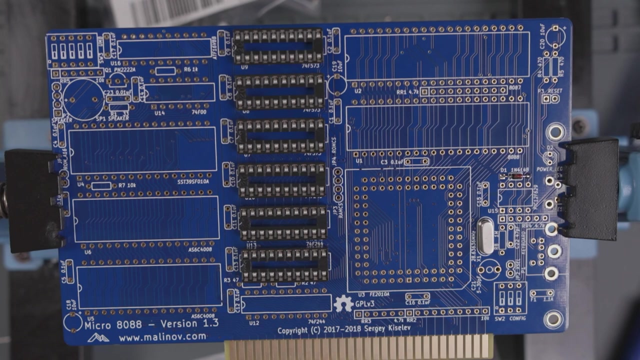 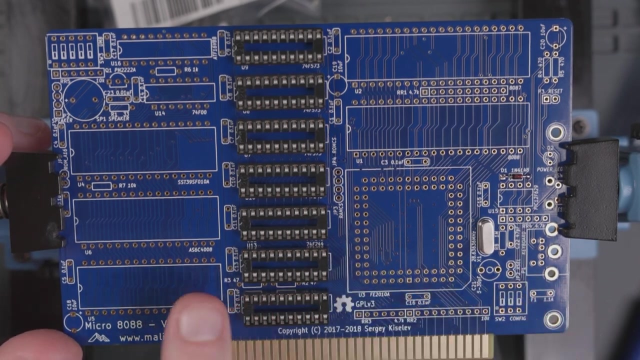 but I have extra VGA ISA cards that we can use just to test it, And we can even throw in Ian's uh pico gas So we can have some audio. All right, Two more of these bad boys Making sure that the notch is notchy. 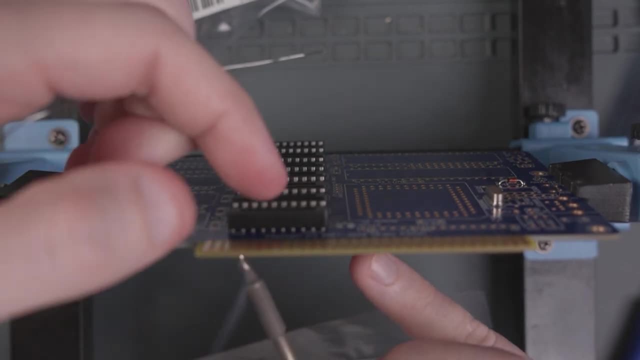 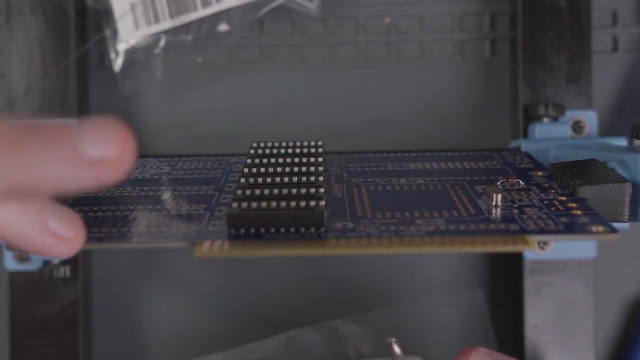 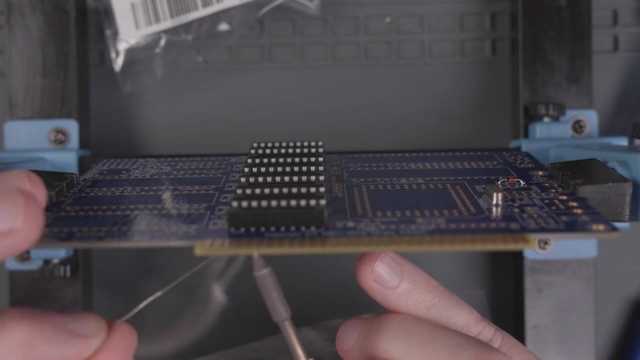 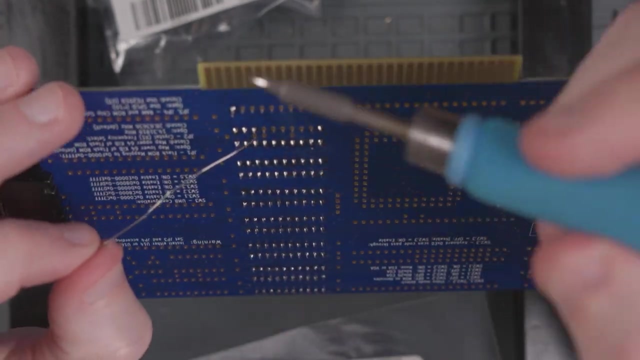 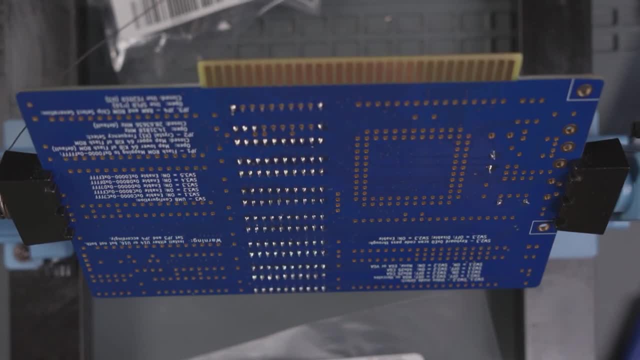 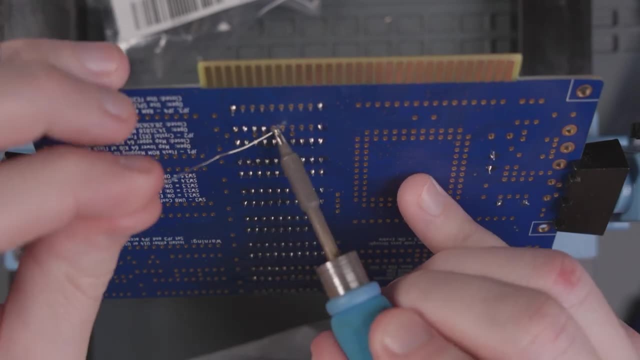 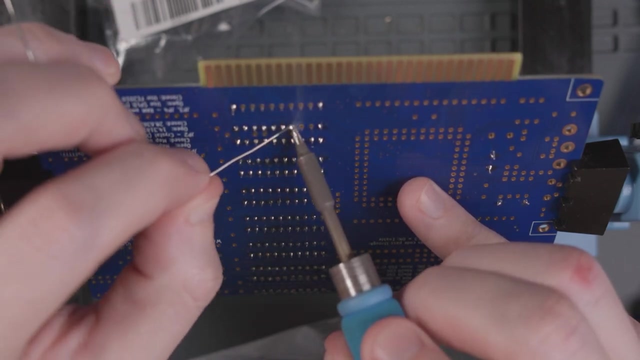 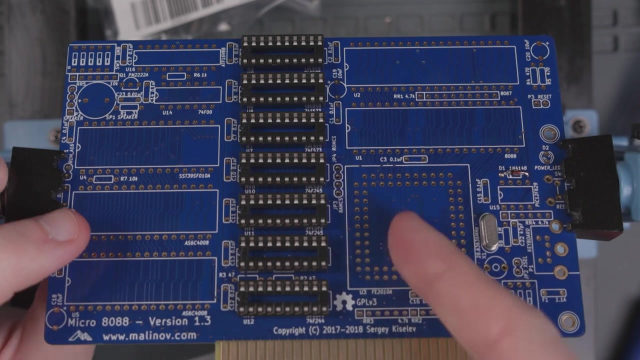 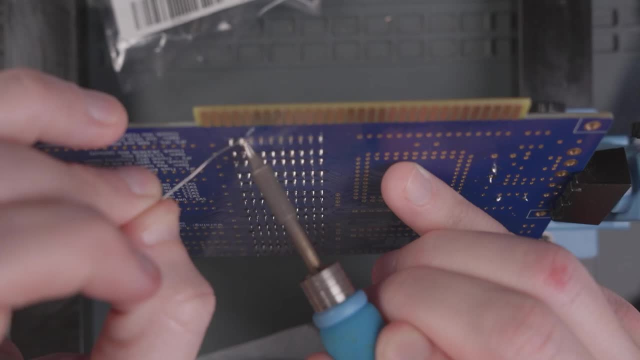 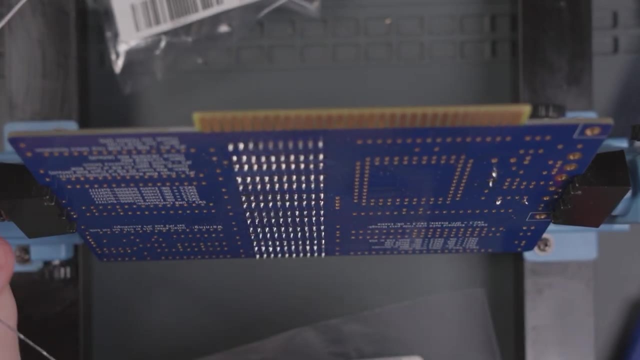 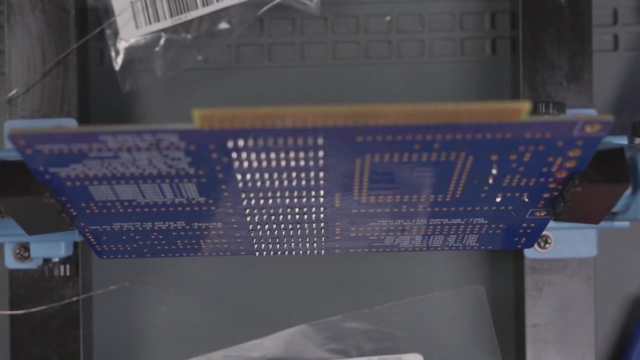 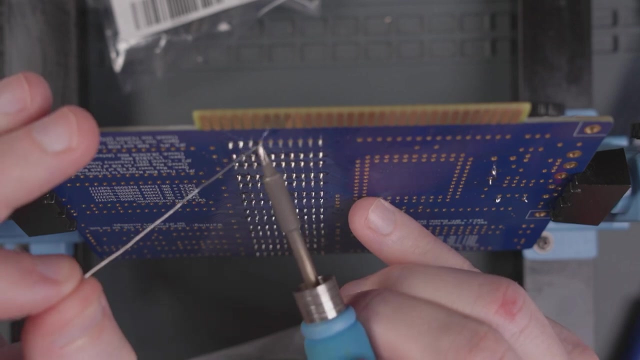 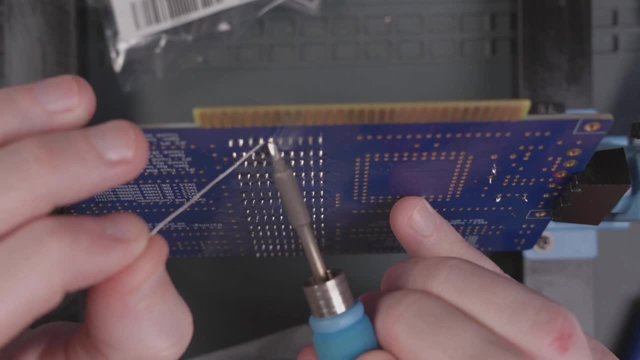 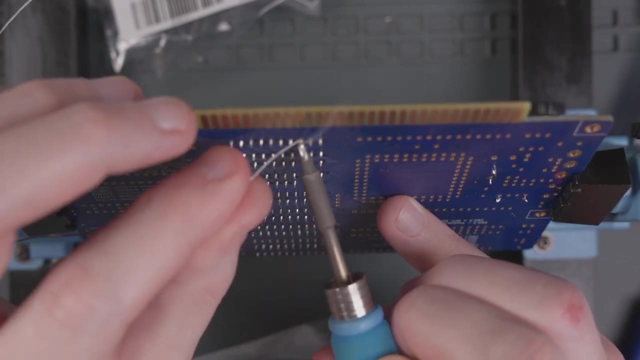 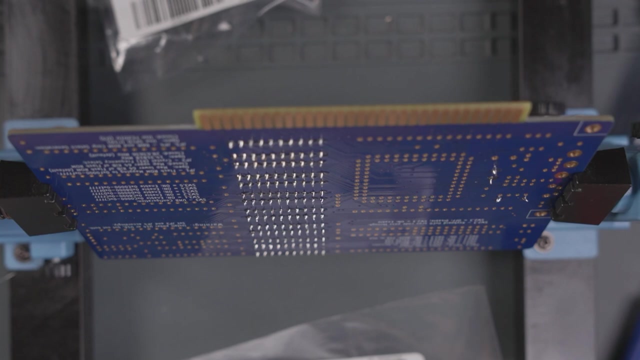 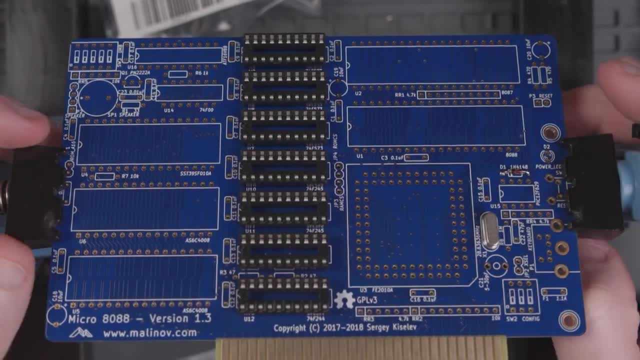 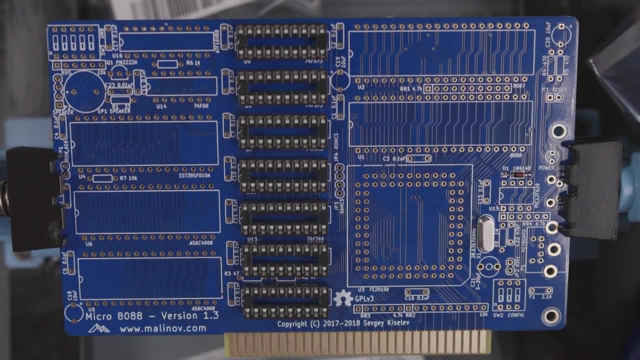 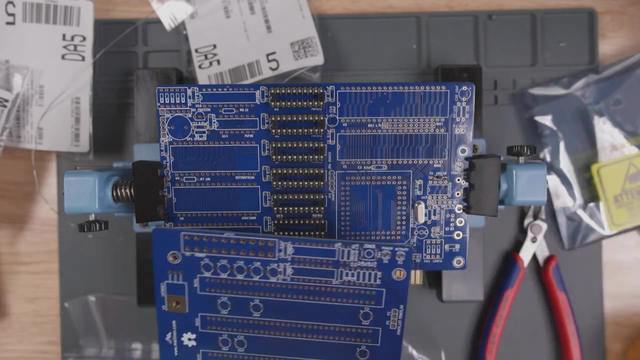 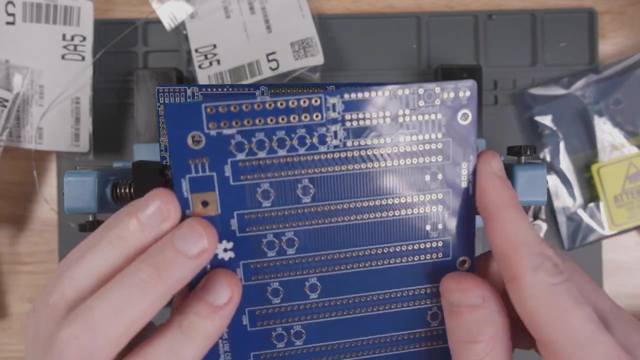 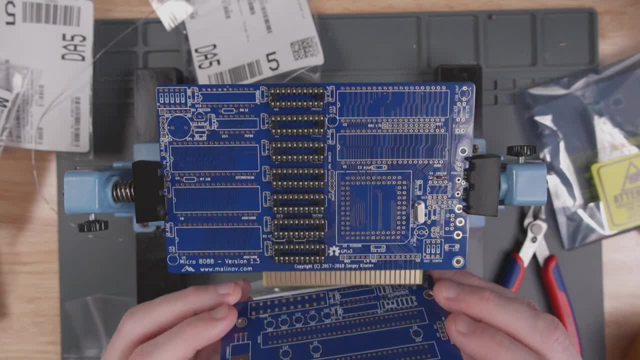 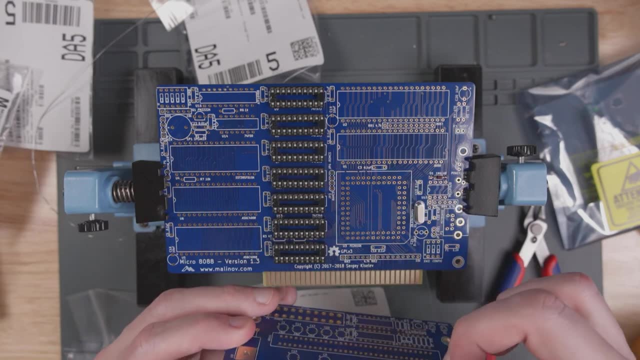 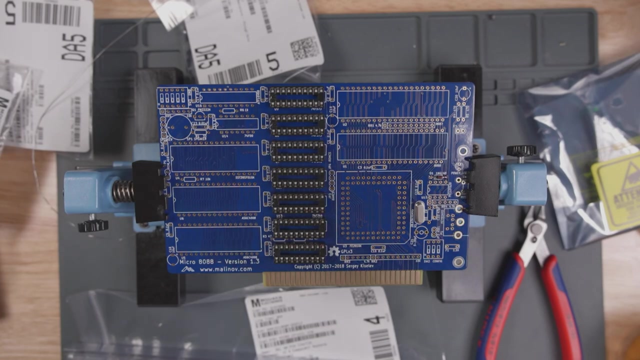 will eventually have a bunch of isa slots and that is where all the the piece- the cpu one, the sound card one, the xtie one- will go on one uh, different slots and then, uh, so the cpu one is kind of on a daughter board, whereas the backplane is really just nothing, just the sockets and the 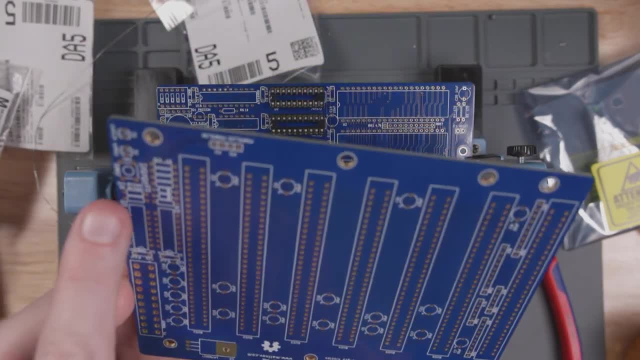 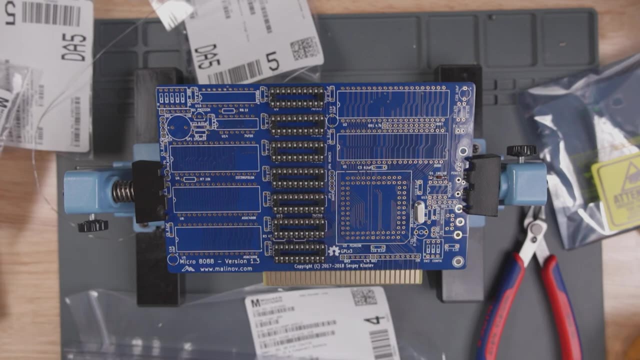 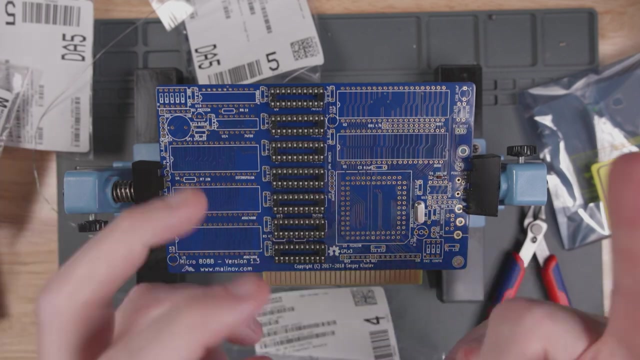 voltage regulator and the power. so, and uh, didn't i say a p, oh, it's on the uh, the keyboard, the ps2 keyboard is on this thing. so it's kind of like you're stuck, you're not stuck. i mean, it's a cool, it's a fascinating project, so it's not like you're you're stuck, uh, it's just a. 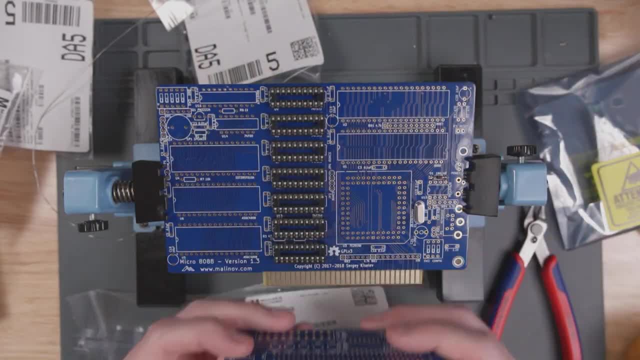 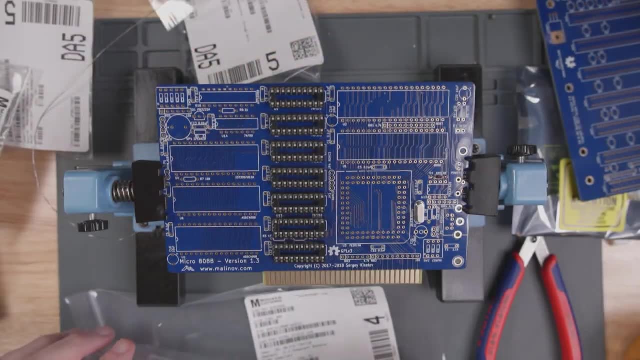 very. it's like a very specialized kind of form factor that is made for this matching um case that the designer made 3d printed. i mean, all right, last you, last one of these things, then we can get this out of here. oh, this is a nice bag, though. okay, so this. all this one goes on u16. 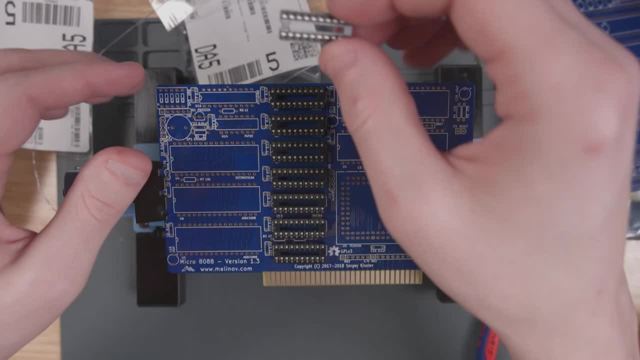 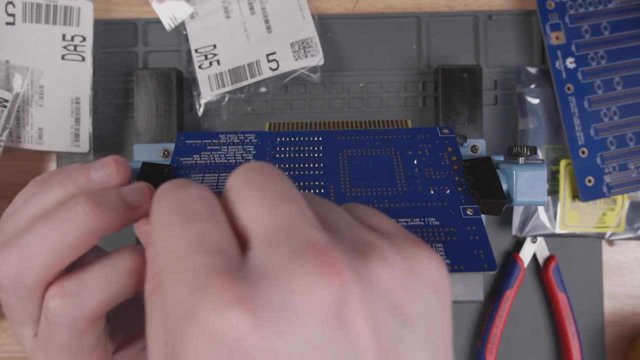 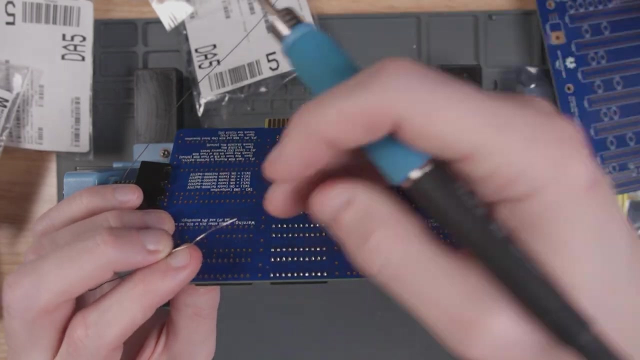 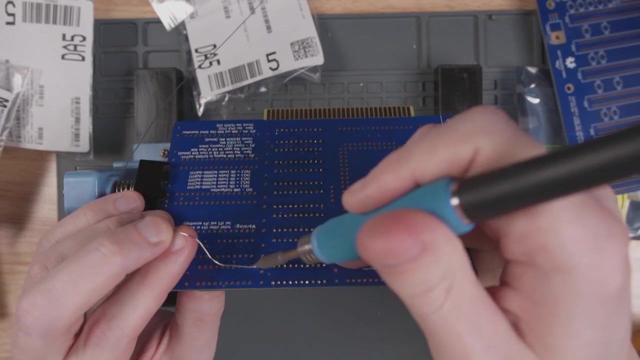 okay, they have some good deals at my center. they sure do. if you don't? if you, there is a website. i want everyone to know that about it, even if you- i'm sure a lot of you have known. but slickdealsnet is itnet, slickdealsnet. 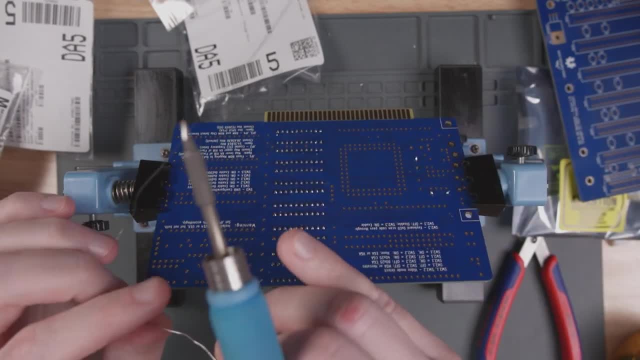 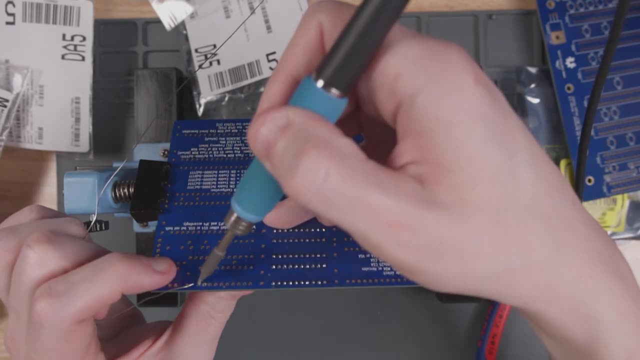 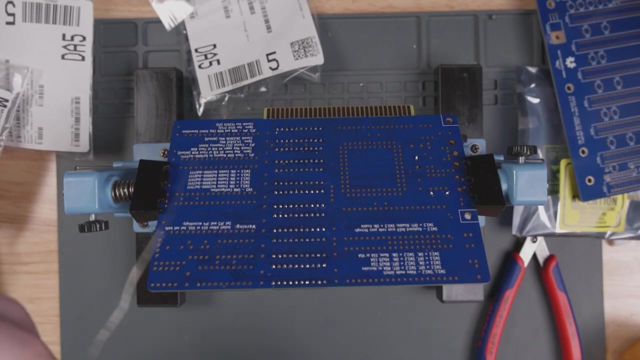 uh, probably where the majority of my, um, my discretional spending goes just finding cool stuff on on slick deals, um. so it's kind of like a- it's a forum, i believe, but they the the home page of the site just like aggregates and shows you really good deals. so it's kind of like a it's a. 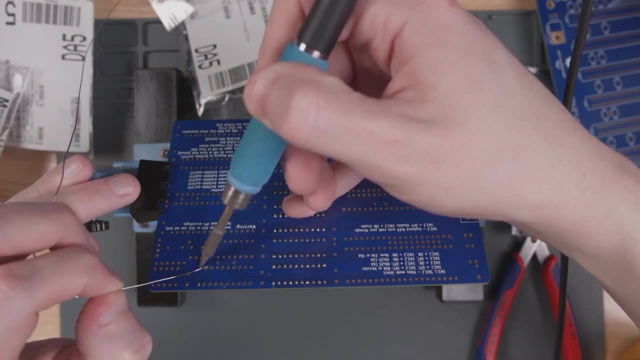 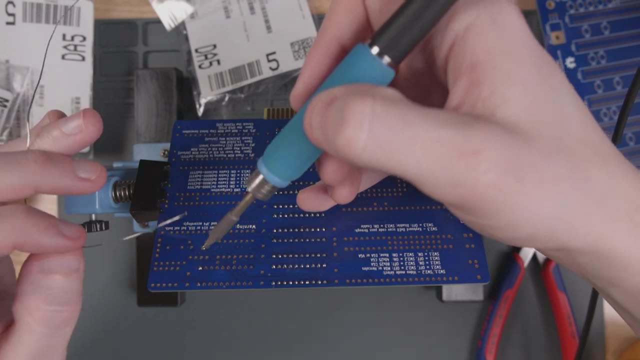 forum, i believe, but they the the home page of the site just like aggregates and shows you really good deals. um, most of its, some of its tech, but some of it is like, hey, you can get granola bars on sale right now. so it's just like crazy stuff. and um, i see a lot of times people list micro center in-person deals. 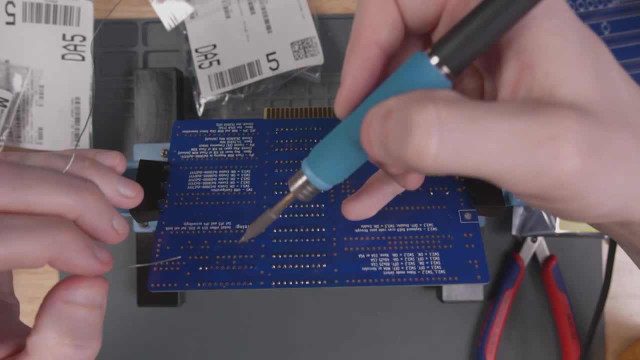 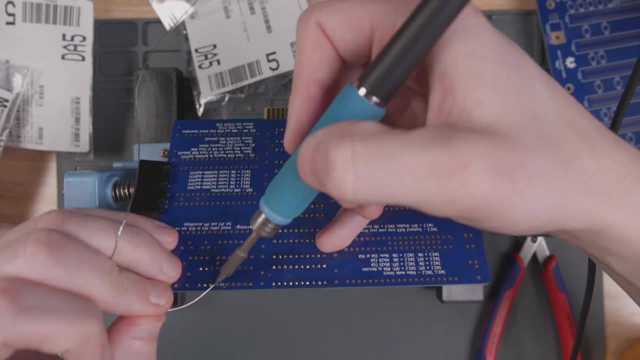 on slick deals so that people know they can go to the store and get a deal, and that makes me jealous every single time. i see like a really good combo, because usually they'll do like cpu motherboard and then something else- ram or something like bundle deals- and they're less expensive to. 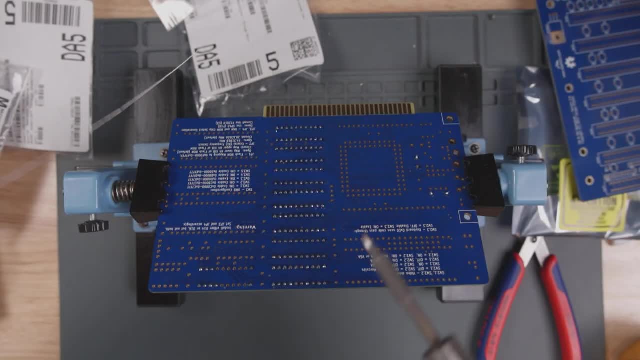 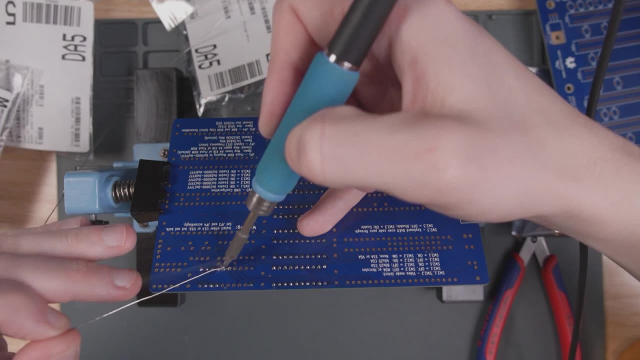 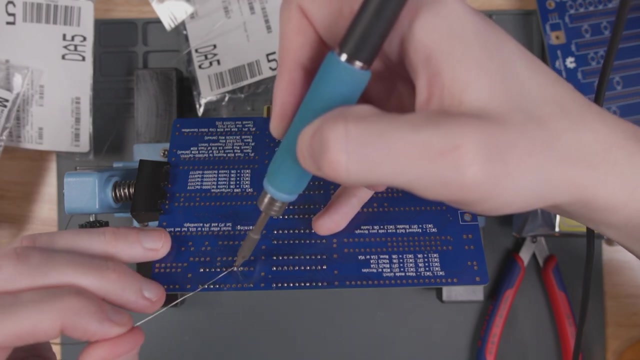 buy all three of the parts than to buy them all individually. so like it's just a cool thing, but you got to go to the store, um, to do it. so yeah, they don't. they don't ship it out online the deals, unfortunately, but with the same. you know, i i make heavy use of amazon refunds, so 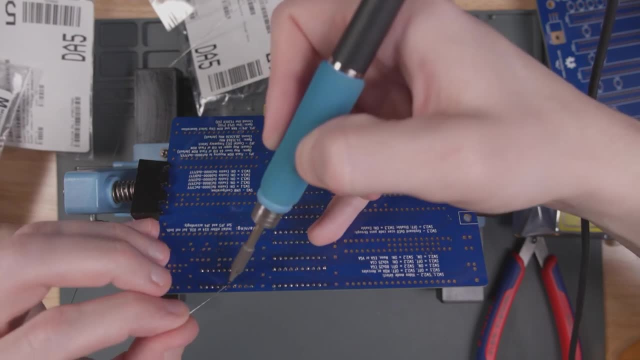 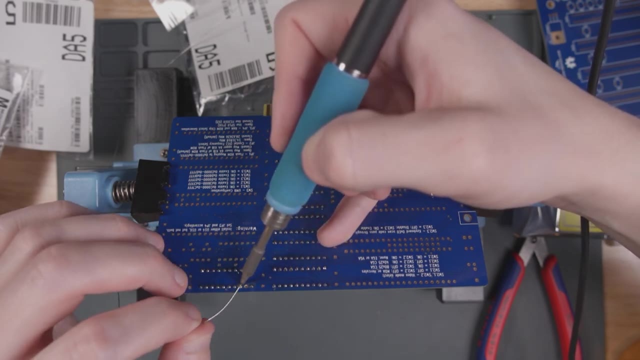 a lot of my stuff tends to be amazon anyways, just so that i have that safety net of like: if i don't like something or and i'm not using it, i don't feel bad about returning it because not like f amazon, because i really like amazon. you know i use amazon a lot in my day-to-day. 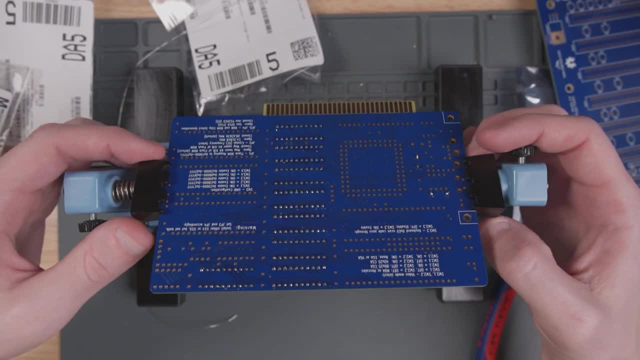 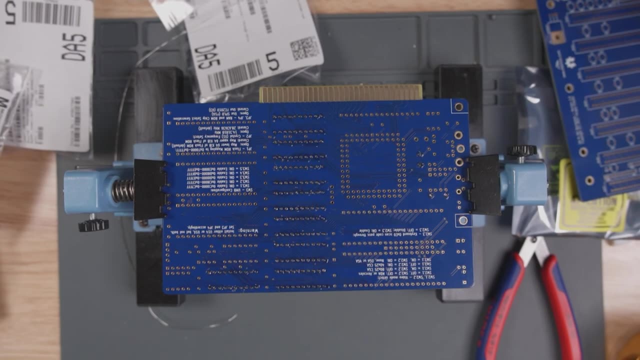 but um, they can handle. the big companies can handle that sort of thing. hundred dollar. end of threes. oh at um. oh, it's slickdealsnet. you have a love hate with slick deals? tell me about your love hate. oh, maybe i should have wrote the. 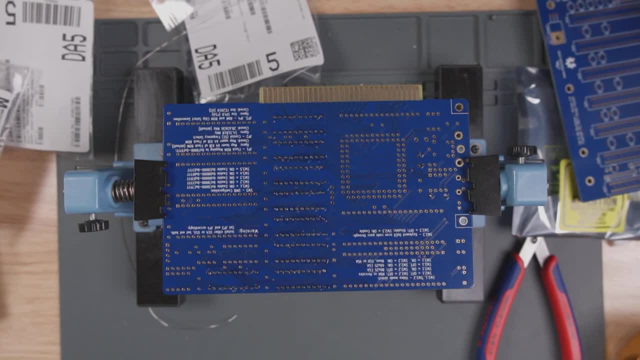 actual url or the actual link. there we go. i gotta get the http. it's coming, it's coming, there we go, there we go. um yeah, you can log in and stuff, but you can use it. you can use it without even having to log in, which is cool. um it, just it just kind of like. 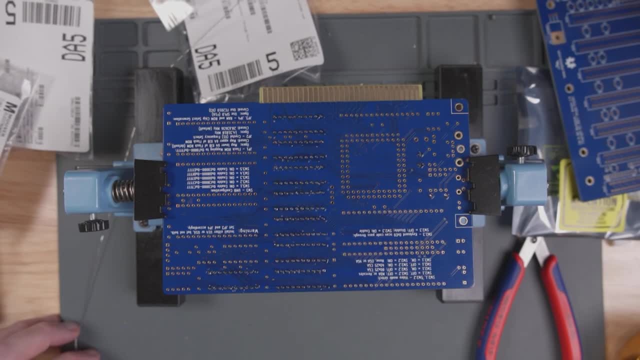 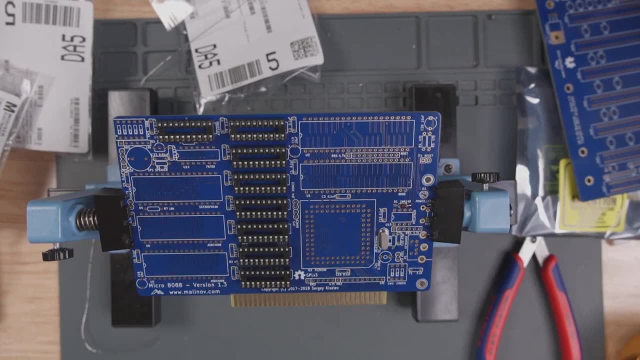 gives you certain deals on your website and you can log in and stuff. but you can use it without your like home page if you sign in and configure it or whatever. uh, but anyways, check it out. i mean, that's where i get. like that'll tell you when there's good like hard drive deals, if you get. 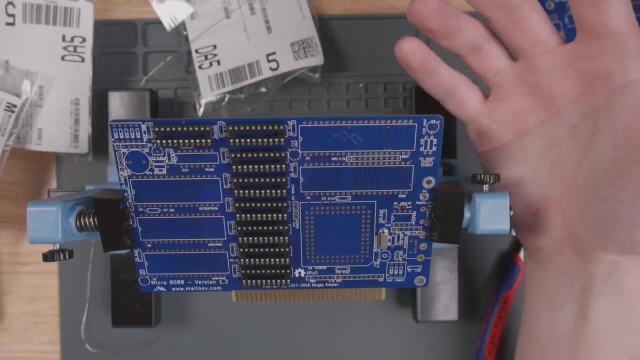 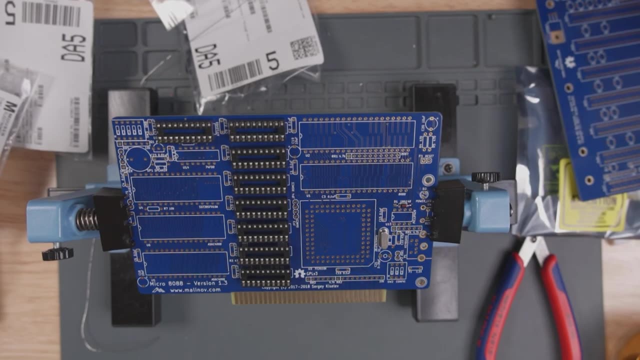 if you want big bulk hard drives and things or just random stuff, like you'll just be browsing it and, like i said, just big box of granola bars that you want or something, and if it's a good enough price, then yeah, but at least it's worth knowing about if you're bored. 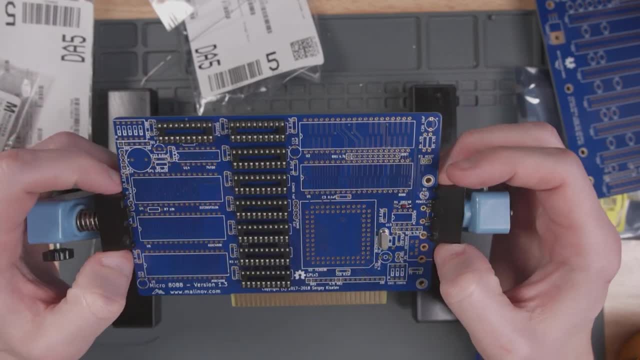 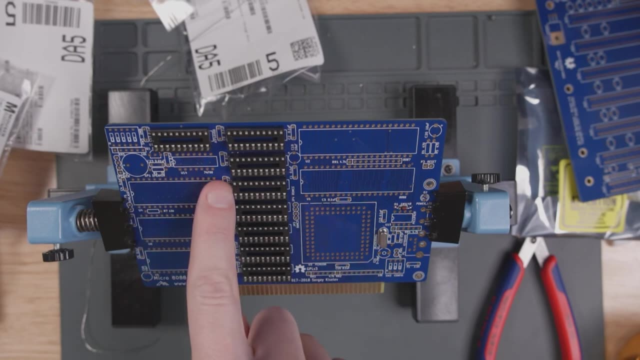 you can just browse it. you buy too much from slick deals. yeah, seriously, all right. um, i kind of want to look. i mean we can, we can dive into some more of these, um, uh, chip things. but i kind of want to do something fun, like maybe. well, i want to see. 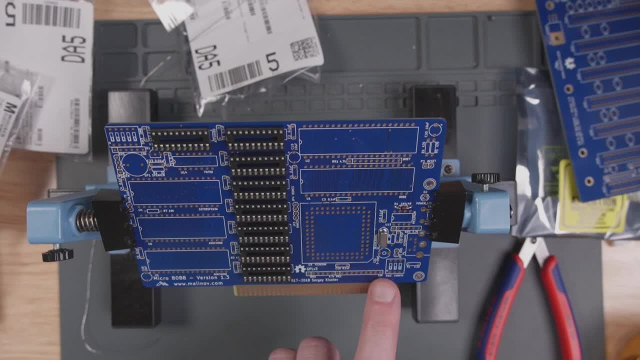 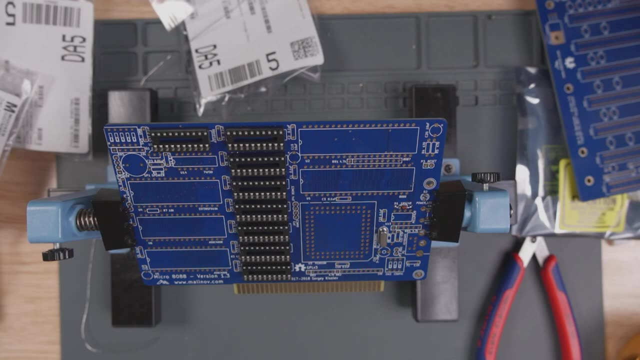 if you can find either this uh socket or one of the dip sockets that i think that would be fun to look at. so i'm going to try to find one of those. you have alerts for things. yeah, i do too. yep, same with ebay. i have ebay alerts for like retro computer parts, like that's kind of the. 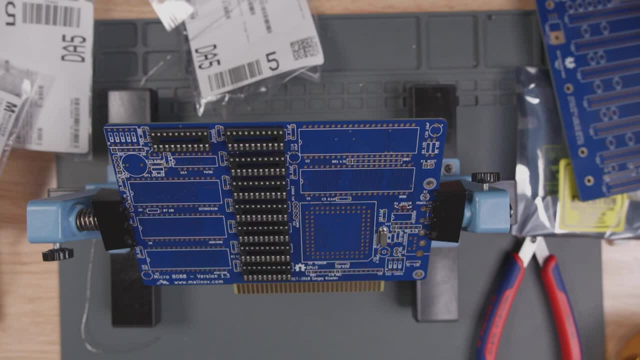 way to go if, you like, you have an idea of a thing that you want to have eventually. um, just put it in now. i know it's dangerous, but, uh, you'll get alerts for it- if it's kind of something that you can't easily find on ebay. 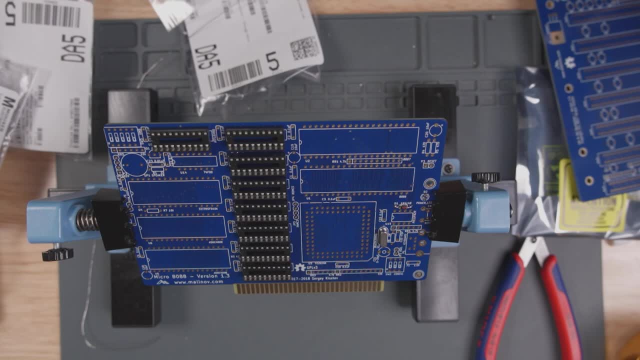 yeah, uh, all right, i hear something rattling. those are screws. that's not rattling. okay, i found a little- oh, never mind, that's a little tiny socket. that's not fun. where's the big plcc? oh, i found the din. i found the- uh, the mouse connector. that's not really. 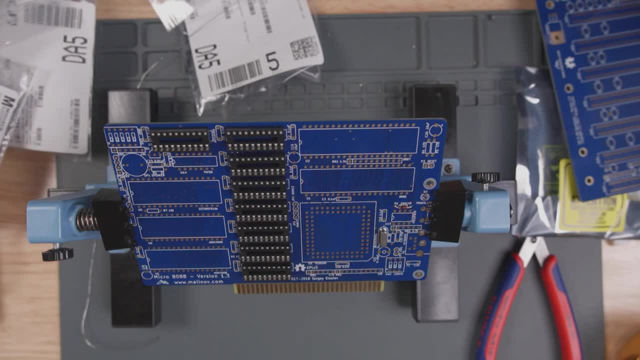 we're not there yet. i'm not affiliate- uh affiliated, by the way, with with slick deals at all, just uh, fyi, i just like to use them for, uh, computer stuff. usually it's computer parts. you get a good deal from you, can you know? it depends. oh, here it is found, the plcc. 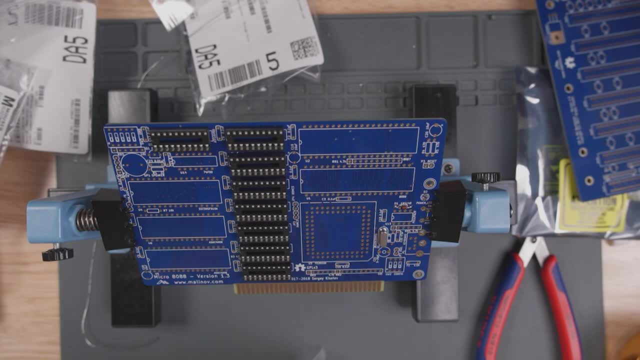 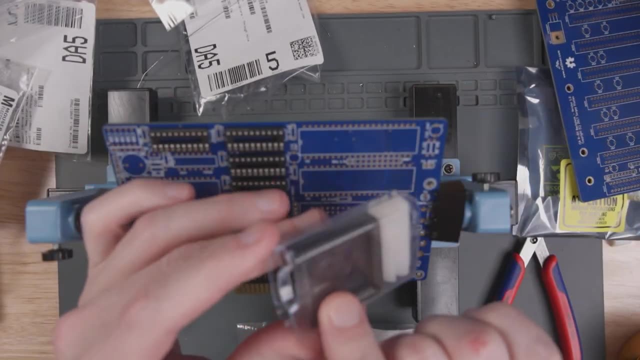 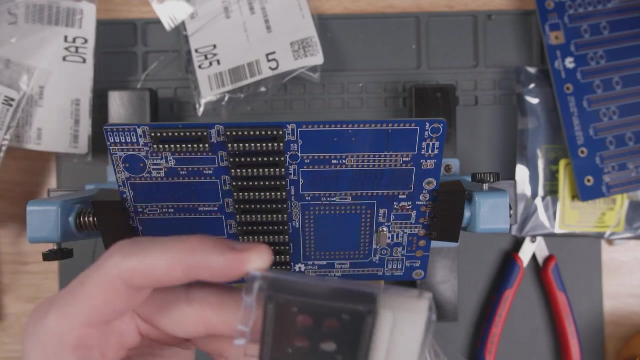 socket, whoa, it comes in a slidey thing. well, this, this is what the if you had a pick and place machine for a a big part like this, like this is. like you know, a pick and place machine can place these on the pcbs when they are soldering them. uh, but they come in these long tubes. they 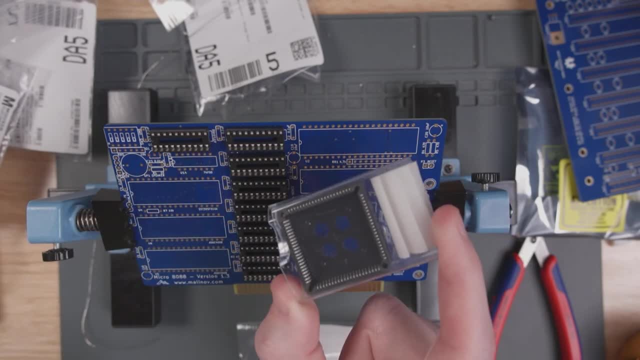 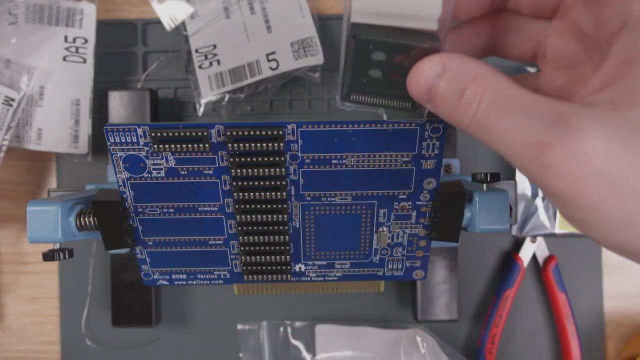 look like this, but a lot you know. obviously this is just a part of it, so i'm gonna cut it. they look like this just a lot longer, and they, they like, load them up like it's like a lot of like, a like, not bullets, but like you know, they're cartridges, that kind of go in there and the stuff. 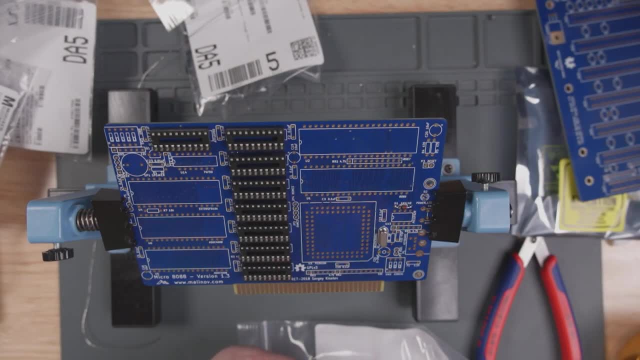 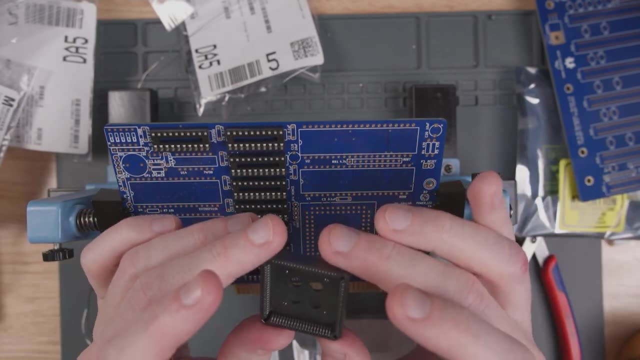 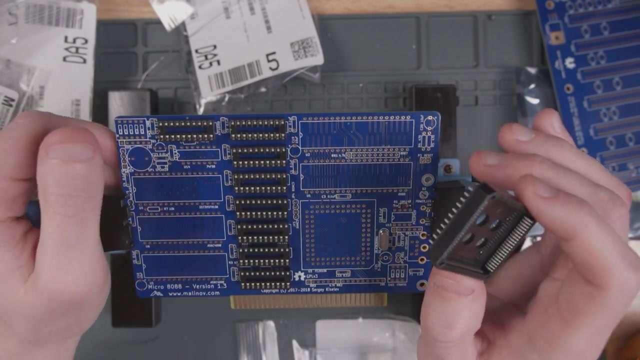 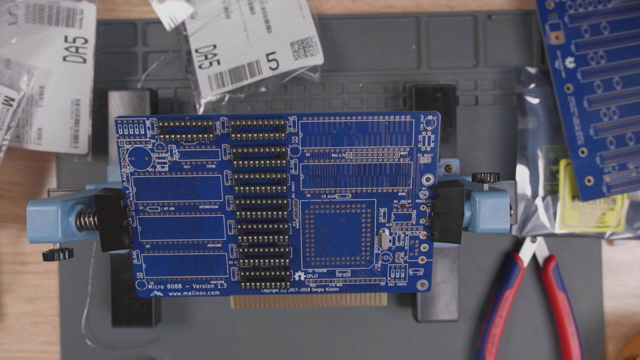 slides down them. so it's just kind of neat. oh, this might be bigger than i thought. oh, maybe not. uh, okay, so this also is directional, i think. i just look, i dislike your mileage may vary. deals, yes, that's, that's. you know, i kind of ignore those because i kind of figure i don't know if it wasn't, if it. 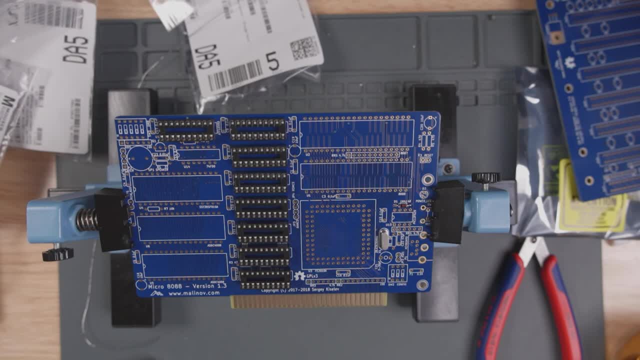 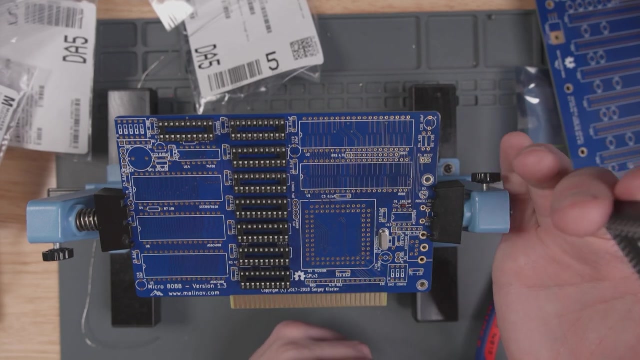 wasn't, uh, meant to be bought online, then not a bad way, it's just you know, i, i just need to limit my spending period, not just. you know, sometimes i don't know, i'm just kind of lazy, plus i work from home, so it's like i don't know. it's complicated, okay. well, uh, i said this was. 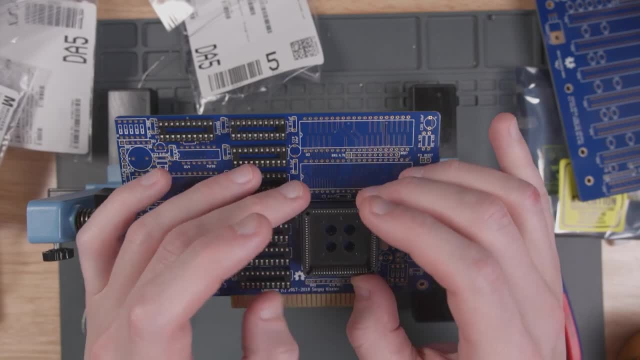 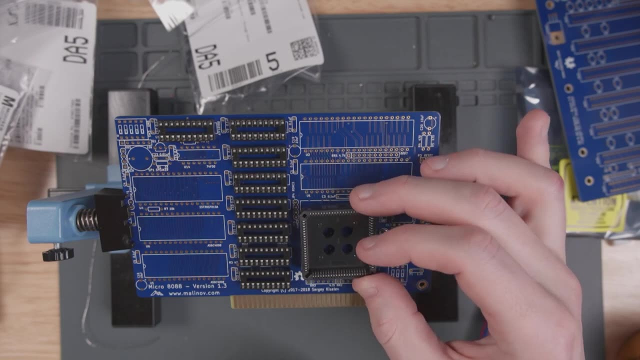 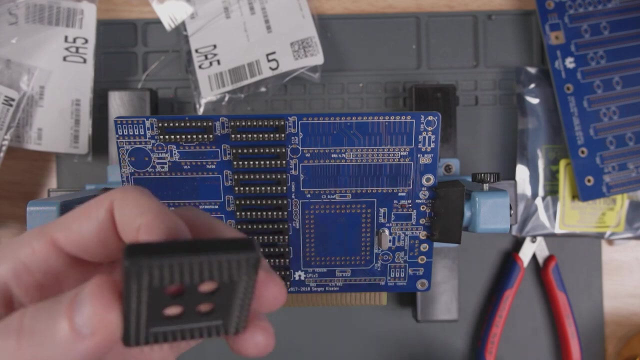 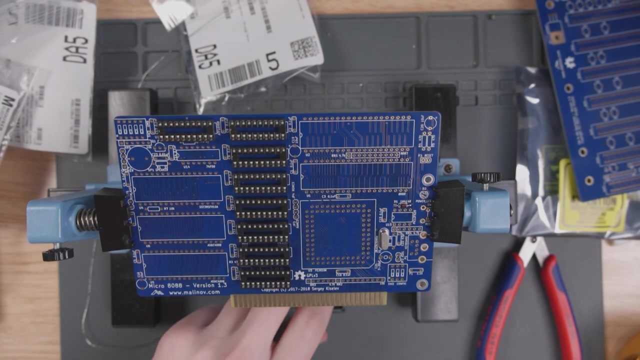 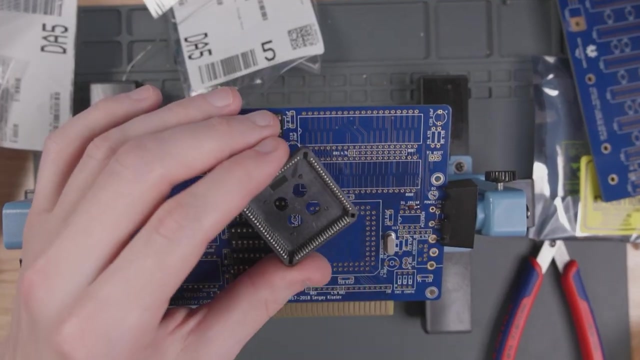 directional, but i'm not sure what the direction is. this is the socket for the, the faraday chip. i gotta figure out which direction it is. all right, let's look at the picture. does the picture give us any guidance? kind of does so. there is a, there is a cutout here. well, let me show you the picture. 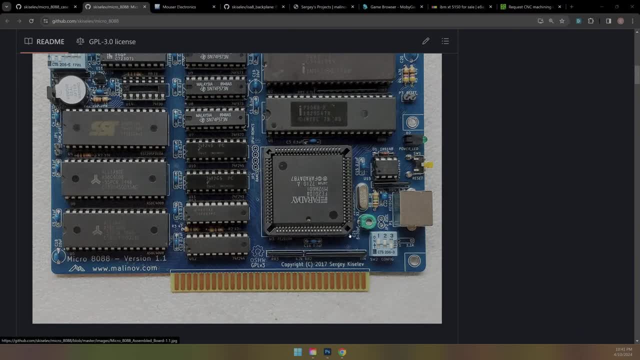 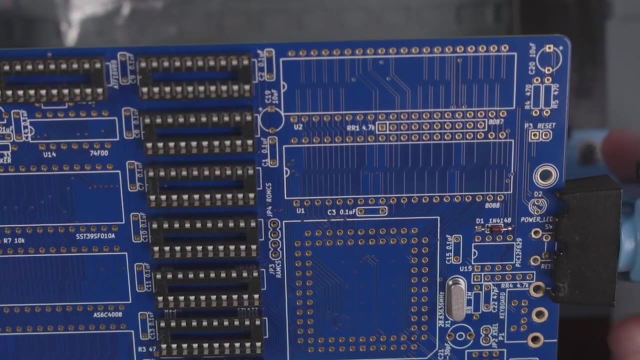 there's a notch in this bottom right corner here, whereas the other sides are kind of rounded. excuse me, oh man, i got hiccups or something. so that is the orientation that we're going to do. so the notch at the bottom here, notch at the bottom here, is going to match the notch at the bottom of this. 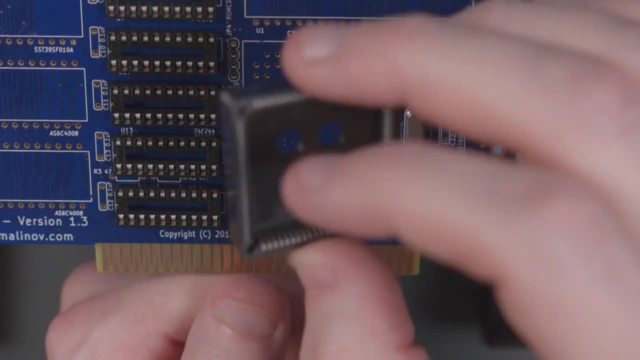 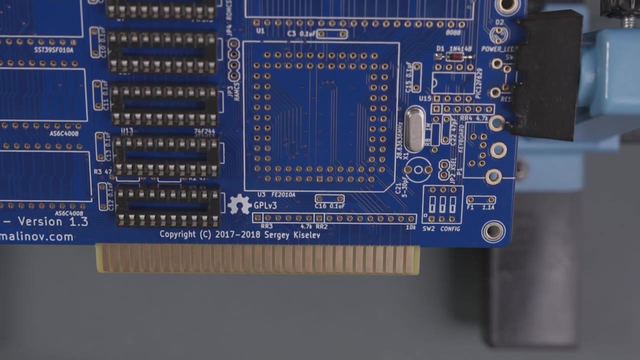 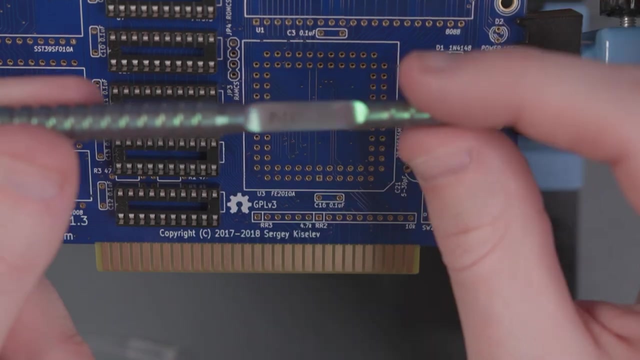 now the second. so that was the first hot tip. now the second hot tip is we need to make sure that none of these pins are bent. oh, this might be a good job, for i got my some new tweezers from northridge fix. i think i overspent, overspent on them, but that's fine, i like supporting them. 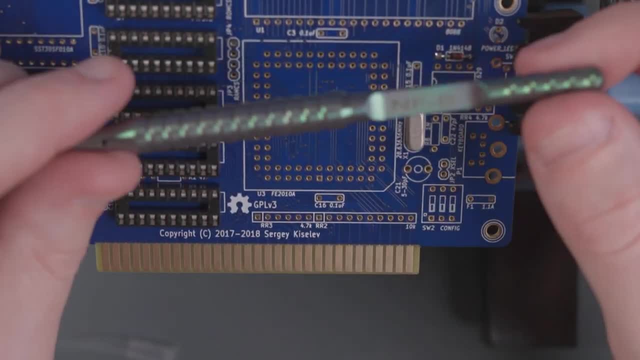 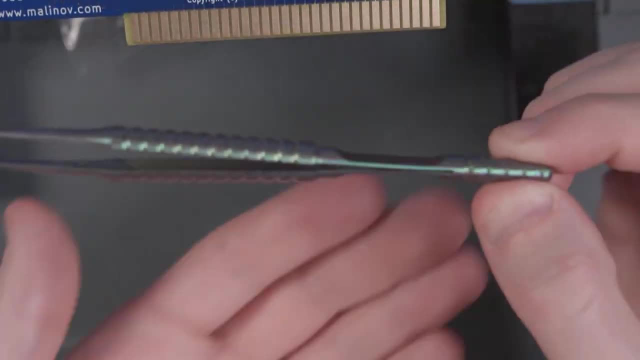 they have this cool. i mean, this is the only the first time i've ever supported them. it has this cool like titanium, like burnt kind of titanium, look, and these tweezers are probably the the pointiest, tiniest little tweezers i've ever. 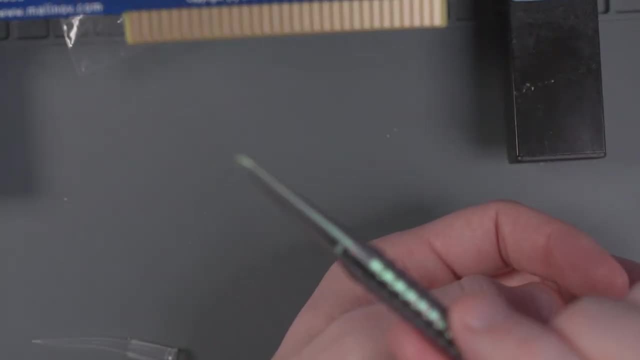 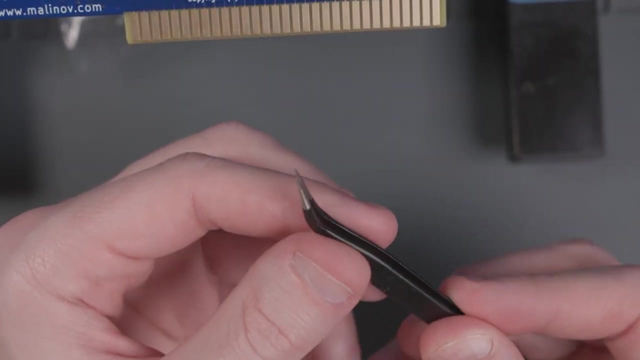 seen in my life. so then, probably better for s and d stuff. but my previous smaller tweezers are just getting a little bit more of a twist on them, so i'm going to go ahead and beat, beat to heck. as you can see, the the tip on is broken off of one of them, so not ideal anymore. 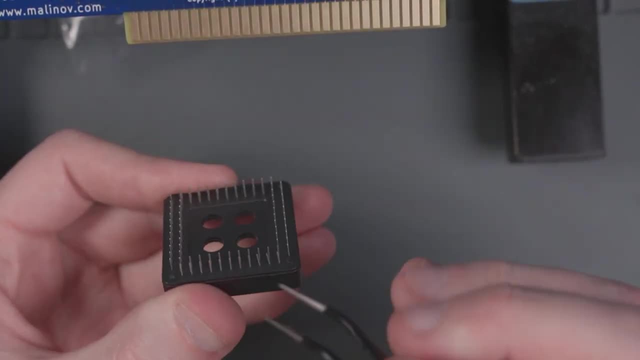 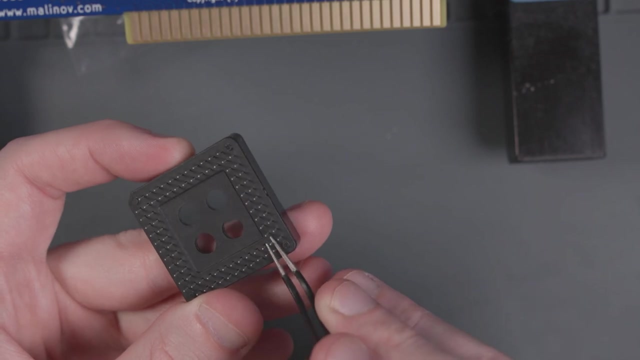 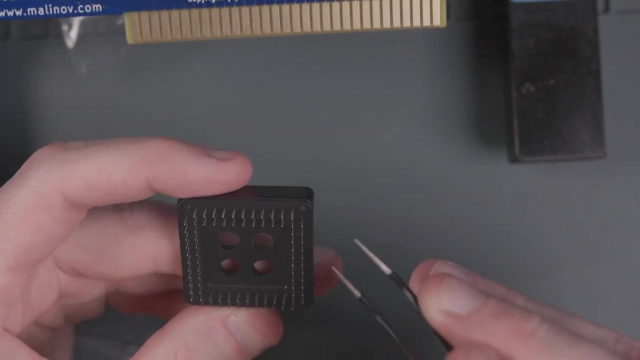 but still good for this which is trying to straighten out pins. so before you, before you even put this thing in there, you just got to straighten them all out, make sure they're all lined up. just got a little little how you doing on the on the uh flight over here. 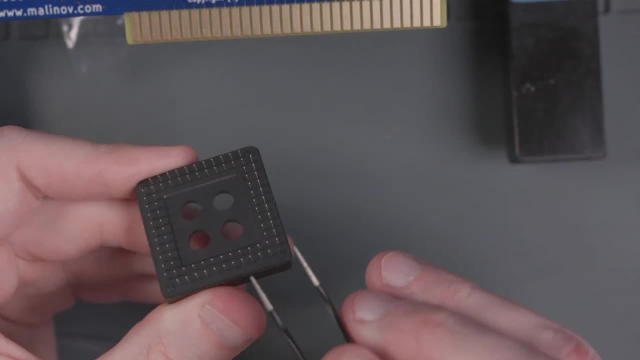 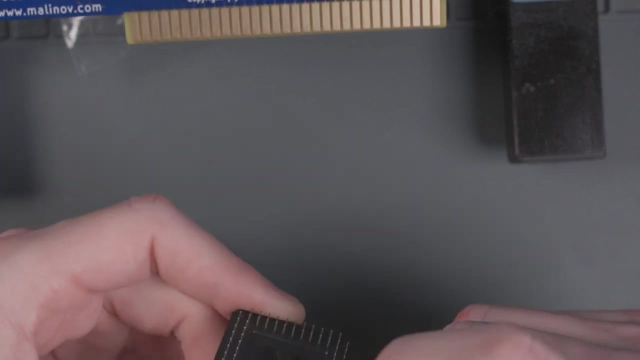 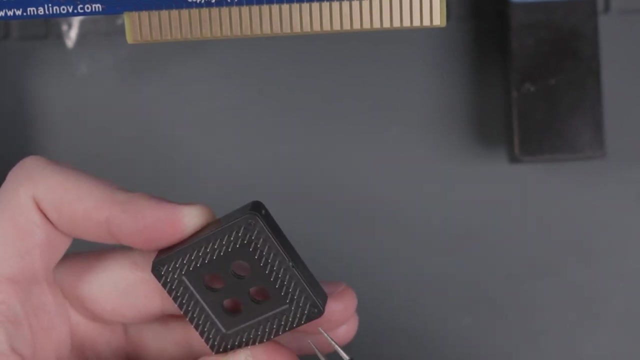 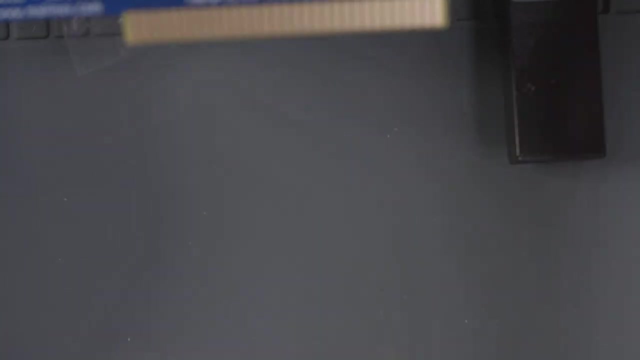 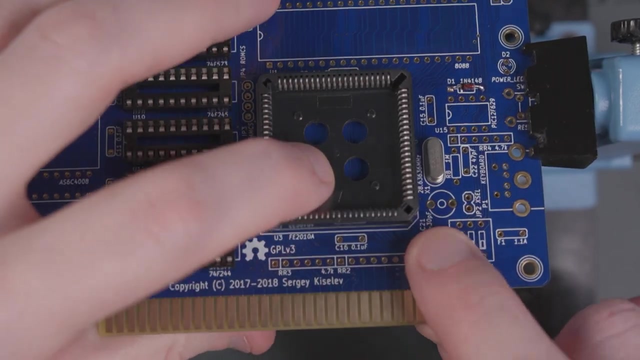 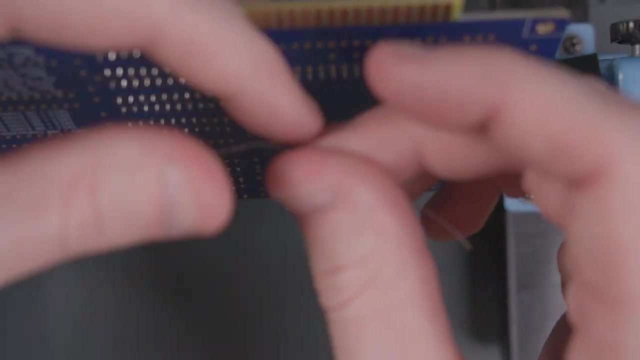 for the drive. i don't really know how they came. okay, all right, let's try that. oh yeah, like a glove, all right, so make sure our notch is in the corner here in the notched spot, and now we just got to start it. it's gonna be a pain in the butt. 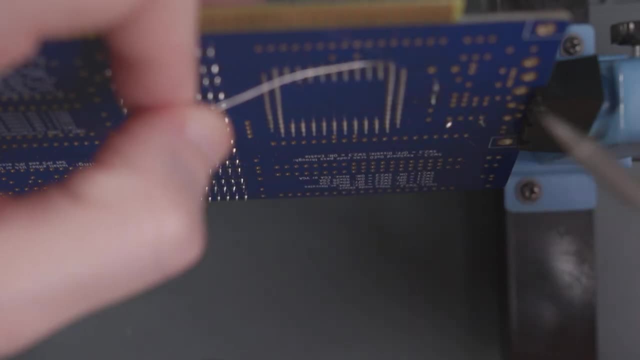 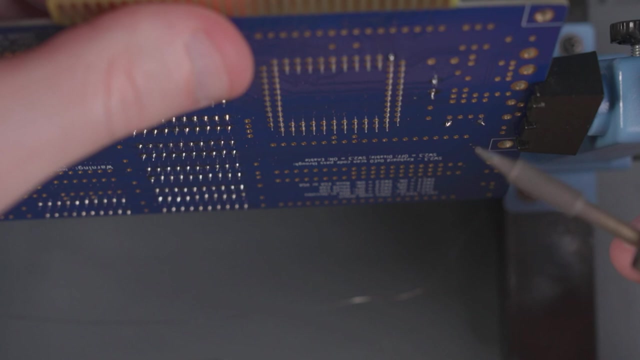 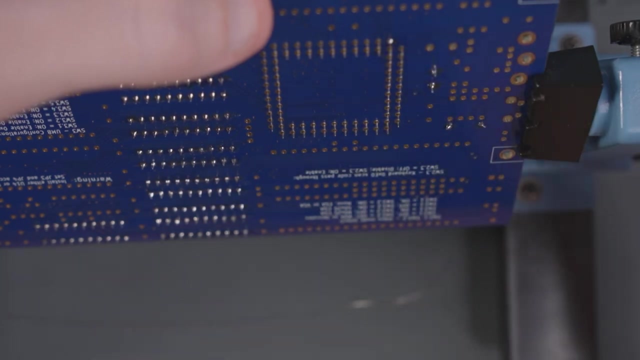 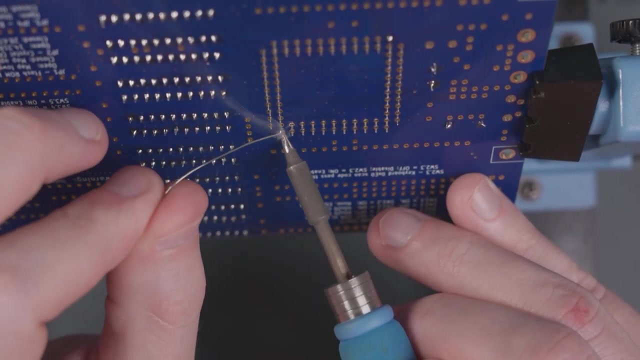 maybe not okay. so for this one i'm definitely going to, um, do this and then push down on that first pin to make sure it's absolutely flat. okay, now, on the opposite side, kind of do the same thing, so like that, and then i gotta make sure to push down. 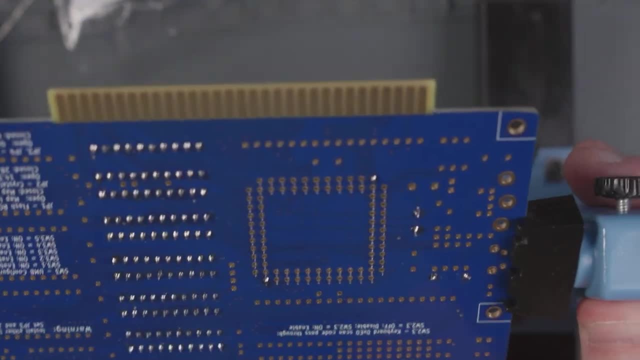 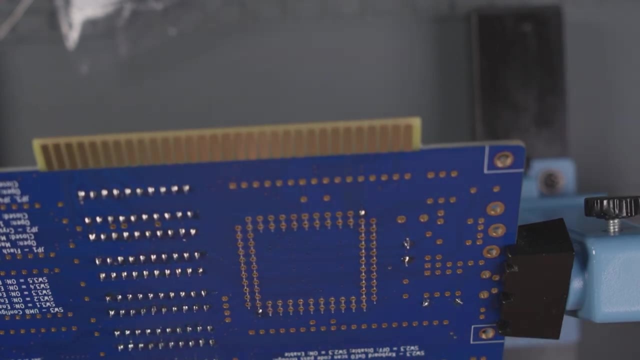 okay, cool, so now we can just start blasting. actually, i've got this now, since i have my quick change tips for my soldering iron, i might as well, so let's do, maybe like a- i don't know, knife edge tip thing. does that sound? i did end up super gluing my- uh, this eisen. 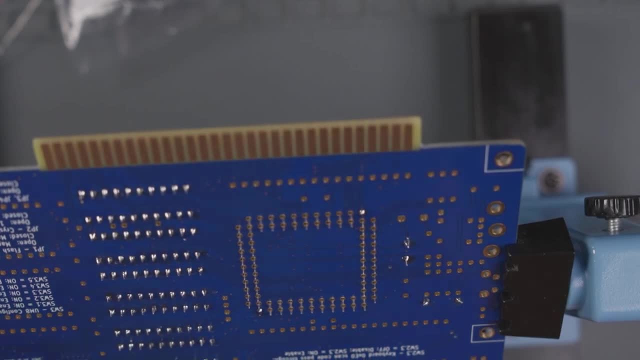 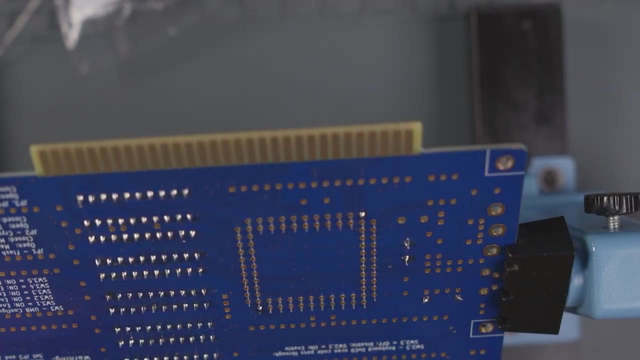 hand piece that kept falling apart. i don't know if you were comp, you heard me complaining about it before. but this, oh, why is that so hot? oh god, i touched something in it. maybe it wasn't hot, maybe it was just sharp. i thought it was hot, so i made me eat my anyways. uh, i super glued these. 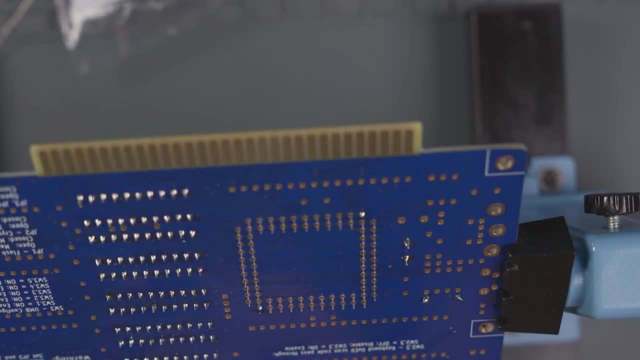 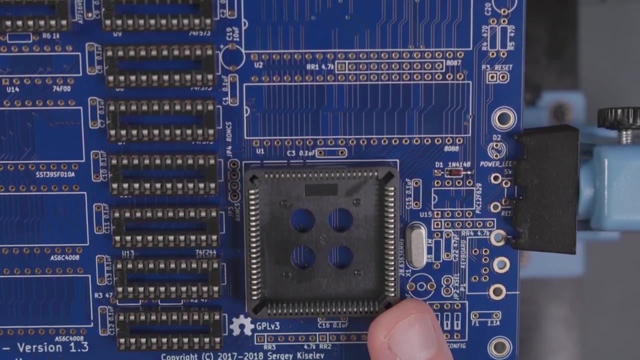 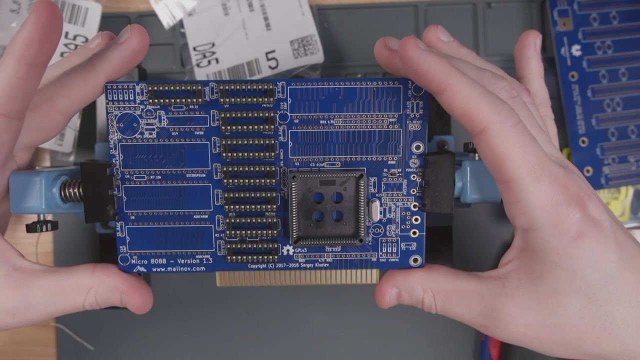 pieces together so that they wouldn't back out anymore. so it hasn't come apart, so i don't see you, not yet this is just the pll or the plcc. uh, holder for the. this, this is um, this entire thing is like the cpu and it's only this. well, and a lot of the additional functionality. 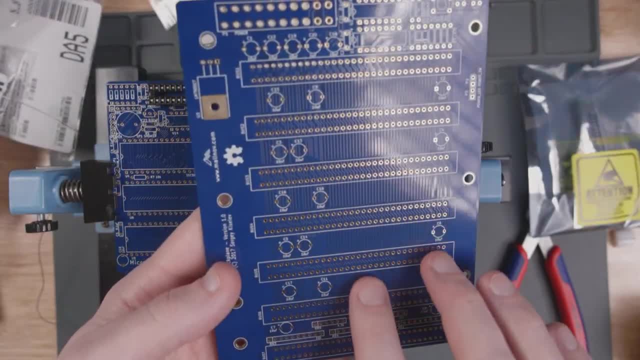 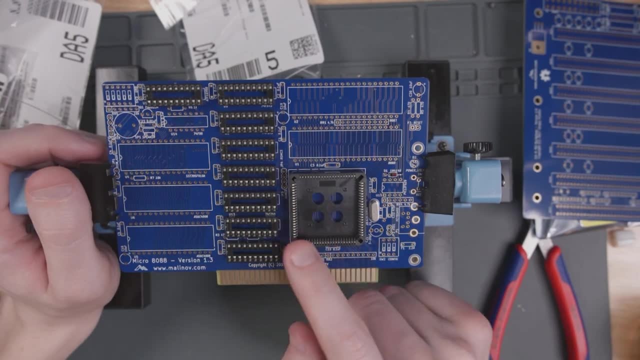 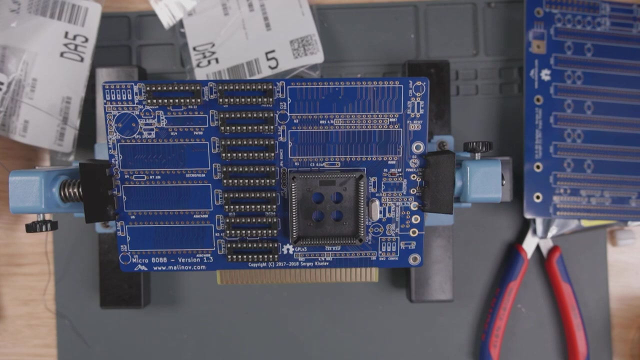 because the the backplane really doesn't have that much functionality either. it has the isa slots and the power stuff, but, um, a lot of the features of this uh cpu are on this. they're on a chipset, specific chipset chip called the faraday, which is in my box of parts. so when this is all said and done, 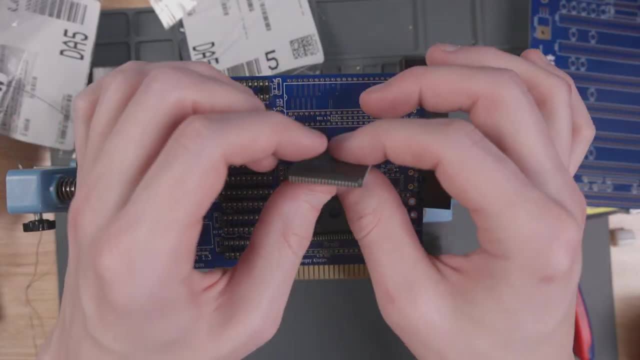 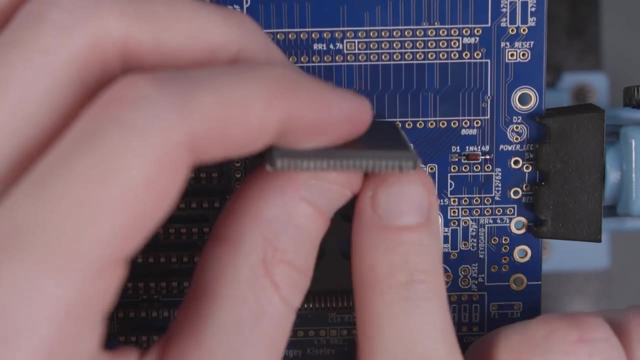 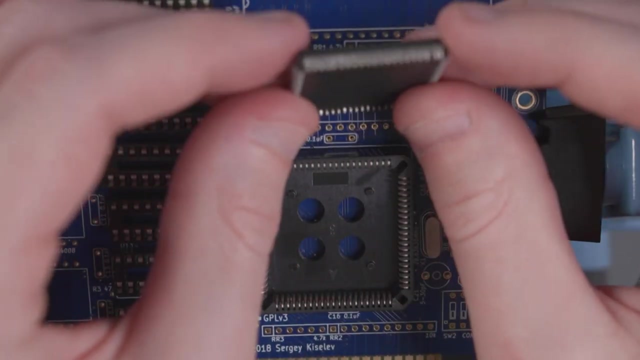 this chip. this has got kind of cool spring fit kind of oops. see, i got to make sure that these are all. you can kind of see that these are all kind of bent out of shape. so before i actually plug this in, i got to make sure that that's, everything is in. 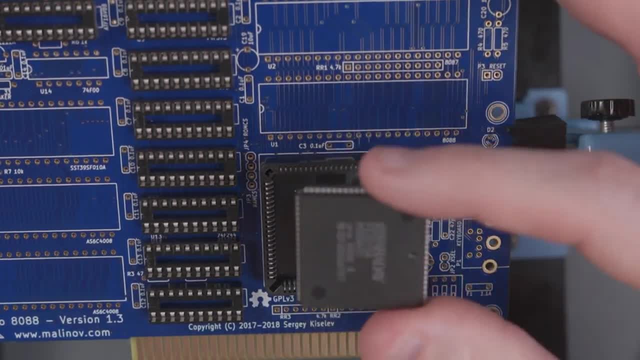 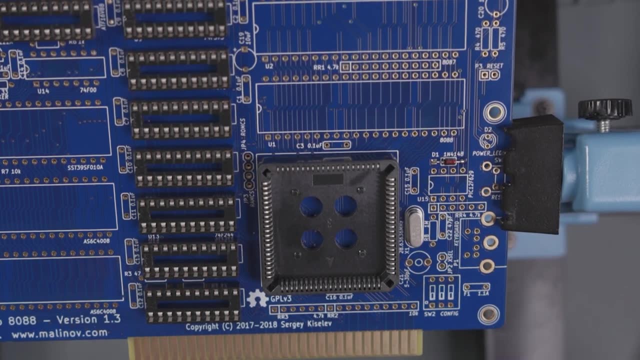 the right order anyway. so this is the. that chipset chip and this uh distributor are in the same type of material, but, as you can see, it provides a lot of the functionality. there's a list of the features on the the thing, but it like i don't know. 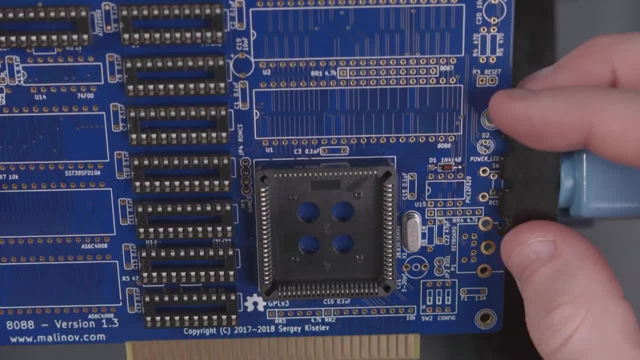 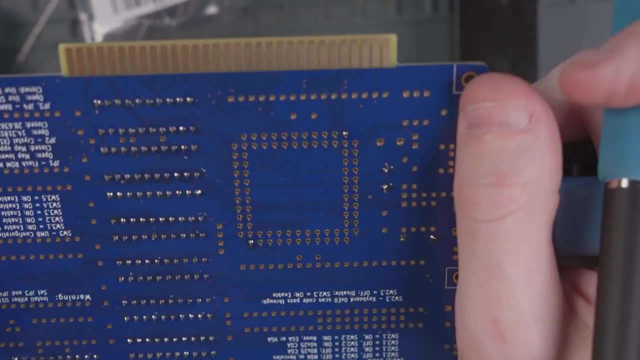 provides some stuff, probably the floppy controller, so not yet just the socket, and we're not gonna. actually we're not sucking or we're not soldering anything in. this is all stuff with sockets, which is really cool. all right, let's do a little bit of drag soldering. i haven't. 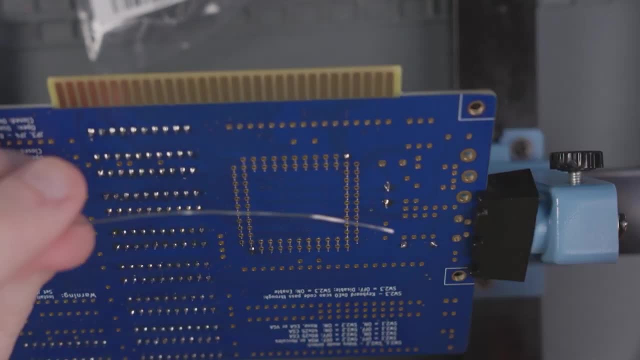 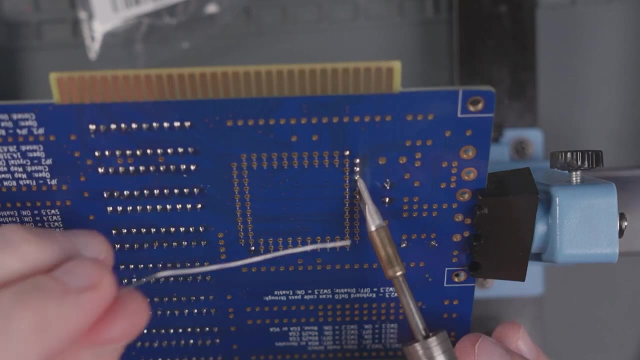 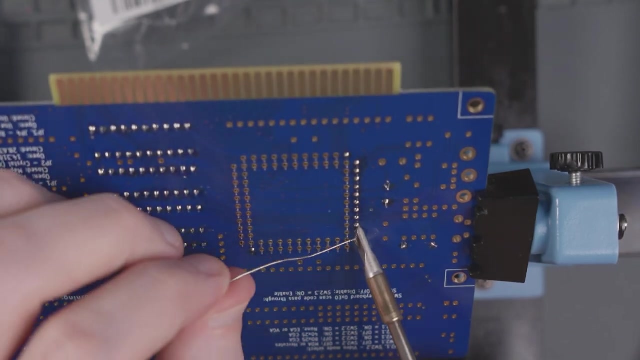 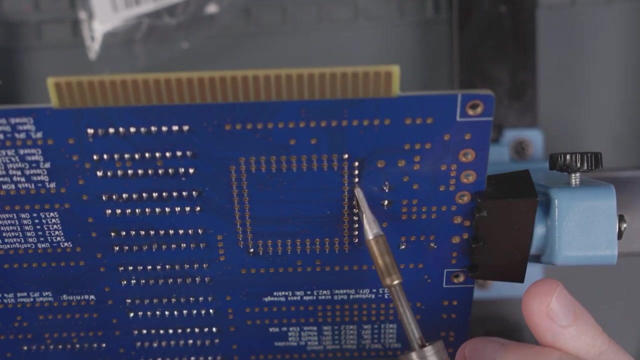 done drag soldering in a long time. but it's like riding a bike. maybe I'm only not adding extra liquid flux because there's already flux in the new solder. If I was desoldering something or doing like an NES RGB, I would add flux. 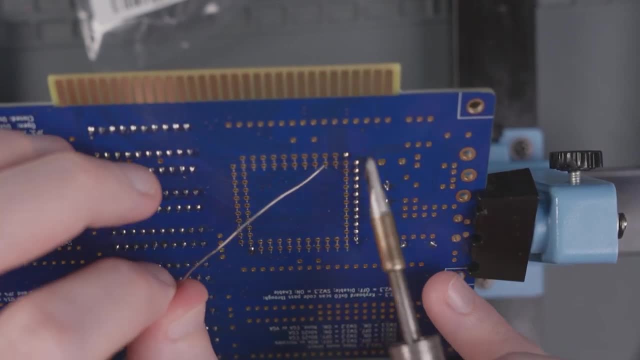 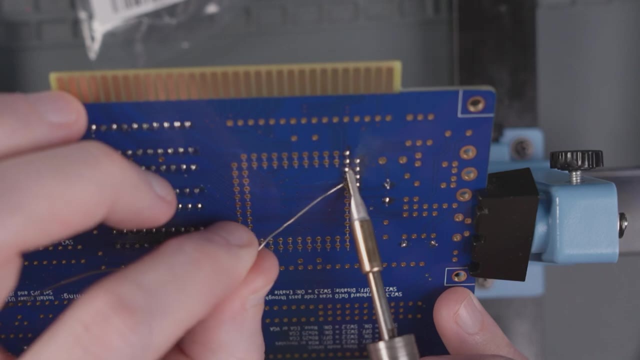 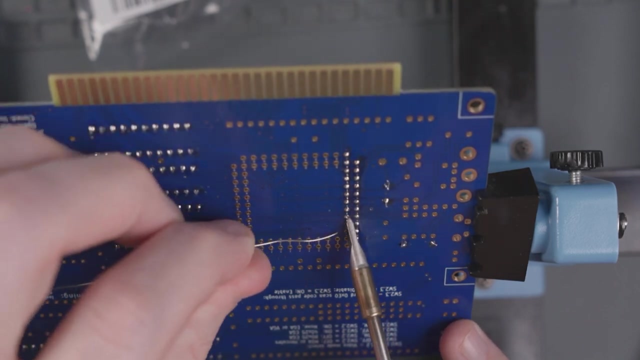 Okay, cool, I'll probably also get more. you know, I'll look at each of these pins when I'm done to make sure I haven't made a bad connection or anything. But this beats having to solder 8,000 pins one at a time. 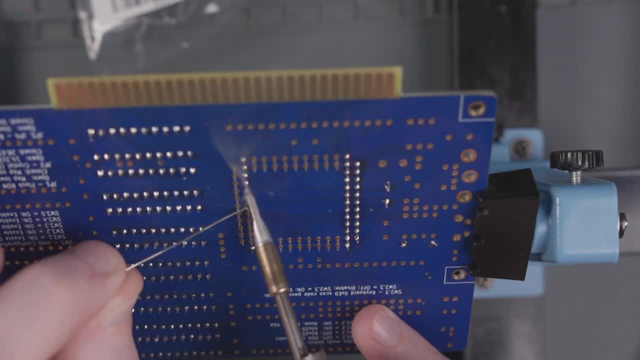 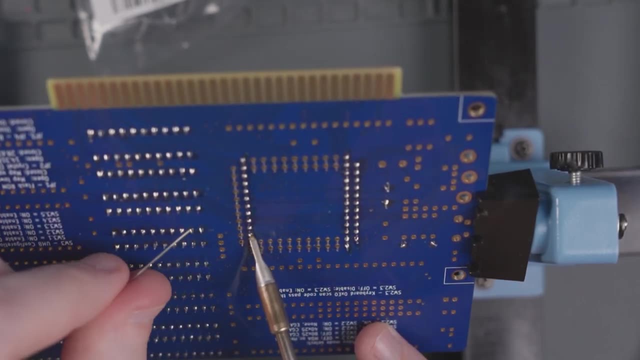 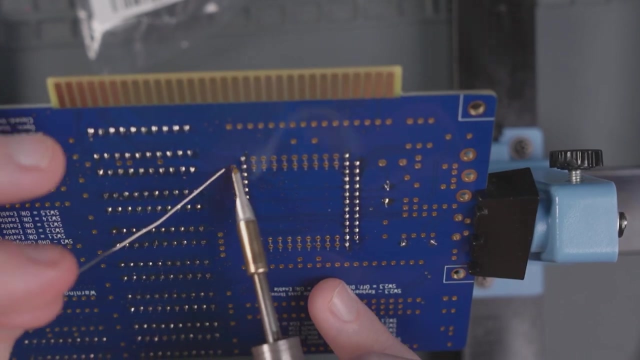 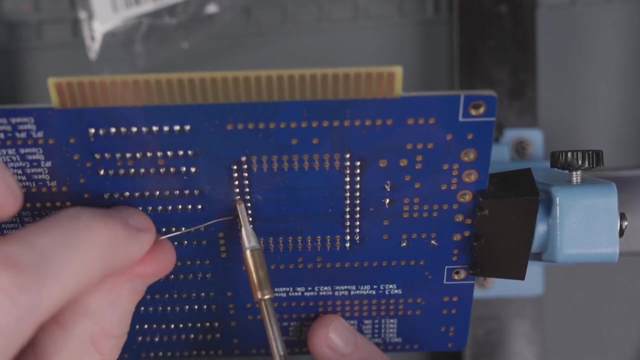 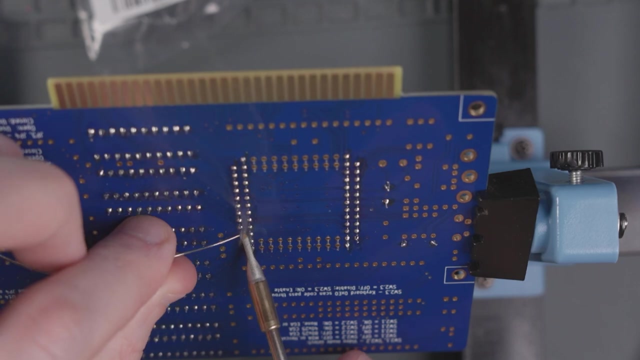 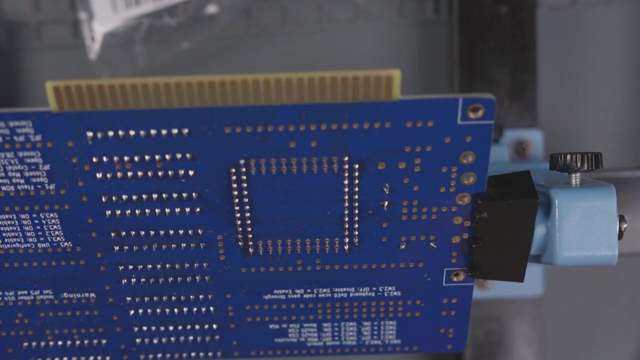 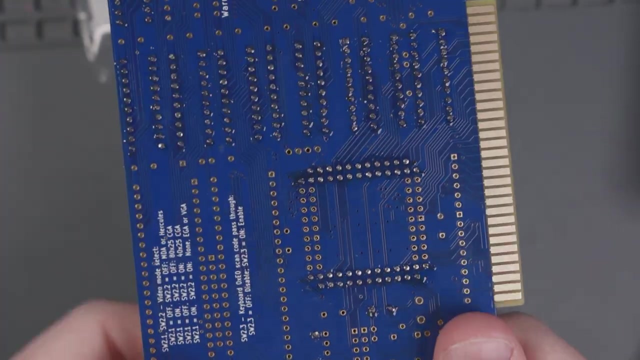 It sounds cool. it's like springy on the back when I'm rubbing the pins. That sounds stupid, but it just kind of makes a fun sound. Okay, Oh, but now what do I do here? I'm going to have to like go sideways on this, I think. 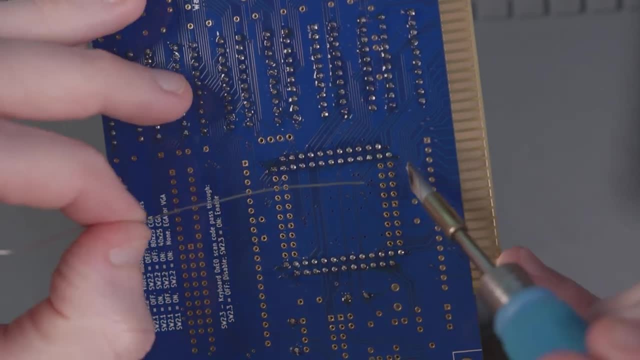 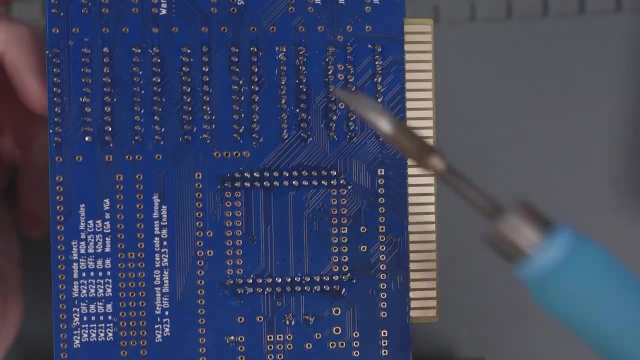 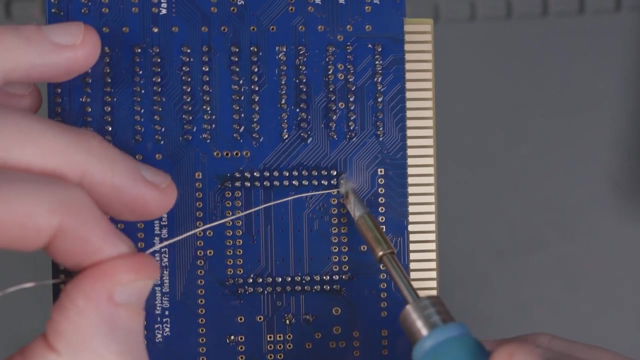 See, this is one of the main reasons I bought this soldering iron was because it has the the removable tips that you can kind of remove stuff without having to use a wrench or something or wait for it to cool down. So that was kind of a priority when I bought, when I bought this iron. 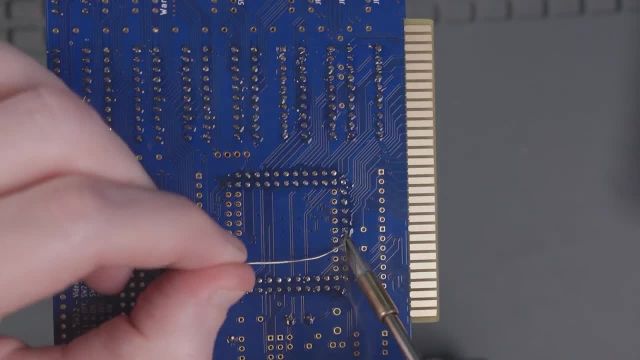 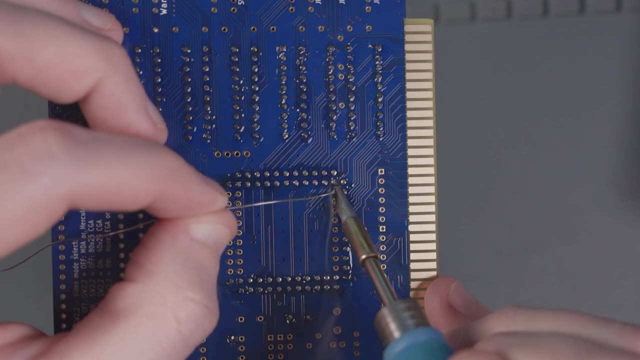 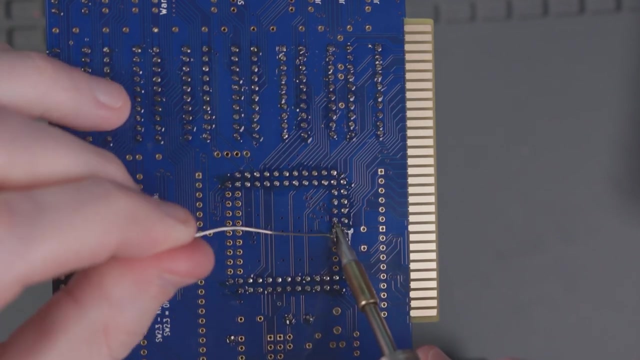 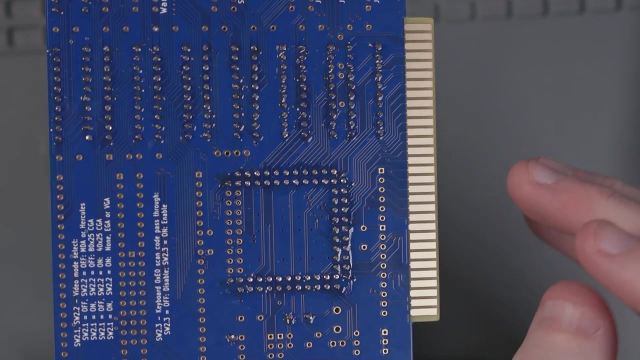 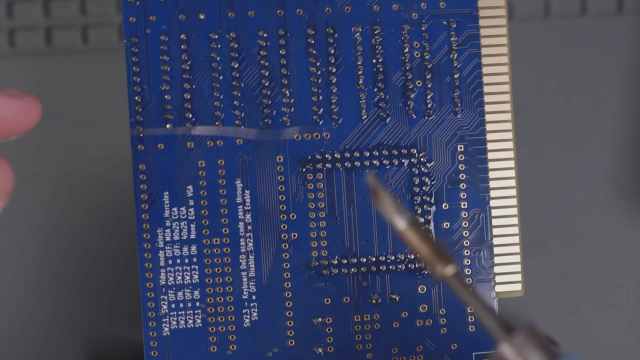 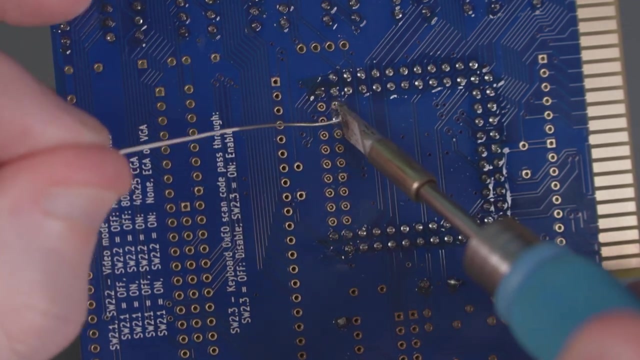 So I had to do that because I couldn't. when I had my Hakko FX80D, I couldn't switch very quickly, So it was just kind of annoying. All right, last part. So thank you so much for watching. 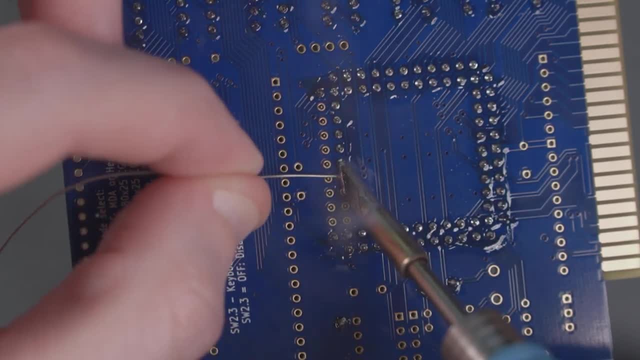 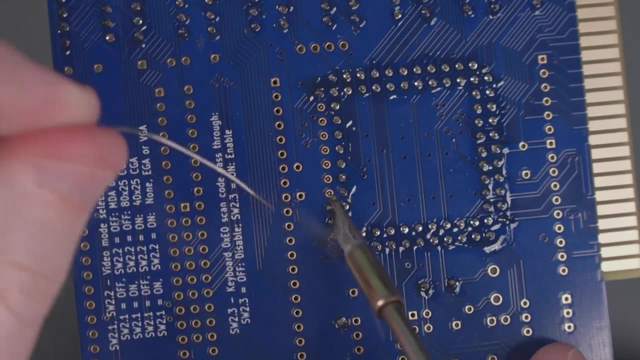 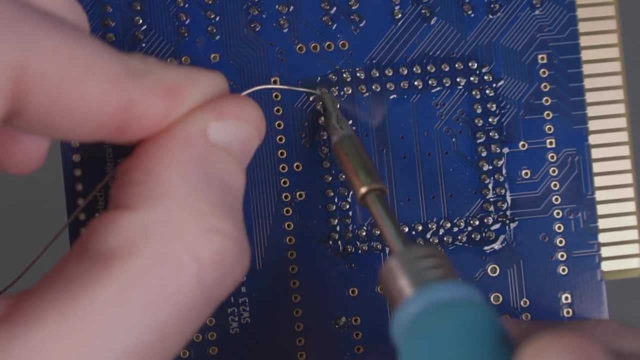 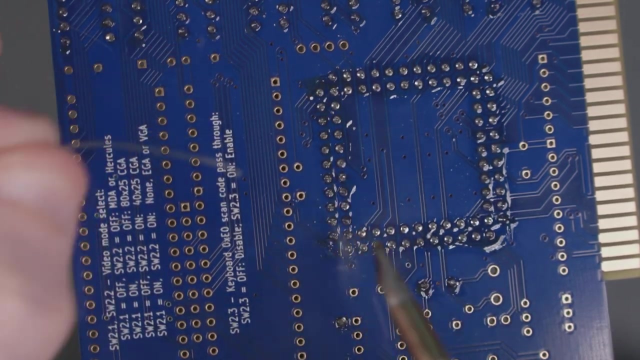 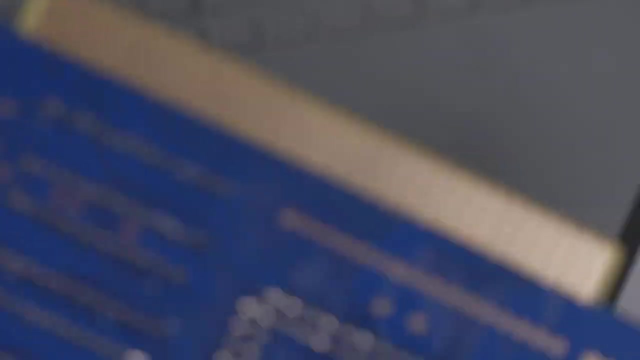 I hope you enjoyed this video. If you did and you got something you like, please leave a comment. This is the end of my video. Have a great day, Bye, Bye, Bye, Bye, Bye, cool, all right, I'm just doing a quick little visual inspection. I know I don't, I can't get. 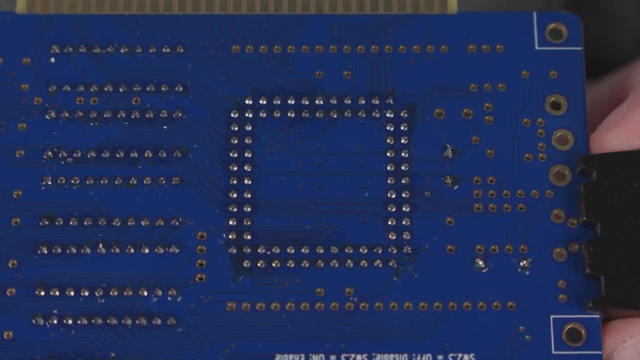 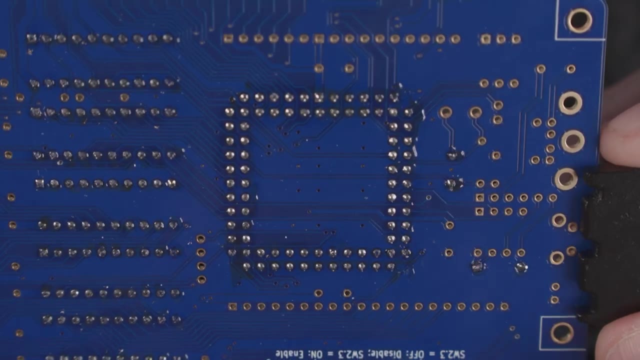 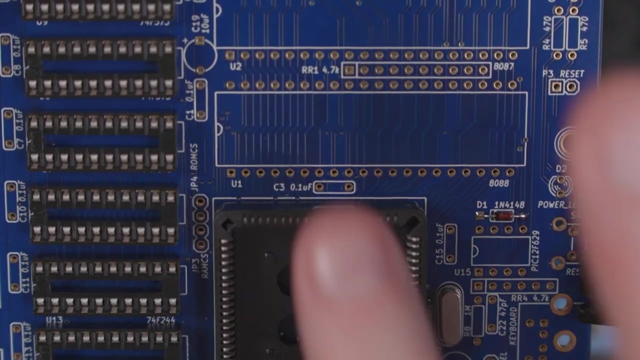 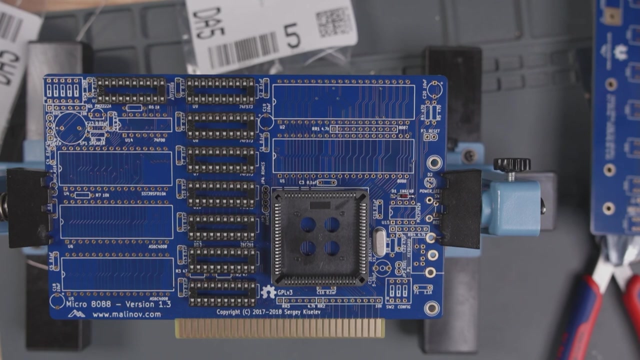 super zoomed in right now. but that's right, it looks fine. I mean not amazing, but everything looks connected. cool, all right, cool. and then then this is where we would stick that big Faraday chip. eventually you get a knife tip. yeah, I mean I would say the three, the three must-have. 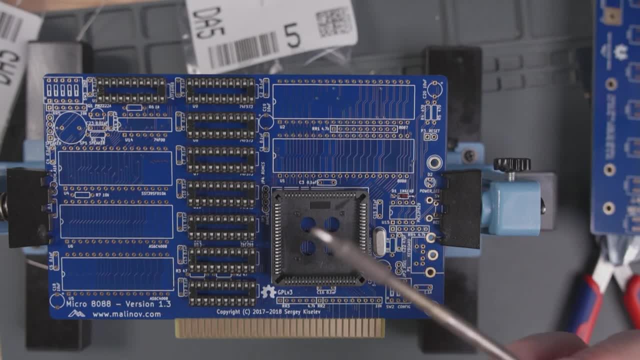 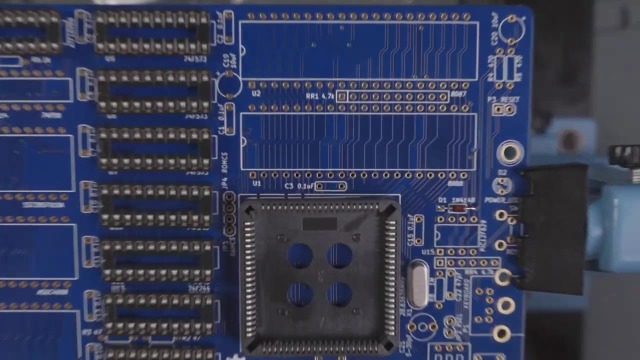 tips the three, three horsemen of the soldering apocalypse is the night the conical, not conical. just think. what did they call this? I guess it's cut in, not circular, but it's like a blunt edge, i guess it's not. it doesn't come to a fine point. 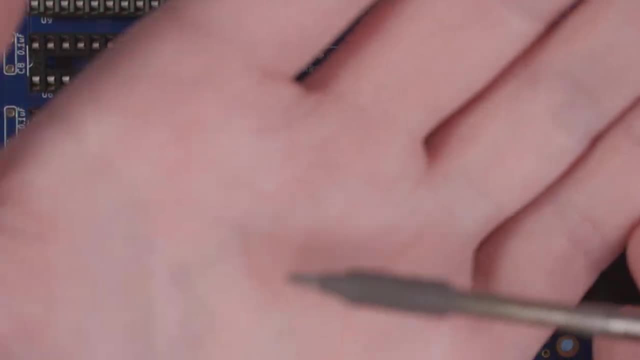 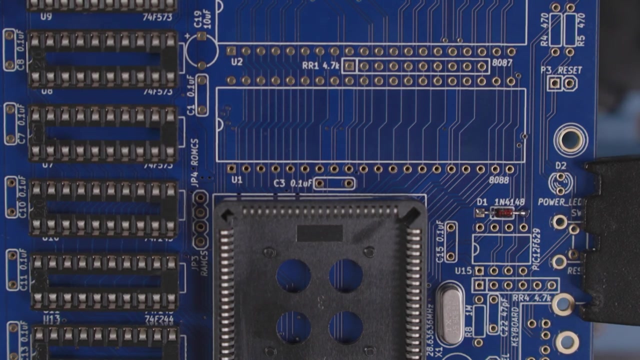 um, this is the normal. i don't know what they call these, but this is like your standard tip, whatever. uh, i actually have that in both that size. so that's like what a millimeter, 1.2 millimeters or something, and i have like a 0.6 millimeter one, i have a tiny one. um, for more, just, micro. 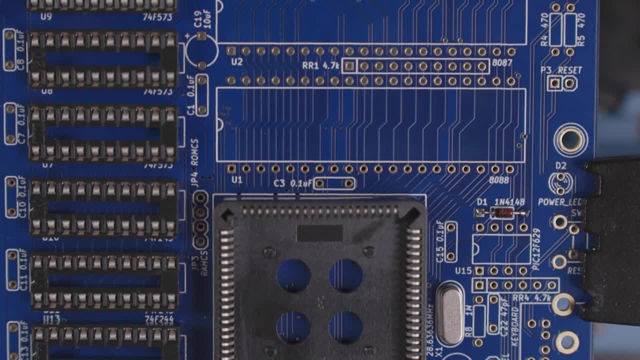 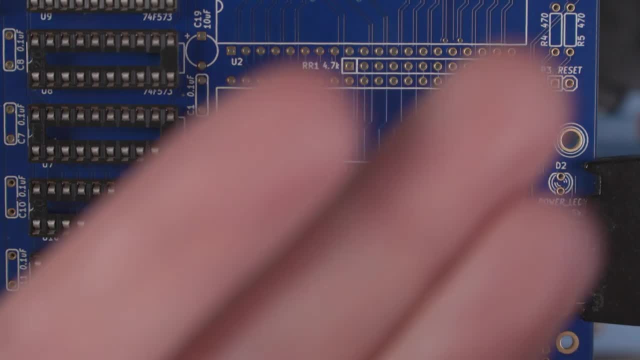 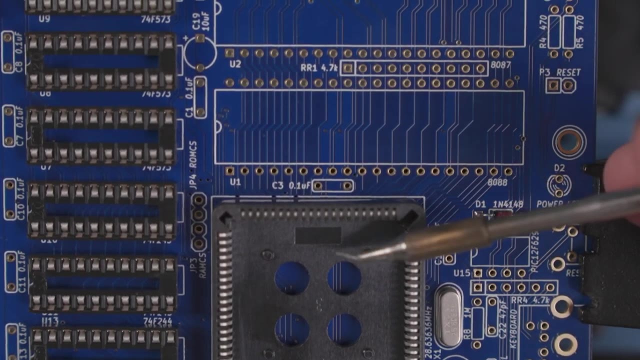 soldering stuff. so that's the first one, that's just the normal. i guess it's called conical, maybe not, i don't know. there's a name for it. then there's the j tip, which is also kind of nice for drag soldering. i mean, some people prefer this over the um knife edge tip, but i you know. 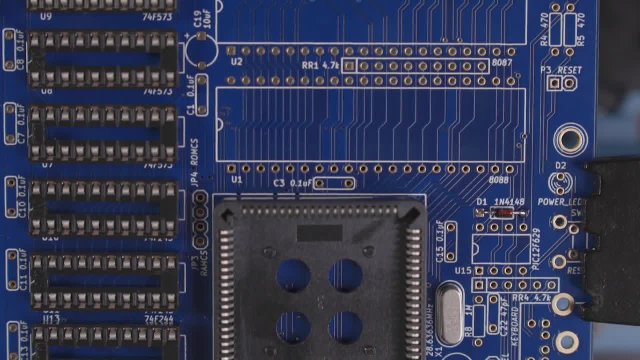 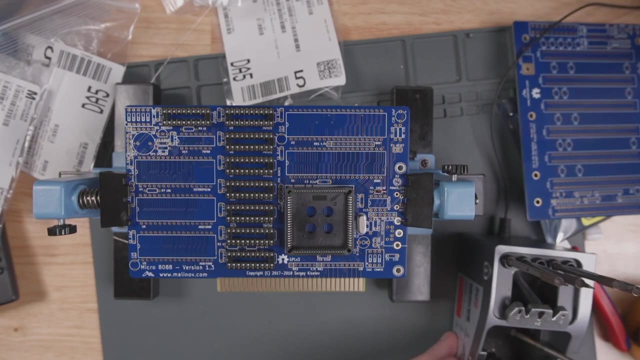 this is called the j tip and then, uh, the knife edge tip. i actually have a tiny one too, but yeah, and then the cool part about these is you can just- i know you guys can't see, but i guess i could bring this over. it comes with this little stand. 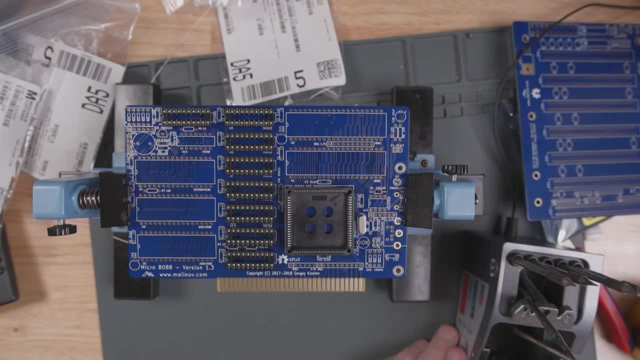 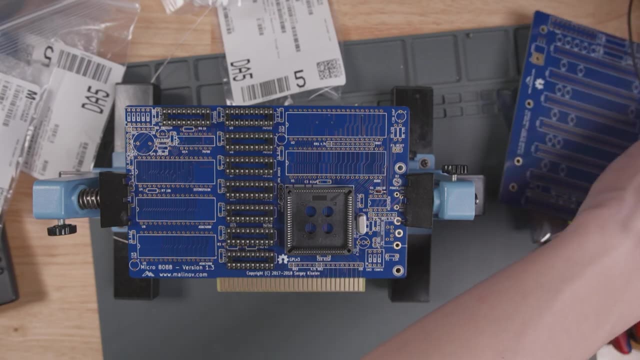 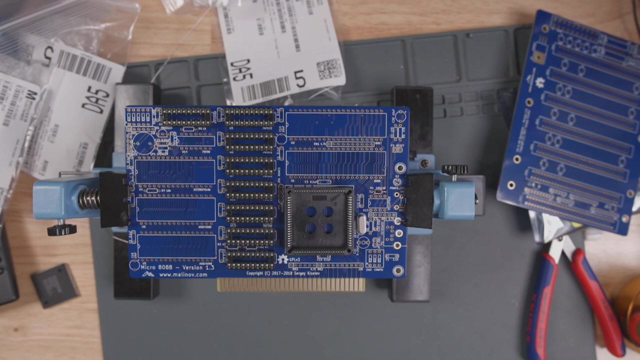 the soldering iron, and then you can just pop it out and then pop, pop the other one back in and that's it. it heats up right away automatically. you don't need to turn it off or anything. so it's really handy for that. all right, what's next? you like the j? 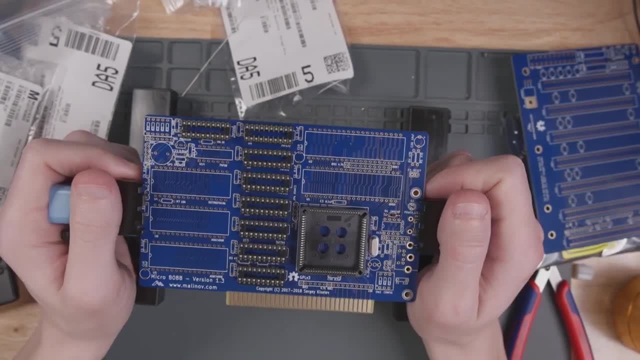 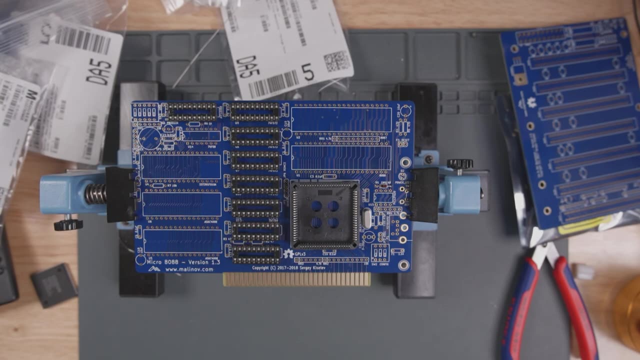 over the knife. yeah, some people like one or the other, but then some people will like only solder everything with certain tips, like that, like i don't understand that. like every soldering they do is with a k tip or a knife edge tip- like crazy in my opinion. um, all right, let's see if we can. 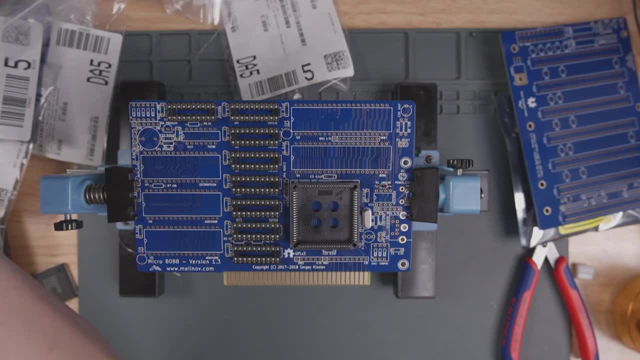 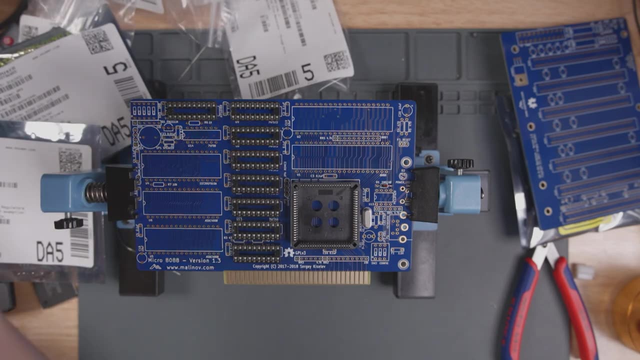 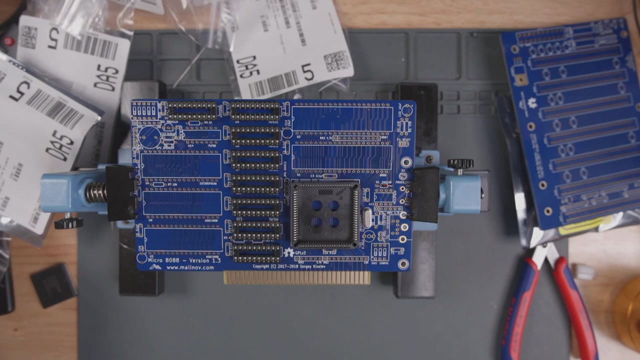 find a dip. oh, i didn't have switch two, wasn't switch two in this pile of stuff, i want to do something fun and then we can end the stream. u3, no, u16, i should put all the chips aside. p1, what was p1, i don't know? hmm, oh, it looks like a. oh, that's the port, that's the uh. 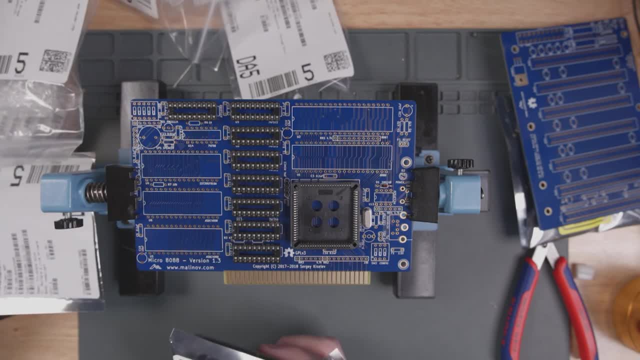 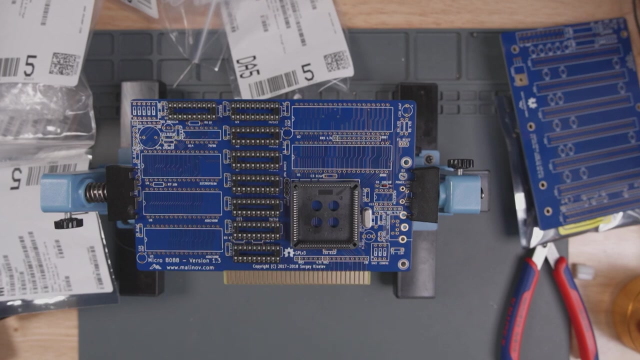 keyboard port: shoot. i thought i had the switch mic, the little dip switches. i gotta find them quickly. looking for micro switches q1. i don't think it's called q, i think it's s, s2, sw2. wait, didn't i see that in the beginning? 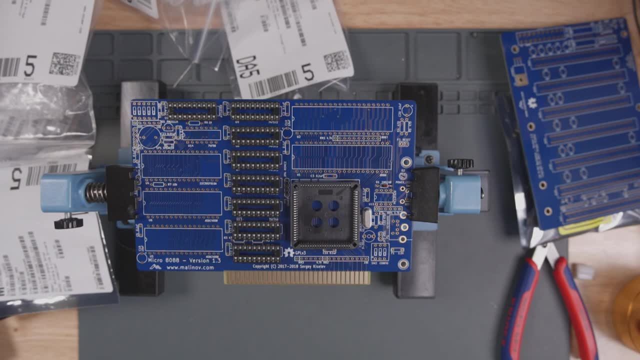 shoot, maybe i put it back. watch, i'm going to dig through this whole pile and it's not going to be in here. u14- socket buttons. uh, u15, what's this? oh, here's the socket for the cpu. oh, here's a face mounted button. i did not know there was a face mounted button, so here's switch. 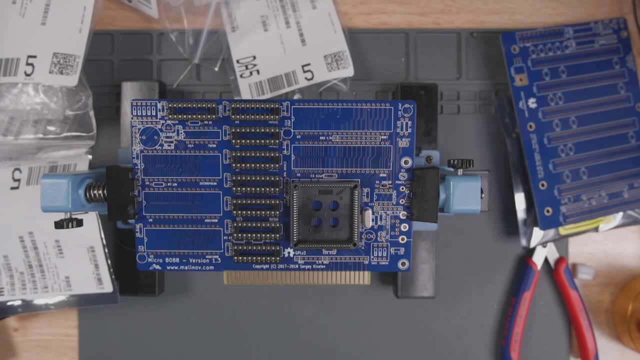 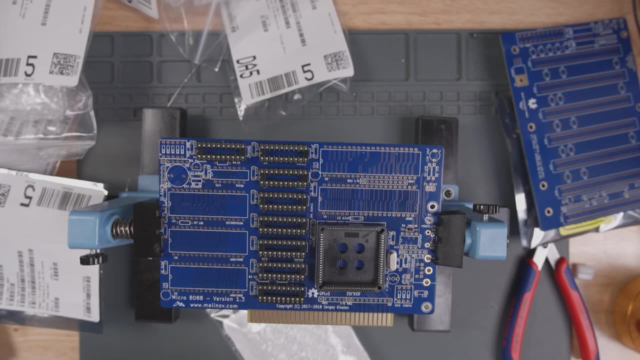 one, switch three. oh, here's one. it's not the one i was looking for, but it'll be. oh, it's the bigger one, it's the one up here, all right, so let's do that, that'll be fun, fun. uh, that's funny. okay, we got this nice. we kind of threw out the thick to fit or the tall to thin thing, like right. 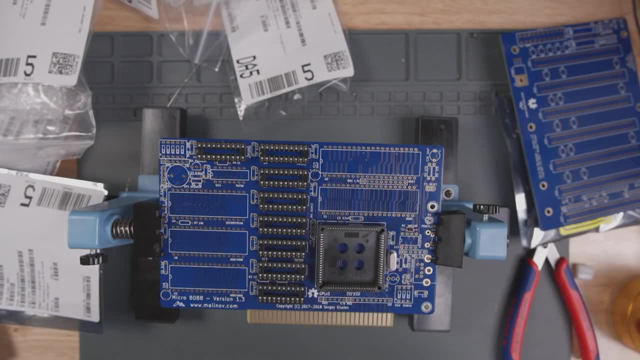 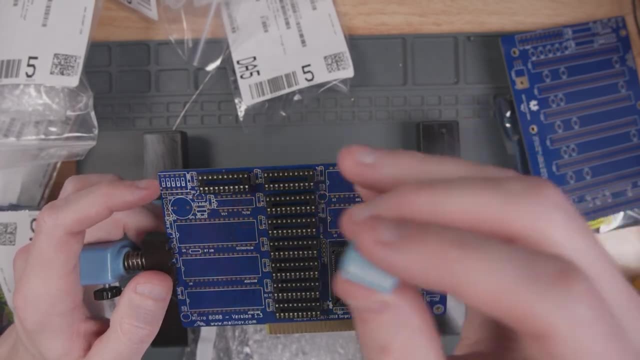 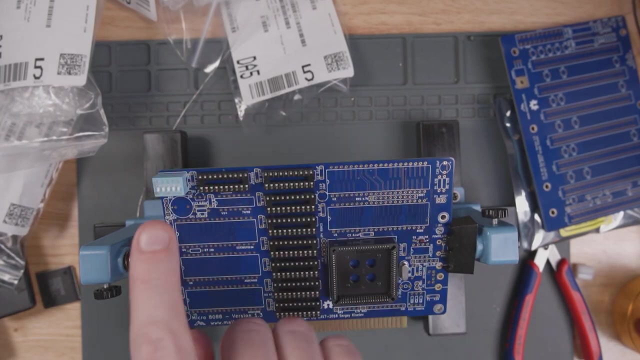 away. okay, so this is switch three, which is ones up here and i don't. you know, switches are not necessarily, are they? i guess they could be directional. um, but it has more to do with how you read it. i'm just going to place that there for a second and then we're going to look on the web. 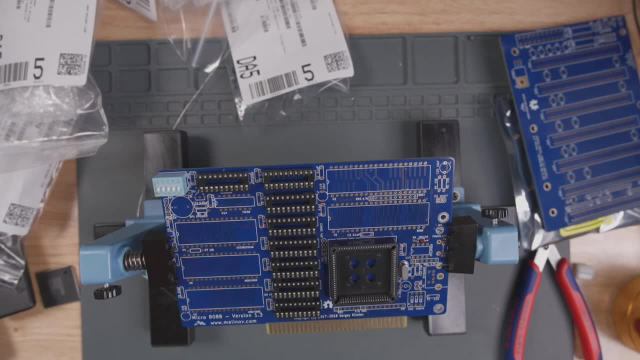 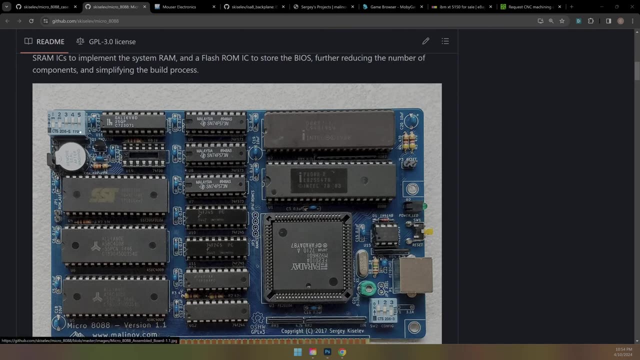 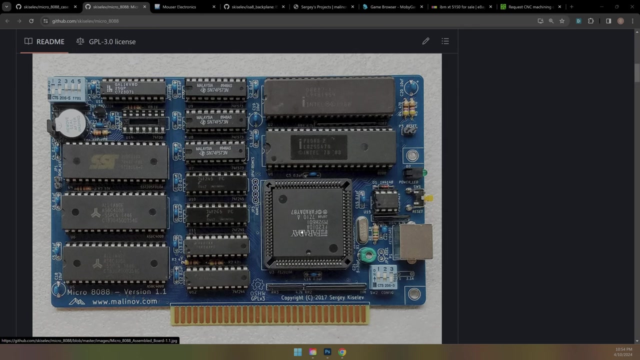 site here we're gonna look on the picture. okay, so it looks like everything. if we take a look at the original or the photo on the github, everything is meant to be so that the labels are readable. well, except for the- uh, the faraday chip is upside down, but the the details on the switch little. 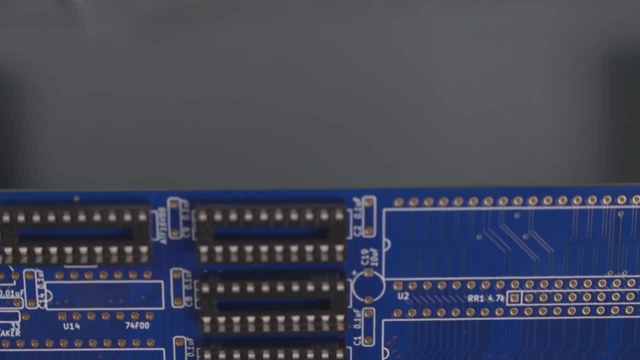 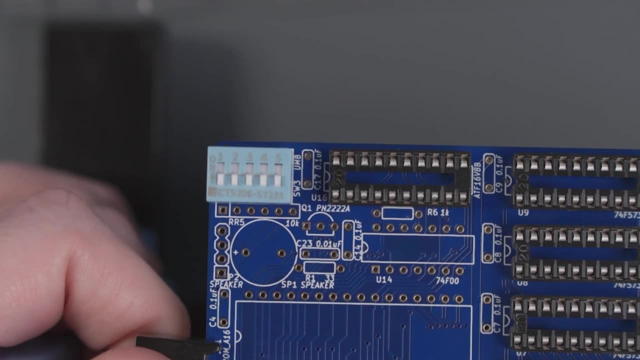 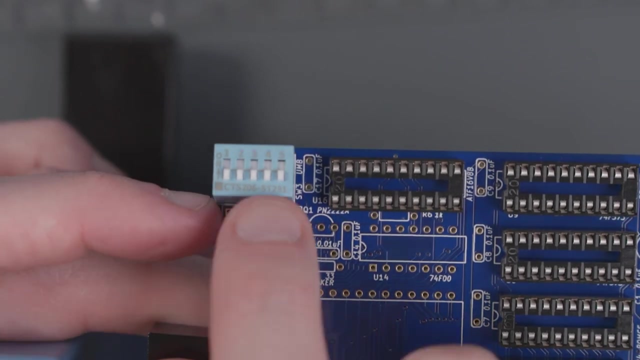 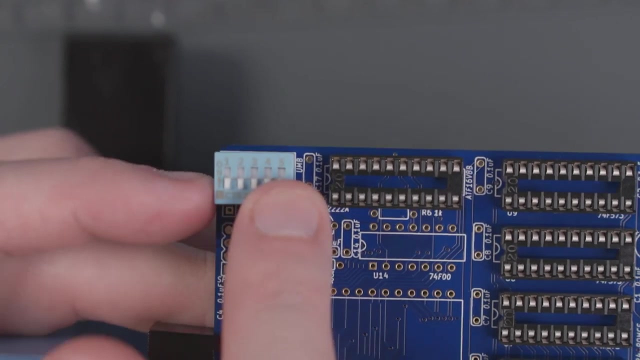 thing. i don't know what that is. uh, the text is what i'm thinking of. the text on the switches is readable like this. i know you guys probably can't read it, but it's not focusing on this part, it's focusing on this um. so uh, with like on is up, so like that's the orientation, i suppose. so let's get. 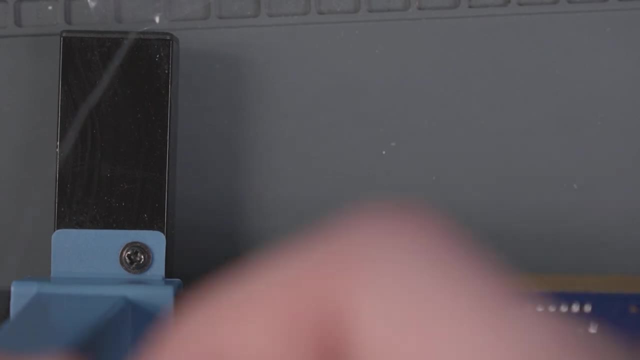 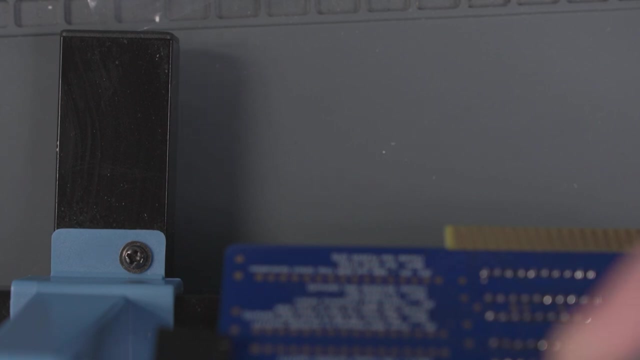 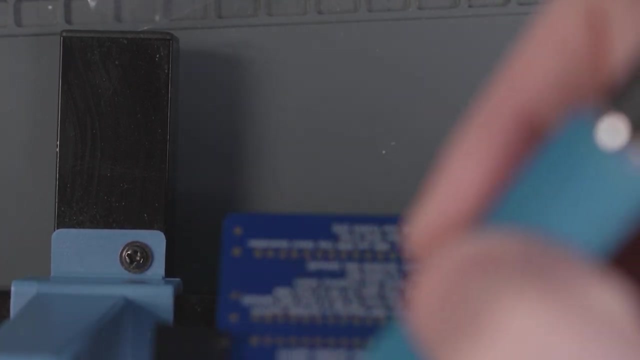 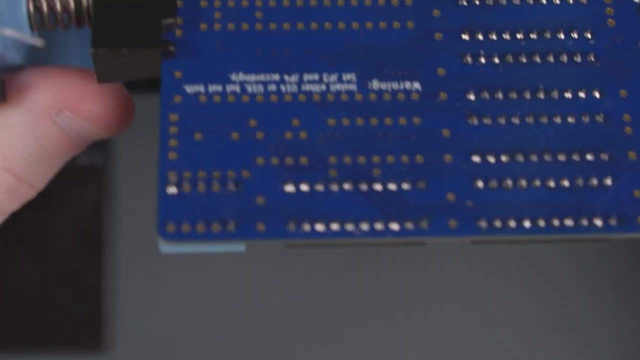 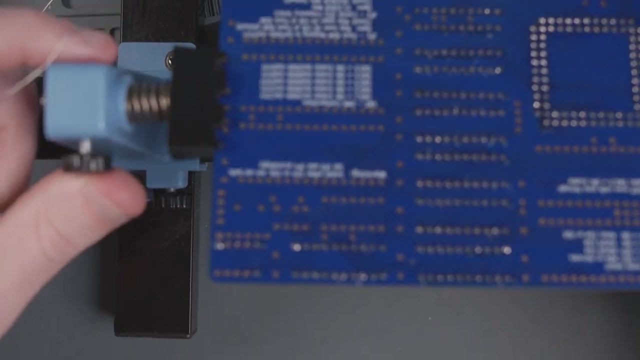 this started and then we could play around with it. maybe not can't really do it anything with it yet. oops, you guys can't see that at all. my bad, it's hard when i tilt this thing down. i can't really tell um what is in focus or not. 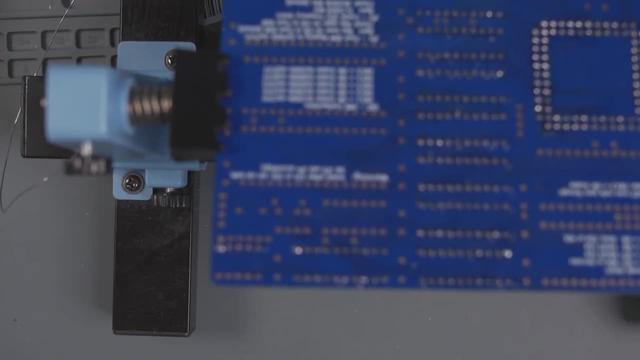 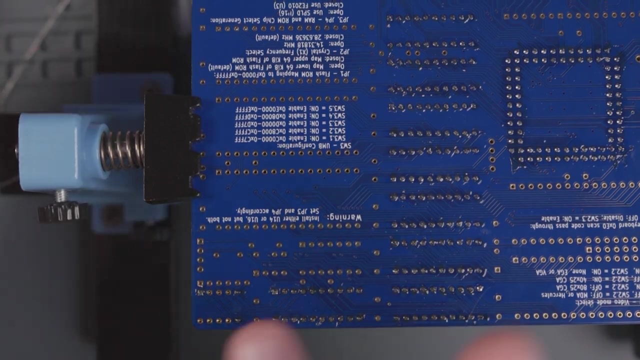 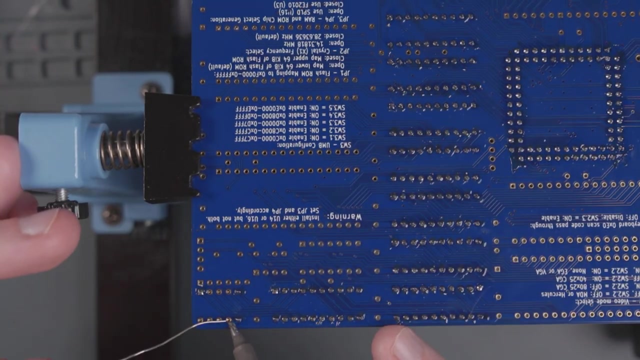 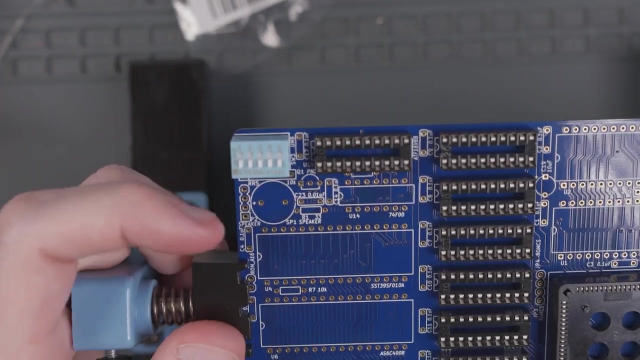 mostly because i should put this up here. yeah, there we go. mostly because this, this thing rise, raises the the part up and it messes with the minimum focus distance on my camera. cool, all righty. so these, this is a dip switch thing and it is going to be super satisfying to do this. 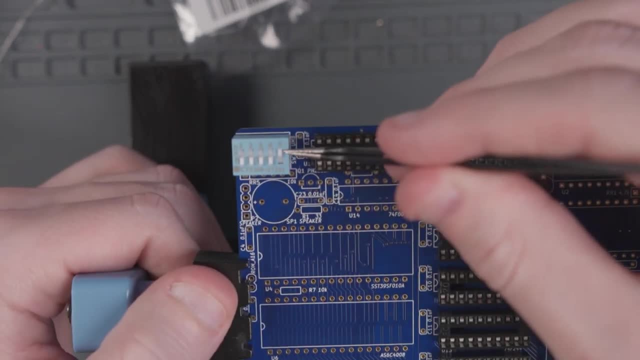 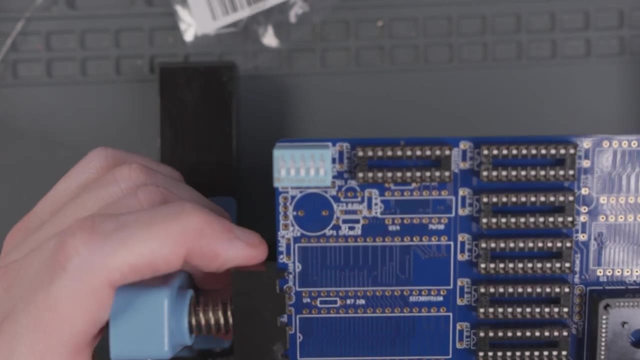 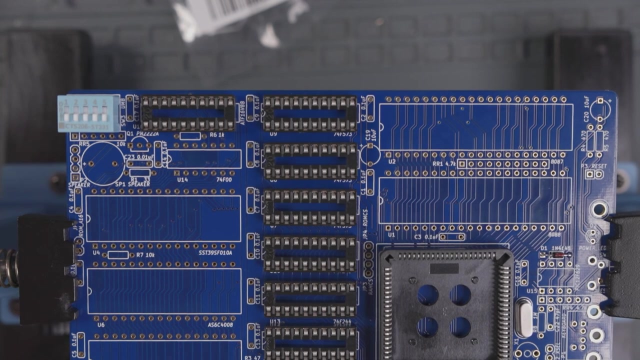 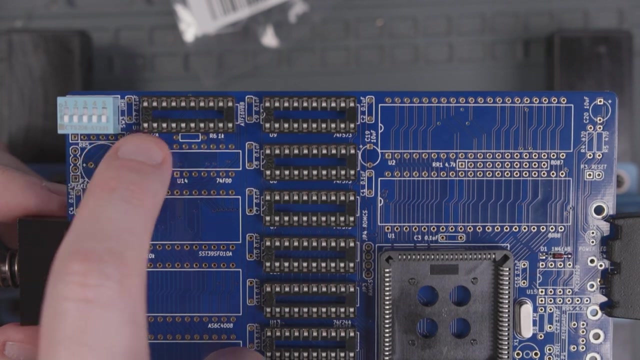 maybe, yeah, sale, yeah, oh, just barely doesn't like to focus. so, anyways, there's a couple of, there's this one here and i don't know what they do yet we'll have to look at the manual, um, okay, so, oh, this might be a little bit annoying to solder. um, this is the spacing between these things i might have to be, i'll have. 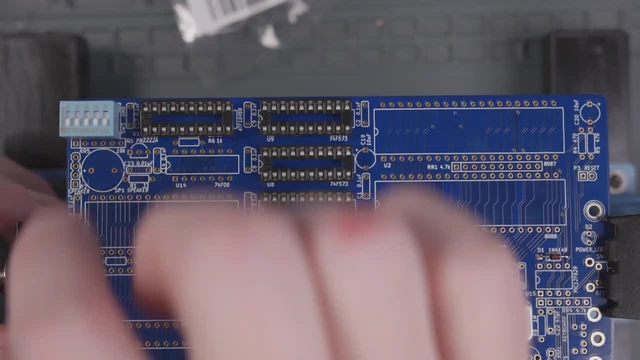 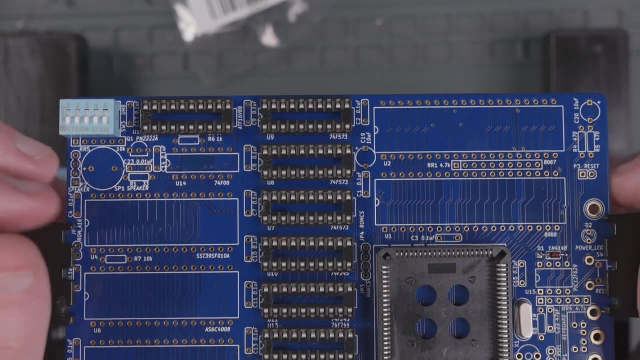 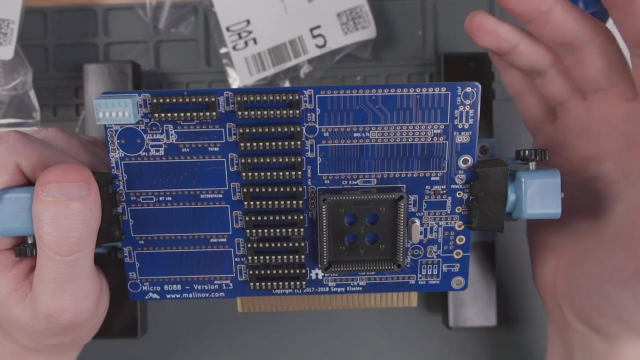 when i, when i continue, so that i'm not like stuck trying to like jam a small part when there's already other stuff all around it, um, all right, well, i think that's where i'm going to end soldering for tonight. i'm going to finish the whole soldering. i. i hope people don't mind that. 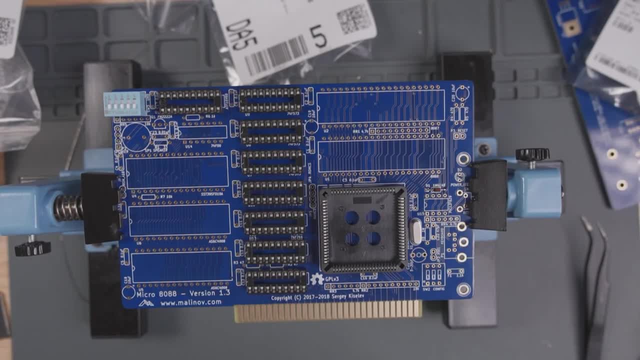 i think you know um. if you want more tips, i do have other videos like open tendo builds. i have a bunch of videos um with that, a bunch of um. yeah, i did the whole step-by-step thing for that entire project. so if you're looking for like soldering tips, um, go watch the open tendo to. 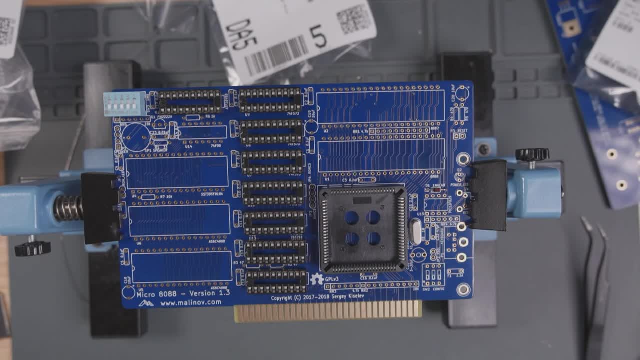 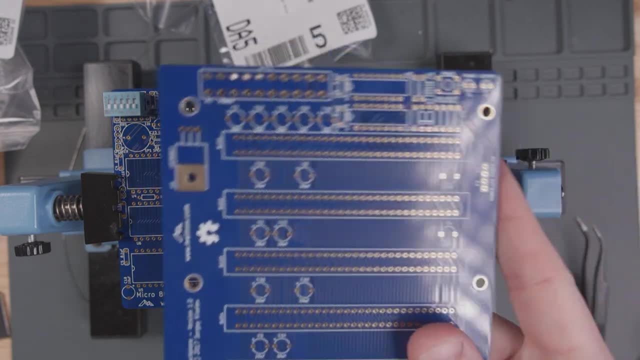 get some more surface um through hole soldering tips and stuff. but next time i will have soldered everything. hopefully i have everything. i hope i have all the build material, stuff. um, i'll have everything soldered and then we can test it up or test it up, and then we can test it up, and then we can test it up and then we can test it up. 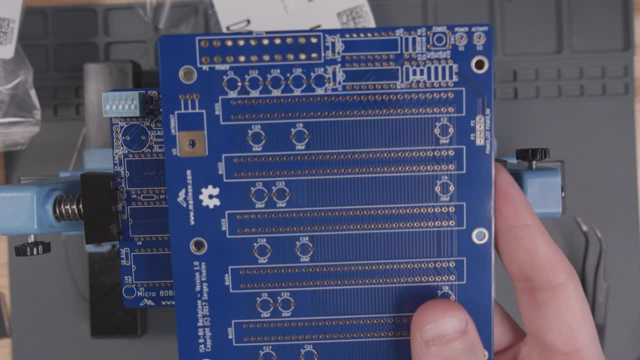 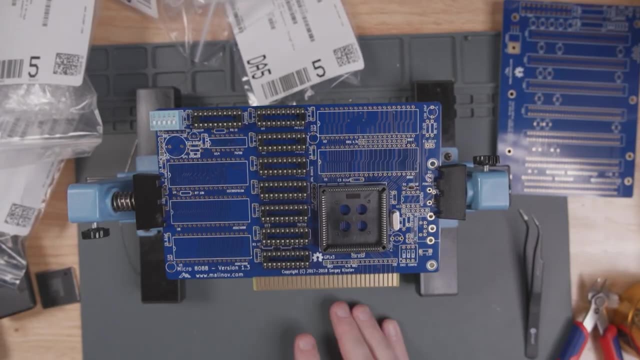 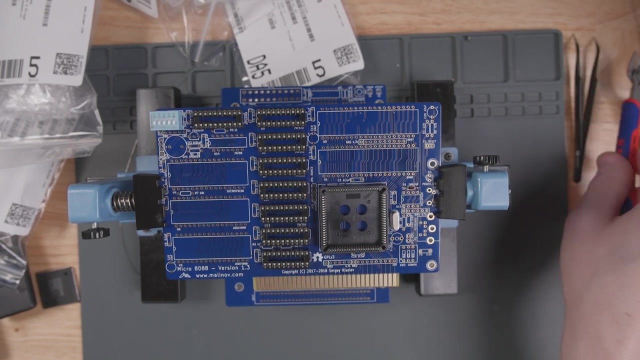 test it, we can boot, try to boot it up and get, get it to work, so that'll be, and then after that, um, that'll be like the end of phase one for the micro build this year. uh, like i said, my long-term goal for this entire year is to build that full computer. so every project that sergey has that is. 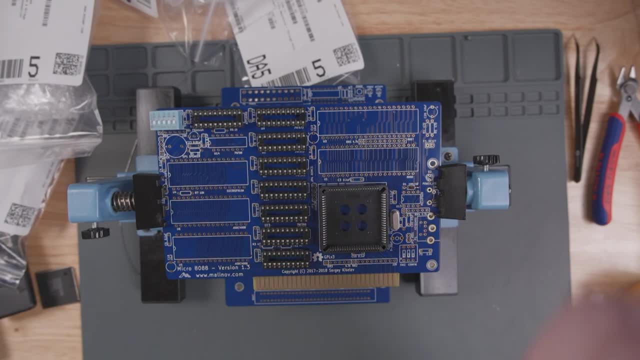 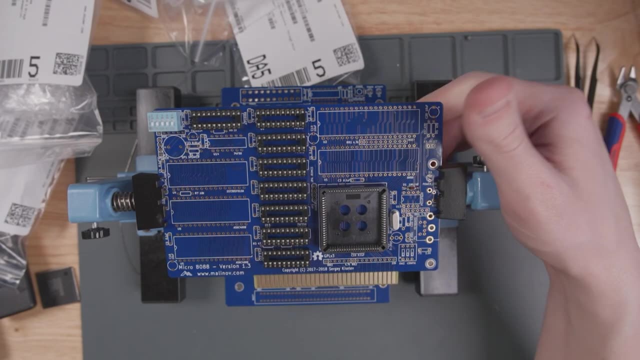 related to it. um, i want to. i want to build the whole thing. so phase one is the cpu in the back plane and the case which i already had. uh, step two is probably going to be- i don't know, i don't have to build the pico psu, but uh, i can't. 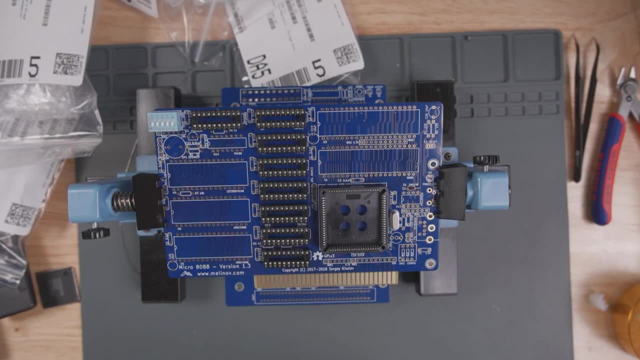 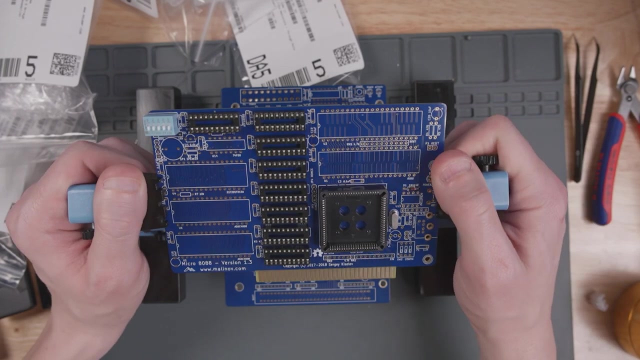 show you my face, because if you weren't here in the beginning that my um iphone isn't working, um, unfortunately, uh, what was i gonna say? step step two, i don't know, maybe it might be the, the pico power supply, but i also want to do like the, maybe like, uh, the sound card. i guess we could use a. 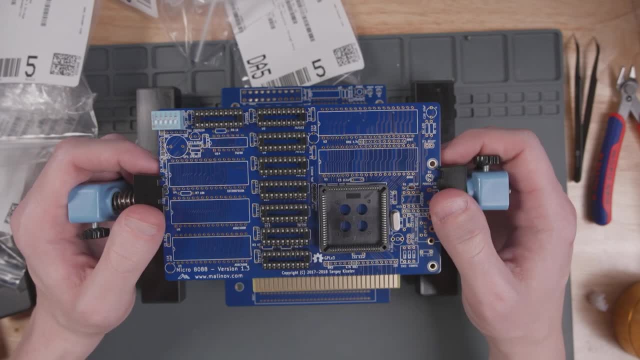 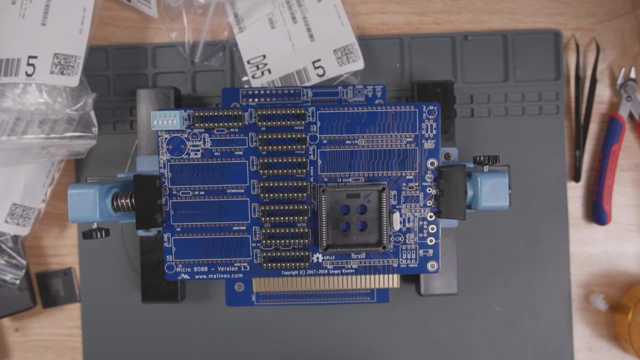 but i kind of want to build sergey's version. so the sound card and maybe the video card will be like step two, and then i think there's a floppy controller and the xtide. maybe that'll be like the third and final phase. so we'll kind of break. 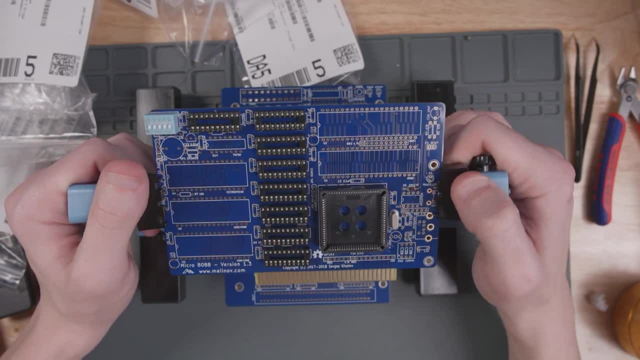 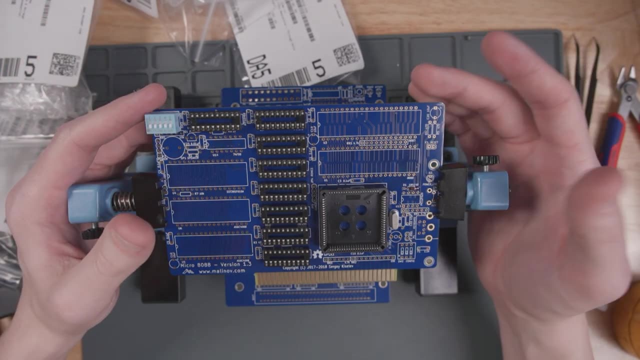 it up like that, uh, so that i can kind of, you know, have the whole build eventually. i hope, i hope you guys found this project interesting. um, you know, let me know, don't, don't let me know if you found it was terrible. but, uh, you know, let me know if it was interesting, because you know, i think it's. 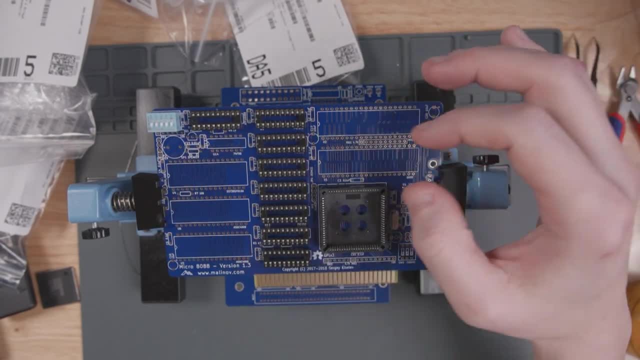 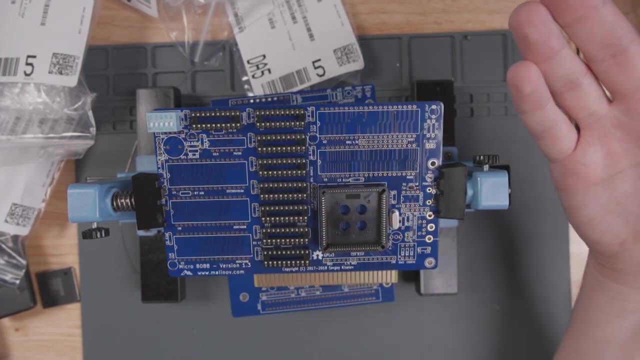 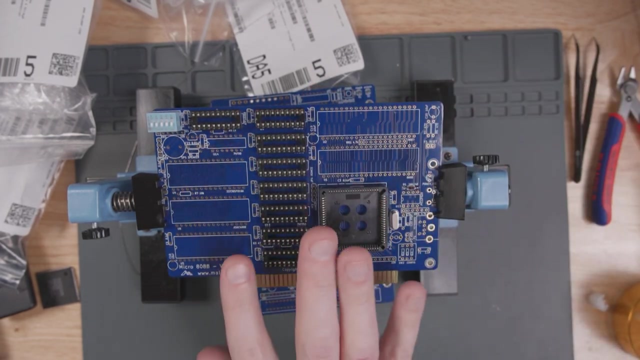 i look out for this stuff all the time, um, kind of on twitter and stuff. i- and just in my searchings for computer stuff or retro stuff, i want to look for projects like this and in my opinion this is kind of like not this, this exact project, but projects like this i think are going to be. 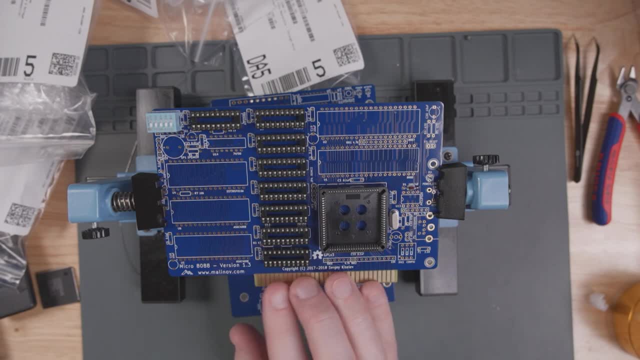 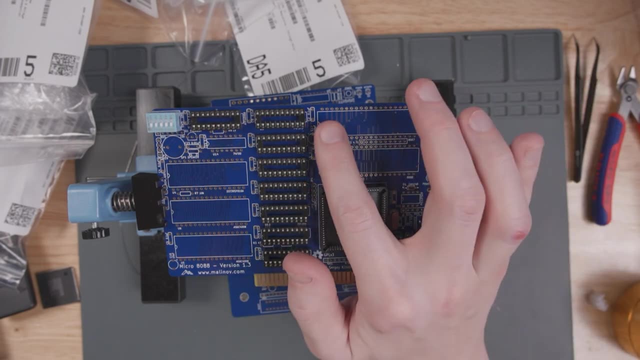 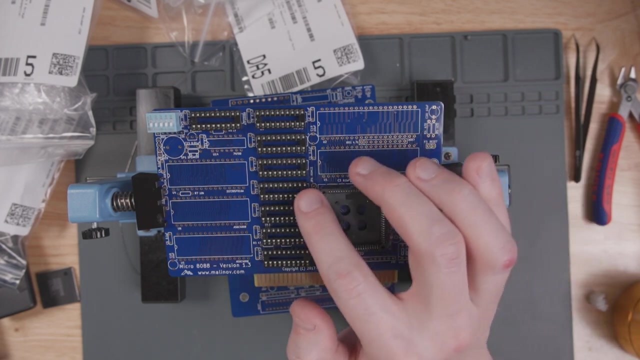 you know i i hope they'll be like the future of retro computing for for new people. i hope that. you know. i think they still make the cpus and stuff nowadays, but i hope we can get probably like fpga chipset replacements probably would probably be the easiest way and then that way. 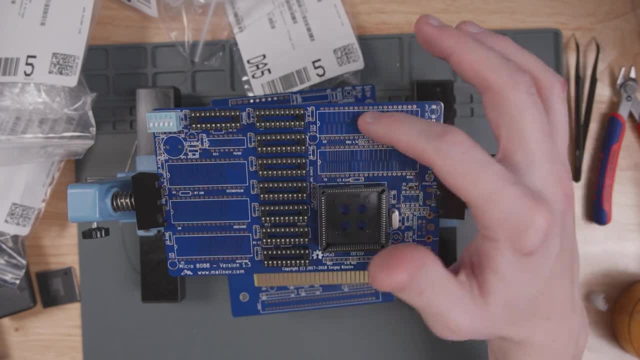 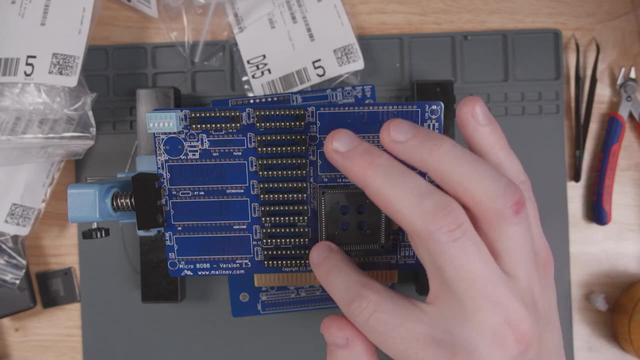 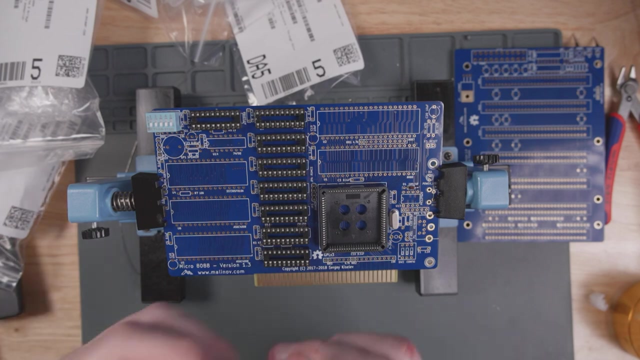 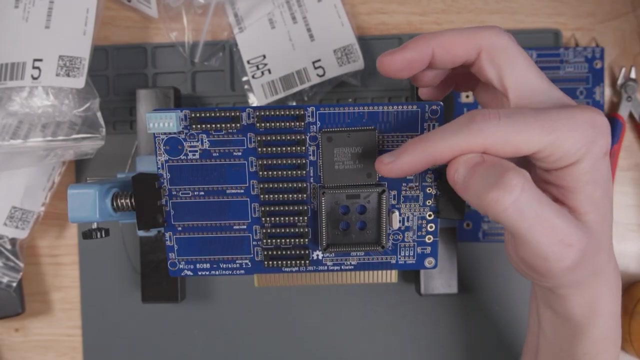 people can have brand, nearly brand new. i know they make the cpus brand new still, but they might be pricey. um, but you're still relying on this, getting this specific fairday chipset, uh chip, which you know they're probably not going to be available forever. i don't know how many they made, but, um, yeah, so if we had, you know, fpga. 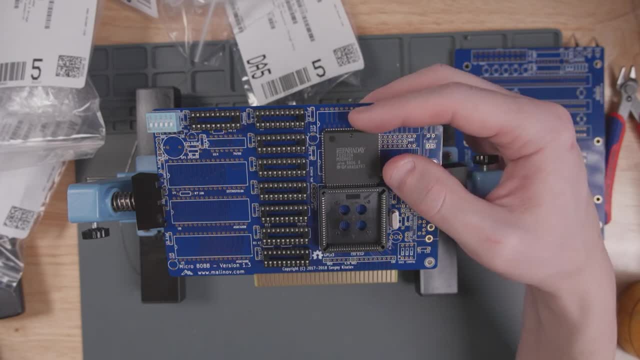 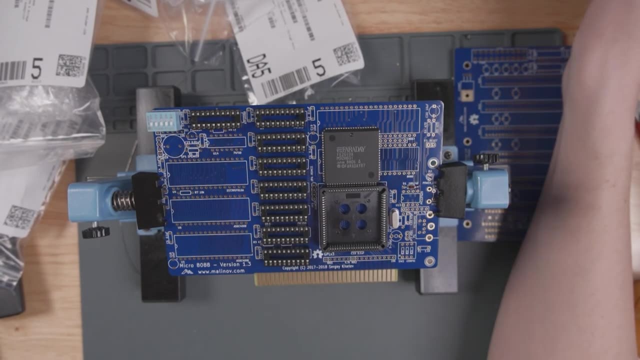 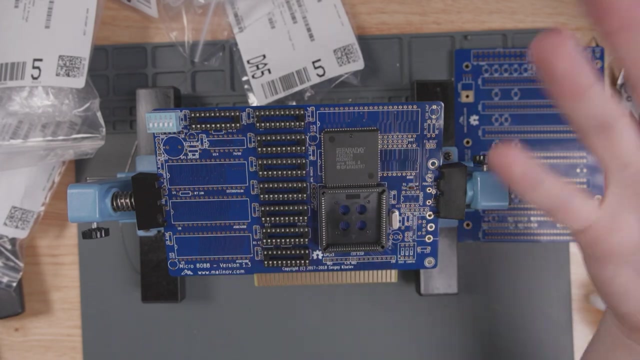 replacement for this chip or something, then i would feel a lot better about this project just existing into the next 10, 20, 30 years. so stuff like that will be cool, so like people could collect these kind of small form factor. but you know, trying to be trying to be, you know, authentic. 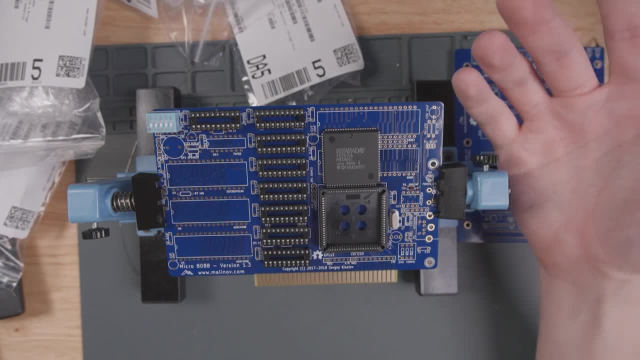 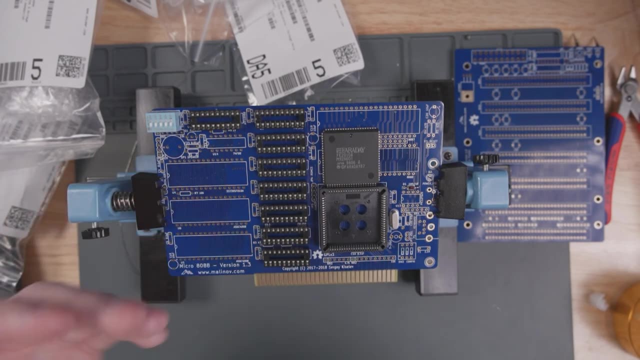 in the same way where you're not like really emulating it. i mean, you know, i'm not talking about like hardware emulation, i'm talking about like software emulation, like dos box, i guess, um, but having the hardware to tinker with and it's not really too much, it's not too far off. 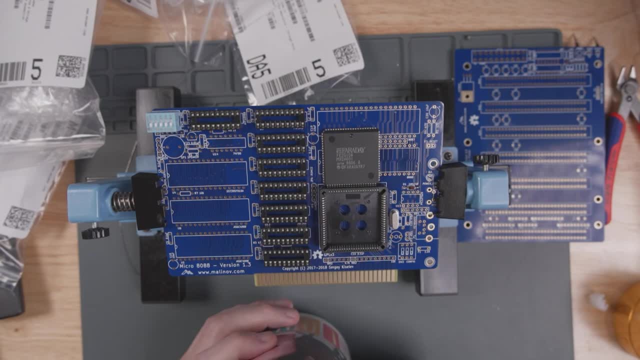 from the original experience. right, if you use something like dos box to try to launch a game or something, you don't get any of the, the the pain and or pleasure of loading it from dos and you know configuring your sound card, and then you know all that stuff, all that stuff which is 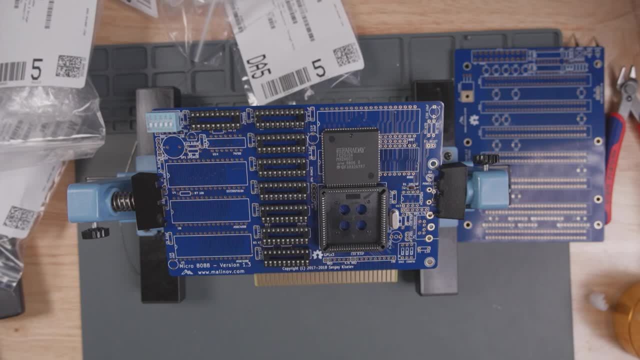 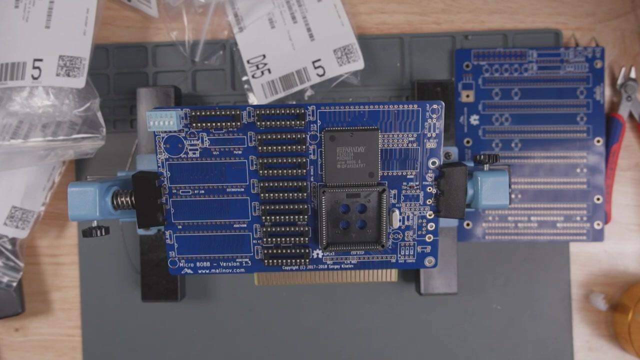 you know part of the original experience, so, all right. well, that's pretty much it. uh, i don't know if anybody here probably cares. i'll probably wait to hold my comments about the. uh, this is better than. oh, hey, mike, this is better than kasumi in the best swimsuit, yeah, uh, so, yeah, i'm excited to finish this, so, anyways, next project. 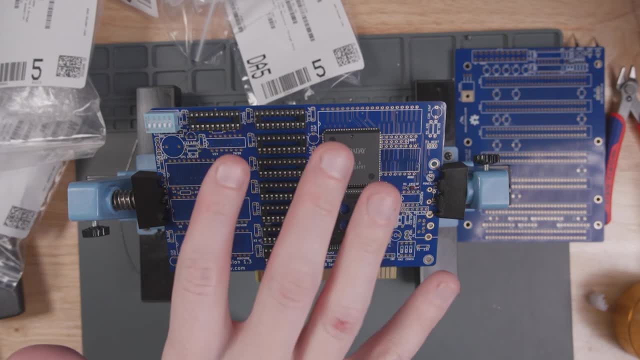 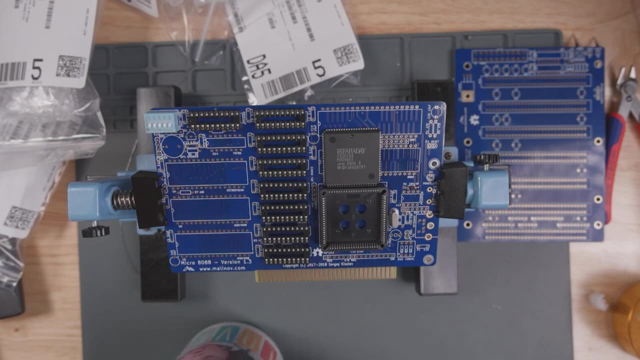 or next stream will be probably the follow-up slash trying to get it to boot slash, the end of the phase one of this uh. and then i'm not really sure, i, i guess i i still have the, the uh oss pro, and i do have to give that back soon ish. so i know people. 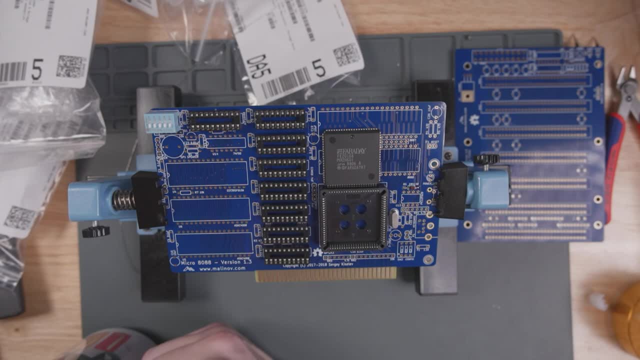 probably still want to see more footage of the morph, right especially after um. you know voltar, you know i wouldn't say that he like destroyed it. um, i did watch, you know some of it. the beginning of it i didn't say like he was like being- uh, what you might expect- like completely negative. i don't. 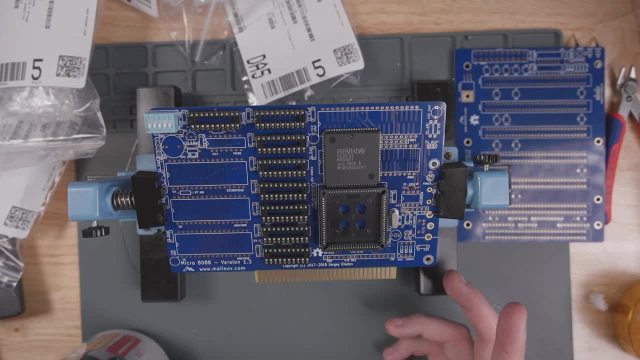 think it was really that um kind of video, so it's really just kind of finding the, the weird things that don't work. really, that's kind of what i'm trying to do now is test, test things that are not just hard to test, really. i mean not just hard to test, but i'm trying to test things that are 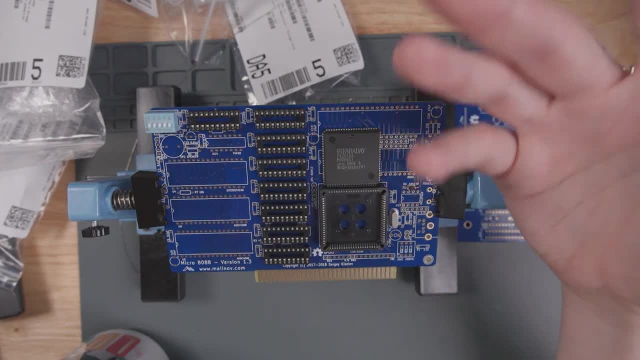 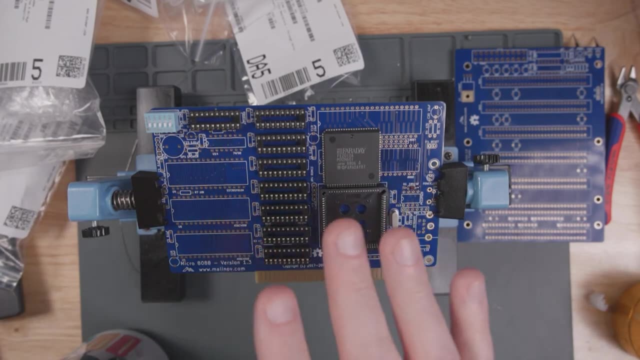 even. you know, i don't know if i'll go to the level of being able to, you know, test the hard stuff, but like being able to test stuff where if i had, if you had, a comparison with one of the other scalers readily available. that's what i'm kind of set up to do. so, um, all right, i've been rambling, thanks. 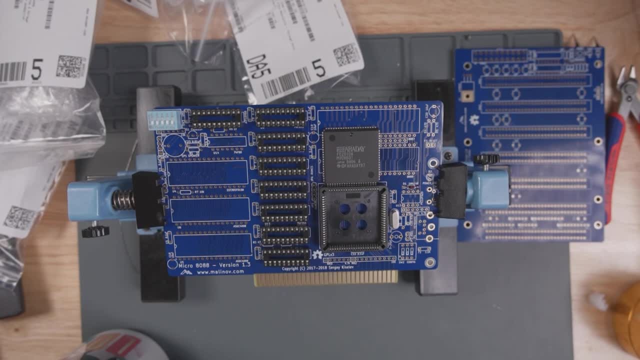 everybody for watching. uh, we'll see you back on sunday for the completed build. oh, i just imagined projects like this and the open tendo, just all slotting into one big x-tron so you can just toggle between. yeah, i mean, that's a cool, that's a cool idea. i mean you'd have to figure out like a, a standard, you know. 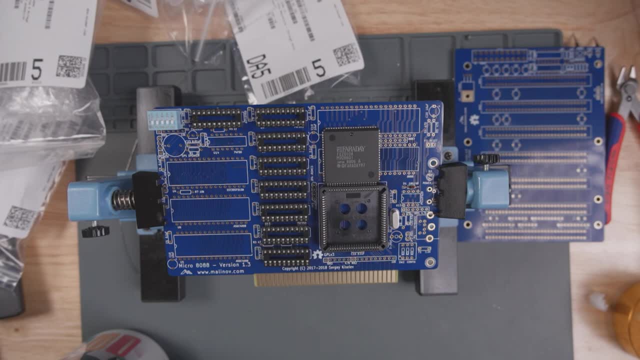 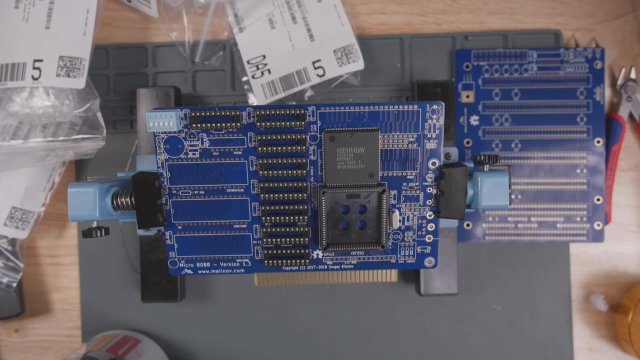 interface, some kind of, uh, analog bus or something. yeah, that'd be cool so you could have like a instead of instead of um. yeah, i mean, imagine an entire computer that is just you slot, you sock it onto like a weird vga backplane or something and like everything that you put is: 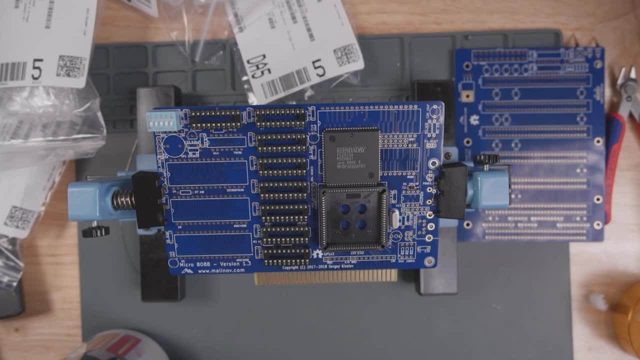 into a rgb or vga backplane and just switch it that way. that'd be. that's a cool idea. all right, thanks everybody. we will see you on sunday with uh part two.